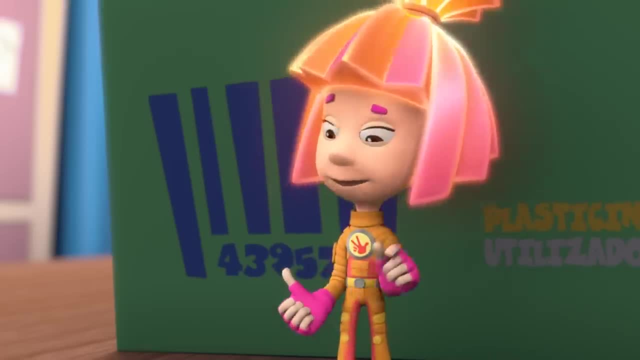 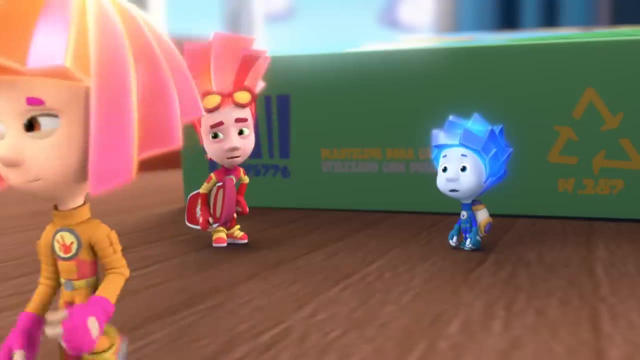 Yeah, Like what? Well? a bathroom hook fell down. Tom Thomas broke the lamp on his desk. the aquarium has a tube that's leaking, so go and play. I have to get a pack-o-mat, Oh-oh-oh. 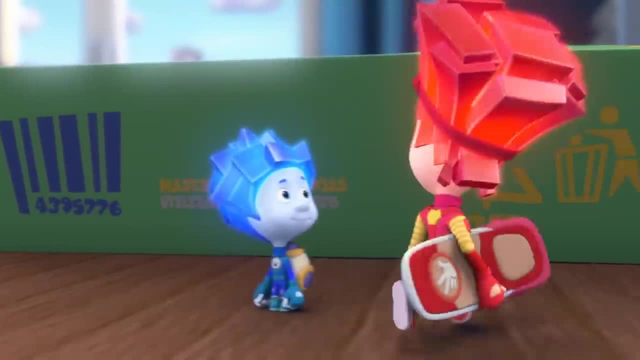 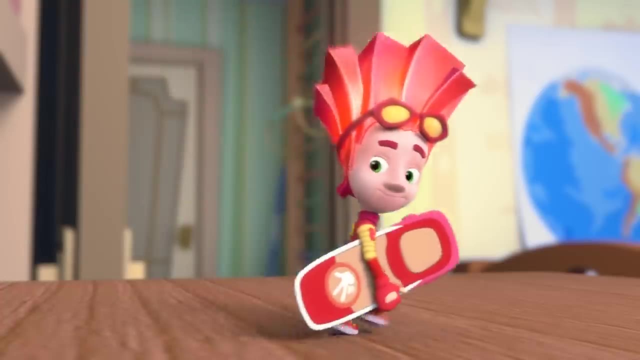 I wish I could play tag Hold on. Nolik, you found a pack-o-mat, Uh-huh, Although I gotta say it looks a little strange. That's because it's…. Let's fix everything before starting, Mr Simka, with your pack-o-mat and my Fixie Board. 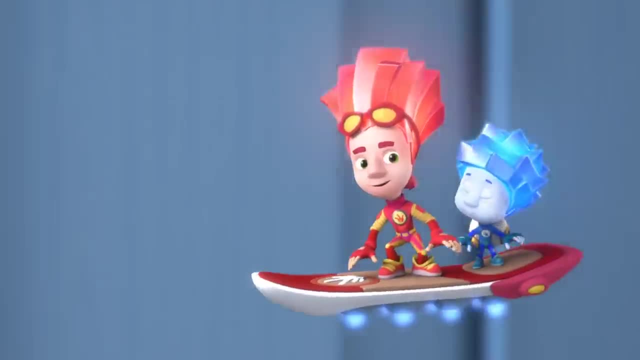 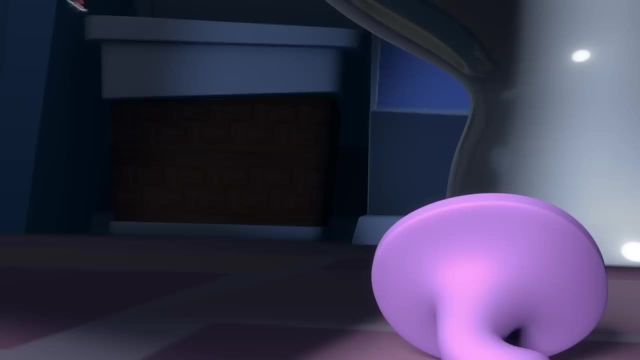 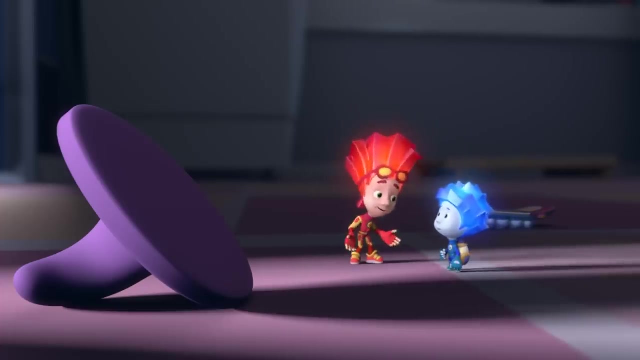 This will be great. So where is that hook that fell down? Alright, Nolik, get out some sticky stuff From where? Obviously from out of your pack-o-mat, But it isn't real. I made it out of modeling clay today. 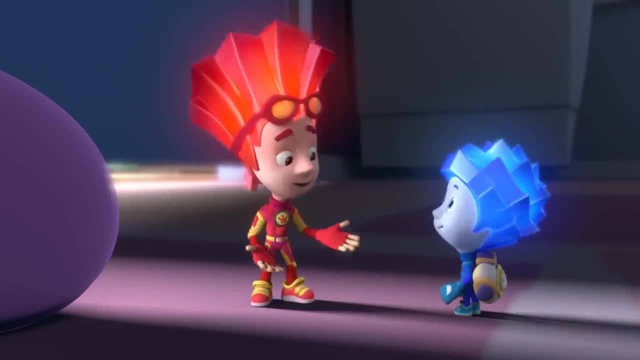 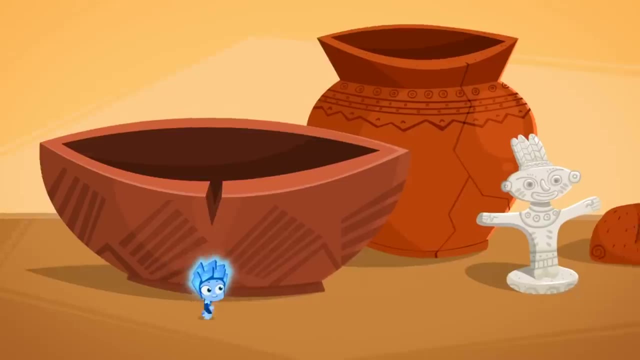 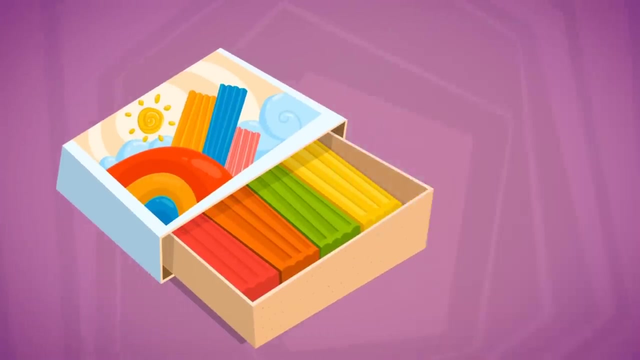 Out of clay. Well, it totally looks real. Now let's take a look Long ago, back in the Stone Age, people learned how to use clay to make their dishes and sculptures, But the modeling clay that we use nowadays was only invented about 100 years ago. 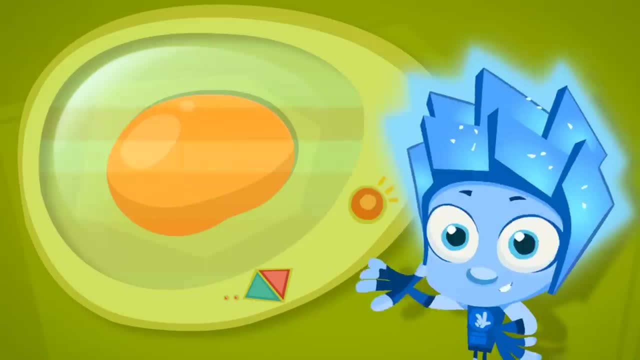 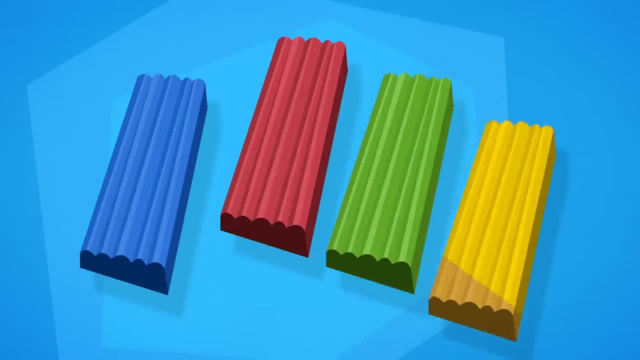 Actually, modeling clay is just plain old clay with some ingredients added so it won't dry out, And dyes are mixed in to make all the different colors. There is just no end to all of the fun things you can make out of modeling clay. 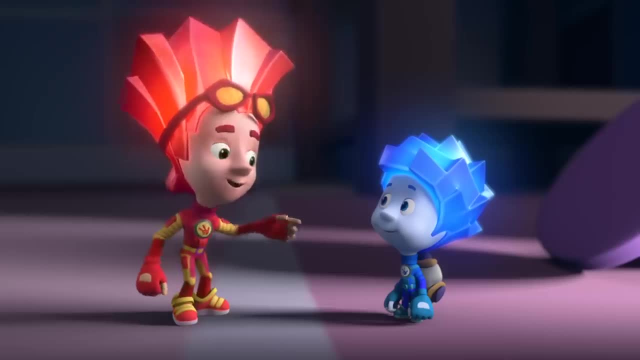 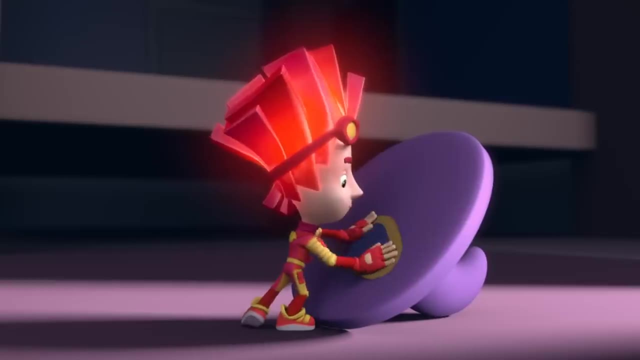 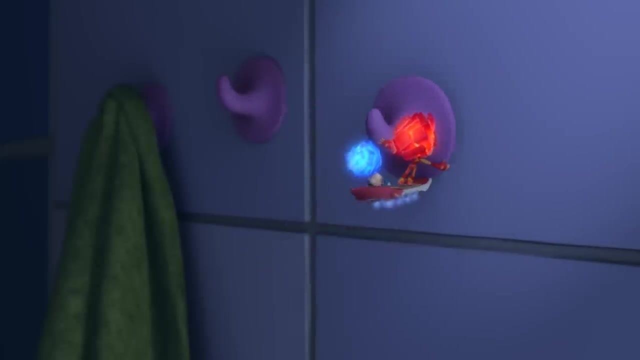 I got an idea. Go on, turn around. What are you doing? Grabbing glue Out of your pack-o-mat? All right, get up here. Will it stick? Yeah, of course it will. Let's go and fix the lamp. 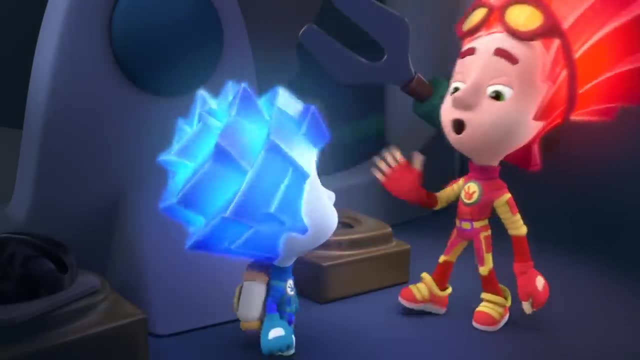 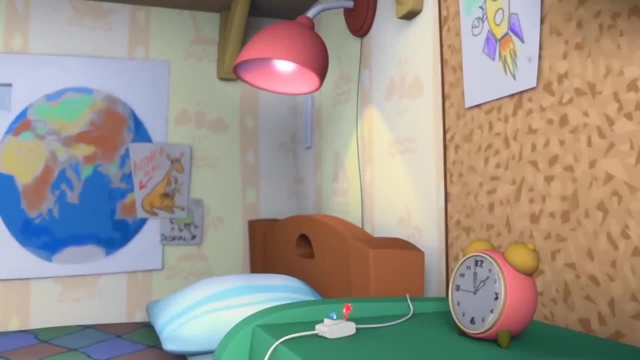 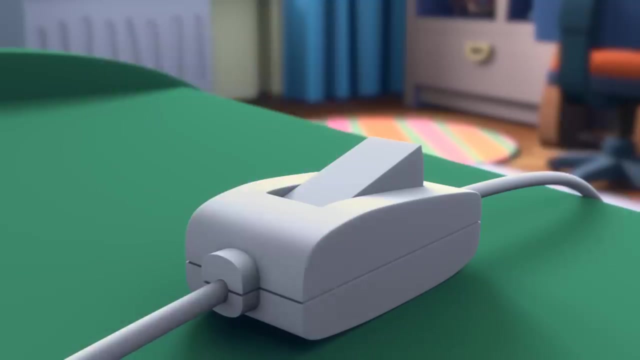 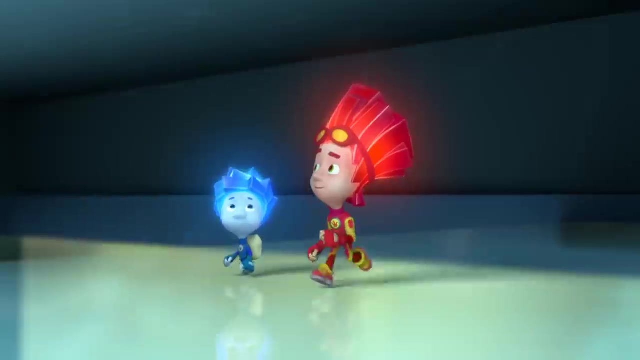 We can't fix this without a real pack-o-mat. Yours will work just fine, Tideesh. So what else did Simka have to fix The aquarium? Hop on. Well, where's that leaky tube? Here, It's lying down there. 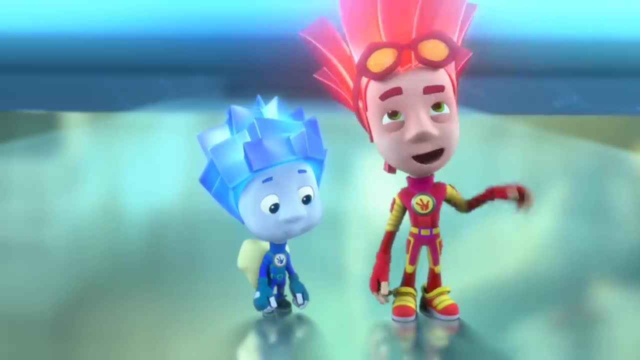 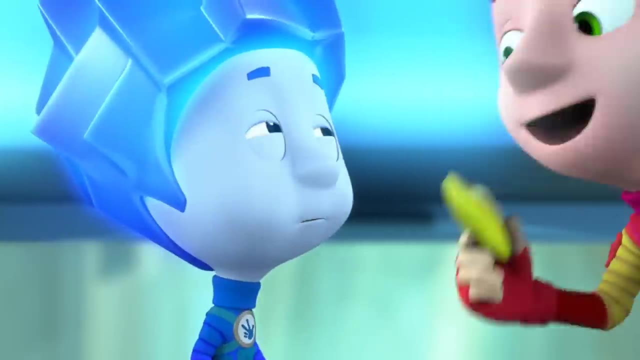 It's lying down there. It's lying down there. It's leaking at the joint. Yeah, this tube is going to need a lot of modeling clay. Give me the rest of your Pac-O-Mat Sure And here's a souvenir. 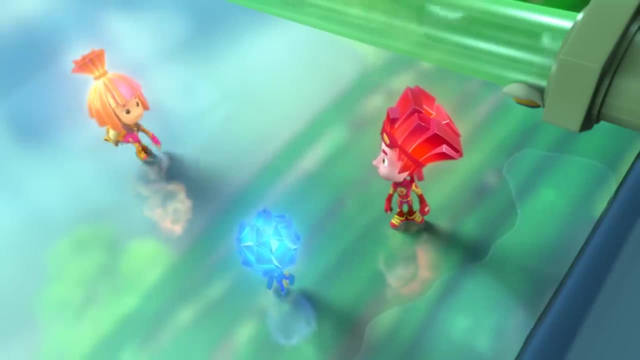 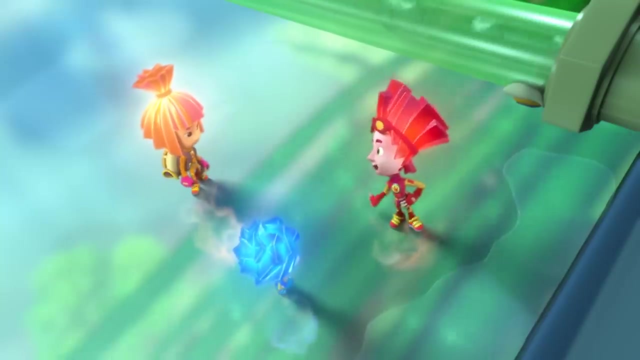 There. all done, What's all done. We already fixed everything. And what did you fix it with Modeling clay. Modeling clay isn't going to hold anything. Well, I say it will. Wanna bet. Alright, Let's see if it works. 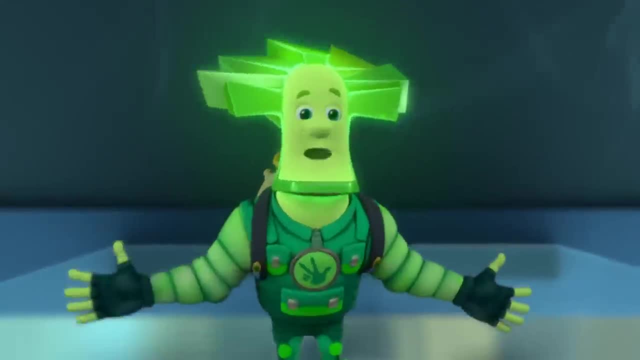 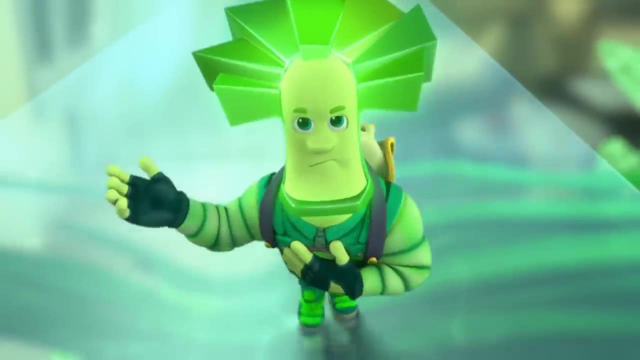 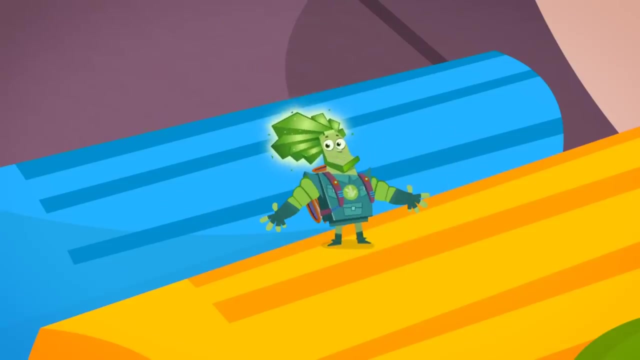 Ah, It's exploding. What in the world is happening here? Flooding water. You just do as I tell you without panicking. Did you know it's possible to make modeling clay in your own home? Just write down this recipe. 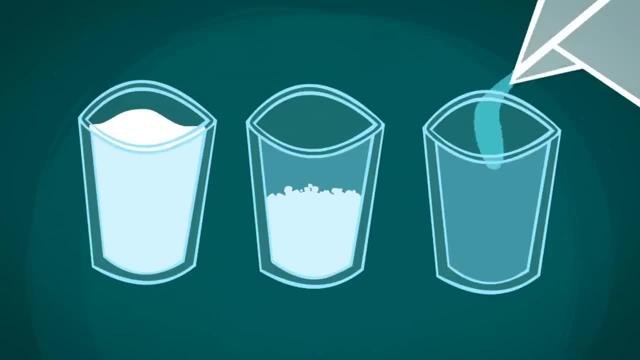 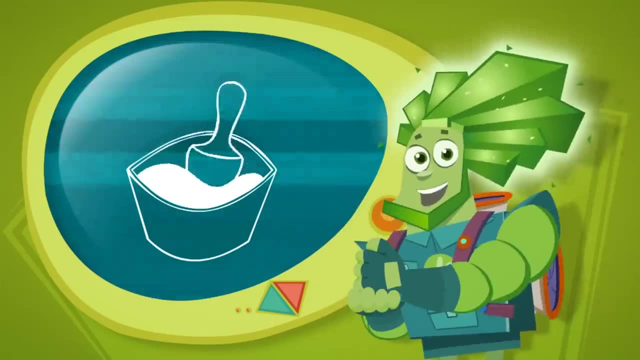 You'll need a cup of flour, a half a cup of salt and a half a cup of water. Now mix the salt with the flour and add the water little by little. Mix it together really well. What are you saying That? it looks just like dough. 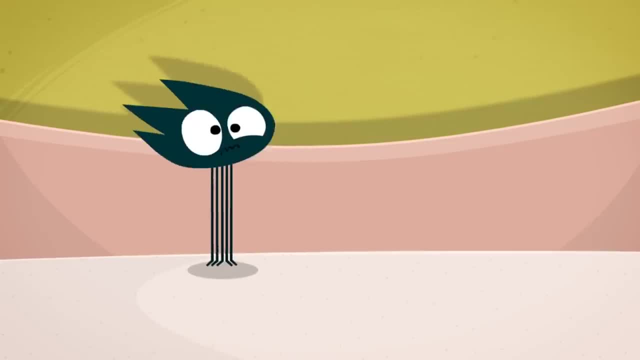 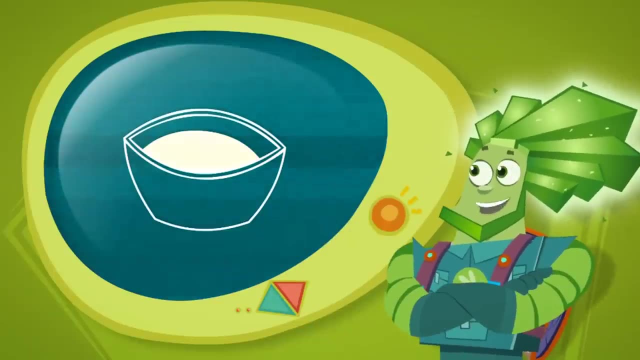 Well, that's exactly what it is. It's just not for eating. It's way too salty, But you certainly can sculpt things out of it. If you want your modeling clay to be colorful, you can add food coloring or watercolors to it. 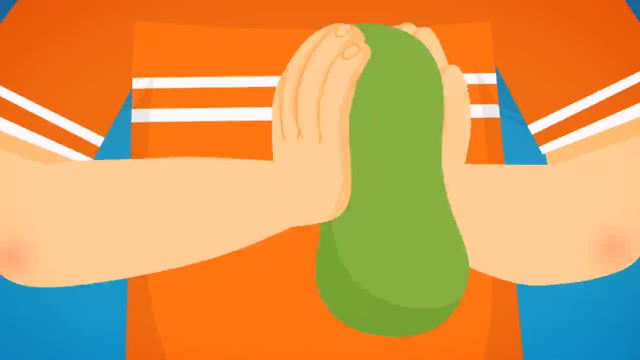 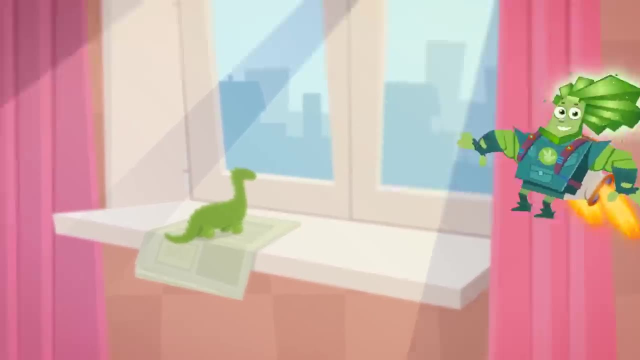 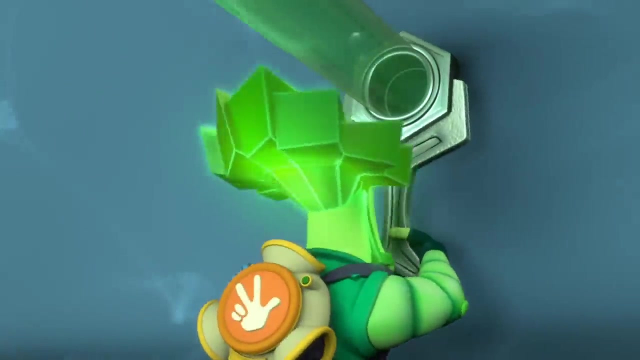 That's it. Your modeling clay is ready to be sculpted. When you're finished, don't forget to let your figures dry in the sun. That way they'll get nice and hard and last you a very long time. We almost didn't make it. 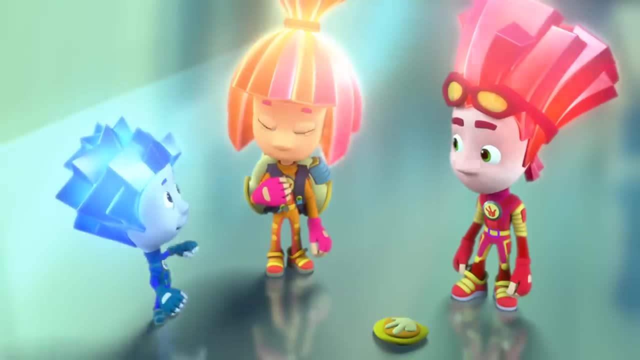 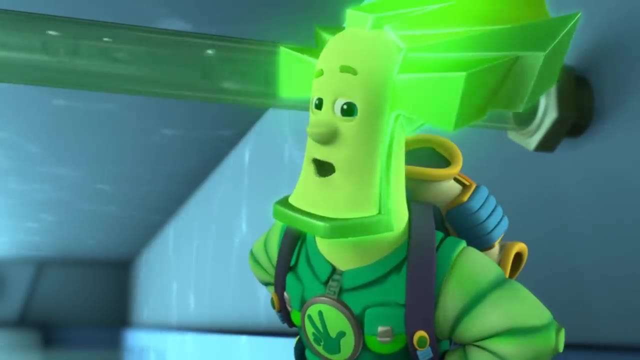 And did you fix the lamp with that modeling clay, Uh-huh, And the hook too. That was not a good idea, But it was really quick. Hey, that's true. That's why I want to give a medal to you. 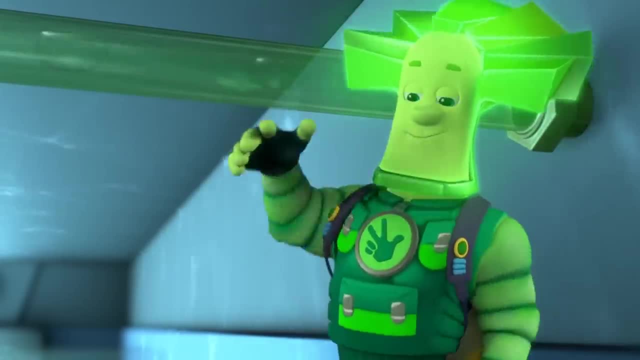 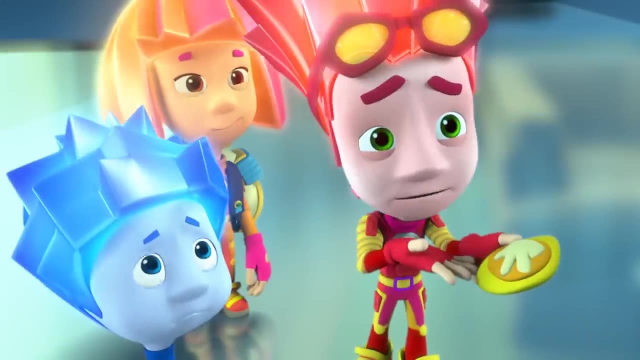 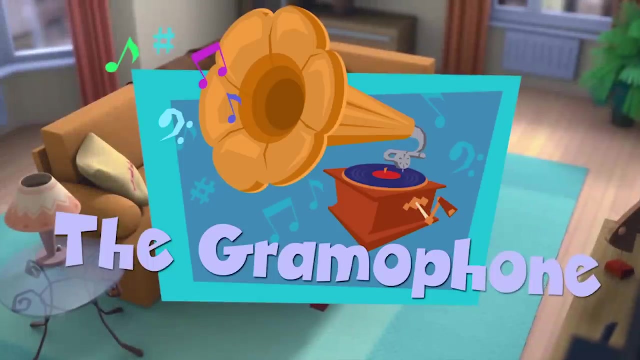 You're heroes For real? Of course you are, And here it is Your medal, But it's made out of modeling clay. Your reward fits your heroic deed: The Gramophone, And that's a photograph of my mom when she was little. 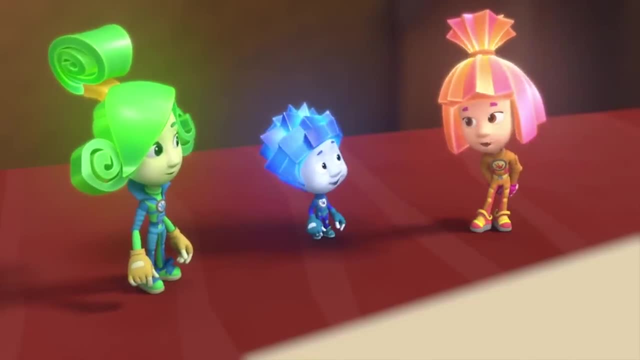 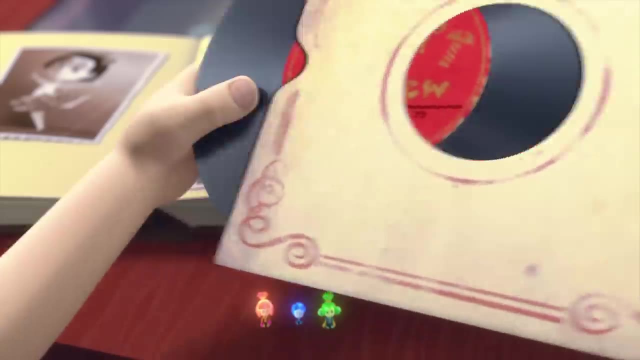 She sure looked happy, didn't she? Because parents were all happy when they were children, But then they grow up and start getting all gloomy and as boring as can be. Oh, what's this? do you know? A song about a screw. 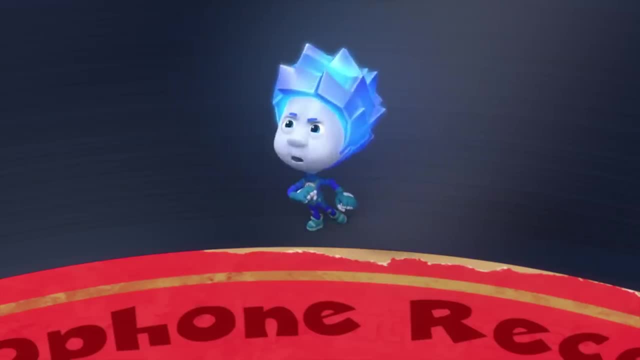 It's total nonsense. Nonsense. It's about a screw, Which means it's practically about Fixies. Why don't we listen to it and find out? If it's good, we can all dance together? How do you listen to this thing Like this? 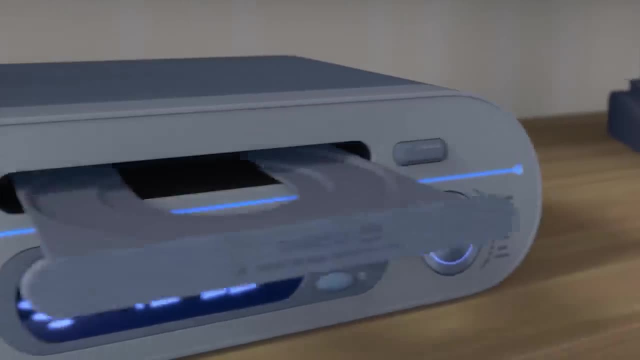 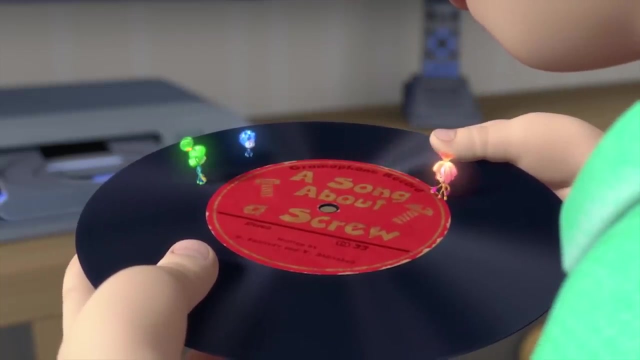 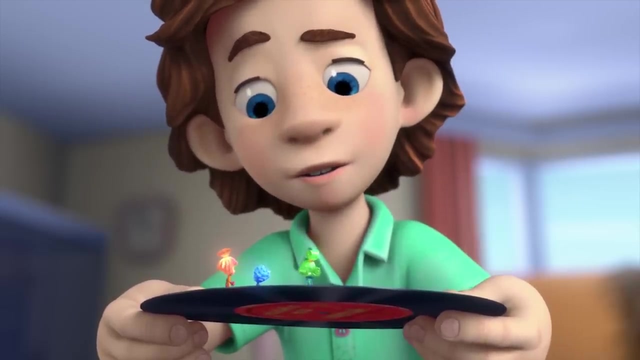 Why don't we try to use the player? It won't fit in there. Look, Right here it says Gramophone record. See, So we need to find a Gramophone player. Find what? Let's go to. Grandpus, Grandpus, we found a song about a screw. we want to hear. 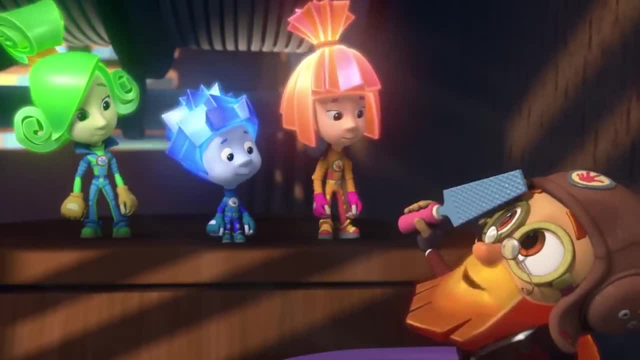 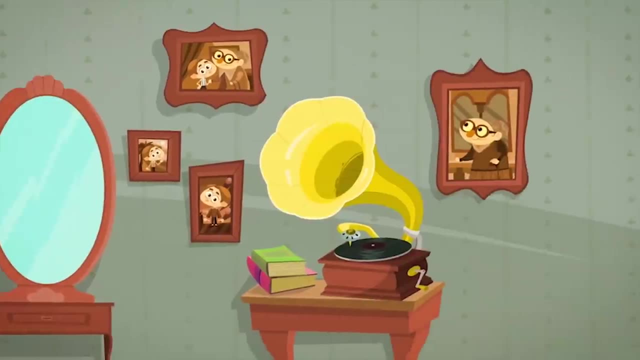 We're looking for a player for a Gramophone record. Ah, I understand. What you need is a Gramophone. A Gramophone is an old aplomb. It's an appliance that was made for playing back sound that was recorded onto records. 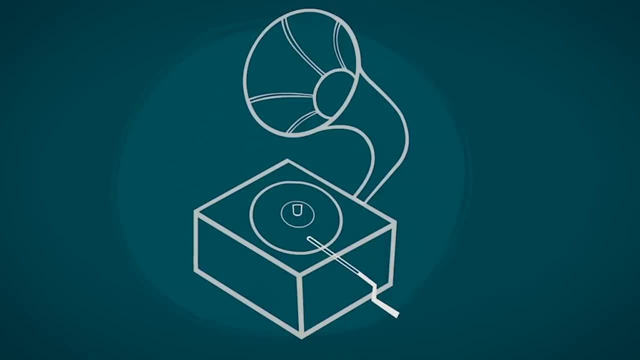 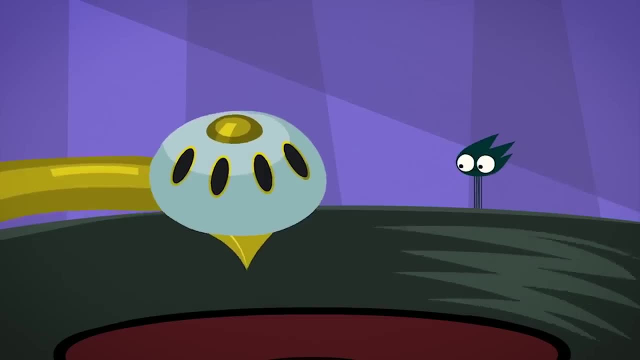 If you want to turn on a Gramophone you need to turn the handle to wind up its spring. The spring makes the record spin. Then a needle is placed on top of the record And as it moves through the groove on the record, 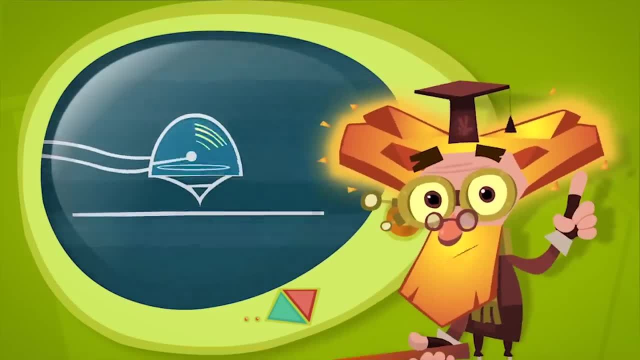 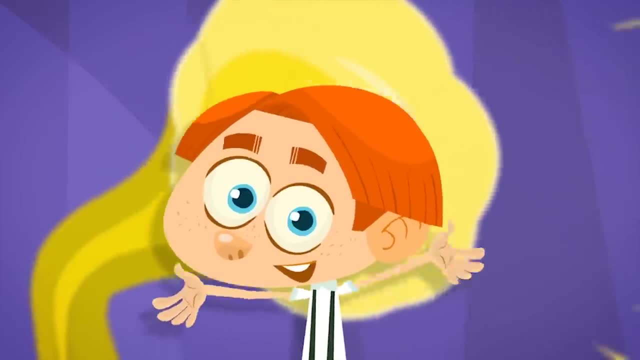 it shakes a little, which makes a diaphragm, a sort of mini drum skin, start to vibrate. The big horn of the Gramophone then makes the sound louder and we hear a voice or music. The most amazing thing is that a Gramophone 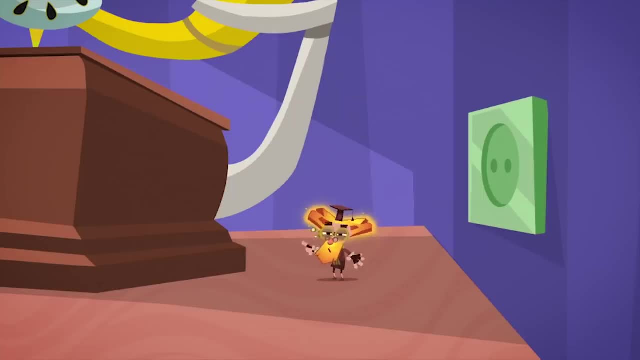 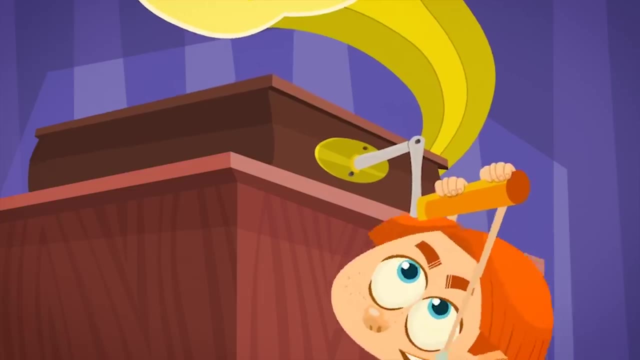 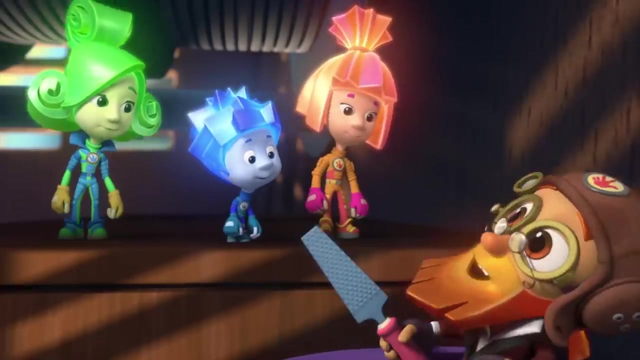 doesn't have an electric motor or any electronics. That's right. You don't need electricity for a Gramophone to play back the sound that's recorded on a record. That's because a Gramophone is an entirely mechanical wonder. If you want to know, there is a Gramophone in the office of Tom Thomas' dad. 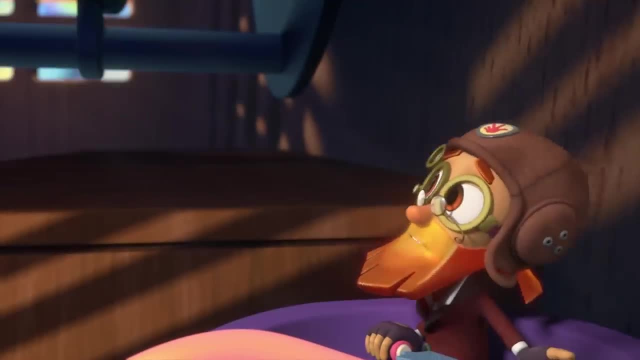 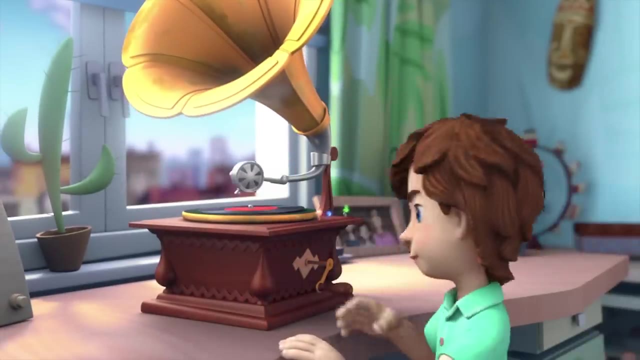 It's on the desk. Great, Let's go. Ha, Thanks, would be nice. I can't find the on button. I can't find the on button. There is no on button. You need to grab that handle and turn it. 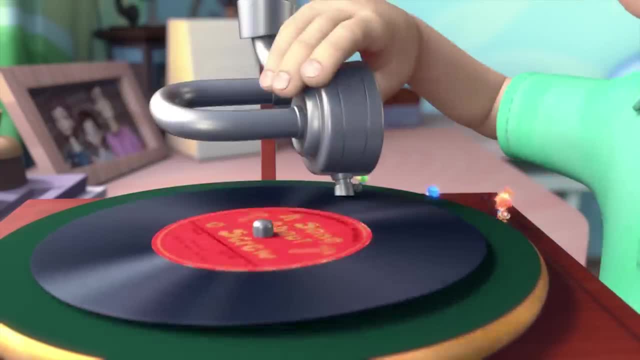 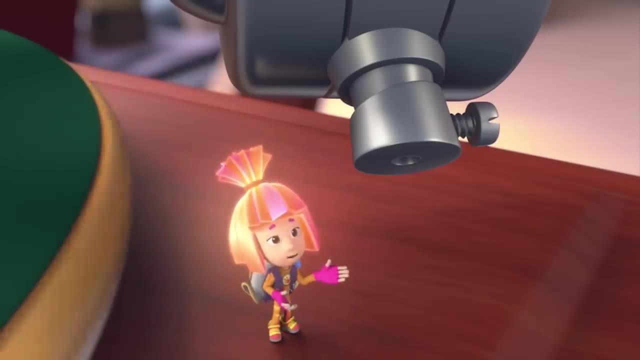 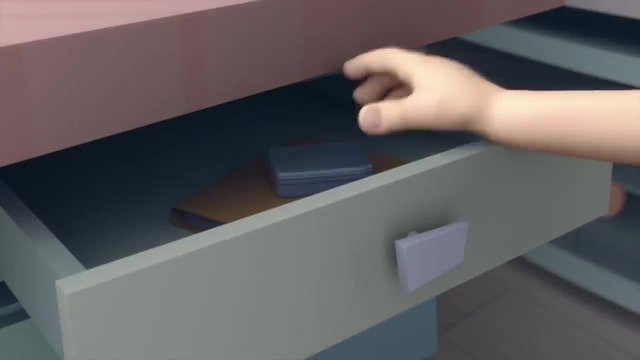 Now take that thing and put it down onto the record. It's not playing. Look, there's no needle in there, And where can we get one from? We can make it. Do you have any nails around here? We can make it. 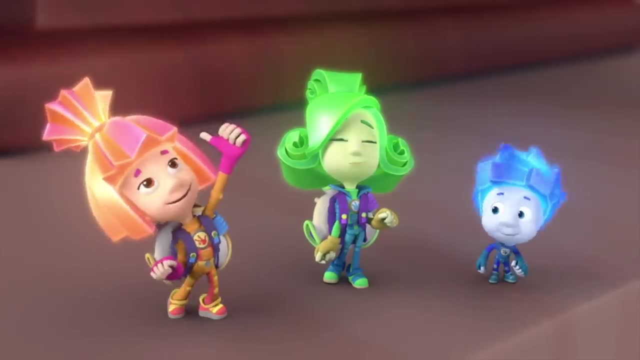 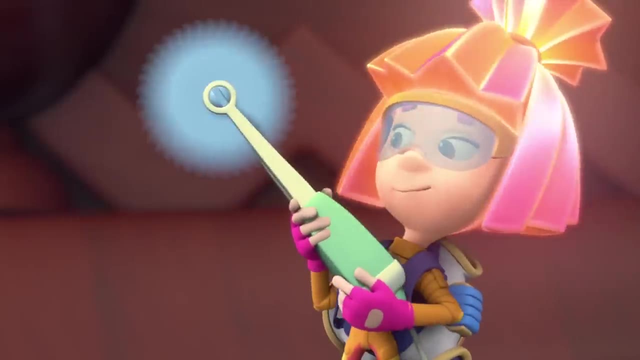 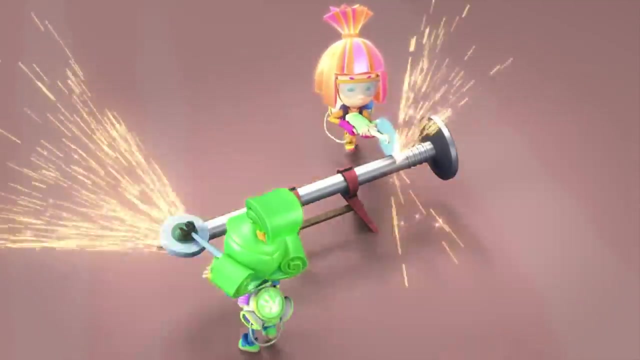 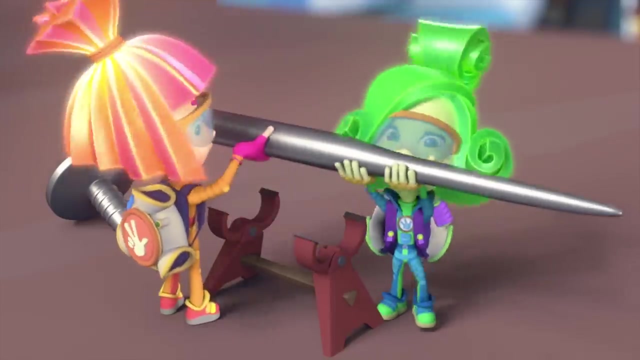 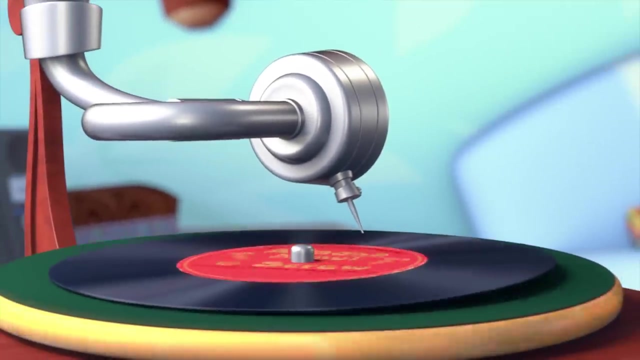 We can make it. Is this good? That'll be great. Verda, are you ready? Totally Better cover your eyes, Tideesh. 5, 4, 3, 2, 1. 5, 4, 3, 2, 1. 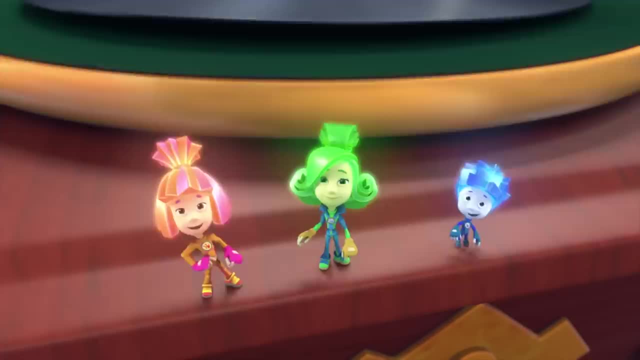 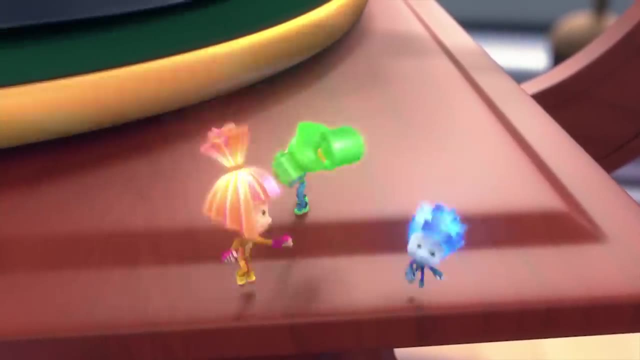 5,, 4,, 3,, 2, 1- It's working. Listen, A little screw went for a run And now, without this little part, Everything just falls apart. If you think a screw is nothing, Take it out, but just beware. 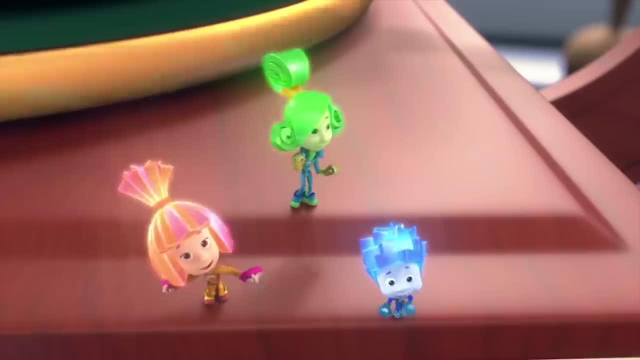 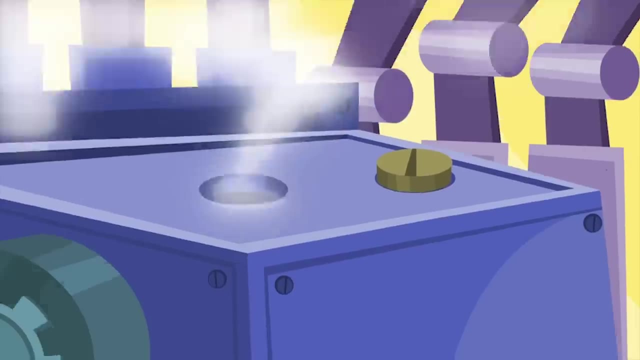 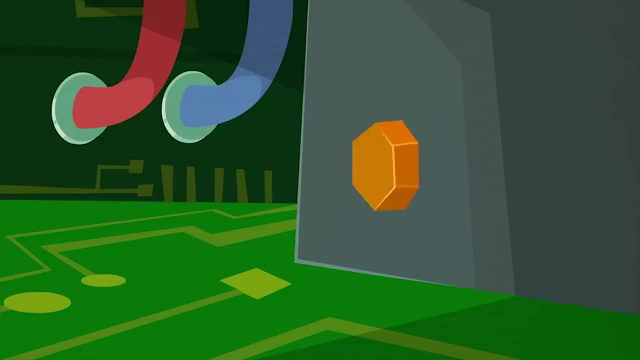 Everything will break without a, With no little screws in there. The bulldozer was a strong one Until there was a throb, And then the mighty giant Fell straight into the mud. 5,, 4,, 3,, 2, 1- A little screw went for a run. 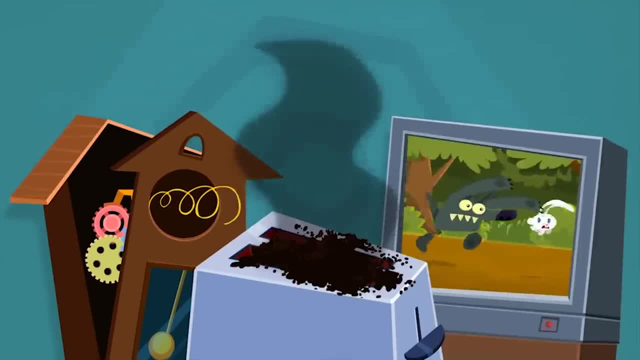 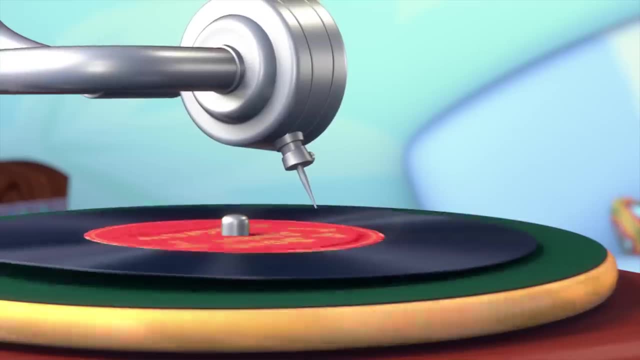 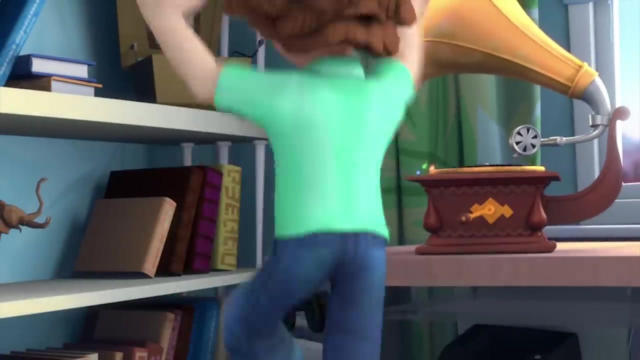 And now, without this little part, Everything just falls apart. If you think a screw is nothing, Take it out, but just beware, Everything will break without a, With no little screws in there. If you think a screw is nothing, Take it out, but just beware, Everything will break without a. 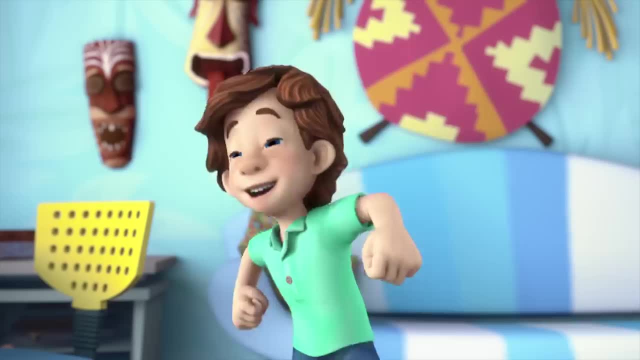 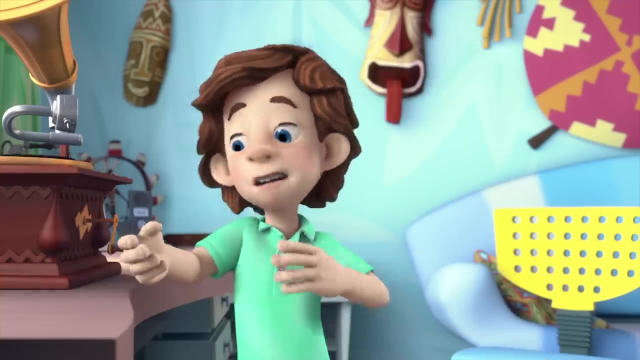 With no little screws in there. Tom Thomas, what's that music playing? It's a gramophone record, A gramophone. I thought it was broken. We fixed this old, Not we, I fixed this thing. Really, What a wonderful boy I've got. 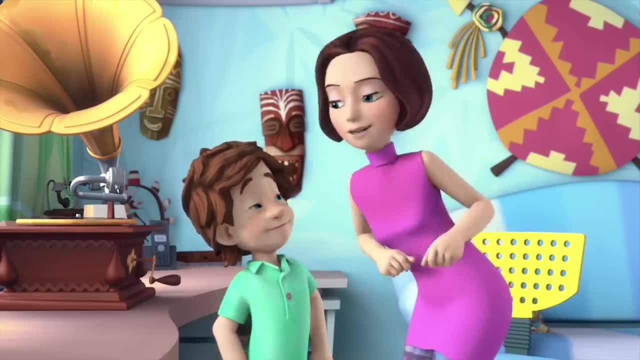 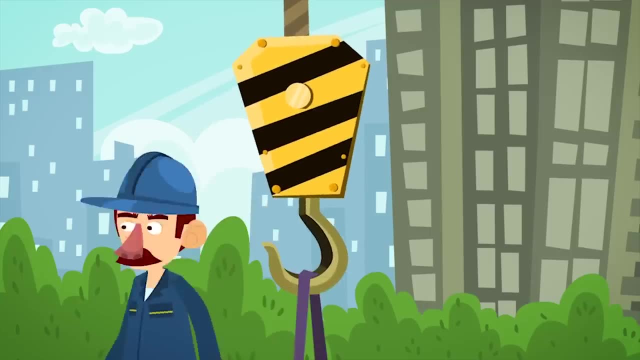 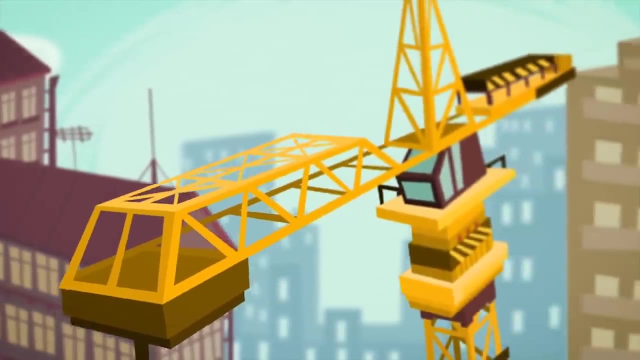 Other kids are breaking things and you fixed them. What do you say? we play that record once more. I used to love it so much when I was little. The mighty crane was working Until there was a pop, And then the mighty giant Gave out and lost its top. 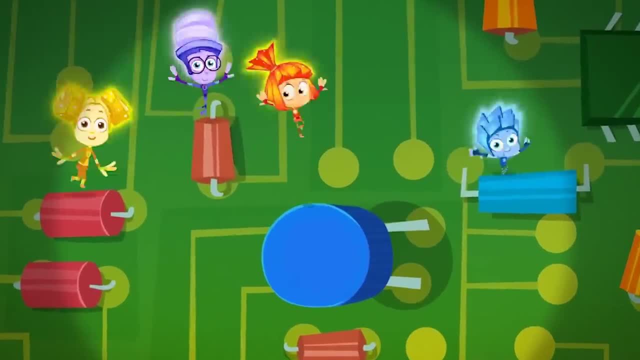 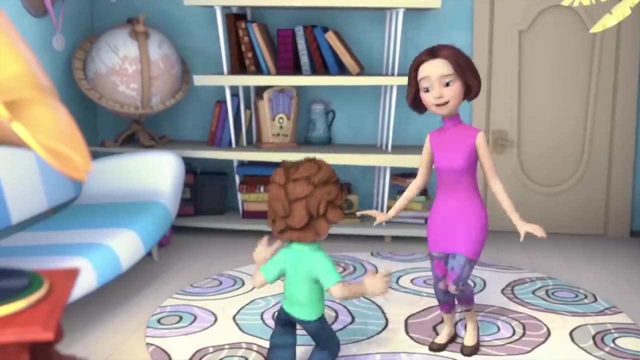 5, 4, 3, 2, 1, 3, 2, 1. A little screw went for a run And now, without this little part, Everything just falls apart. If you think a screw is nothing, Take it out, but just beware. 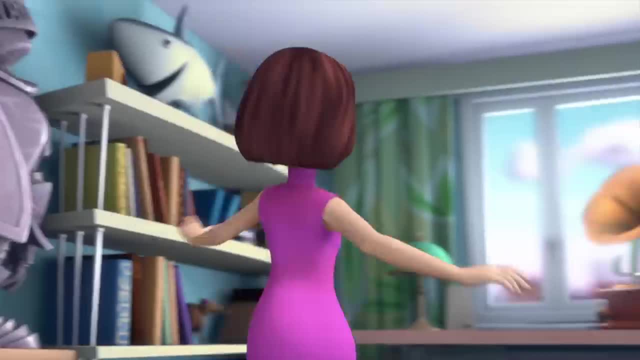 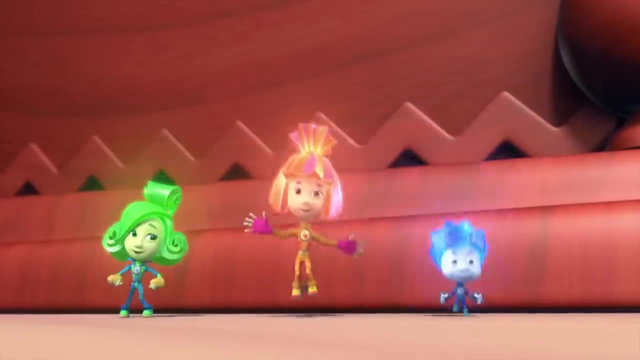 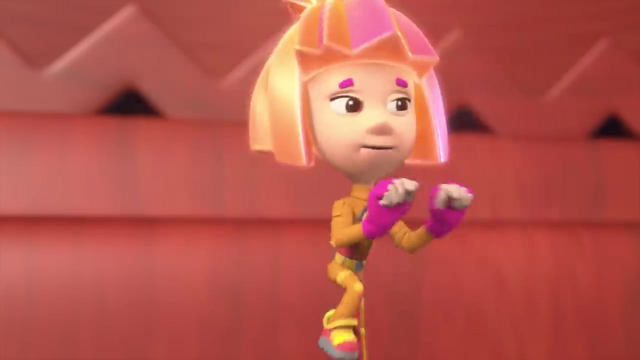 Everything will break without a With no little screws in there. If you think a screw is nothing, Take it out. but just beware, Everything will break without a With no little screws in there. Tom Thomas' mom really dances super. Yeah, she knows how to have a good time. 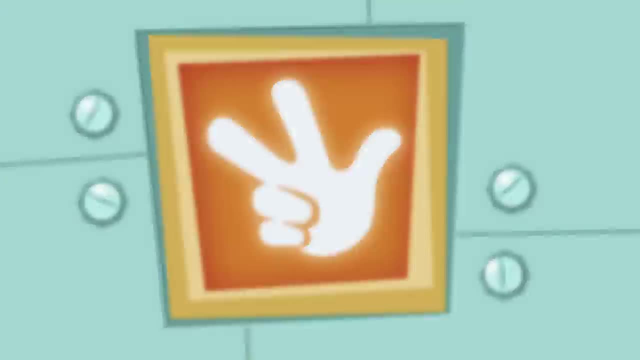 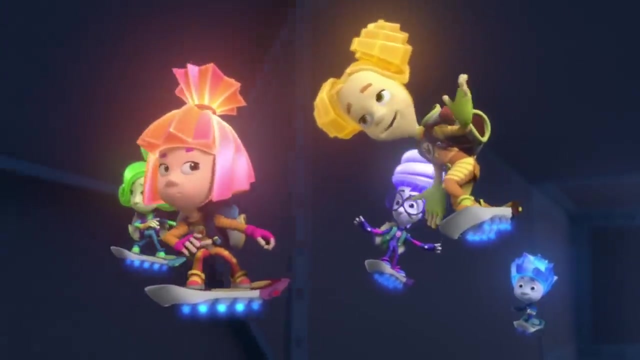 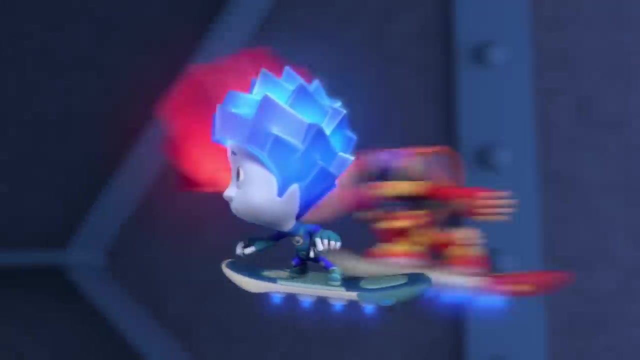 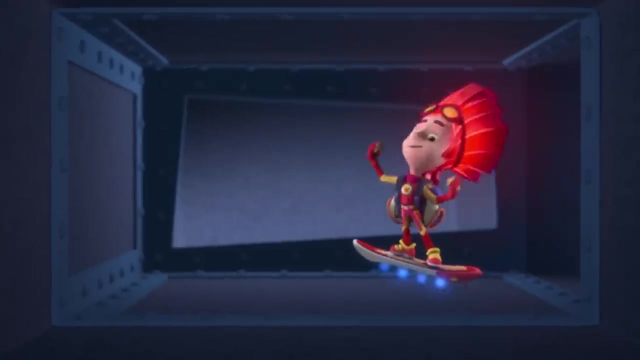 Even though she's a grown-up. If you think a screw is The airbag, We're gonna be late. We'll make it. Whoa, Oh, wow. Hey, slow down there, I'm a super-duper racer. 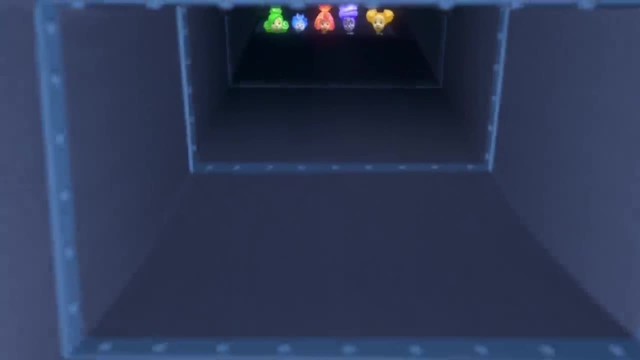 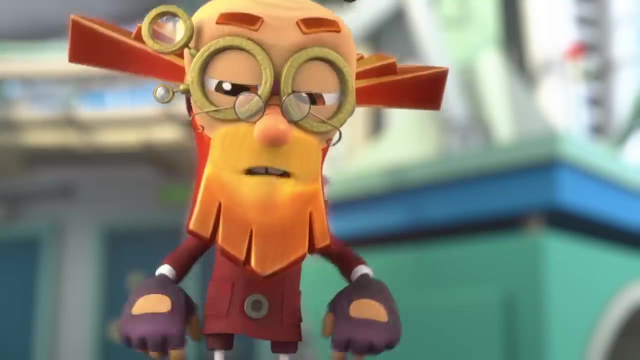 Ha-ha-ha-ha, Ha-ha-ha-ha, Ha-ha-ha-ha, Ha-ha-ha-ha. Well, well, Fire Again, risking your life, And super racers like me can always count on luck. 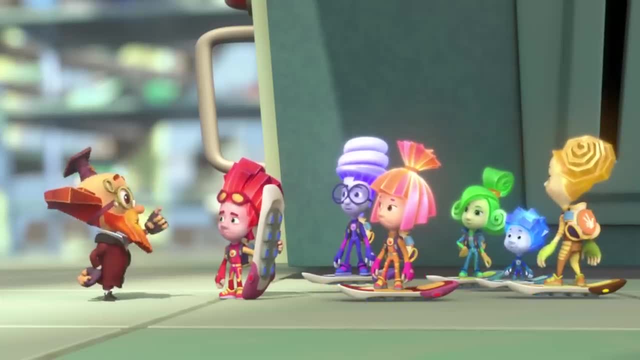 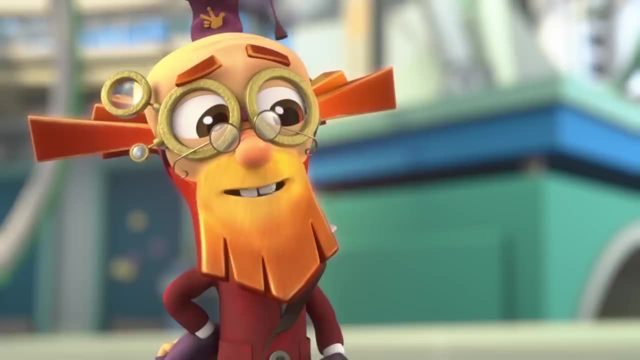 You know, Fire, counting on good luck is stupid. It would be better if you would keep your mind on safety. Actually, today, Professor Eugenius has something really special to show us. He's going to be testing an airbag. Uh, what's that? 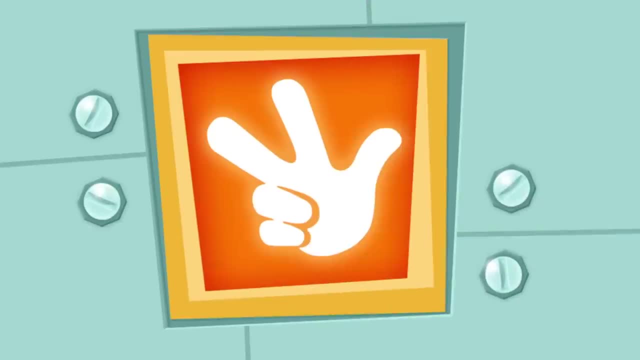 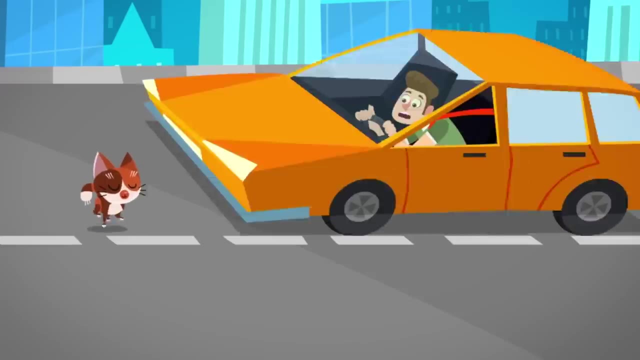 Ditch it, Explain it. Ditch it, Explain it. Everybody riding in a car has to wear their seatbelt Because if the car has to stop quickly, the belt will hold the person back. But there are times when even seatbelts don't give enough protection. 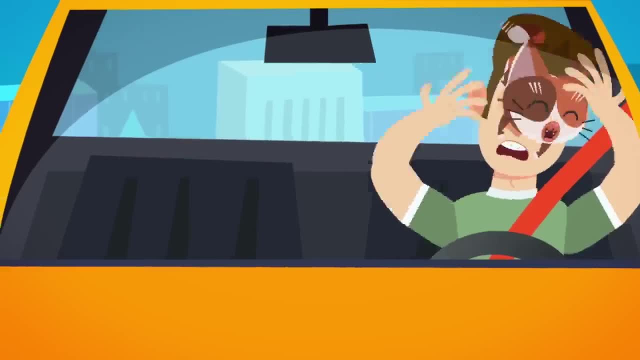 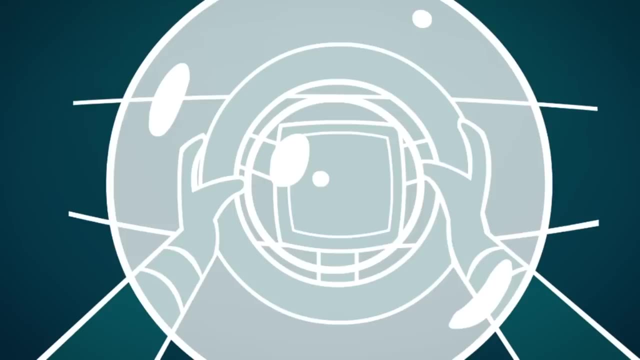 Like when a fast-moving car crashes into something. When that happens, the driver and passengers can be protected by an airbag. You can't see them when they're folded up because they're hidden, But if the car is in a crash, the airbags flow up very quickly. 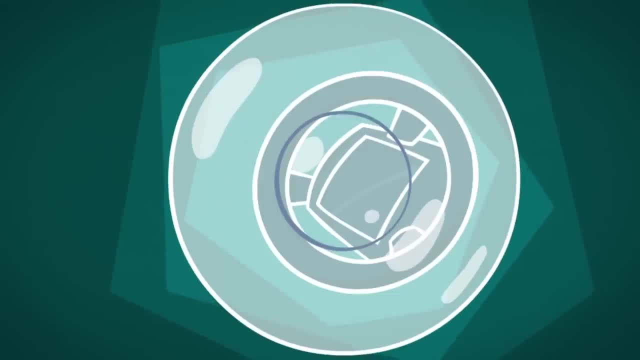 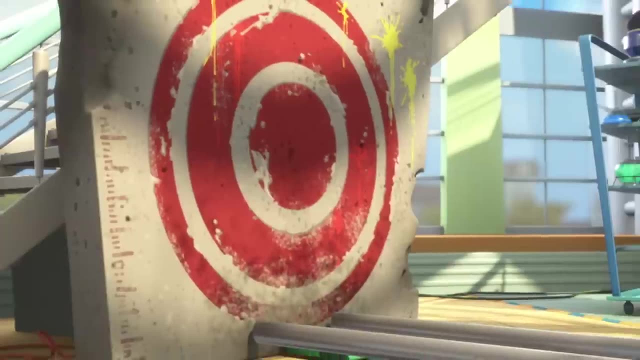 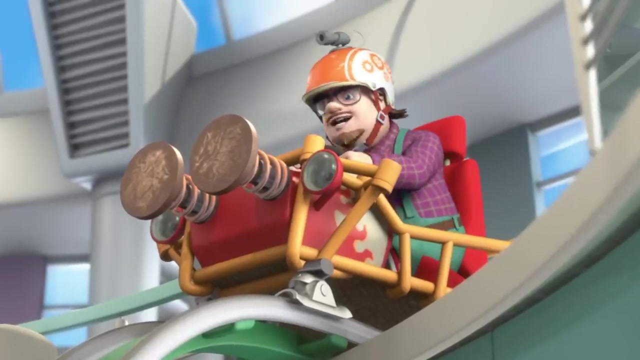 And the person bumps into the bag instead of bagging it to the steering wheel, And that's it: Either bagging it to the steering wheel or flying through the windshield. Here I come, And once again when something dangerous must be tested. 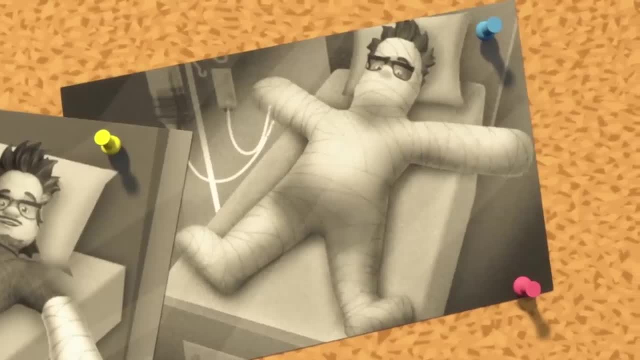 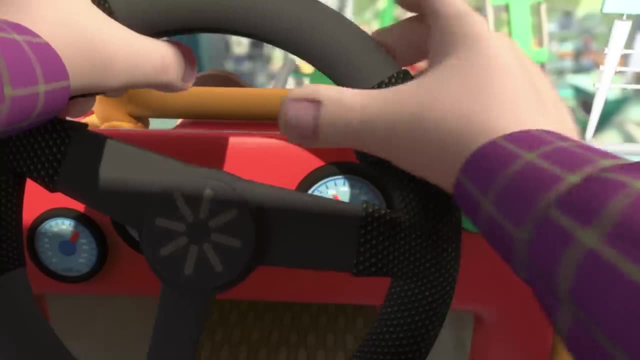 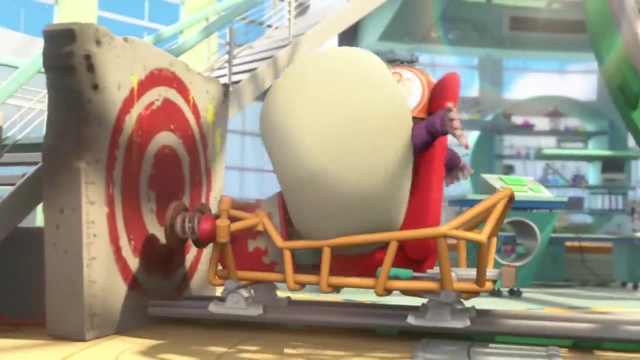 Professor Eugenius tests it on himself. But, Grandpus, aren't you scared that it won't blow up with air? Don't worry about the air. A three and a two and a one. The airbag filled up in an instant, Did you notice? 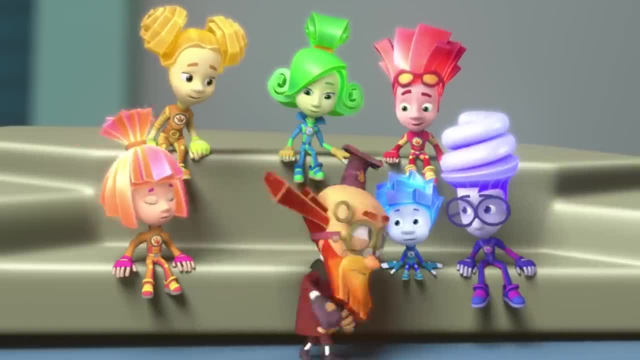 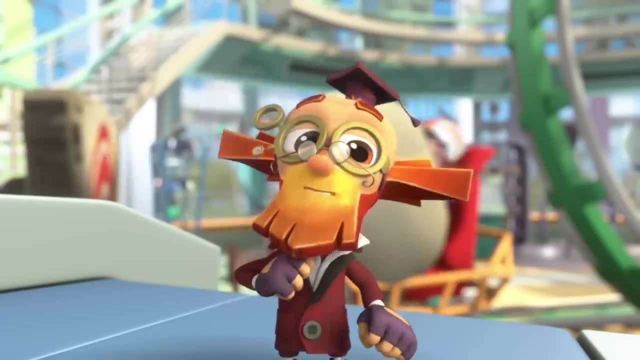 Yeah, But how does it do it? There is a chemical inside of there that quickly burns and instantly turns into a gas the moment the crash takes place. The gas fills the airbag and there you go. Did I explain that right, Professor? 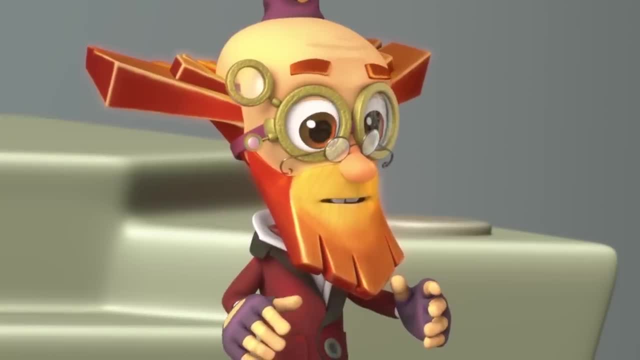 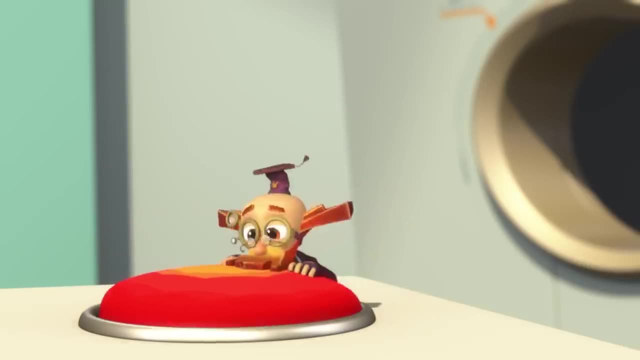 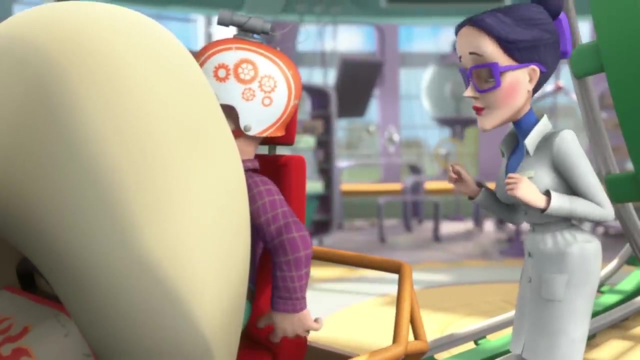 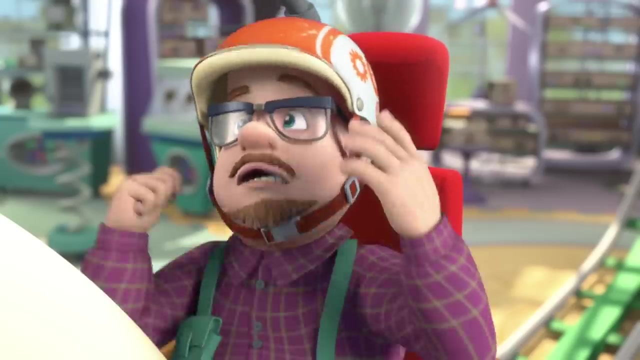 The crew is over here. We've got to get him out. Stop, We'd better call for help. Professor, do you need some help? Thank you, Elisa. Sorry to take you from your work. You're free to go. 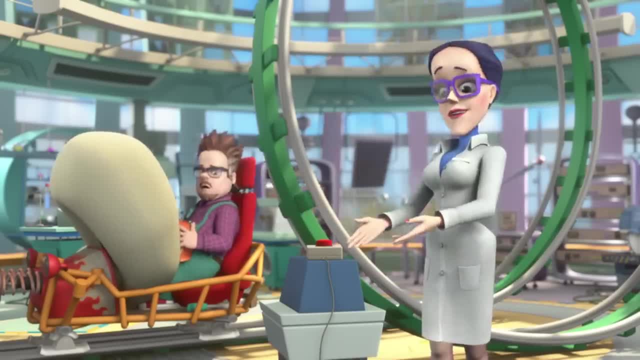 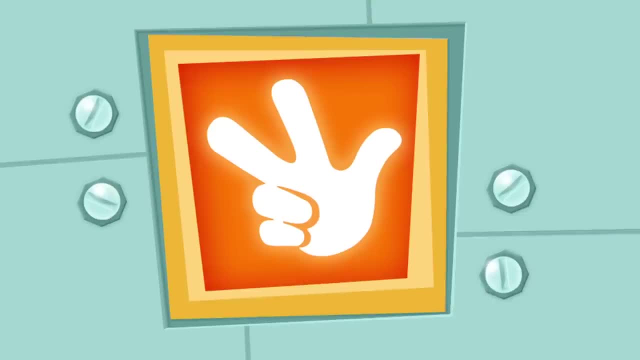 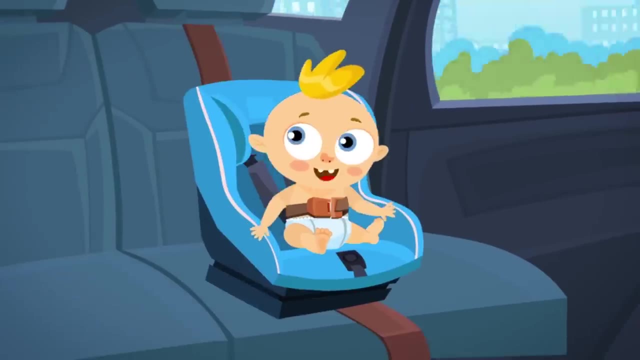 Professor, how did you manage to press the button from way over there? Uh, I managed to hit it on the fly. You are just astounding. To keep small children safe while they're riding in a car, they must be buckled up with a seatbelt inside of a special booster chair. 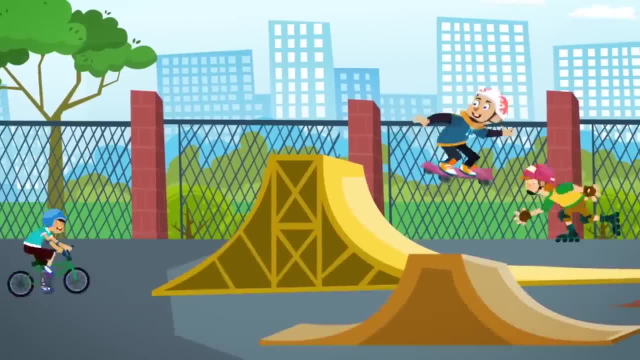 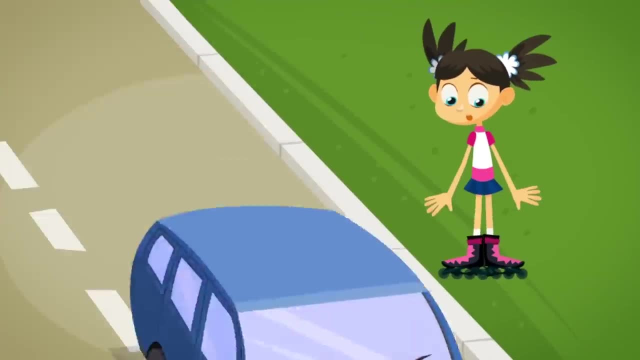 But kids also need to be careful when they're riding a bicycle, skateboarding, roller skating, riding a scooter. First of all, it's best to keep off of roads so there's too much traffic. Second, put your protective gear on. 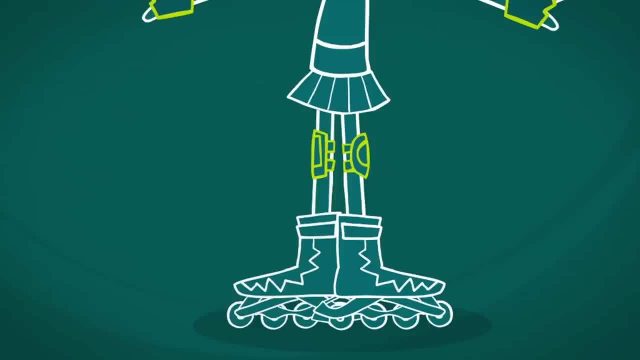 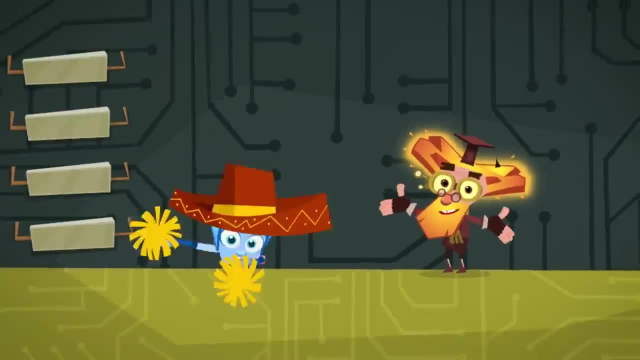 For your arms and legs, wear elbow pads, gloves and knee pads. For your head, wear a helmet. That way, if you fall down, you won't get badly hurt. And third, make sure that people can see you If you're out riding in the evening. 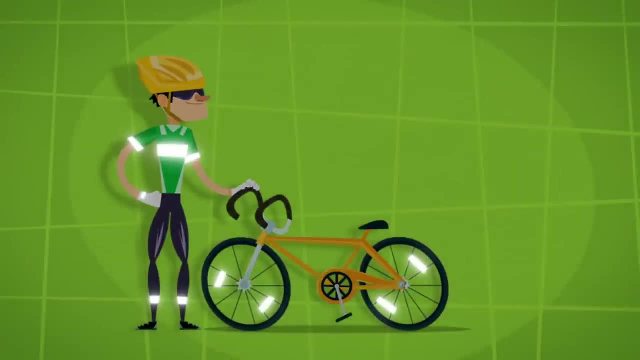 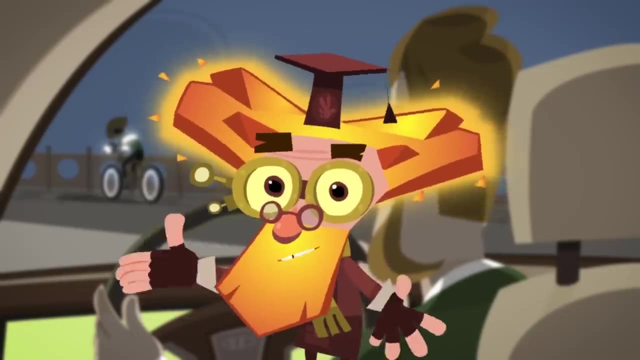 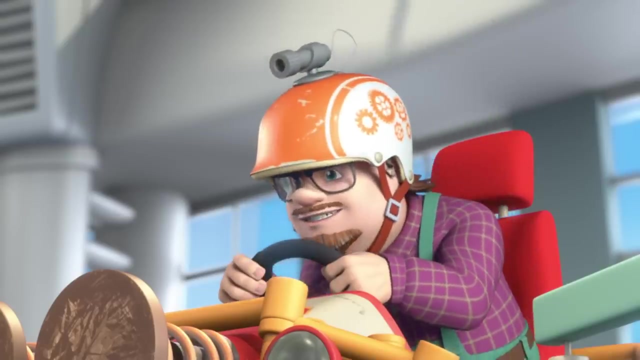 your clothes and bike must have safety reflectors on them. They let drivers see where you are by reflecting the light from their headlights back at them. Remember, better safe than sorry. Sorry, Here we go. I hope this time I've got it. 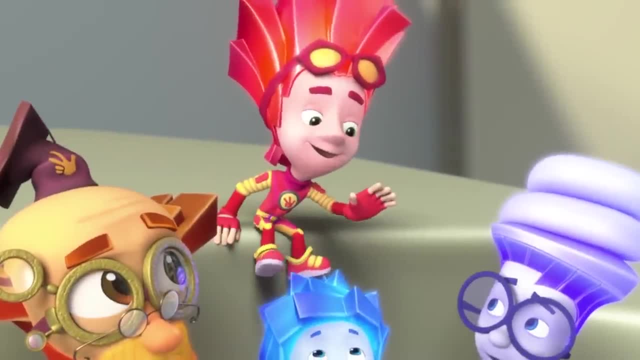 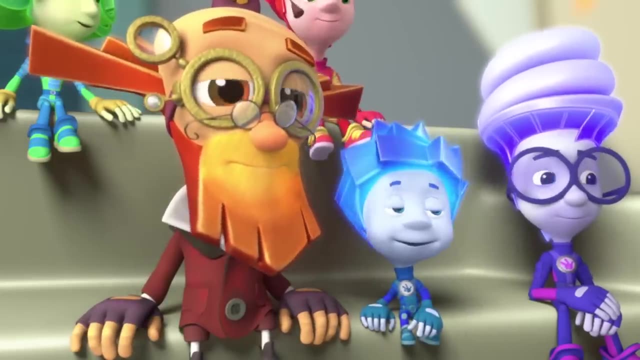 Should we call his assistant right now, just in case? Let's just wait and see Ready set go, Grandpus, he needs to be rescued. Uh no, need I made a change to it Now? the bag not only inflates automatically. 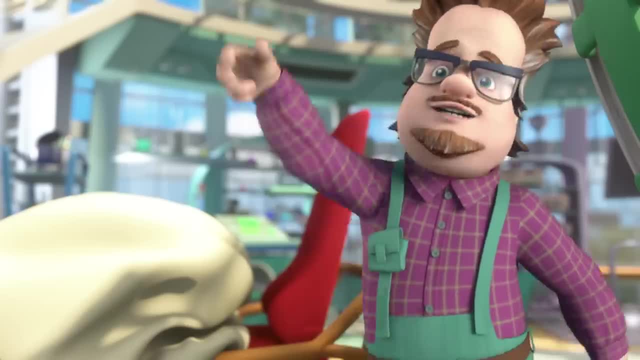 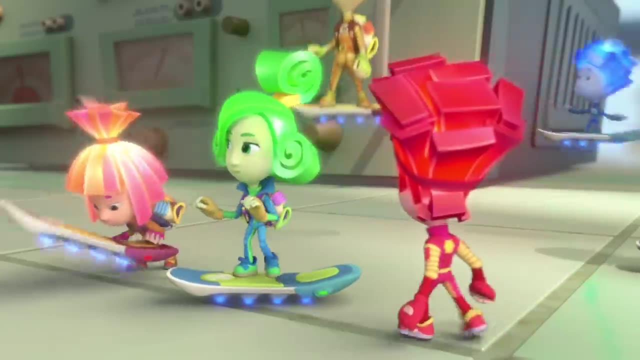 it deflates itself as well. Splendid, As you Fixies say, De-leesh. Today's lesson is done, Hooray, Come on. Where's my Fixie Board? I've got your Fixie Board. Fire, Here you go. 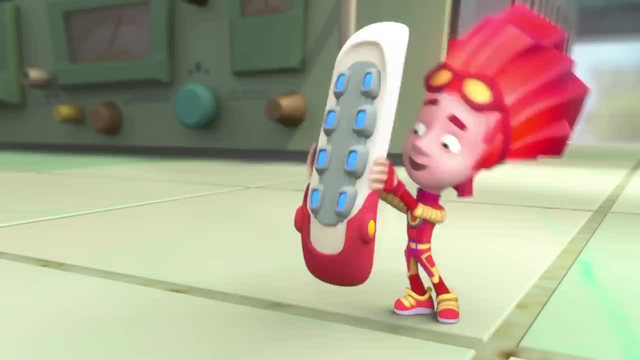 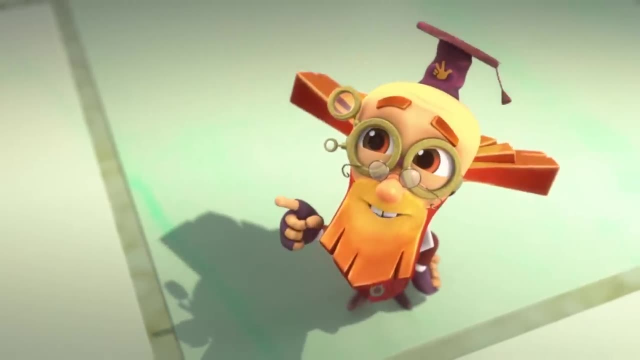 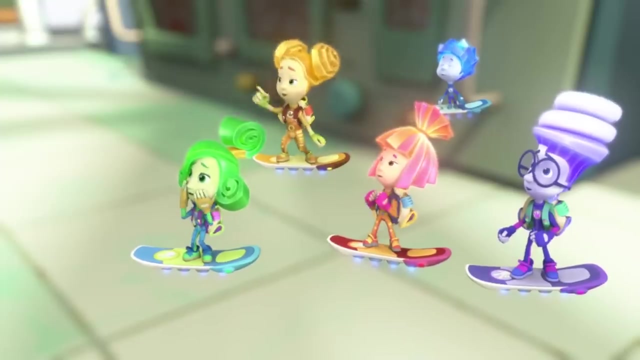 I just went and equipped it with an airbag. Really, Ha. How come? You know I'm a super racer, See Woo-hoo, And that's why I installed it. Super racers don't need airbags. We never, never, ever, ever. 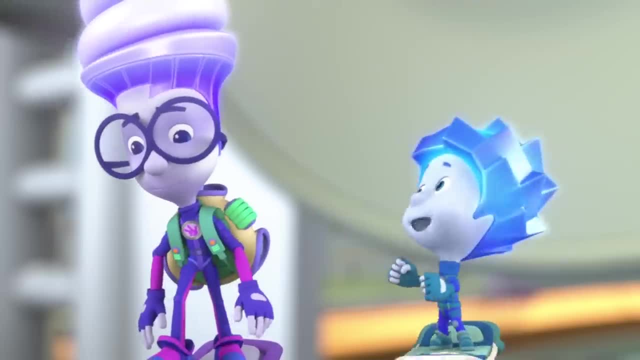 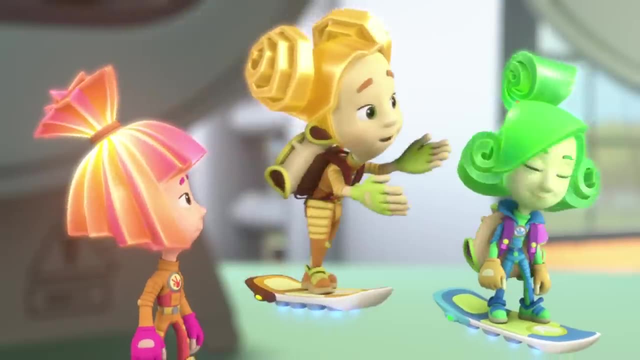 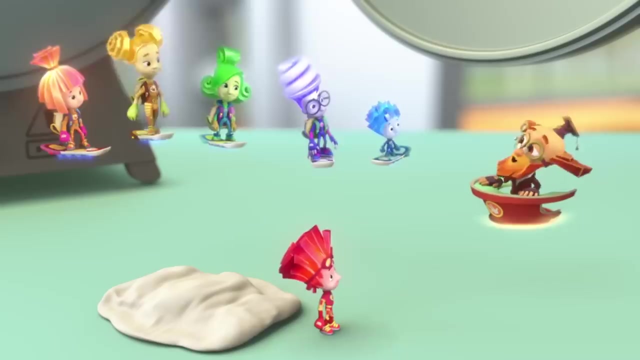 Oh wow, Is that airbag cool or what? It's a very original design you used there. That design is my own And Fire ran the test. Professor, will you make an airbag for each one of us? You all will get them Real soon, But even so. 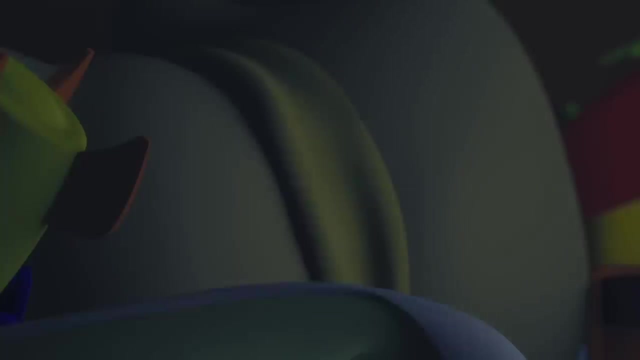 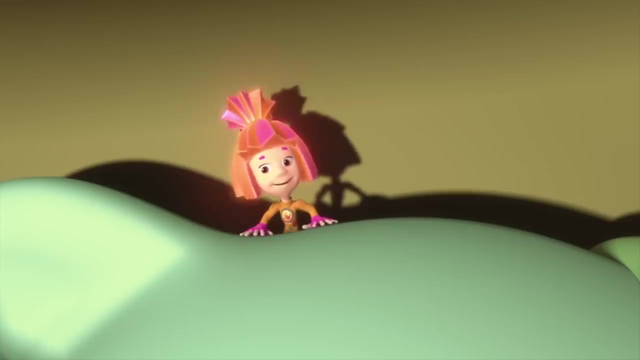 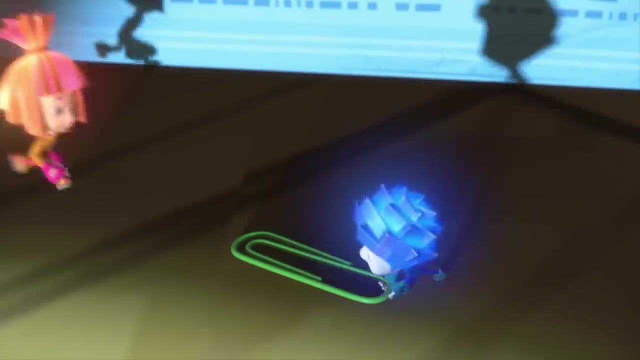 Caution and care make accidents rare. Ah Ah, The shadow play. Oh, hi there. Tom Thomas, What are you doing here? I dropped a paperclip. Give me some light. What's so funny? huh, We're trying to help you out. 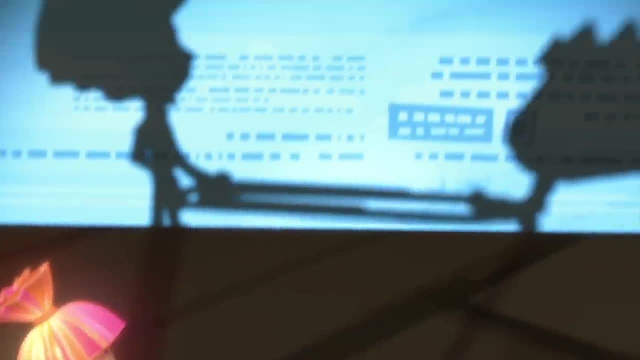 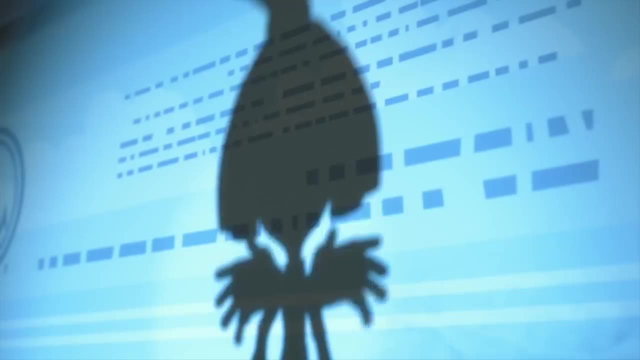 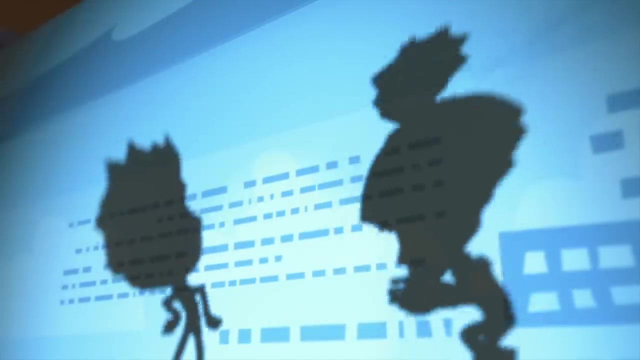 You've got funny shadows. that's what. Hey, check this out, It's an eagle And Zipka is a goose. Ha-ha, She looks more like a moose, I do. huh, Alright, then take that. 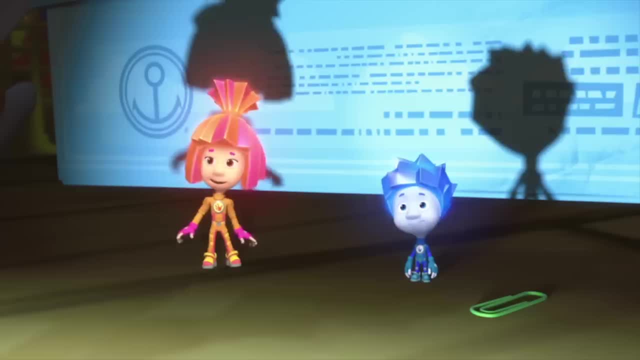 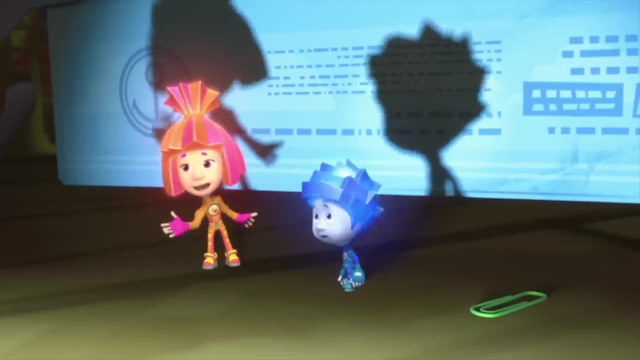 You're like real actors performing in a show. Uh-huh, Actors play in a theater, you know, And we're just under a bed. And so what? How about we make our very own theater, A theater with shadows Class. 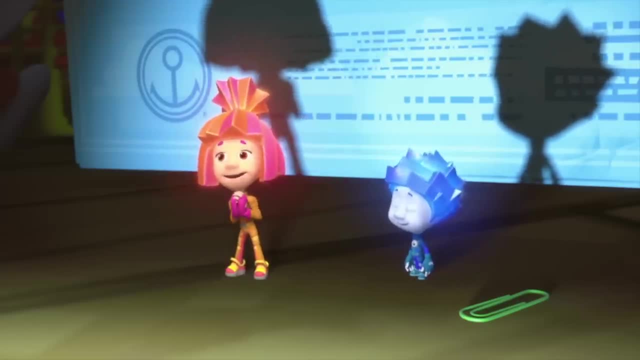 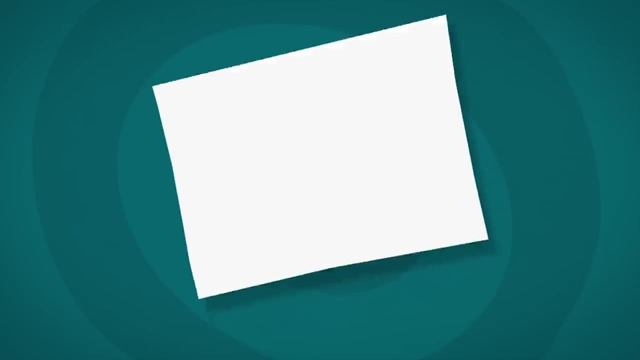 Tom Thomas, we need a piece of paper, a huge sheet. Let's do it, Let's do it, Let's do it. It's really quite easy to make your own shadow theater. You can make the screen out of a white sheet or a big piece of paper. 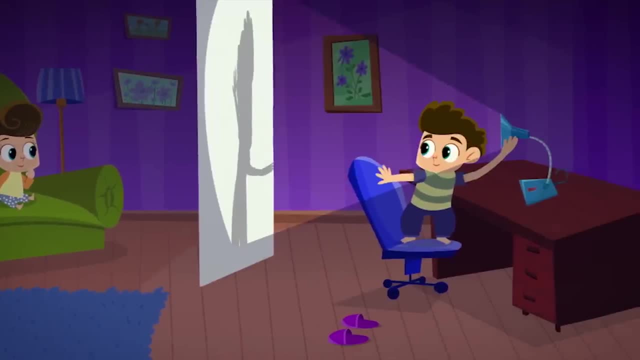 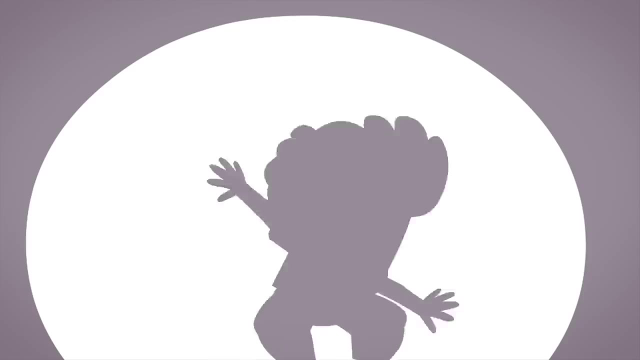 Next, make sure the room is dark and shine a desk lamp at the screen. Now to make the shadows, just put yourself or a cardboard cutout between the lamp and the screen. Your shadow, or the shadow of your puppets, will come to life. 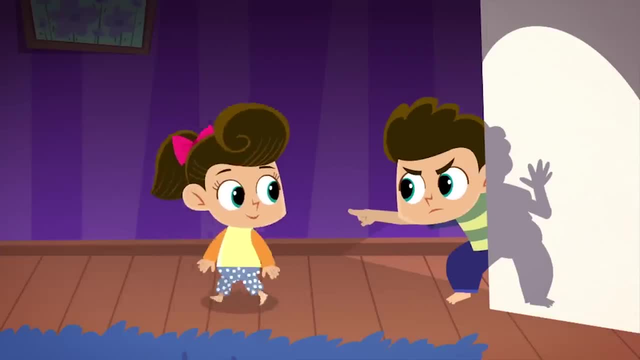 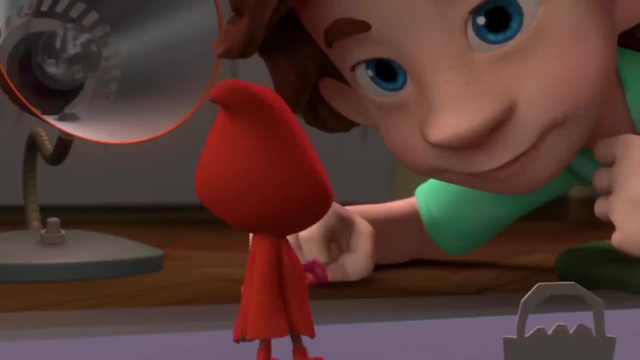 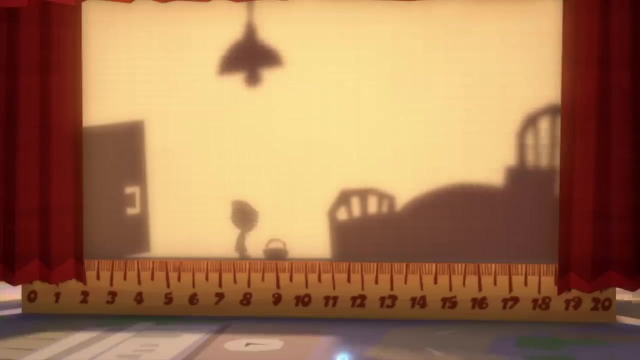 But make sure that the audience sits on the other side of the screen. The play will be much more magical for you. It's going to be really cool for them from that side. Tom Thomas light. Oh wow, Simka, You look totally like the real Red Riding Hood. 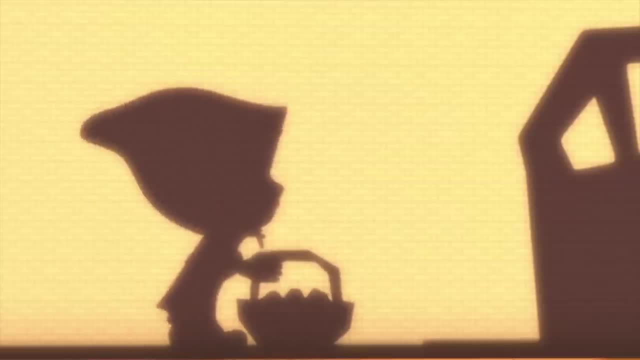 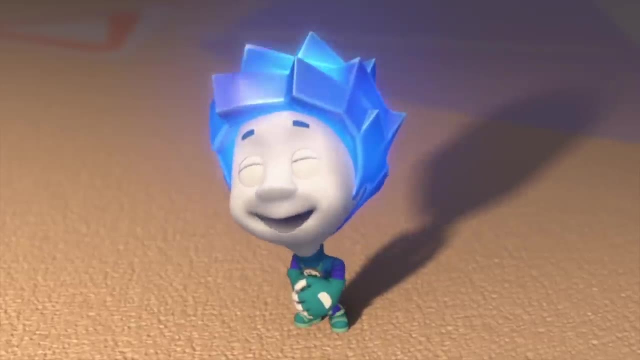 Hello, dear Grandaughter, Hello, dear Grandmother. Grandmother, what very big eyes you've got. The better to see you with my dear Nolik. come on, We're rehearsing. The wolf's voice is funny. 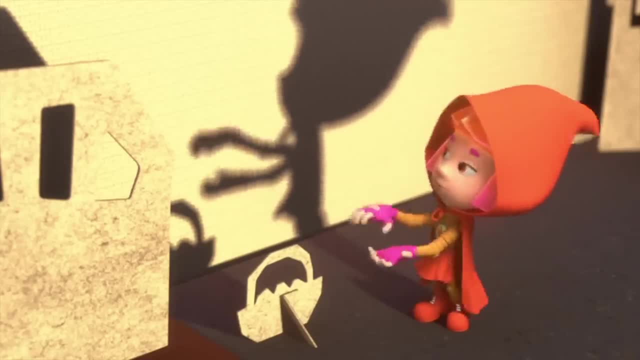 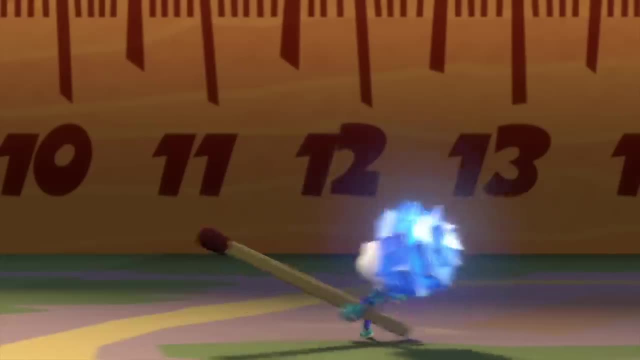 Grandmother, I never noticed what very big teeth you've got. They're so much better to eat you with my dear Yum, Yum, Yum, Yum. Let them out, wolf, Or I'll… Or I'll…. 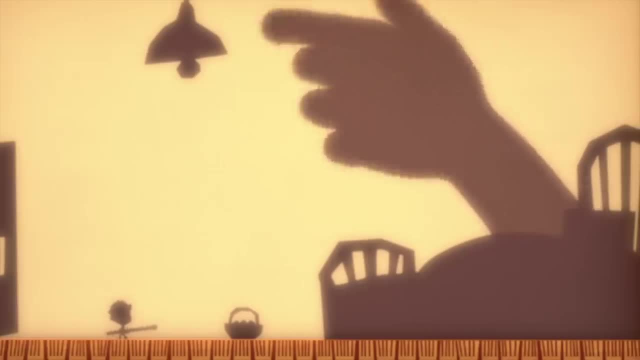 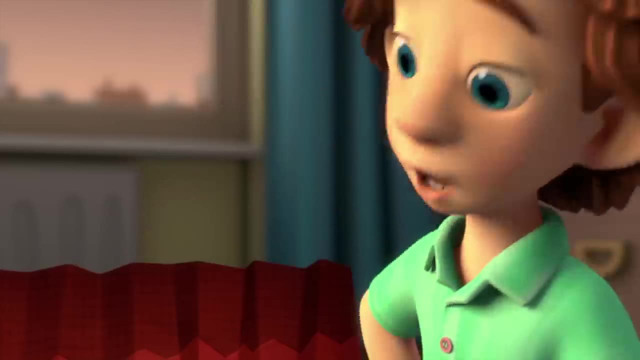 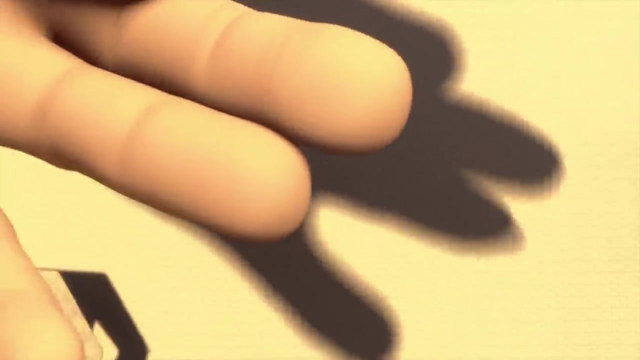 Get them out myself. You'll stop me with that little stick. Hey, That's not in the fairy tale, But in the fairy tale it's a normal hunter. And what do you think I am? Look for yourself. You're way too small to be the hunter. 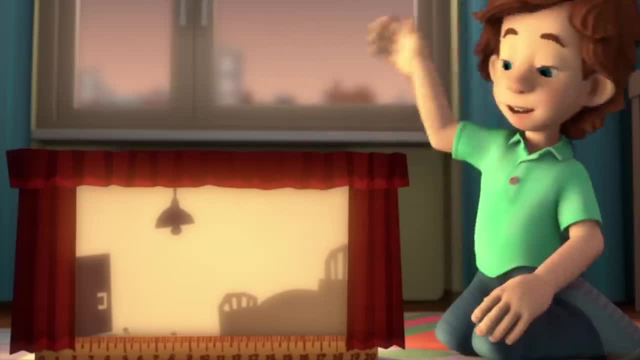 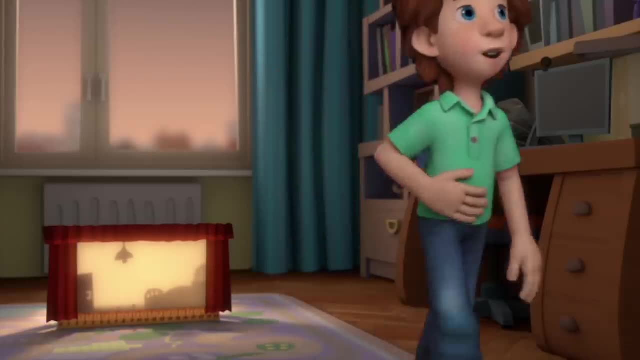 Fine, Then go to your play without me. Well, I guess I'll have to make the hunter out of paper then That's all. Take a break. I'm really thirsty. She was so salty that Grandma Nolik don't be upset. 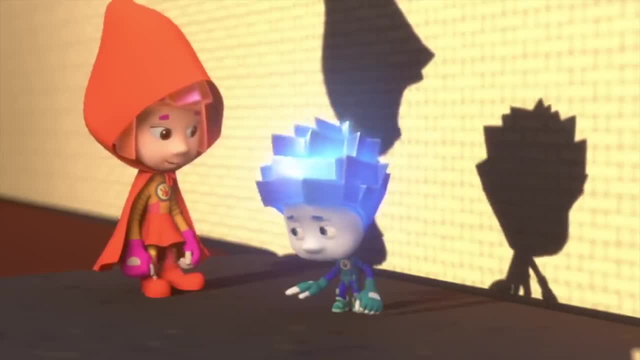 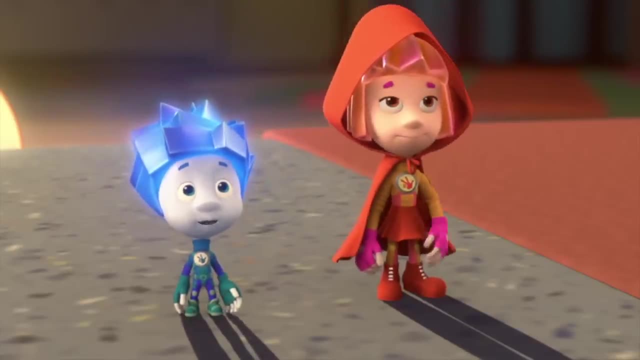 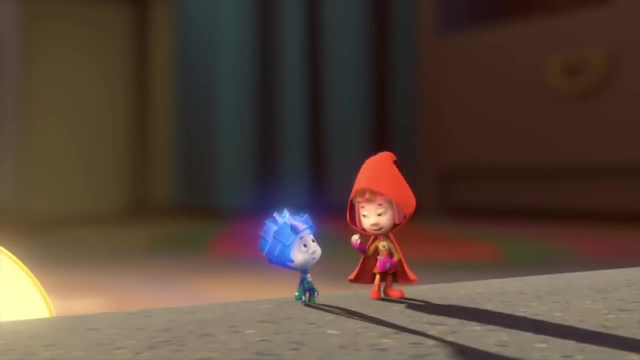 The wolf is huge and I'm so little, Then let's make you bigger. You see, Now you're bigger. Yeah, you're right. And if we go back here… Then I'm even bigger. Now, you know, If you go back here near the lamp. 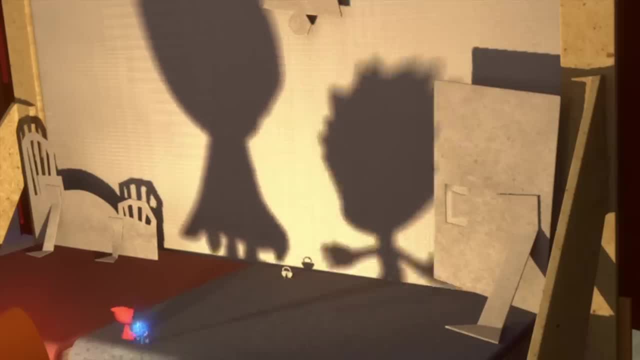 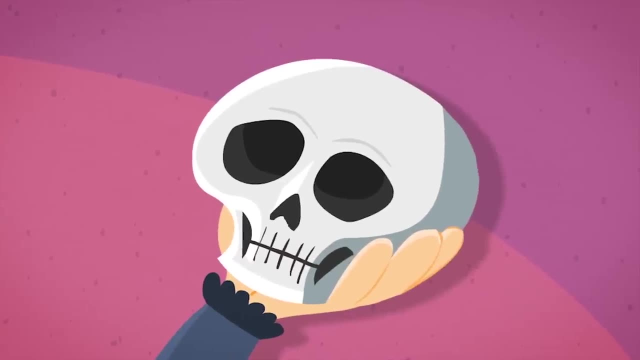 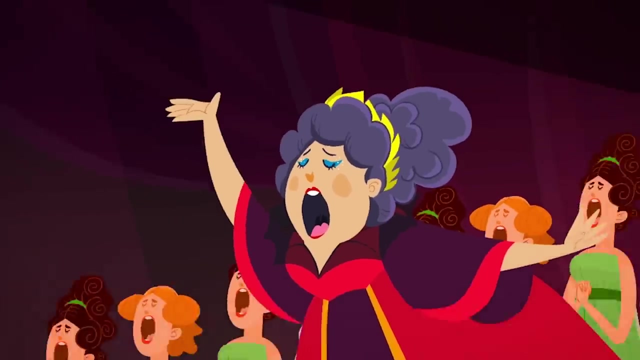 your shadow will get bigger on the screen Clash. There are just so many different kinds of theaters in the world. In the dramatic theater, the actors speak the lines of the playwright. At the opera, the actors don't speak their lines, They sing them accompanied by an orchestra. 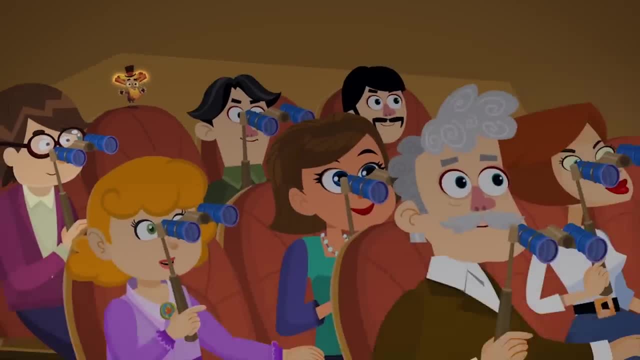 And here at the ballet, the performers don't sing their lines. And here at the ballet, the performers don't sing their lines. And here at the ballet, the performers don't speak their lines. Here, the story is told with dance. There are also theaters where the performers are animals. 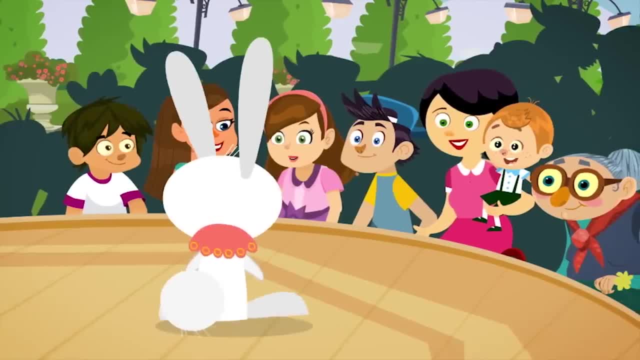 There are also theaters where the performers are animals. In an animal theater, you can watch performances by cats and dogs In an animal theater. you can watch performances by cats and dogs In an animal theater. you can watch performances by cats and dogs. 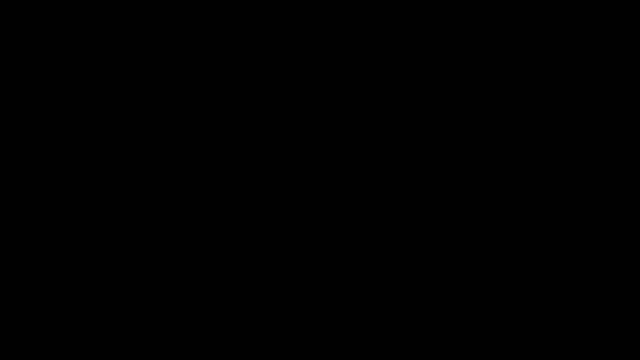 Or goats and pigeons, Or even bears and seals. There are also theaters where the stories are told by puppets. There are also theaters where the stories are told by puppets. To tell the truth, the puppets are brought to life with the help of people. 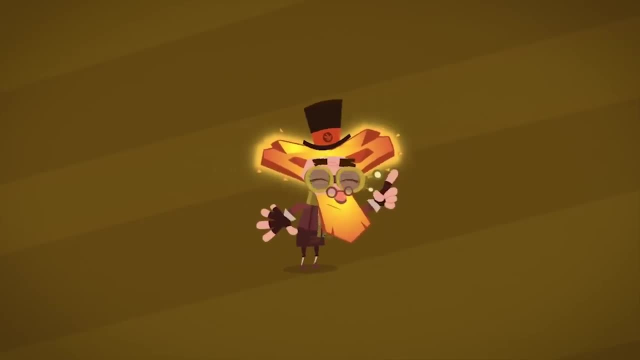 To tell the truth, the puppets are brought to life with the help of people. Yes, there are so many different kinds of theater. My favorite is the shadow theater. I think it's the most beautiful and mysterious theater of them all. I think it's the most beautiful and mysterious theater of them all. 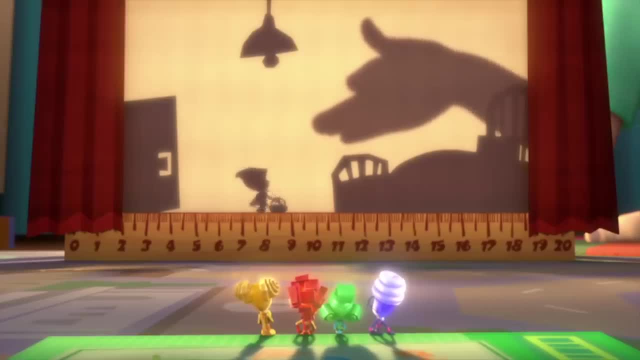 Hello, dear Grandmother. Grandmother, what very big eyes you've got. Grandmother, what very big eyes you've got. The better to see you with my dear And Grandmother, what great big, sharp teeth you've got. 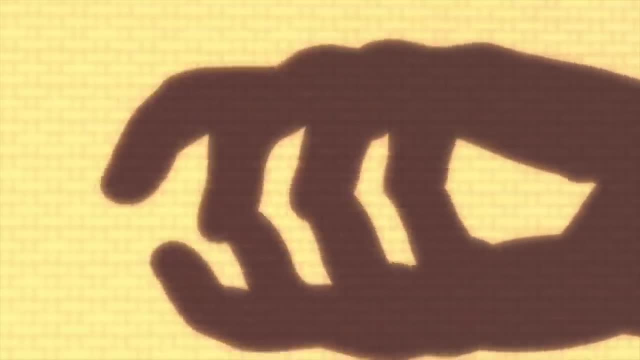 And Grandmother, what great big sharp teeth you've got. Oh, the better to eat you up with my dear. Oh, the better to eat you up with my dear. Oh, just wait. Aha, Wolf, I've got you. 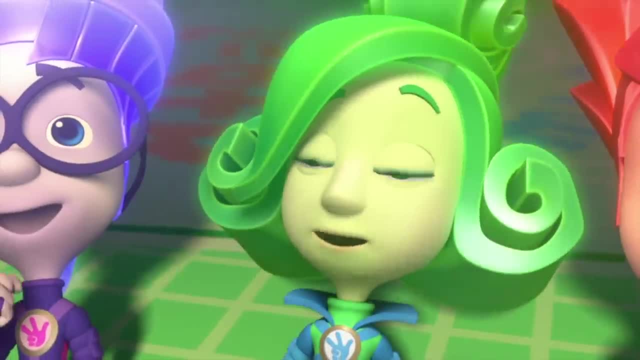 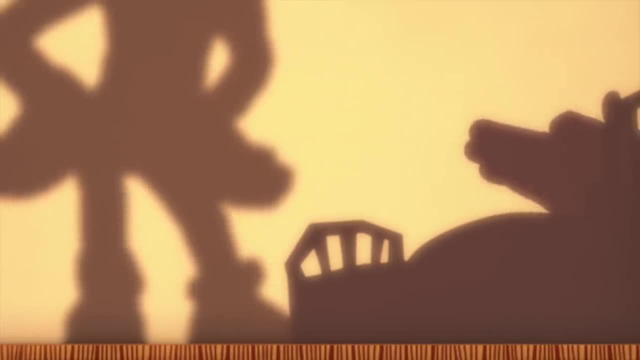 Aha, Wolf, I've got you. The hunter looks so strong. You're a hunter, Then where's your gun? You're a hunter, Then where's your gun? Why do I need a gun? You're so tiny, I could use a fly swatter. 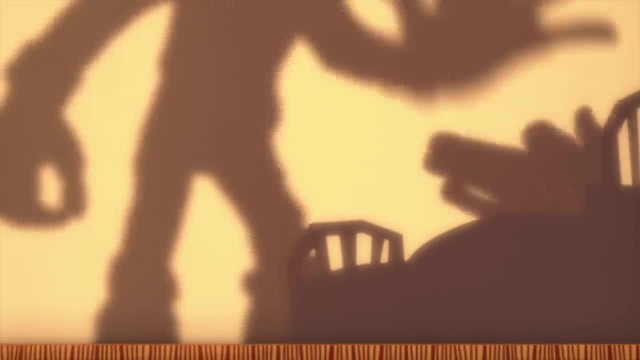 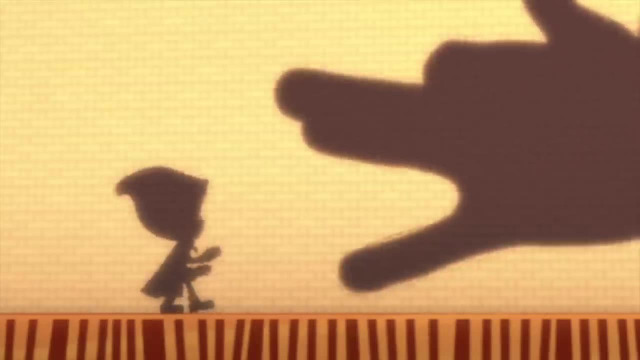 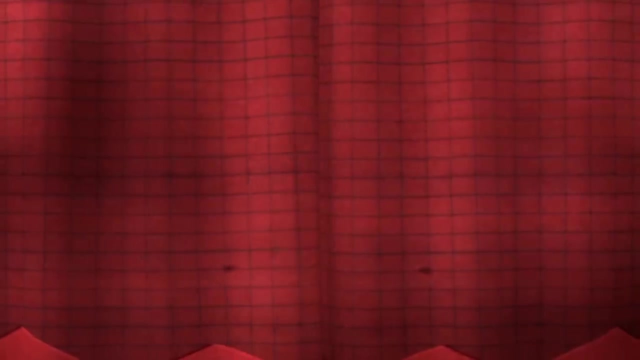 But I'd rather do it like this. Like what, With my bare hands. Way to go. Hooray, Splendid. Who was your favorite? Mine was the Grandmother. Well, I think Red Riding Hood was the best For me. the hunter. 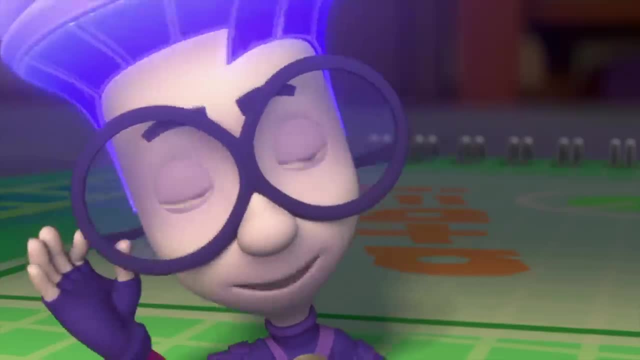 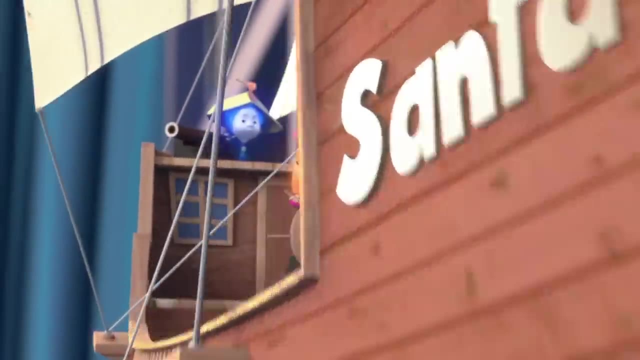 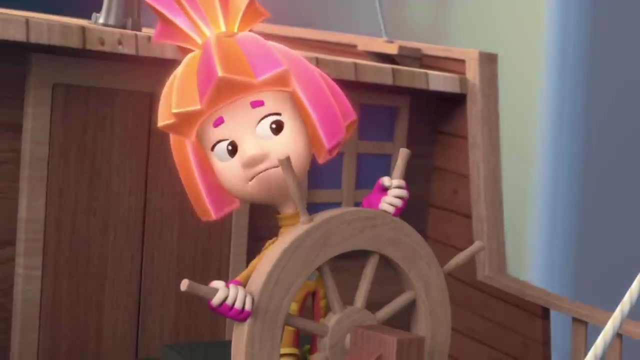 He was so mighty And so fearless. And for me the special effects Knots. No, look, There are pirates off the starboard side. There are pirates off the starboard side. Battery Fire. Hey, I'm not a pirate. 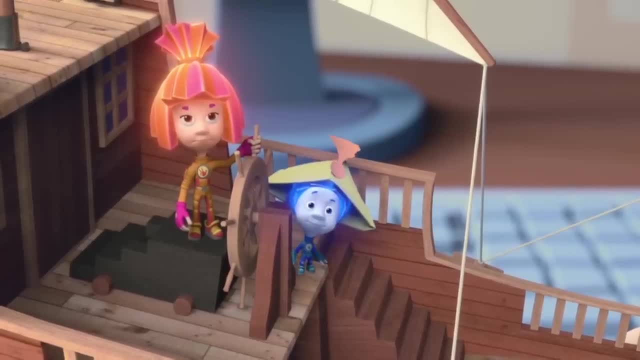 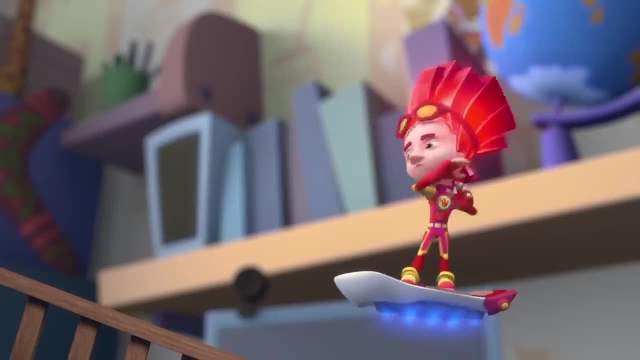 Why'd you hit me? That's it. I'm tired of playing the wind. Where are my pirates? This looks great. Can I board your ship And what are your skills? Tons Like protecting the ship and yelling hooray when we win. 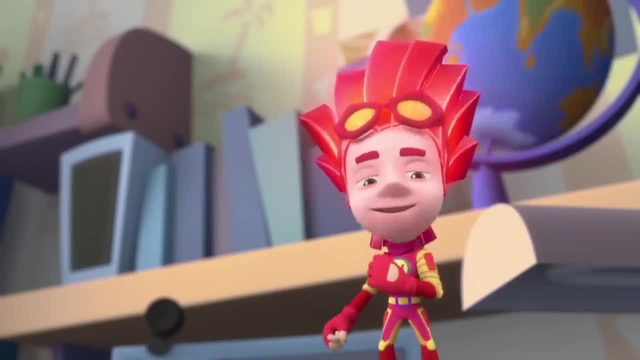 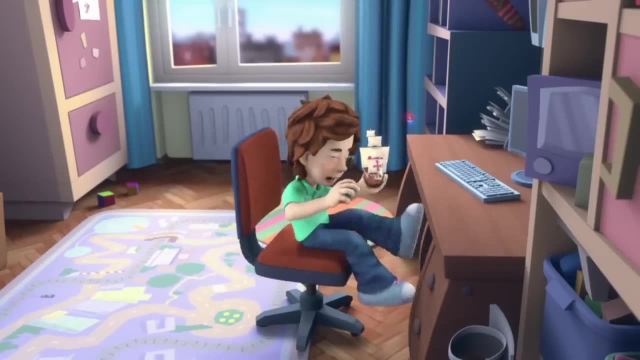 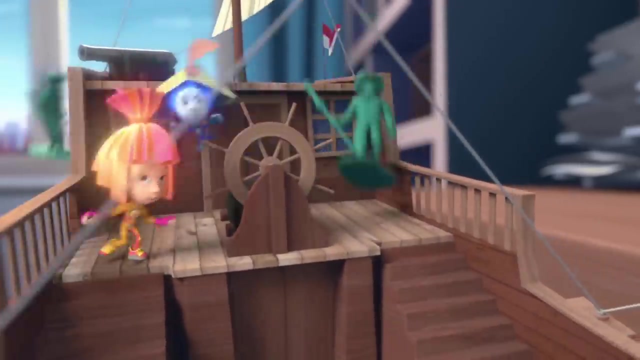 And how about good sea knots? Can you tie them? Of course I can tie them. Then tie up our treasure And make sure it's good and tight. Pirates prepare to attack. I got it. Hooray, That's done. 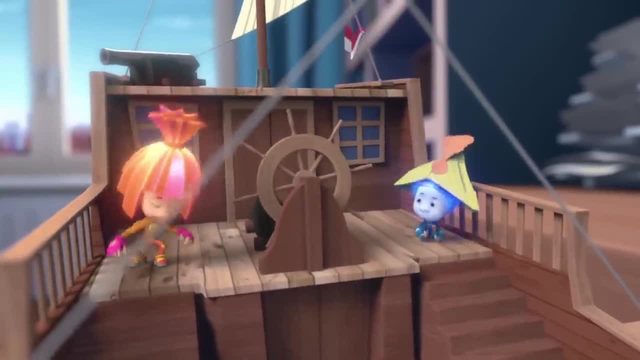 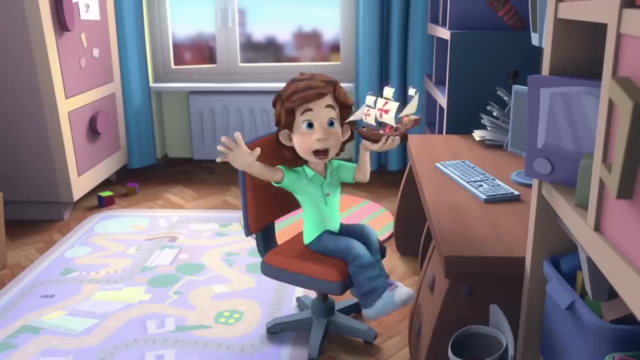 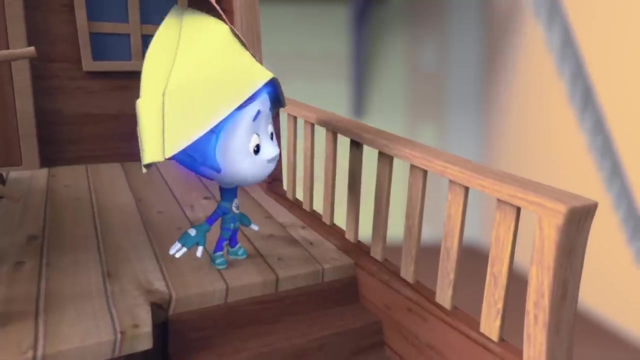 Good enough, Hooray. It's good and tight. Now can you survive a storm? Without a doubt, Our treasure. It sunk into the sea. That was my mom's necklace. we sunk. I'll pick it all up, don't worry. 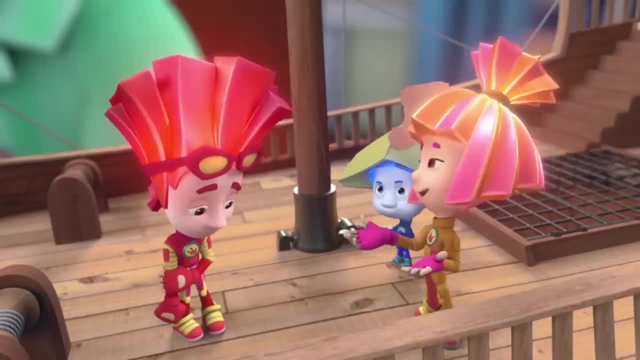 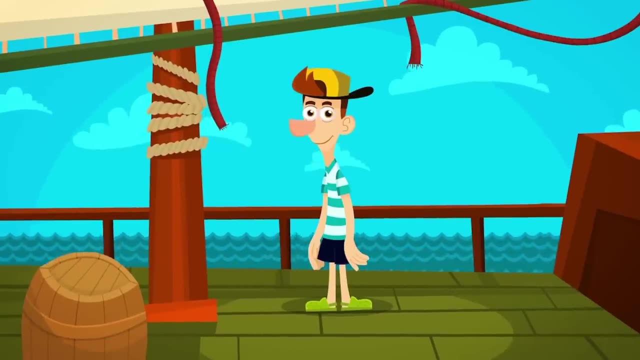 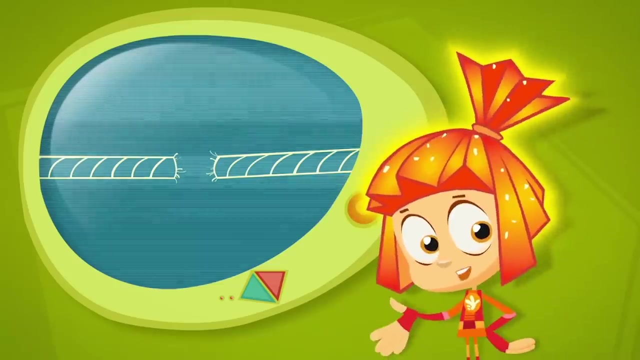 We'll manage ourselves. He calls himself a sailor. Go and learn to tie some knots. Try tying two ropes into a knot. You think it's easy? A badly tied knot will untie itself before you know it. Here's one way to tie it right. 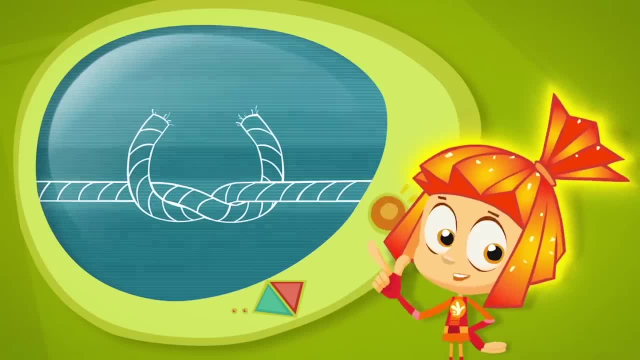 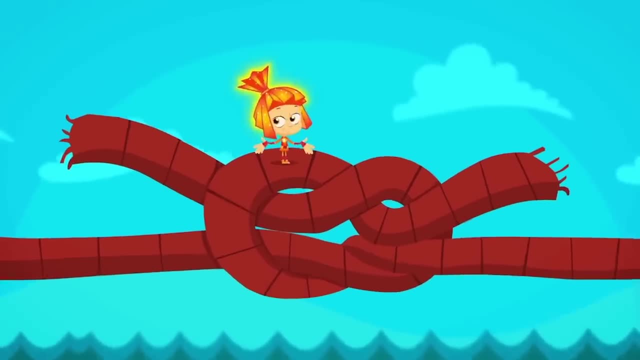 First cross over the two ends like this: Now to finish the knot, you've got to cross them over again, But not this way. It's got to be in the opposite direction. When it's done, tie one loop inside another. 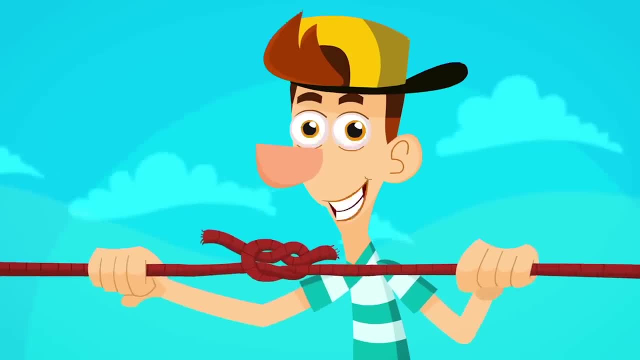 This kind of knot is called a square knot And it won't untie as long as you tie it right. And that's just one of the many kinds of knots a sailor has to learn. And that's just one of the many kinds of knots a sailor has to learn. 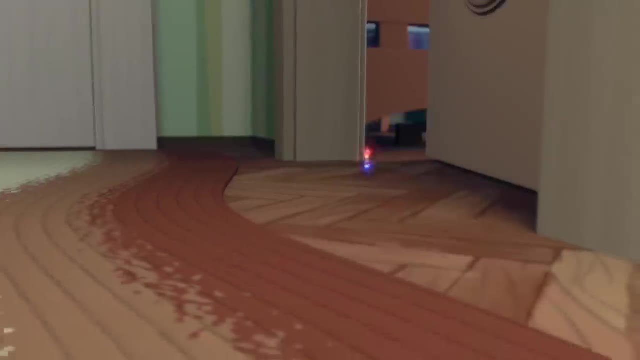 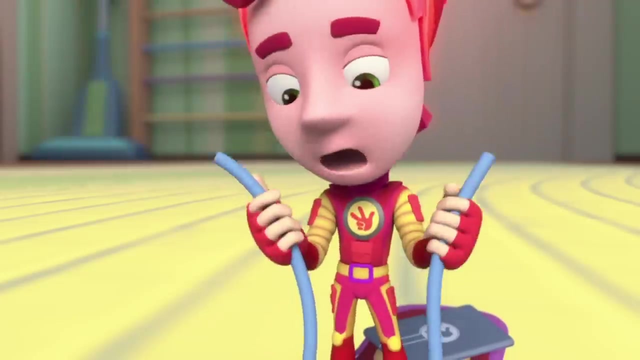 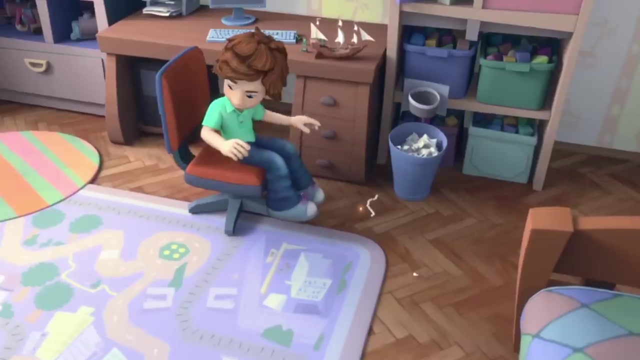 And that's just one of the many kinds of knots a sailor has to learn. Okay, I knew I could tie it, Now what else is there to practice on around here? I found some more of our treasure. I found some more of our treasure. 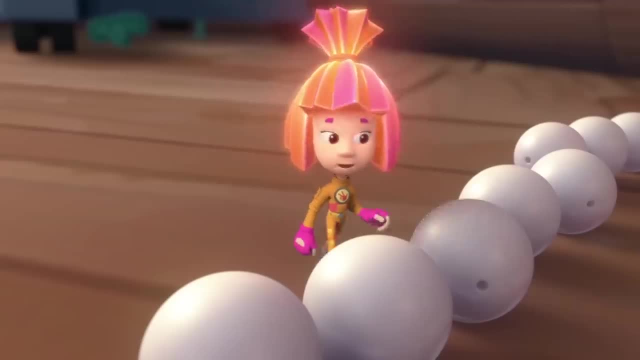 Here's another one. That's 19,, but we're supposed to have 20.. That's 19,, but we're supposed to have 20.. I know it because I'd counted our treasure. So what happened to the last one? 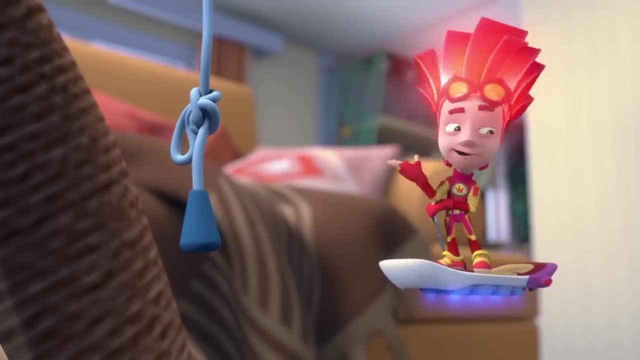 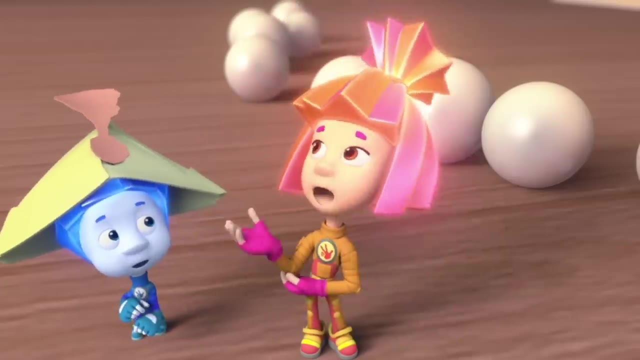 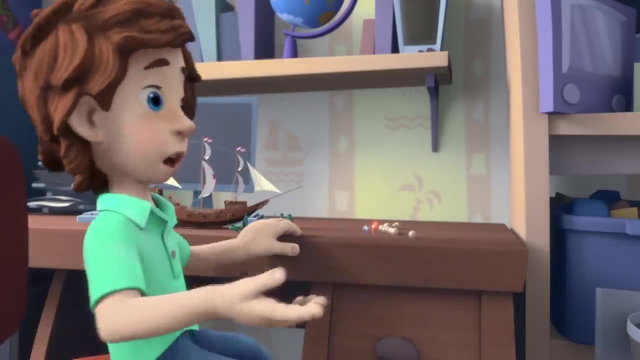 Well done there. So what else could I tie? Perfect. I even remember what it looks like. It's a different color, It's a bright red one. Mom's going to notice right away that the red one's gone. I gotta go find it. 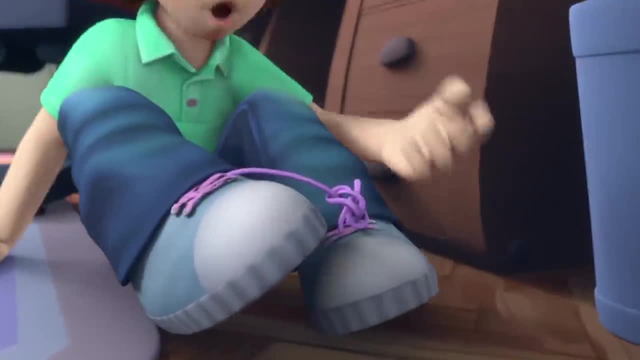 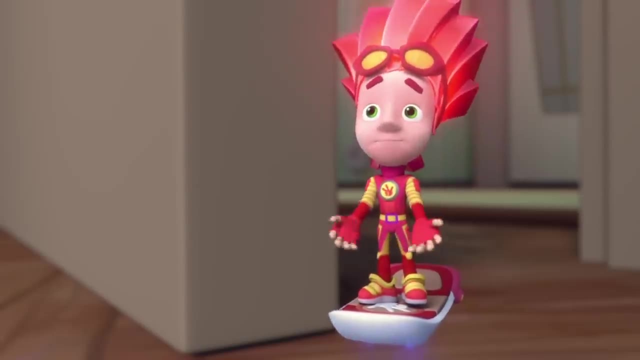 Yeah, I think it's on the floor. Who tied my laces together? I was just practicing, Sorry. And what else did you tie up to practice your knots? I'm not sure you want to know. You're funny, Let's go untie them. 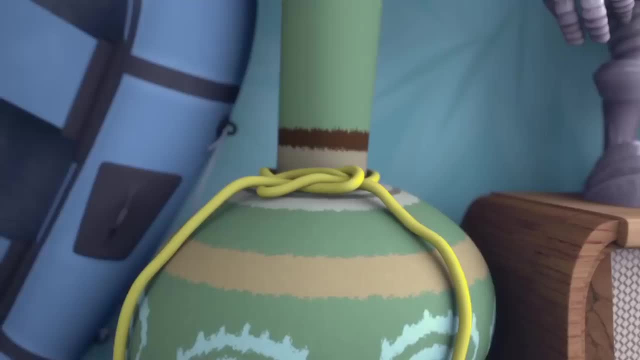 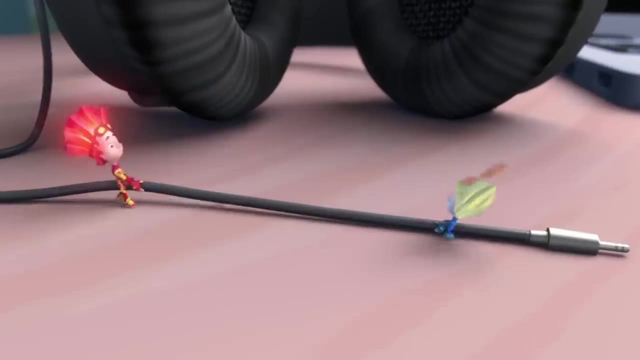 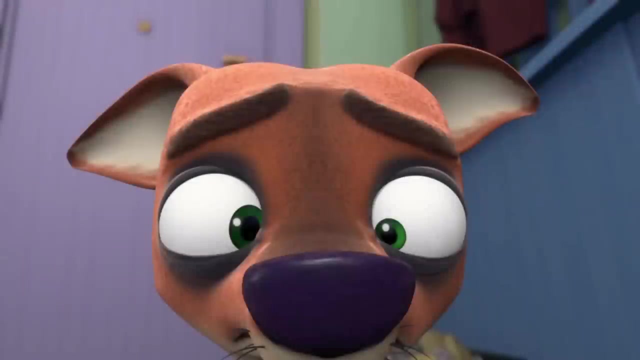 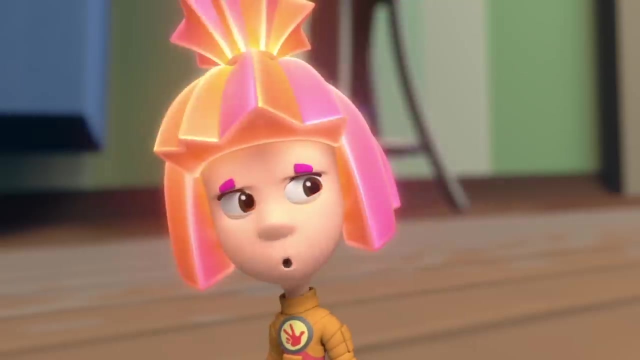 Let's go. Chewsocka, don't look at me that way, I'm scared. She's just staring at her own whiskers, Nolik. And what have you done to her whiskers? Well, I tied them with the square knot. 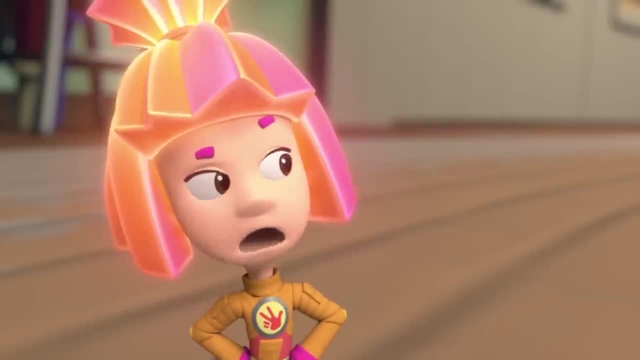 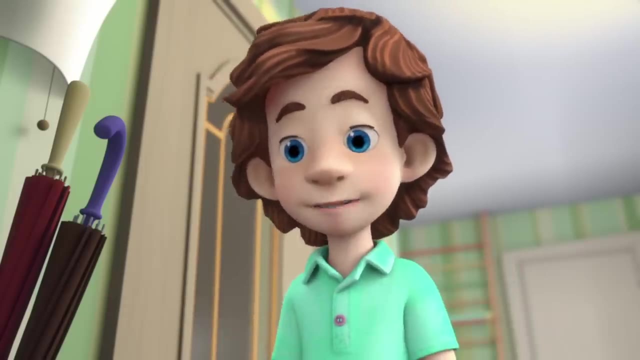 Fire, you're just a blocker, And why don't you tell us what else you've done? Well, okay, I tied a decoration on her tail. That's where it is. We were looking everywhere for that thing. Fire, go and fix everything you've done. 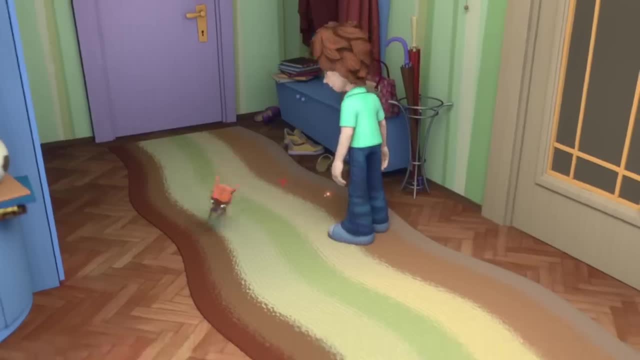 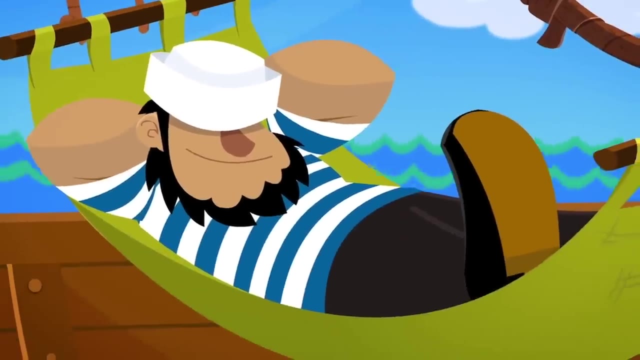 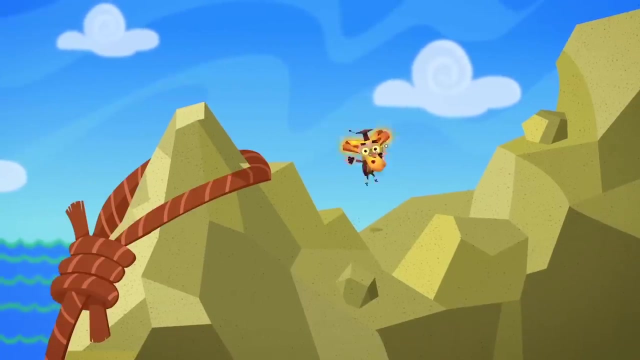 Chewsocka, don't run away, Don't be scared. We just want to untie the knots. Sailors have developed all sorts of different knots. Without them they couldn't control their sails, But we couldn't get by without knots. 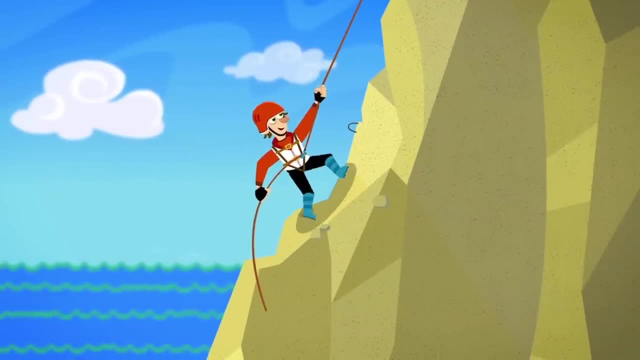 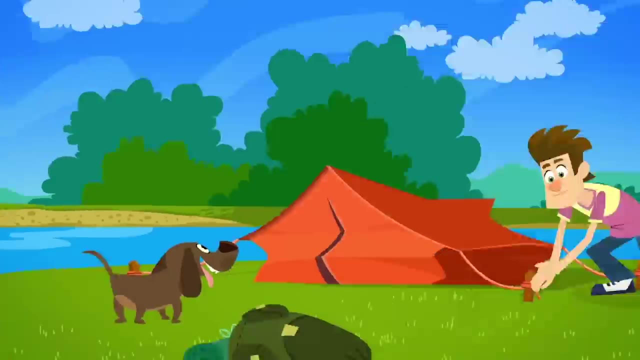 on land either. Mountain climbers use tightly knotted ropes to help them climb and keep them safe. Fishermen tie hooks to their fishing line using special knots. You can't even pitch a camping tent properly without making a knot. When people sew, they tie knots in the thread. 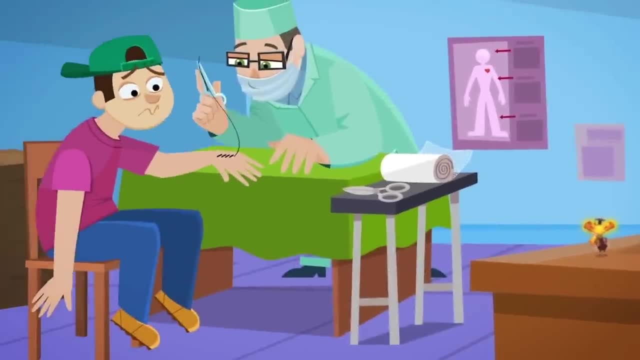 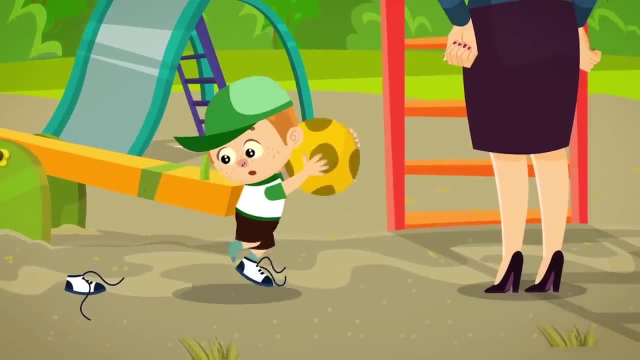 to hold it in place, And doctors use knots when they stitch and bandage a wound. And a tie wouldn't be a tie if you didn't tie a knot in it. Sneakers won't fall off your feet And the laces won't drag on the ground. 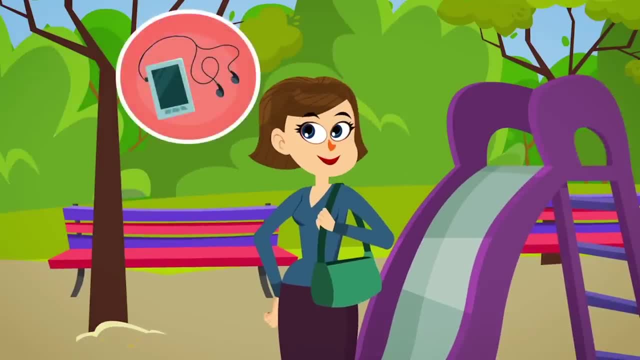 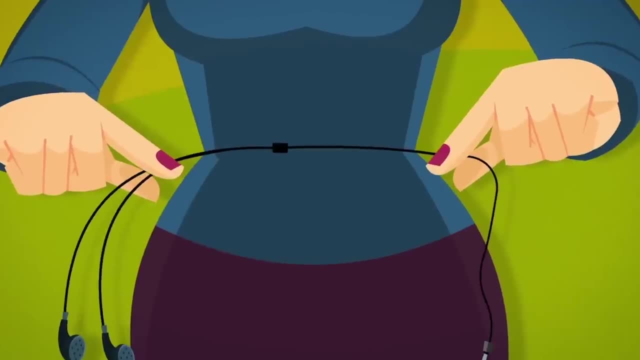 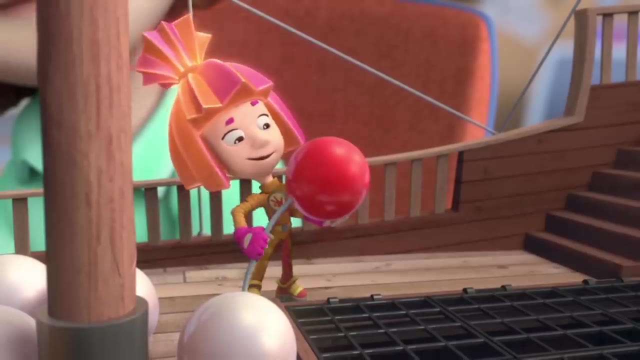 if you're tied with a proper knot. But sometimes things can get knotted up by accident, And that's one time when you don't need to know how to tie knots, but how to untie them All aboard Like that. Now, the only thing left to do is tie a knot. 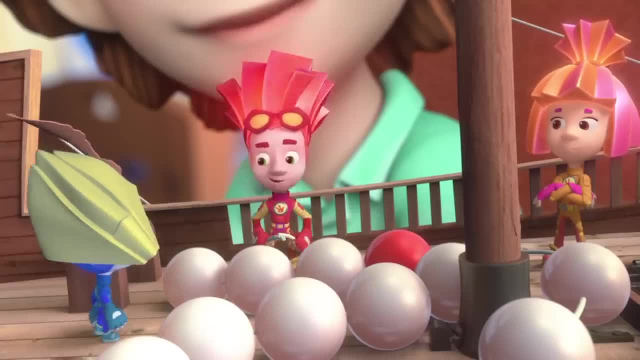 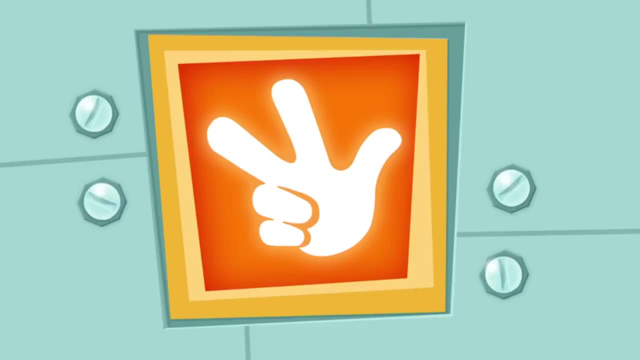 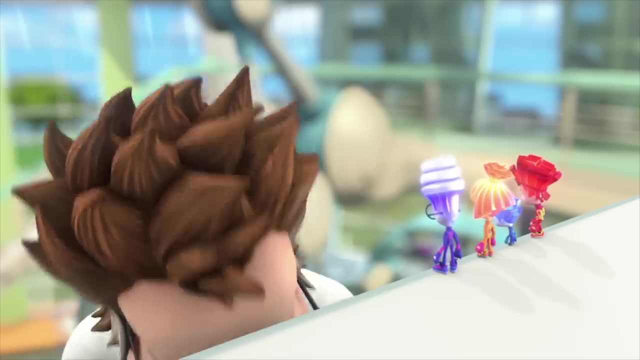 Should I tie it? Are you sure it won't untie? You're joking. Why don't you go ask Chewsocka and tie a knot like a sailor? The motion sensor. This part has to be replaced with one that's new. 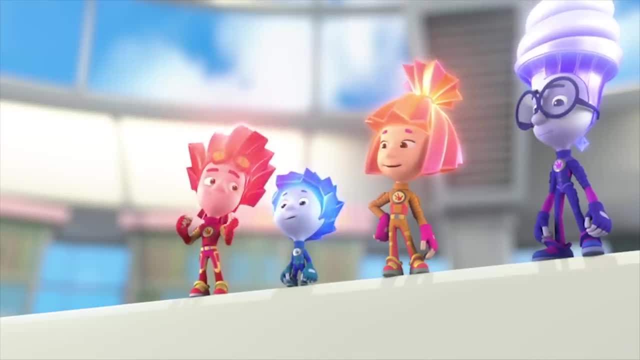 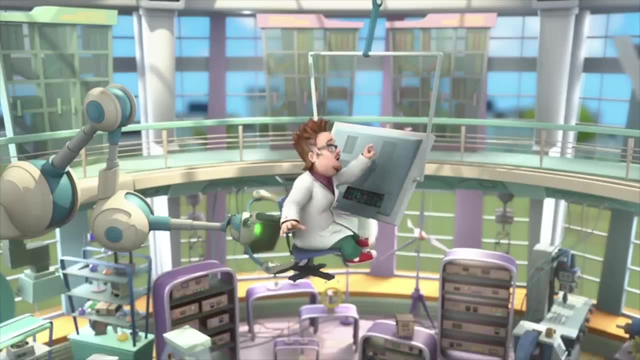 I've got an idea: How about we run to the warehouse and get it, Because you don't have time to go there, And that way you can keep on working? All right, then, Only remember the code for the part A-8375. 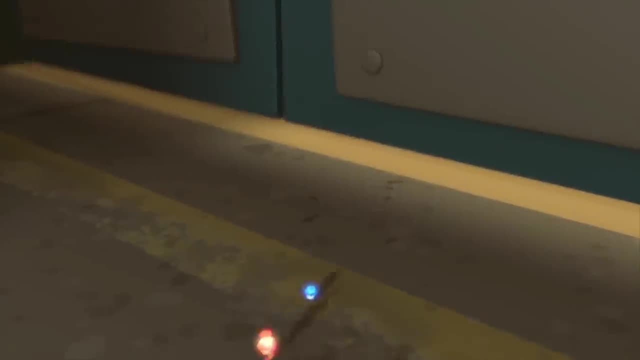 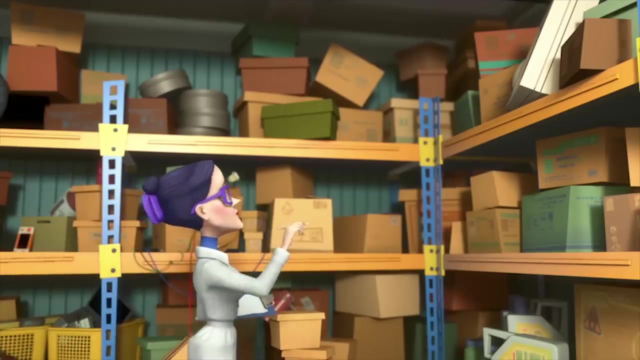 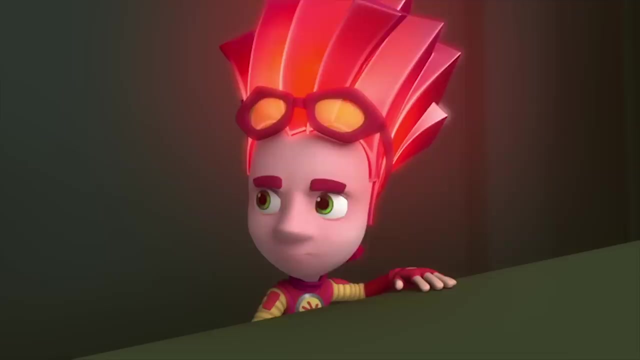 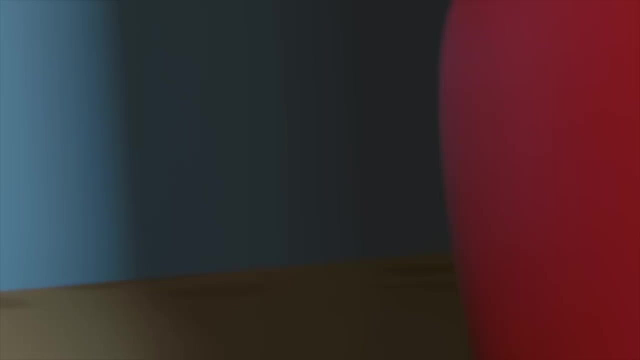 I'll remember it for sure. All right, Why is Lisa always there at the wrong time? Do we have to wait till she goes away? What for We'll sneak out behind her Digit. did you find the part? It's here. 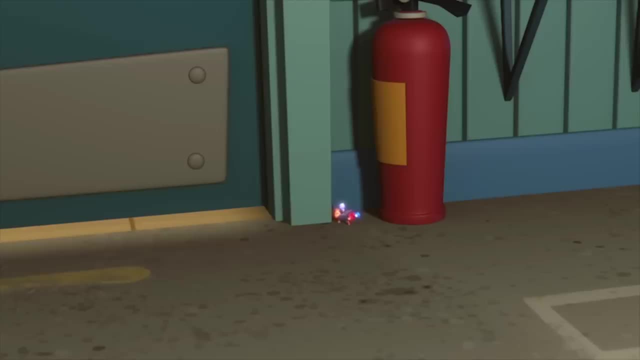 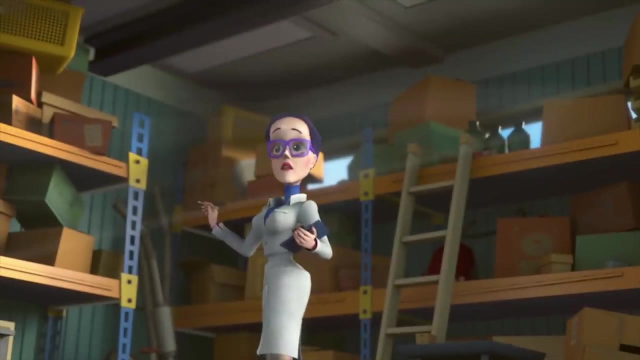 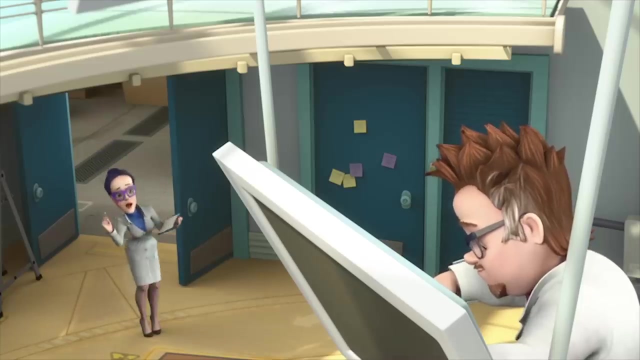 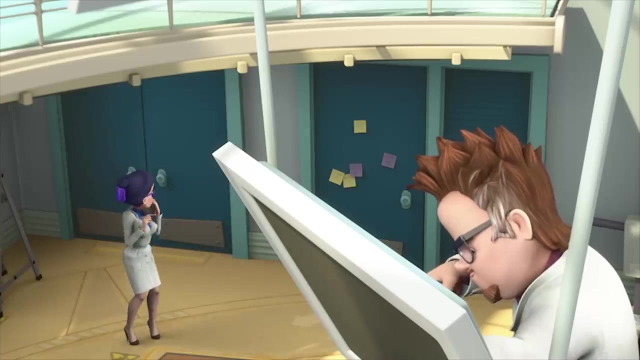 Are we ready? Yeah, we're ready, Let's do it. Huh, Professor Eugenius, you're in here. Do you know why this door just opened and closed by itself? Of course I know, Elisa, It's because I converted it into an automatic one. 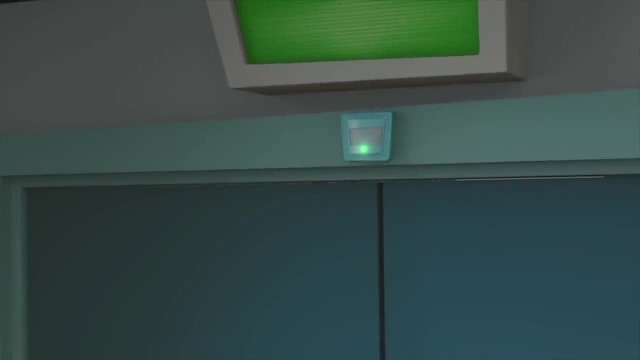 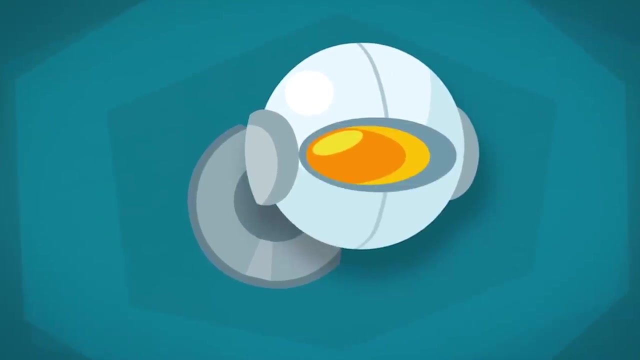 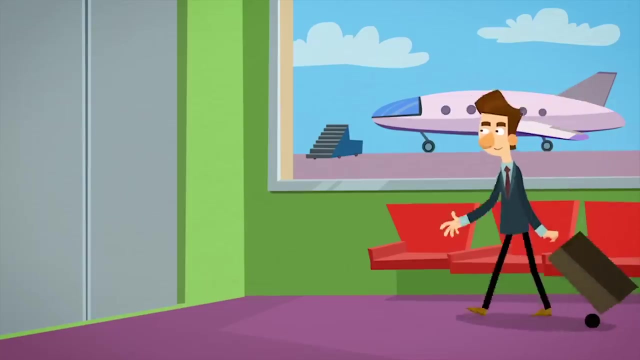 You see, I installed a motion sensor above it. A motion sensor. A motion sensor is like an electronic eye that watches everything that moves in front of it. Did you ever wonder how doors open by themselves at places like stores or at the airport? 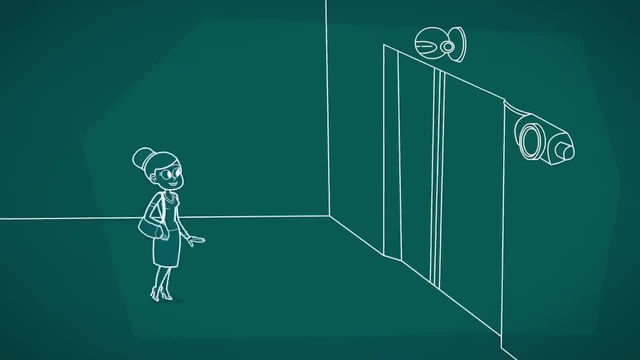 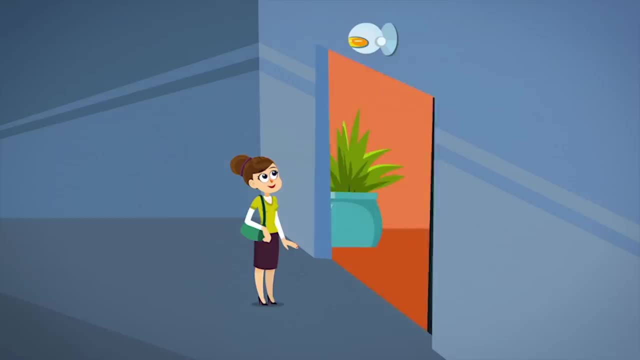 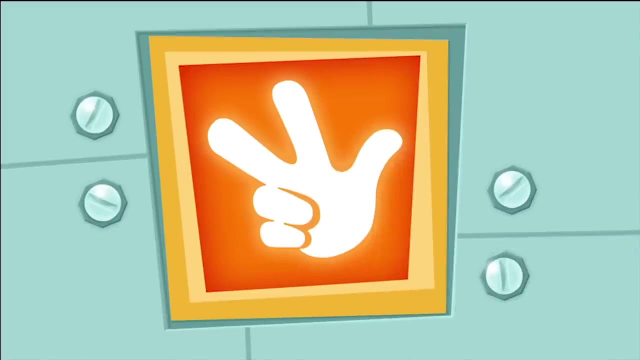 They open with the help of motion sensors. If the sensor sees that someone walks up to the door, it sends a signal to the door's electric motor. The electric motor opens the door and then automatically closes it after the person walks through it. That man is just astounding. 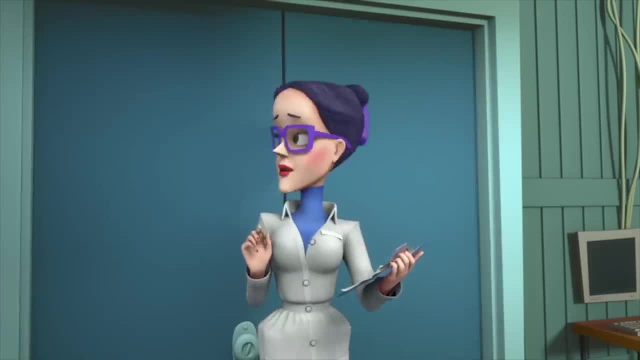 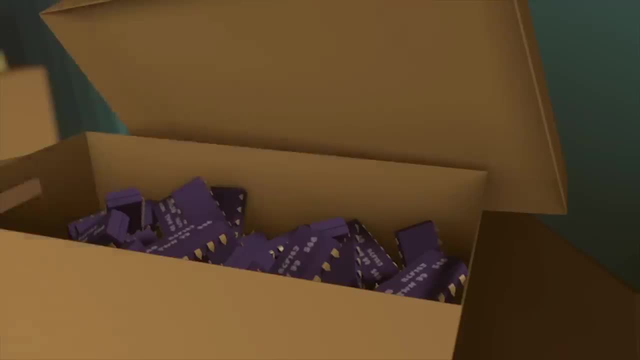 Only a bit untidy. The door is automatic now. Then why didn't it open for us on the way here? Because we're too little for that motion sensor, But the part's bigger than we are, Big enough for the sensor to see it. 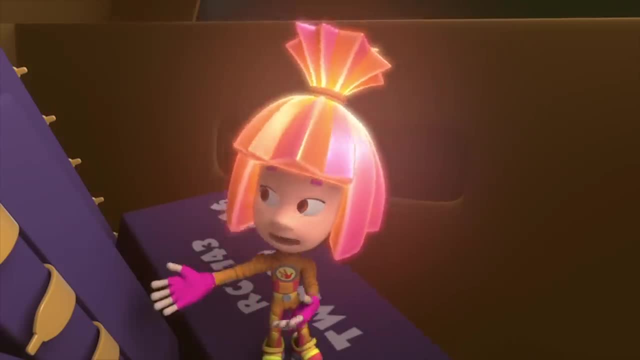 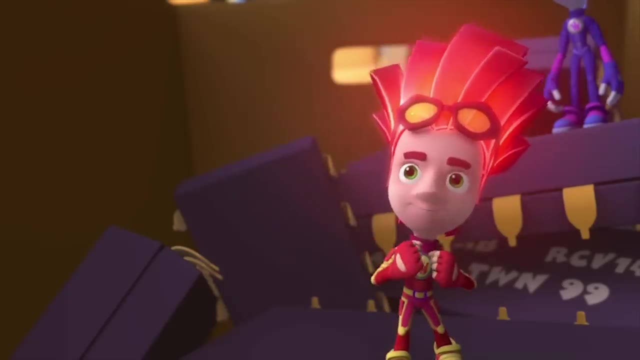 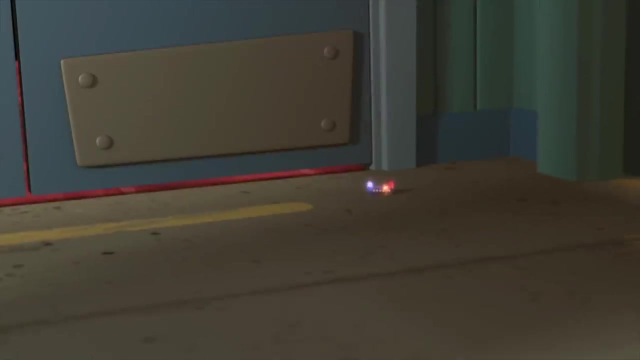 Then how do we get in there? We can fool that thing if we stay close by the wall. But how do we get in there? Well, we can fool that thing if we stay close by the wall. Now, let's keep this as close to the wall as we can. 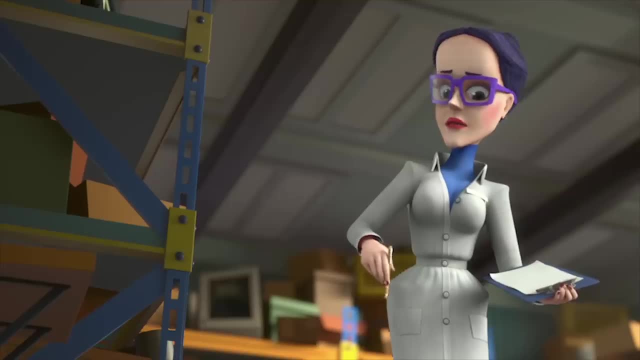 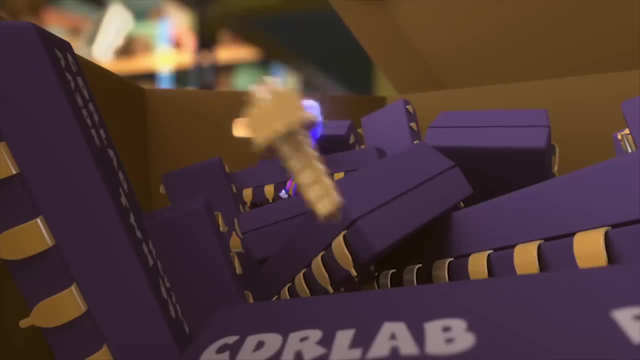 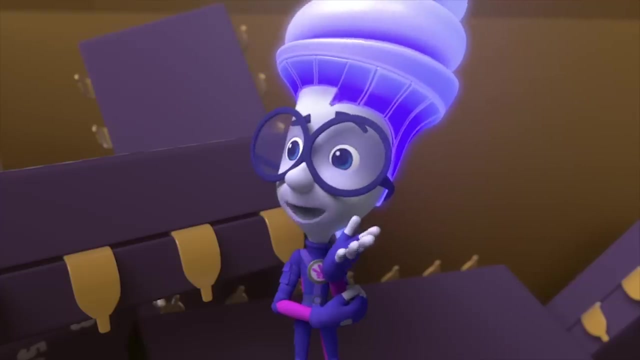 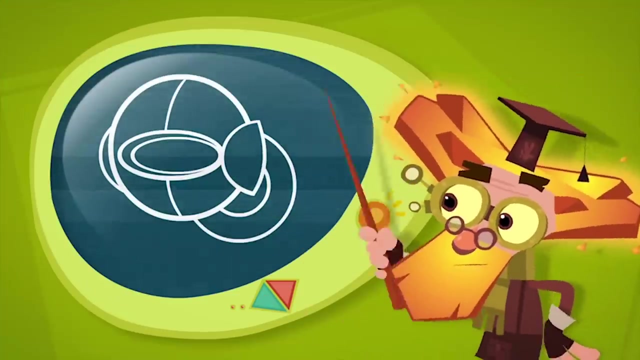 This door is a little too automatic. And these parts are here again. Didn't I put them away? The sensor still noticed us. Here's what we gotta do: Let's break it. All we have to do is deactivate the unit. Sensors are used. 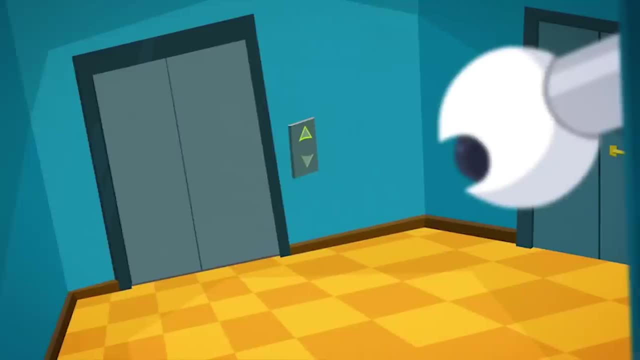 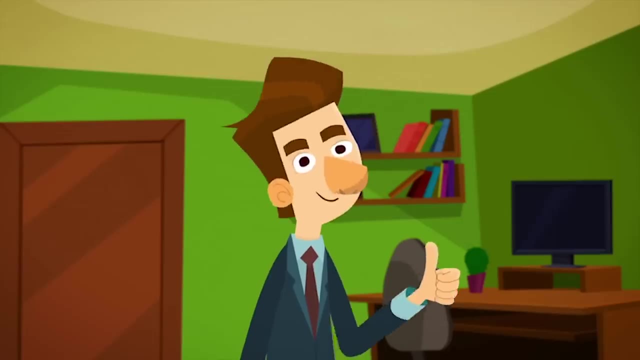 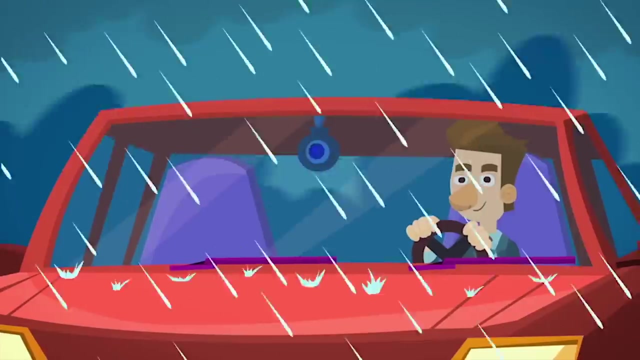 to help people in all sorts of different situations. For instance, motion sensors notice when someone is moving, so they can automatically open a door or turn on a light. Some automobiles are equipped with rain sensors. If it starts raining or snowing, the sensor automatically turns on. 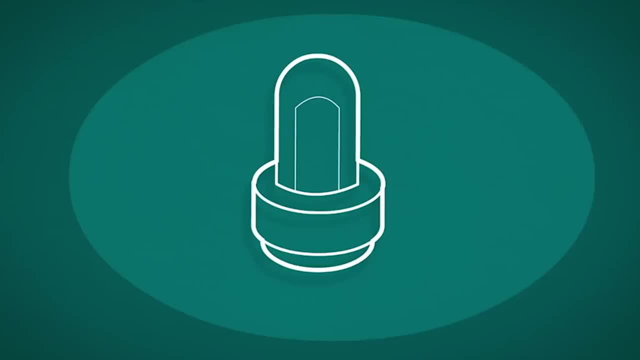 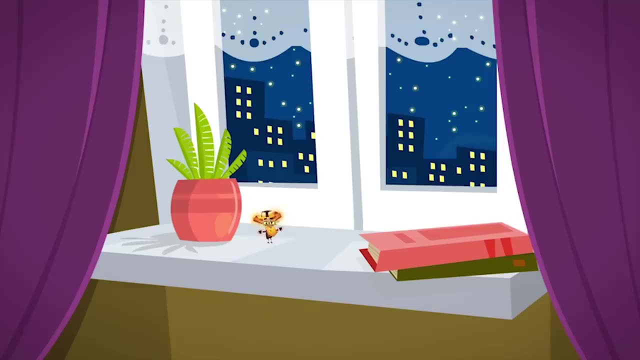 the car's windshield wipers. There are also sensors that react to how much light there is In the evening, when it gets dark. light sensors can be used to turn on street lamps And in the morning, when it gets light again. 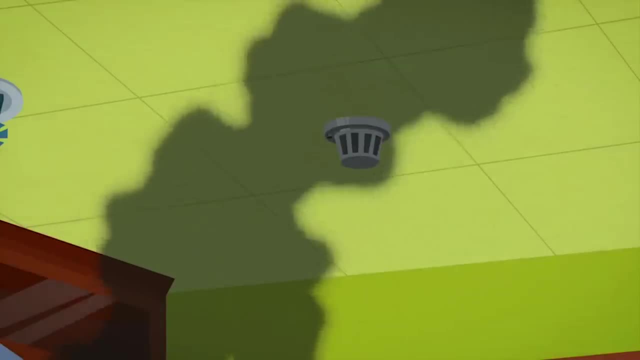 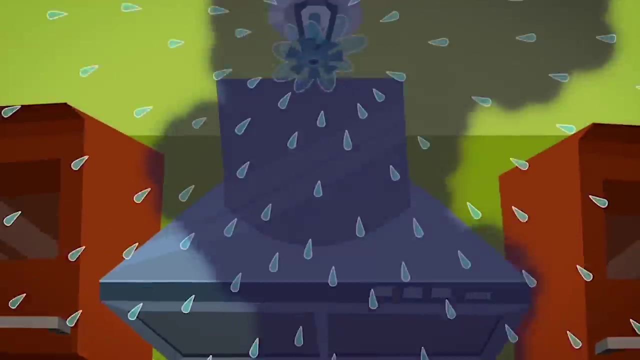 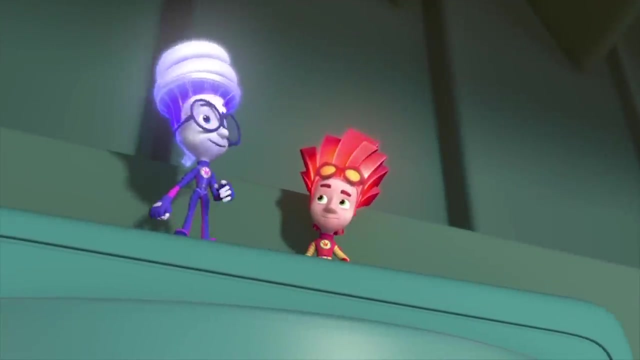 the sensor switches them off. A smoke detector can sense when there's smoke inside. The sensor can be used to turn on a fire alarm or even an automatic fire extinguishing system. I turned it off. It's a trick. Great job, Let's go. 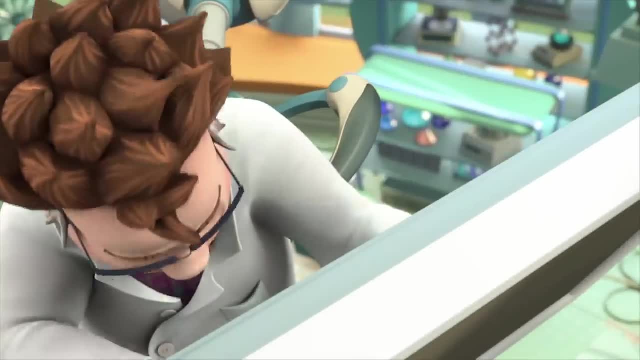 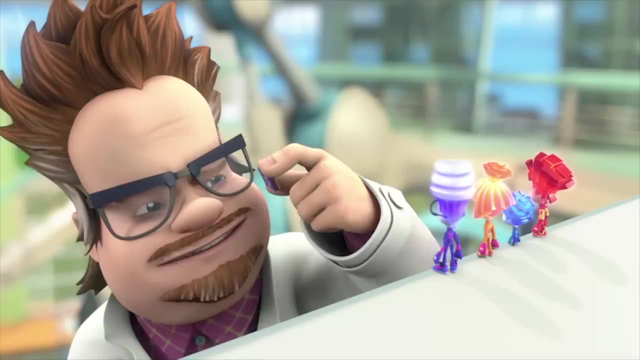 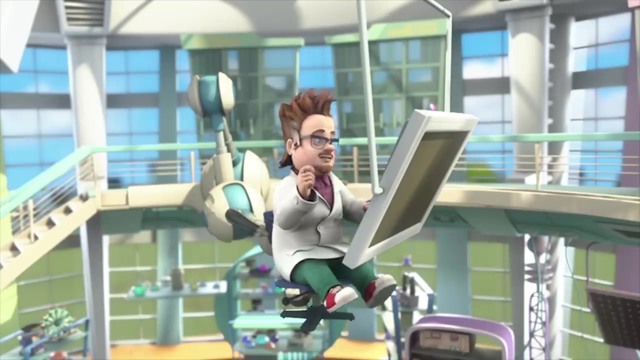 Tideesh. Professor Eugenius, Mission accomplished, Well done. Fixies Actually not that well. This part here is A7583.. And I asked for A8375.. Digit, Didn't you say you knew the code number? 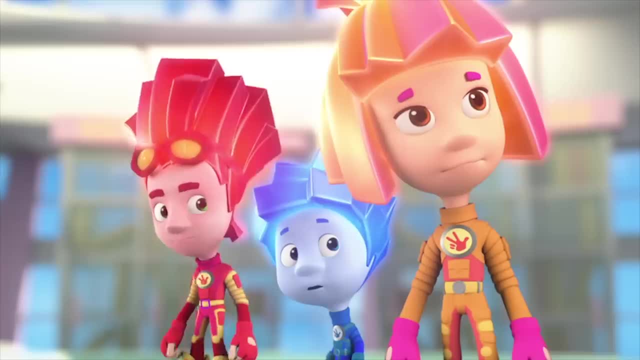 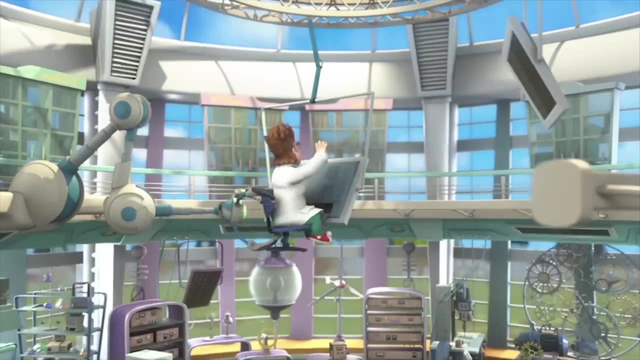 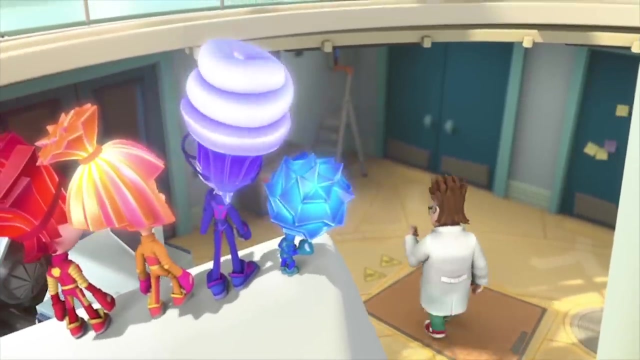 I did know it. I forgot it. Digit, I can't believe that you forgot it. All right, We'll just have to go out one more time. Thanks, but no, thanks, I'll get it this time. I forgot to warn the professor. 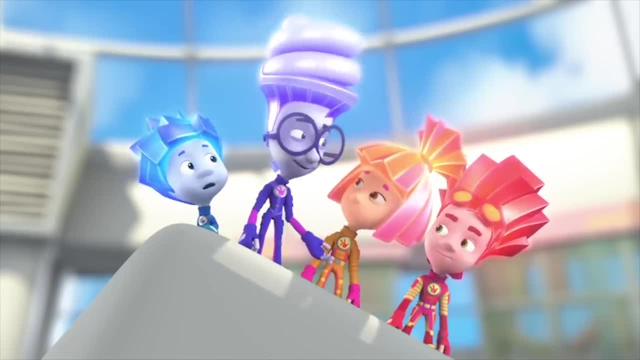 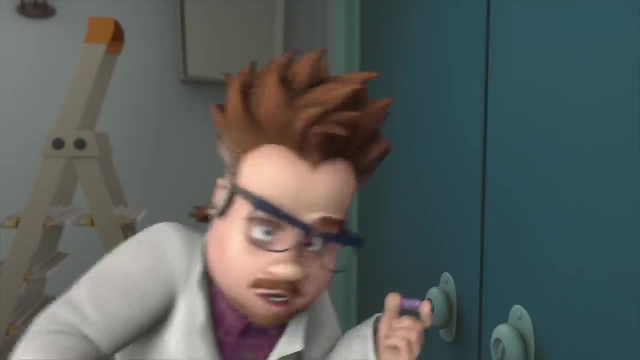 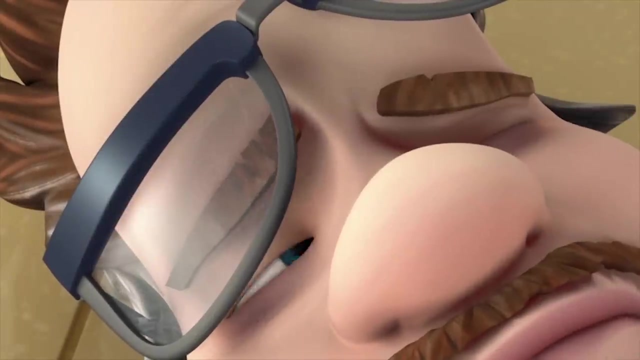 that we've turned off the sensor, And I'm afraid he's expecting that the door will automatically open up. Professor, Stop Ouch Gosh. Whoa, Whoa, I can't believe you're going through all this stuff. 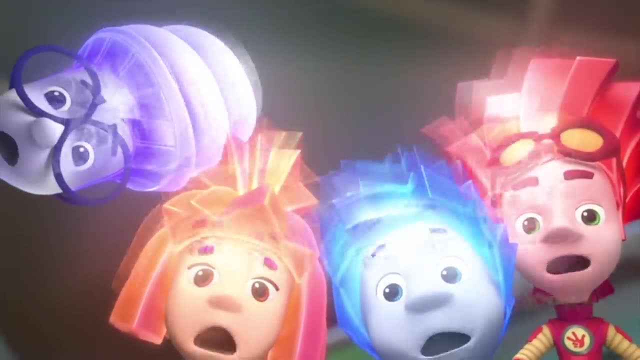 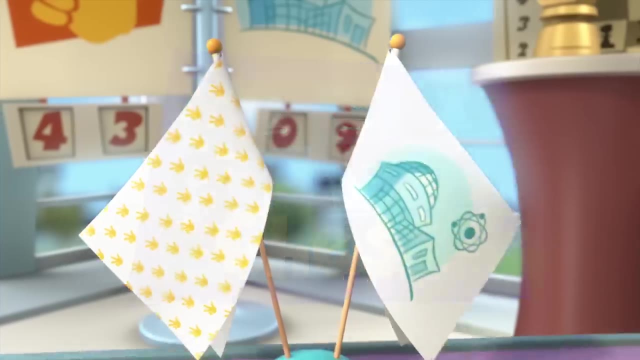 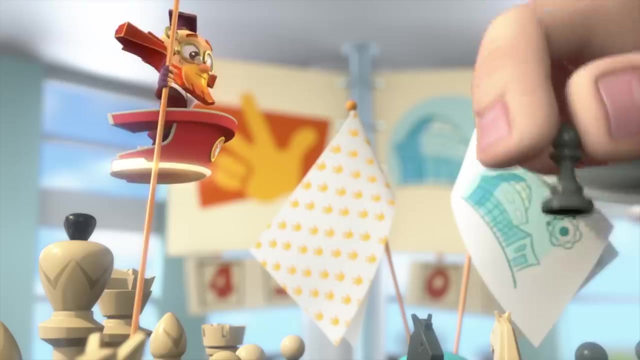 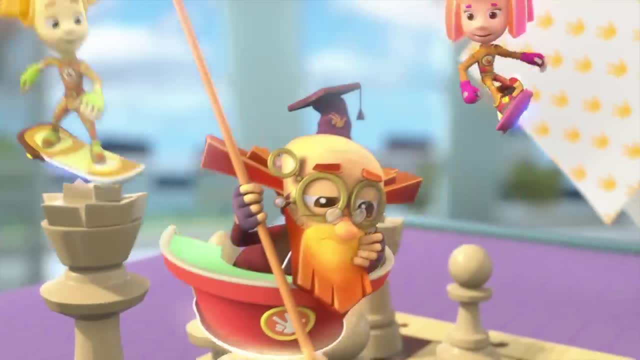 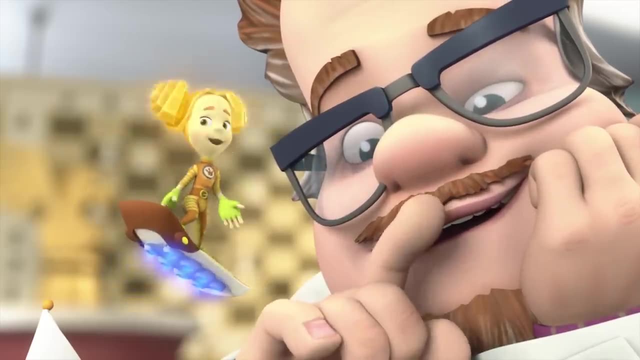 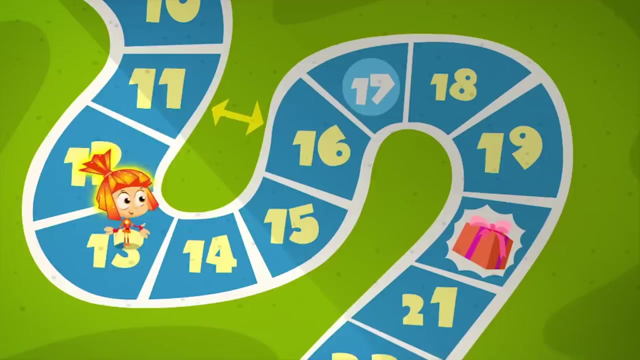 My paw Grandpus. we need our spool and it's missing. Congratulations, Professor. have you seen it anywhere, The spool? I haven't seen it. We're playing chess, can't you see? Do you like board games? 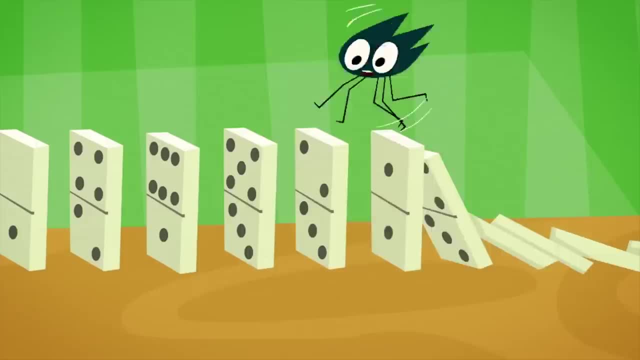 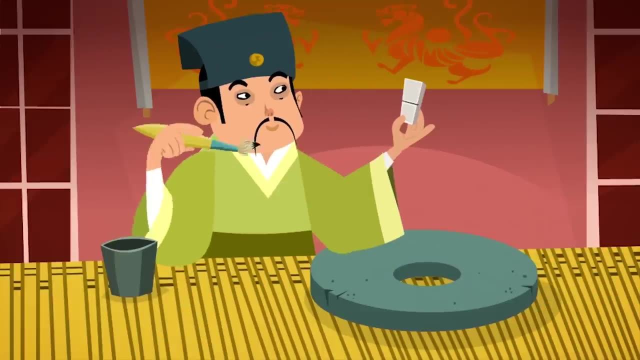 Like dominoes, for instance. Just about everybody has played it, But do you know where it came from? Dominoes was invented by the ancient Chinese. They made tiles and decorated them with dots, like on a pair of dice, And this is a game that looks a lot like checkers. 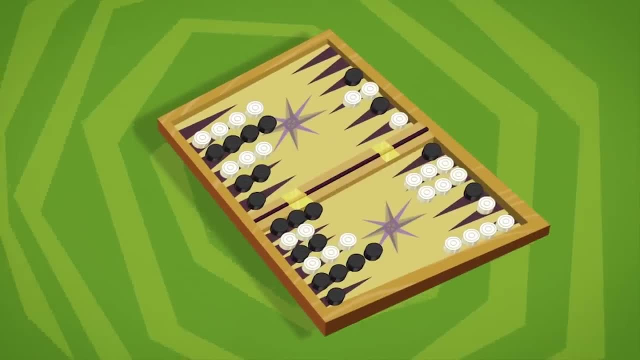 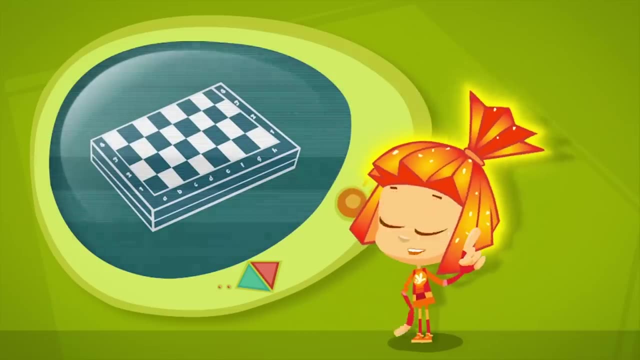 but it's a lot more challenging. It's called backgammon. Backgammon originated in Persia and from there it spread all over the world. But the most challenging game of them all is the game of chess. Chess was invented in India. 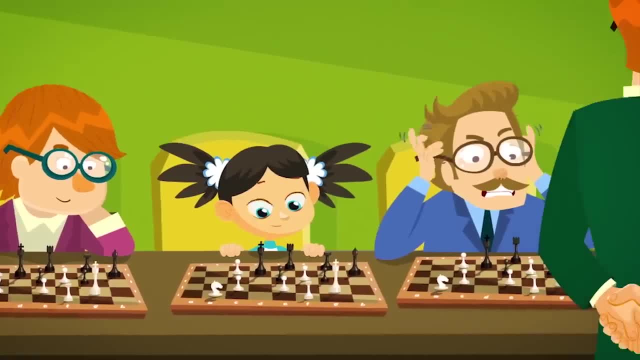 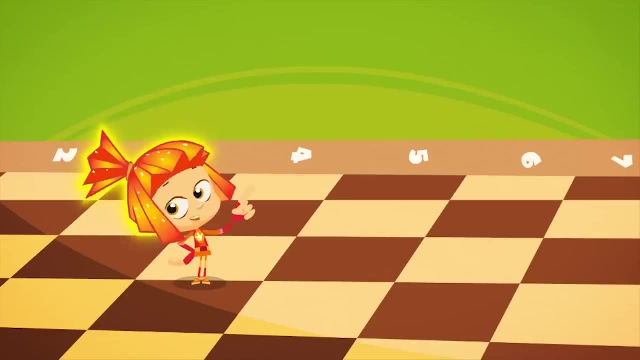 and today the game of chess is loved in every country. It's played by adults, by children and even by computers. Chess is a real sport. But the most important thing for playing chess is not the power in your arms, but the power in your brain. 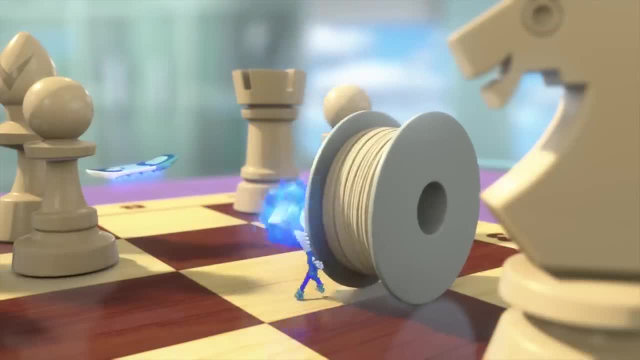 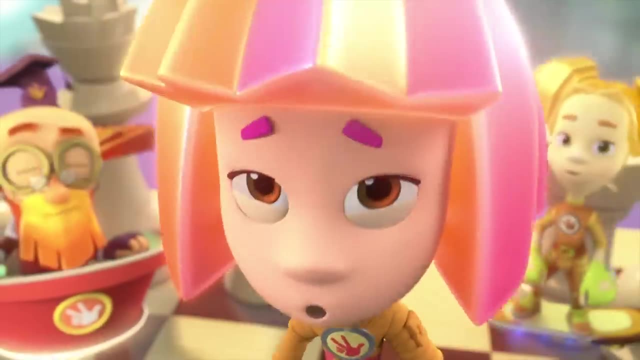 Hey, look, I found it. Hey, what's going on? That's our spool. Please let us take it back. There's something we have to do with it, But we're using it. Can't you wait? It's a replacement for the missing pawn. 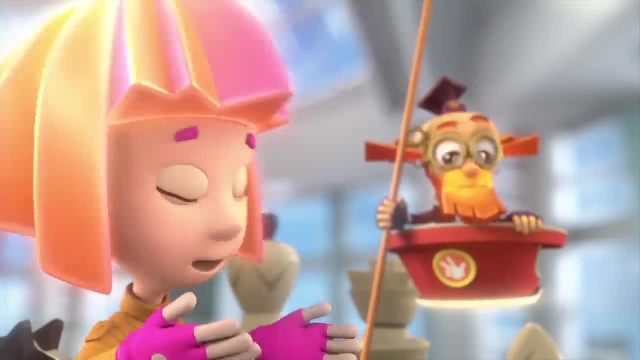 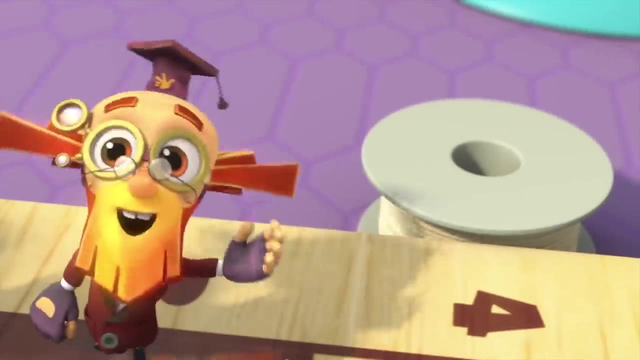 Oh, Oh, Nolik can work for a while. It's the pawn's replacement. Yeah, I can do it. Alright, you can take it And you stand right over here. One, two, three up we go. 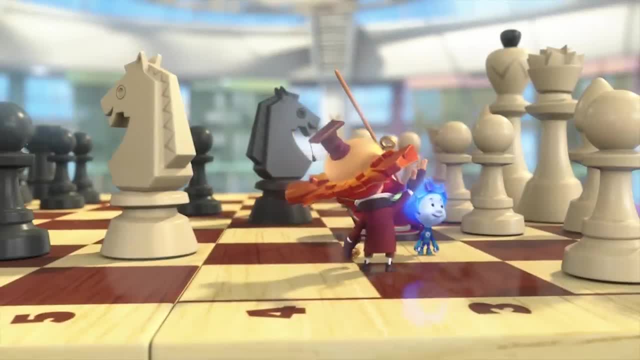 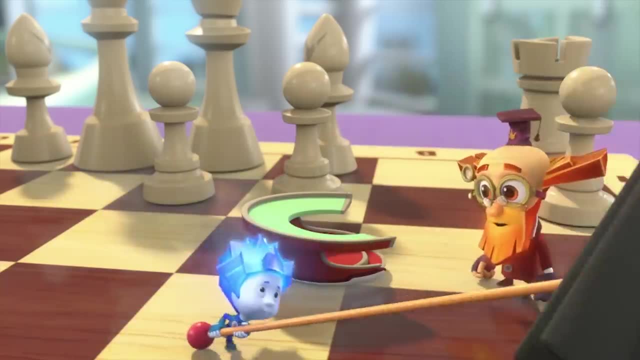 Class. So how do we play? You're going to play for the whites And now I'm going to capture your knight And we… We're going to knock over yours. Take that. Whoa, whoa, whoa, young man. 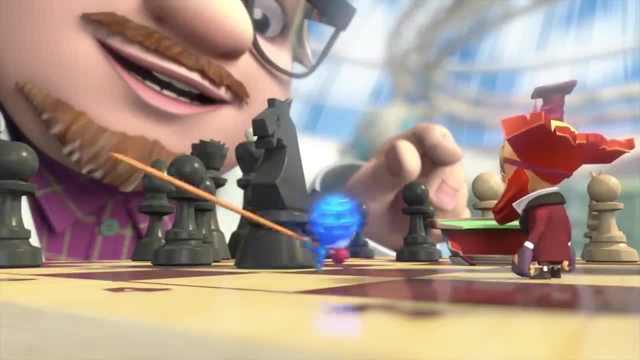 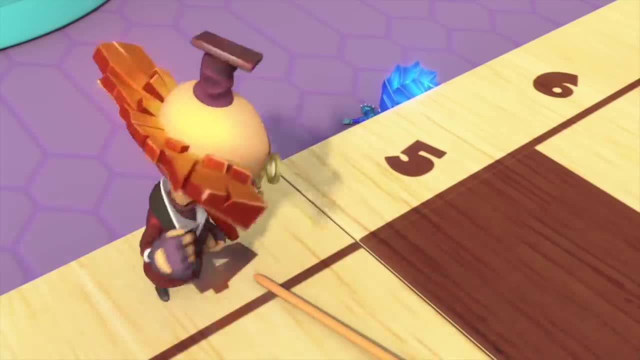 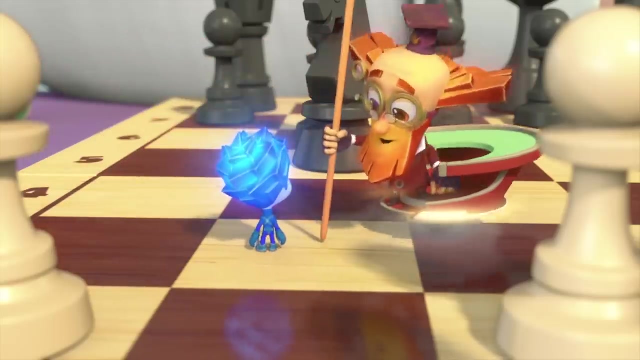 Slow down, It goes…. Back here, Nolik, get back to your square. What for Pawns don't move like that? Then how do they move? Only one square per move and only forward. Of all of the pieces, the little pawn is the weakest. 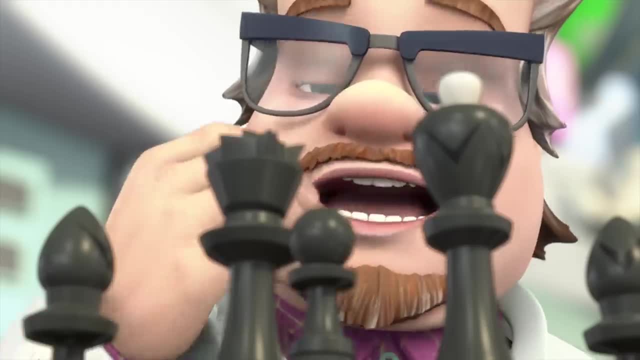 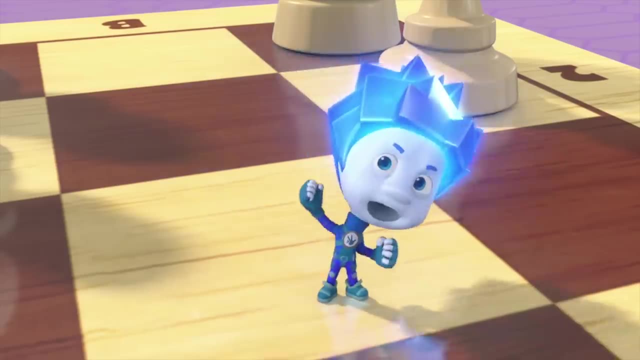 What a mess. So which one's strongest? huh, This, It's the queen. She's the most dangerous threat to the other king. Aw, how come I couldn't be queen, Then that black king would have to deal with me. 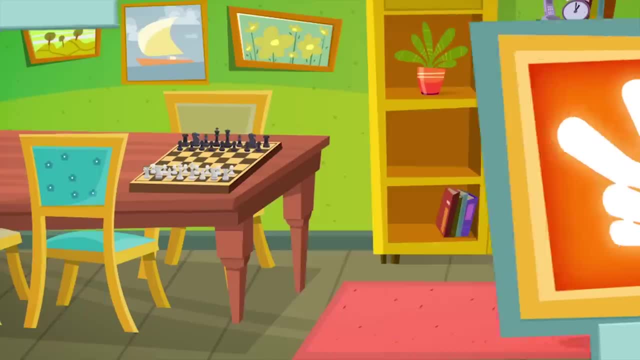 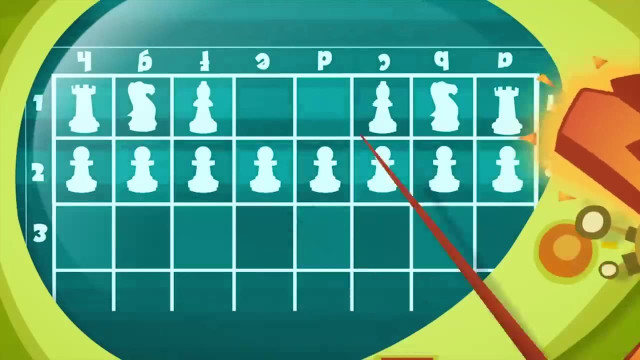 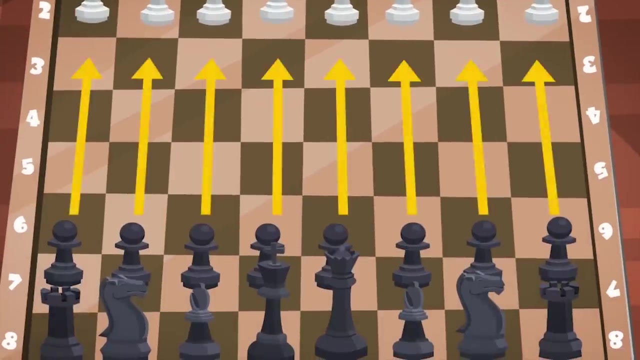 Oh yes, In chess, each player has a black or white army with eight pawns, two knights, two bishops, two castles and a queen. All of them work together for their king, trying to protect him while attacking the enemy's king. 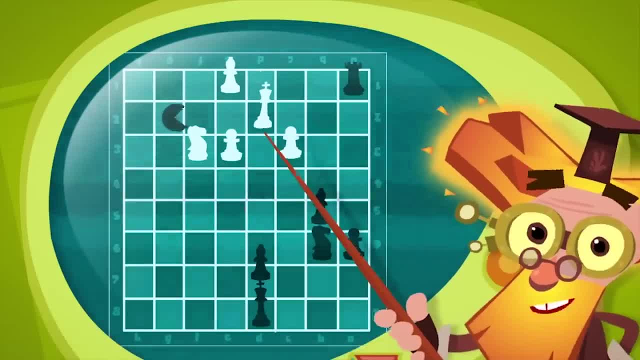 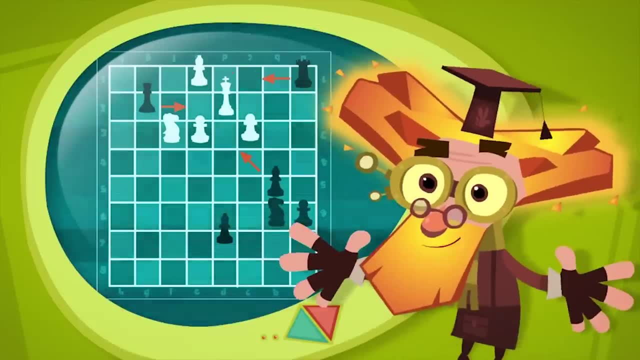 If the king finds himself in a position where he can be captured, the attacking player says check, And if the king finds himself with nowhere to run from the attack, it's called checkmate. Whoever checkmates the other player's king first is the winner. 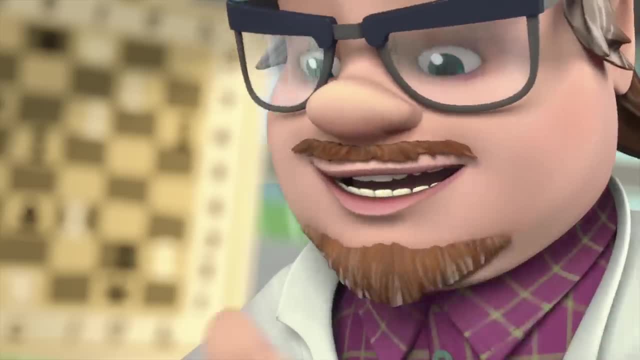 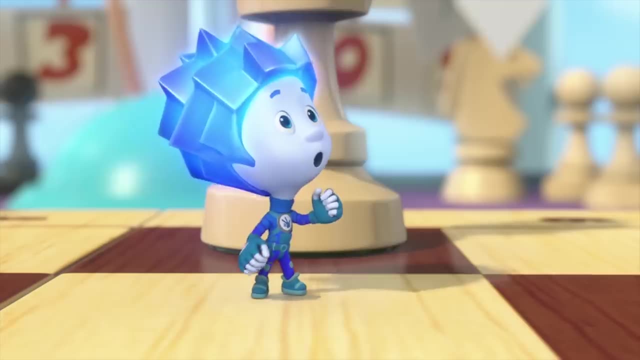 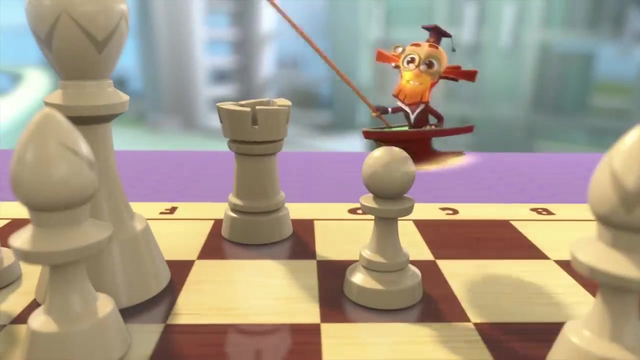 I'll move my queen, Yeah, And me my queen. Then I'll just capture your queen. Aha, Really, Then I'll just capture yours. Grandpus, should I go now? Not yet. So do you feel like surrendering? 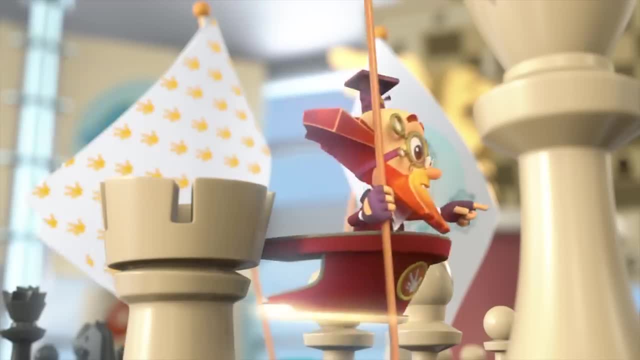 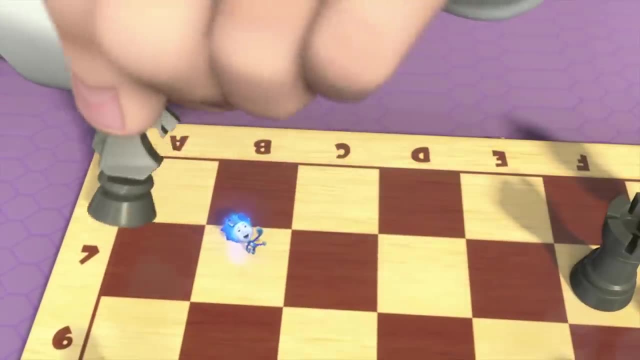 Ha, You're kidding, do you? Nolik, forward, Hurrah, We'll step aside Forward, Aha. Next I'll go and capture the knight He got away. Alright, pawn and once more, go forward. 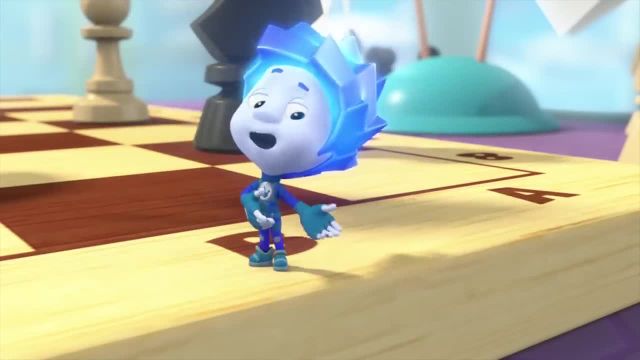 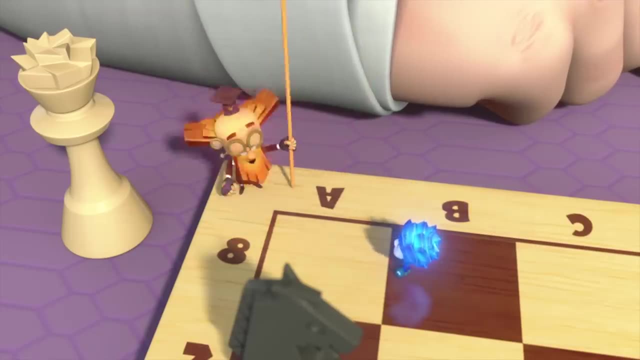 Grandpus, where do I go now? Don't you see the edge? Don't go anywhere Now. you're the queen. What? The rules of chess say that if a pawn makes it all the way to the other side, he can become anything that was captured earlier. 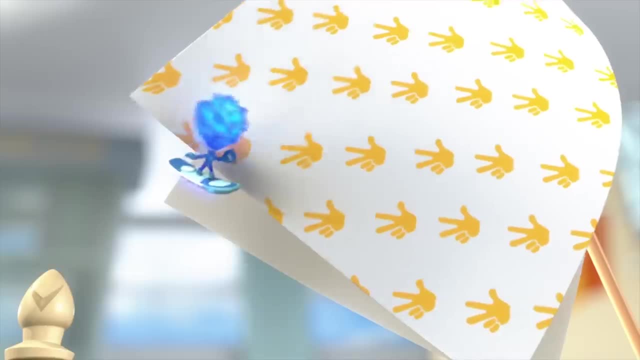 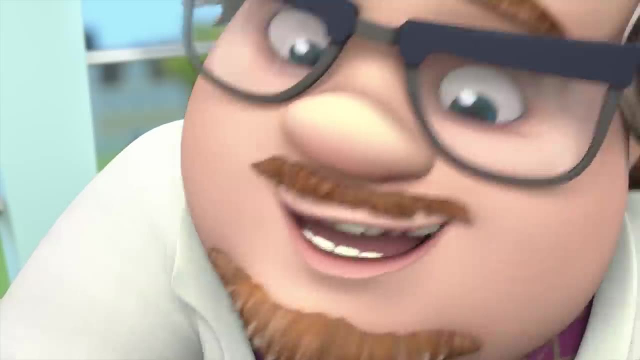 Hurrah, Then I'll be the queen And I'll be the strongest piece in the whole game. Hey queen, Get back here. In case you don't know, this isn't over yet. We capture the pawn with the queen. 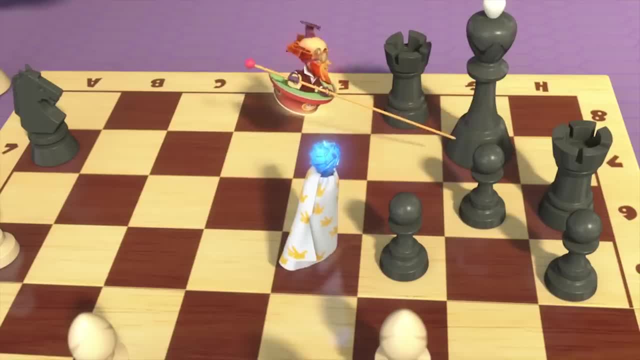 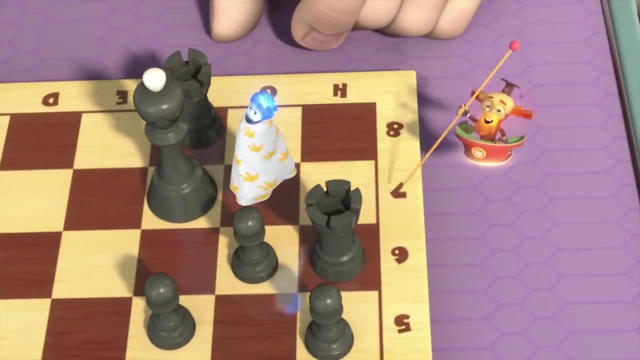 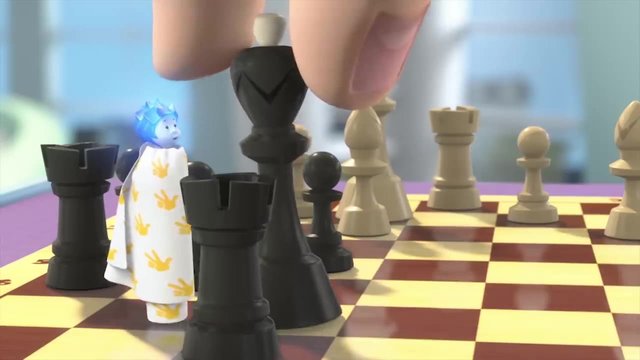 Queen, this is your new place. Check, Check, Huh, Yeah, Heh, Now come to here, Checkmate my colleague. Of course it is. It is mate. Yeah, I lost Hooray. Tideesh, Tideesh, Tideesh. 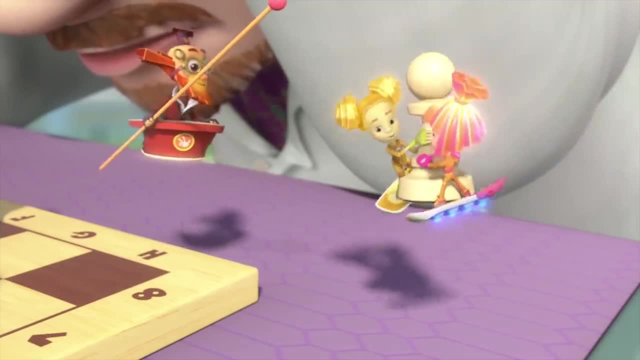 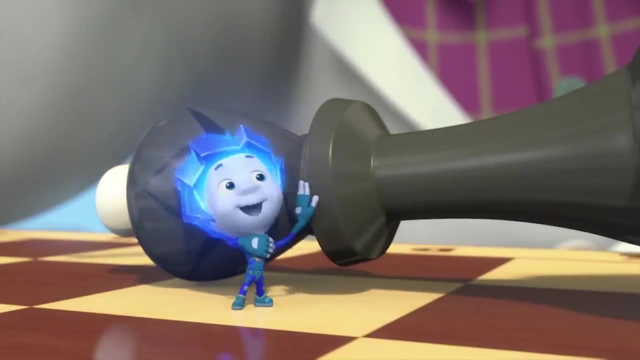 Professor, we found the missing pawn for you, So that means Nolik can leave with us. I'm not going anywhere with you. Chess is the greatest game you'll ever play in your life. Oh, you should have seen how I put Professor Eugenius in a checkmate. 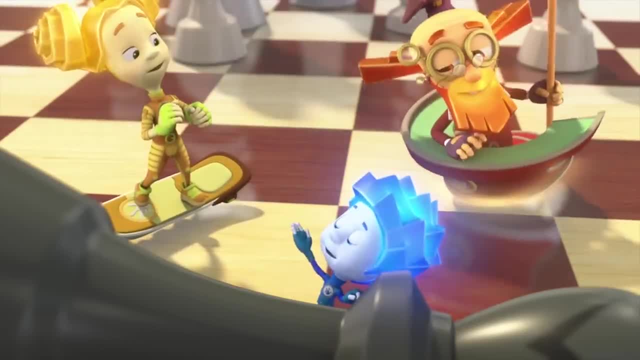 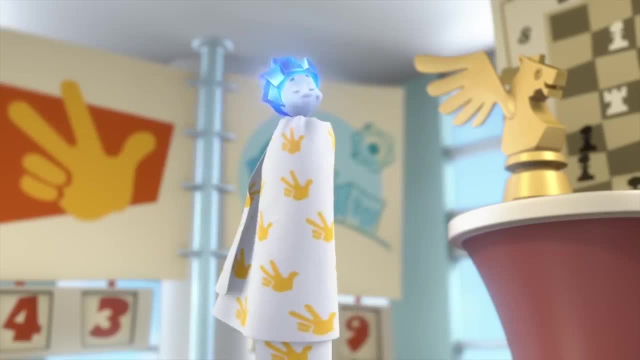 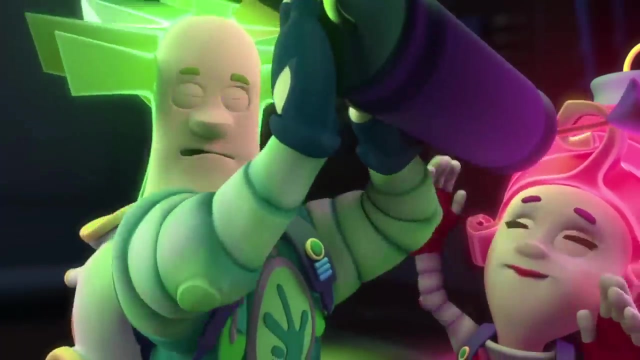 Really Well. Grandpus helped me a little. Actually, it was Grandpus telling me where to move. Huh, But I'm the queen now. Papus Masiya, we've got to hurry. How come Tom Thomas is going to see the circus? 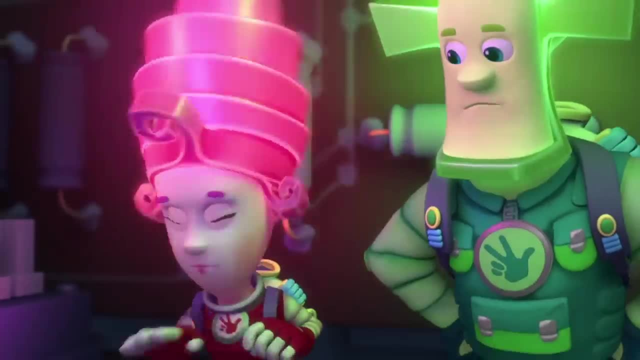 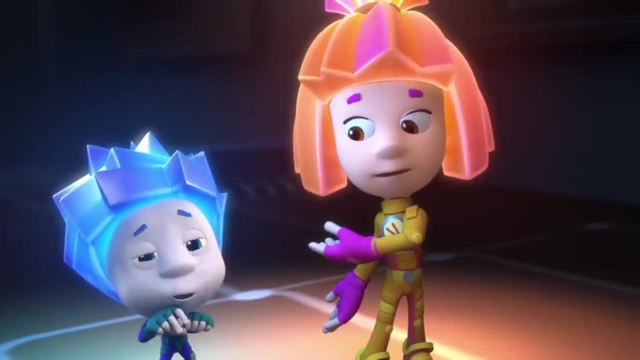 Ugh. And what We want to go with him, can we? The answer is no. Just you, kids without supervision. Who said no supervision? His parents are taking him there. Well, be careful, Don't worry, They won't even notice us. 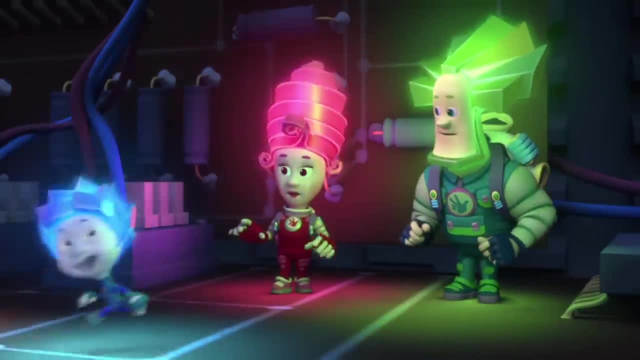 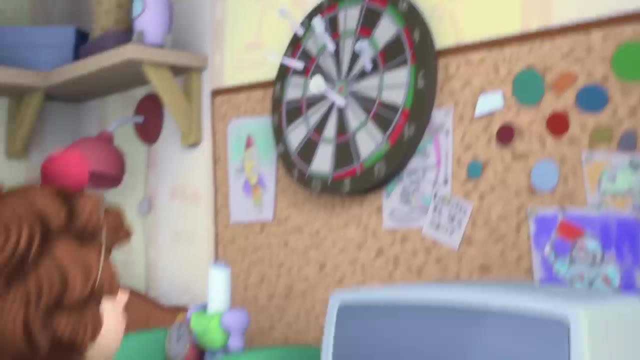 Hmm, Well, if Tom Thomas' parents will be there… Hooray, We can go Wait a second. I didn't even say yes yet. Yeah, Simka, Nolik, where are you? We've got to hurry up. 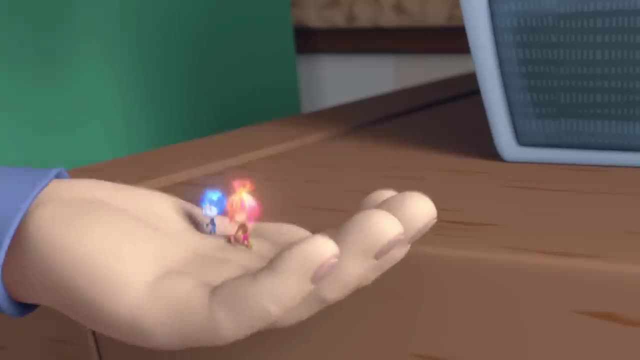 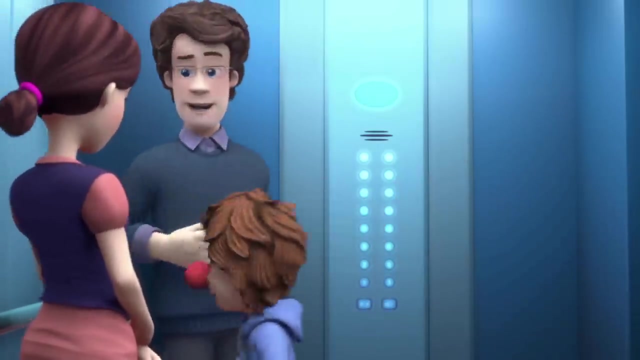 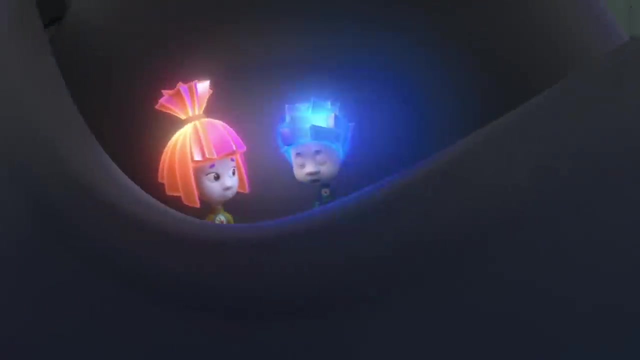 Tom Thomas, it's time to go. I'll be right there, We're ready. Climb into my hood. Ha, I know who's going to the circus today. Whoa, Huh, What just happened? I think that the elevator broke down. 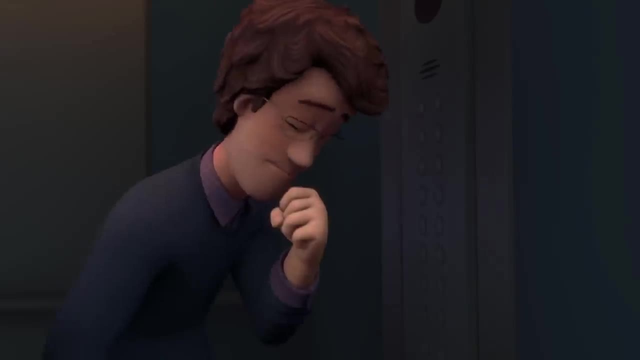 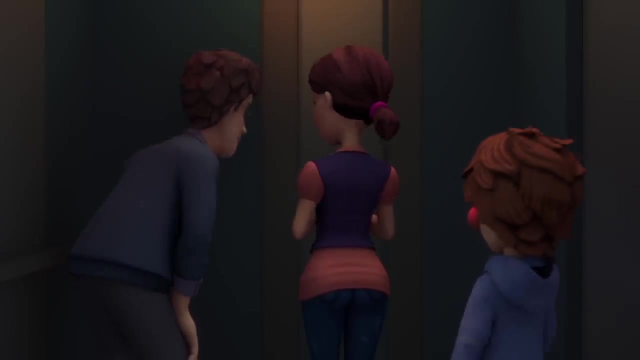 Don't you worry. Emergency operator. Um, we got stuck in the elevator… Understood. Please wait, We'll have the elevator fixed within the hour. That long That means we won't get to the circus on time. Tom Thomas, we'll go get Papus and Masiya. 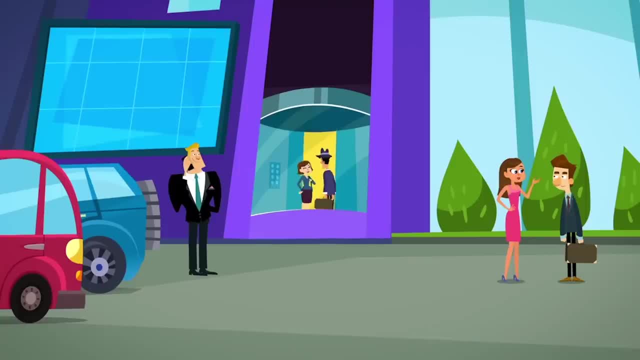 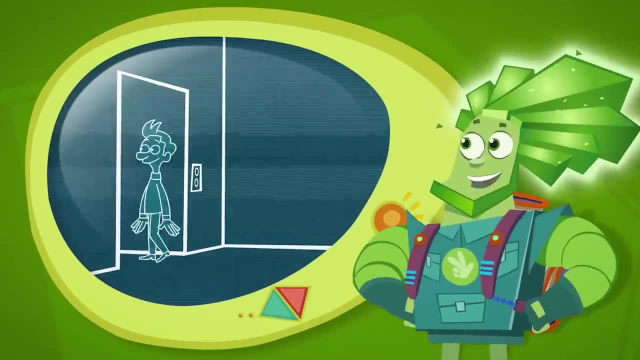 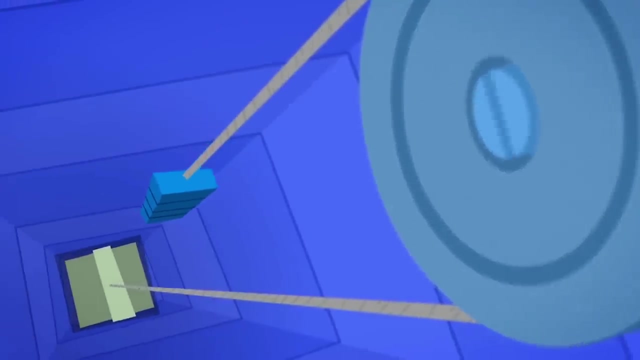 I'm sure they can fix it. People need elevators to help them get to the upper floors of tall buildings. When someone steps into an elevator and presses a button, the elevator's electrical engine starts up. It pulls the cable that is attached to the elevator cabin. 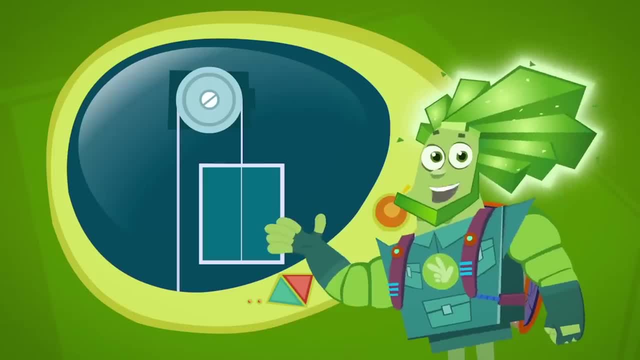 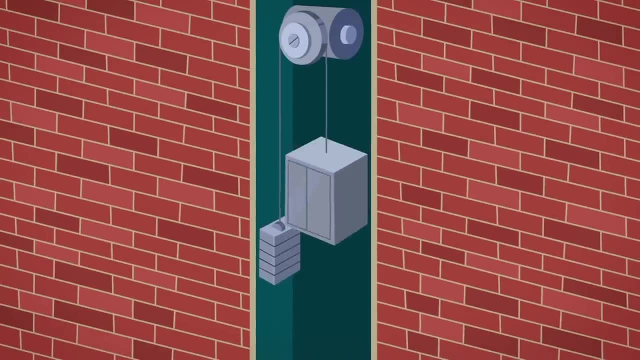 and the elevator goes to the desired floor. The cable hangs over a wheel and it usually has a heavy counterbalancing weight attached to the other end of it. This counterweight balances the elevator and helps the electric motor do its job. Oh, 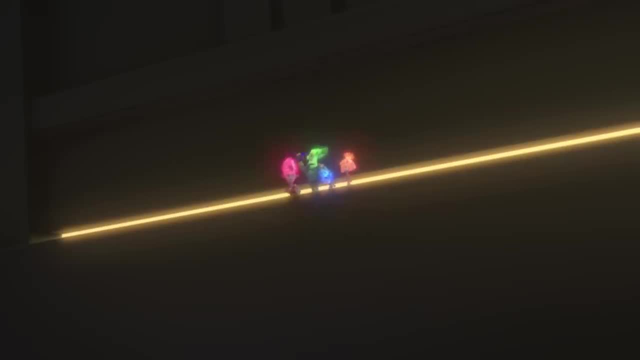 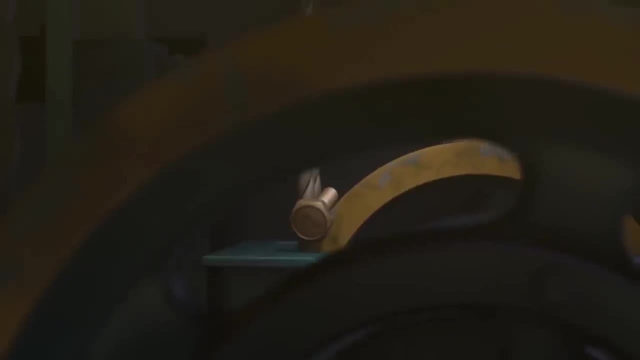 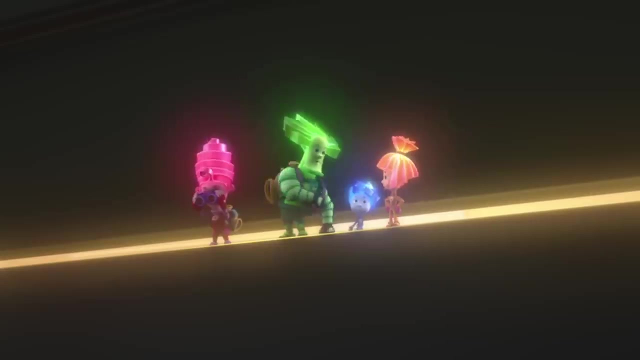 Oh, Oh, Hmm. I wonder what the reason is. I think I see something over there that got stuck. Looks like you found the reason. We gotta go and fix it now or we'll never get to the circus on time. You know, we can just have it right here. 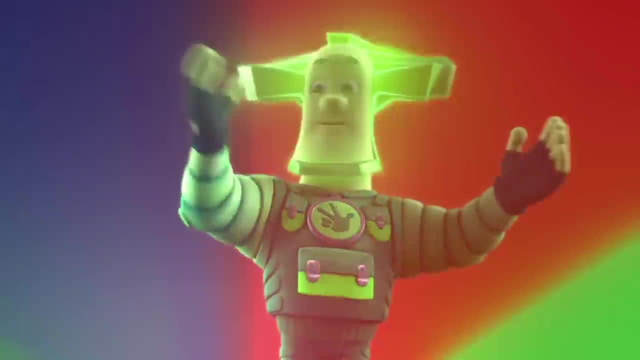 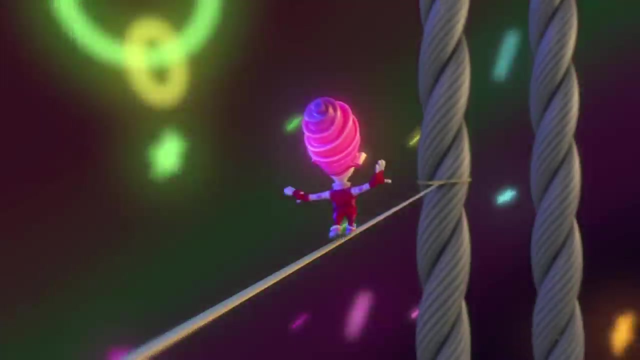 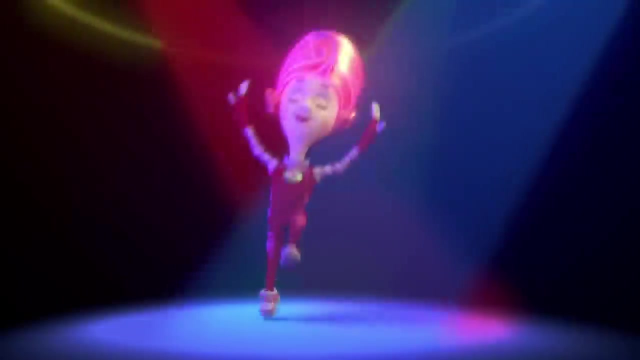 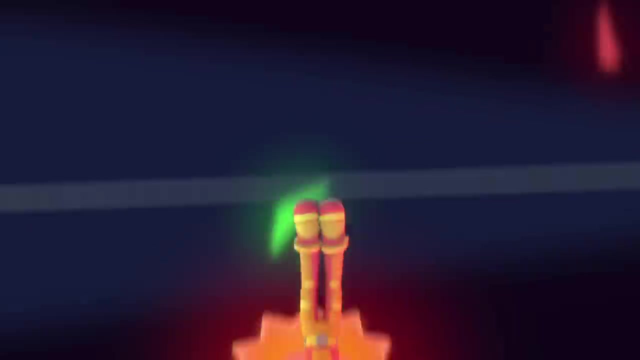 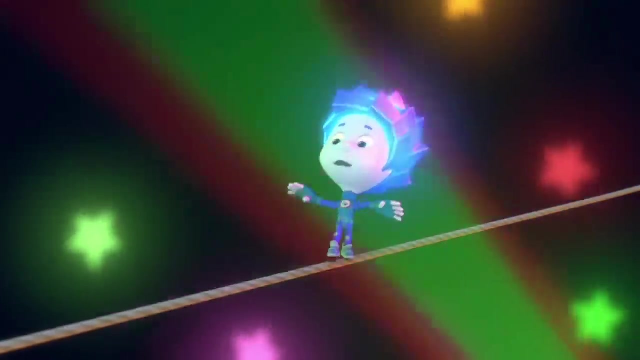 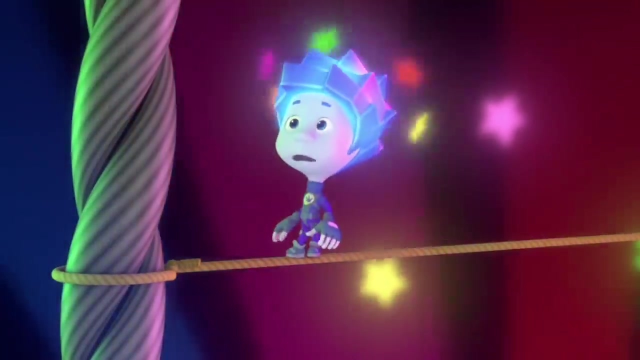 Ladies and gentlemen presenting the Fixie Spectacular. And now your attention, please, on the high wire, The Fast and the Furious. Whoa, Just don't look down, Then I'll close my eyes and I won't look anywhere at all. Ow. 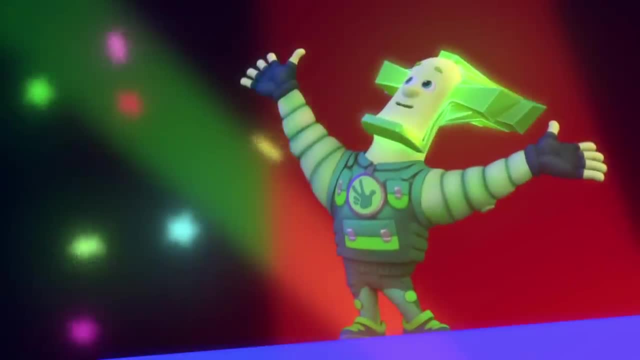 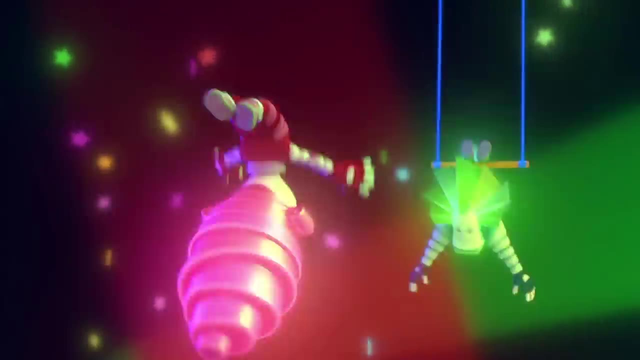 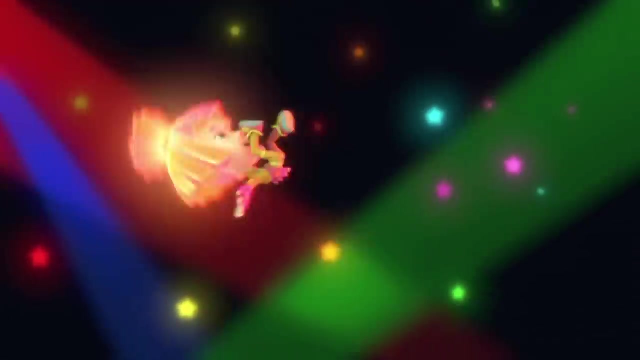 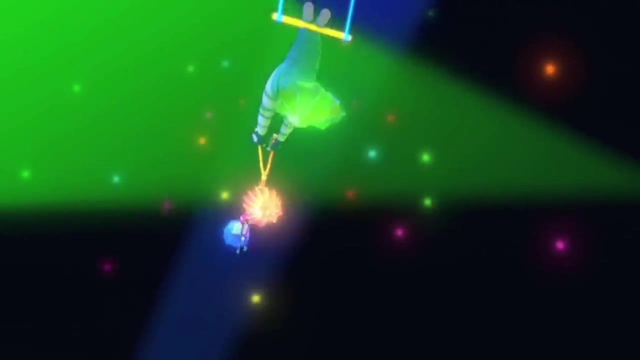 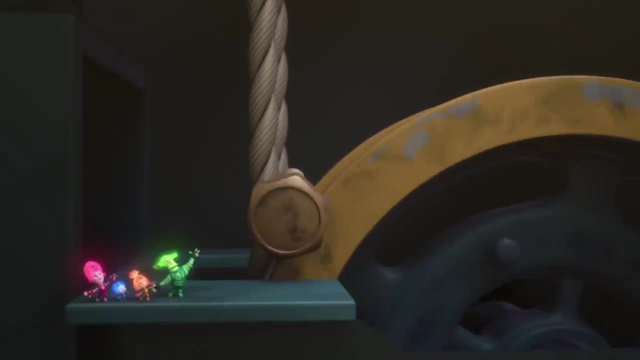 And now we bring you our very own aerial gymnasts. Uh-huh, Uh-huh, Hmm, Hoop, Hoop-pa, Hey, Hey, Yep Hoop-pa, Tideesh, Oh, Tideesh. Our next act: feats of strength. 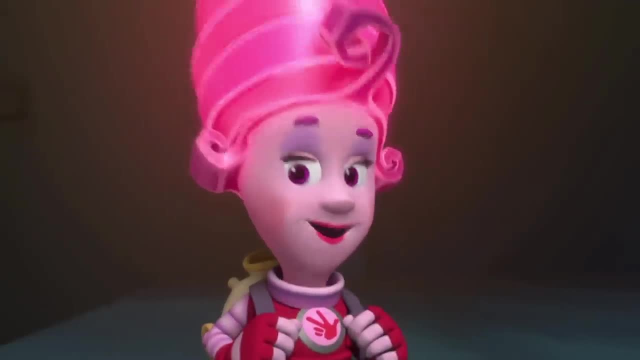 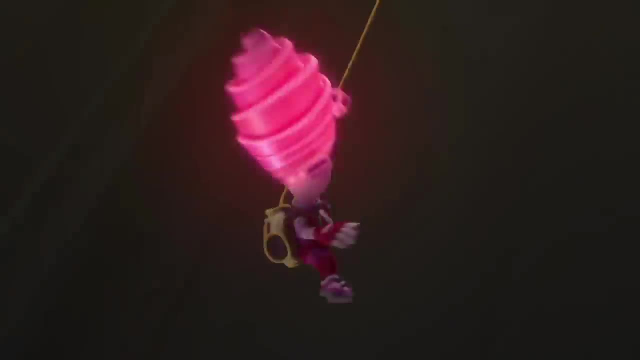 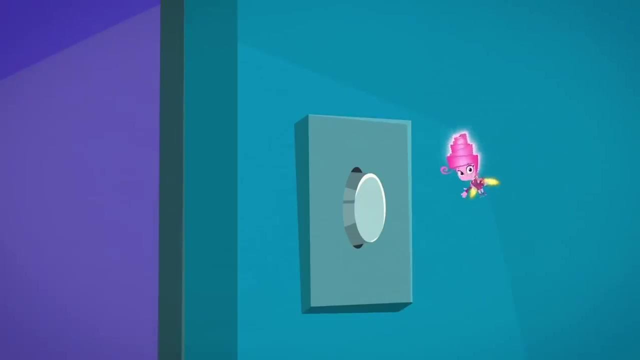 It won't come out. I know how to fix it With a death-defying circus act. Point your eyes up, Marzia. where are you going Up to the electric motor? Do you know the right way to behave yourself inside of an elevator? 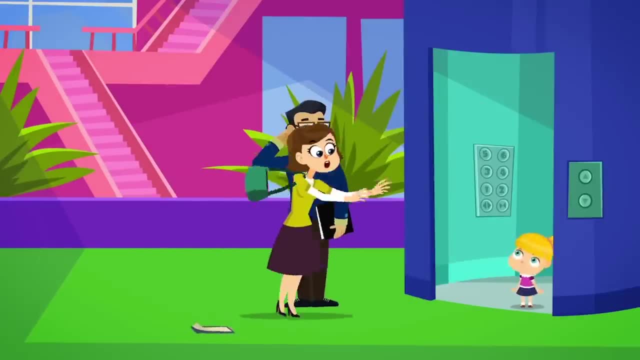 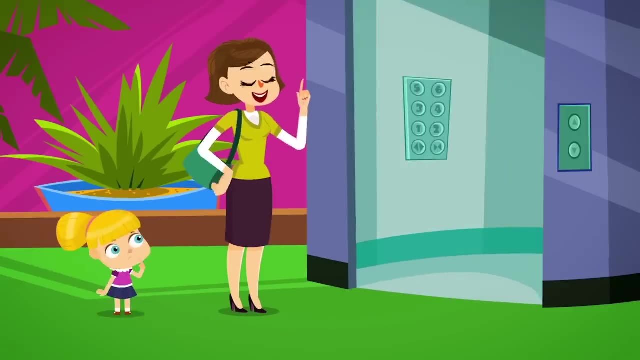 First of all, small children should never get into an elevator by themselves. They should only go in with their parents or other adults they know well. When getting on to an elevator, the adult should always enter first and then the child When it's time to get out. 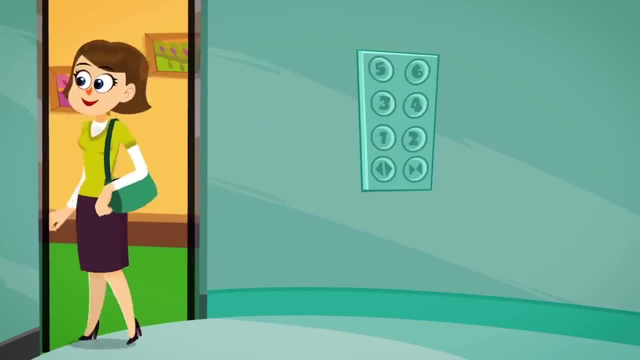 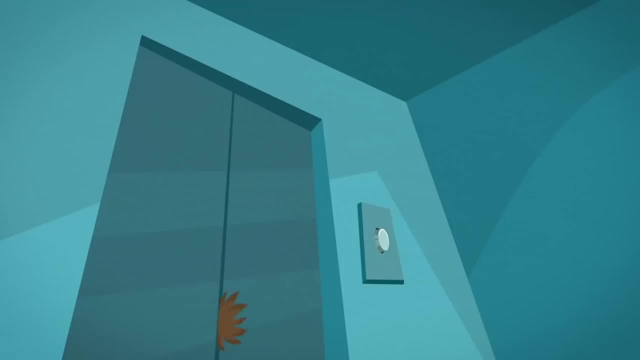 it's the other way around: First the child leaves and then the adult. If you are taking a dog onto an elevator, make sure its tail and leash are completely inside so they don't get stuck in the door. And there's one more thing. 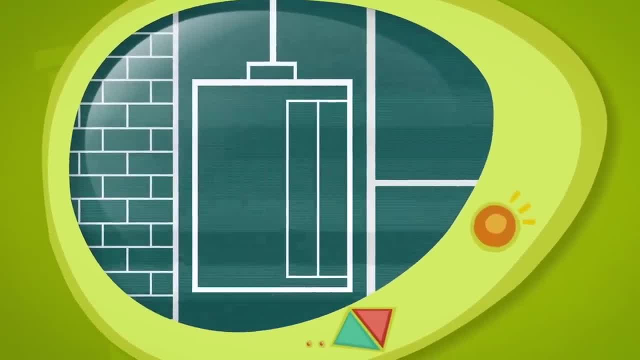 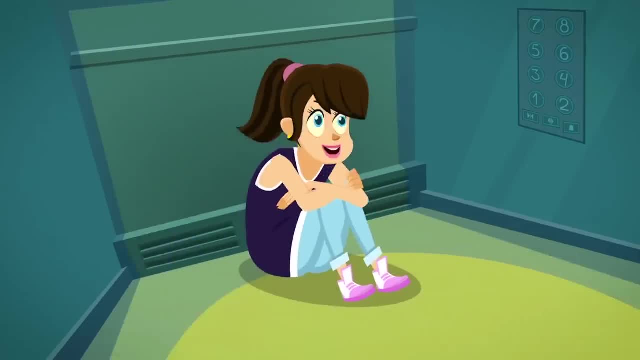 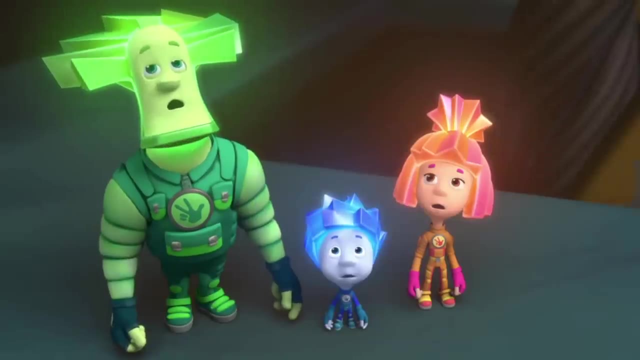 If the elevator suddenly stops for some unknown reason, don't try to break out of it yourself. Press the button that calls the emergency operator and wait for help from the elevator repairman Or the Fixies I've reached the motor. Turn it on. 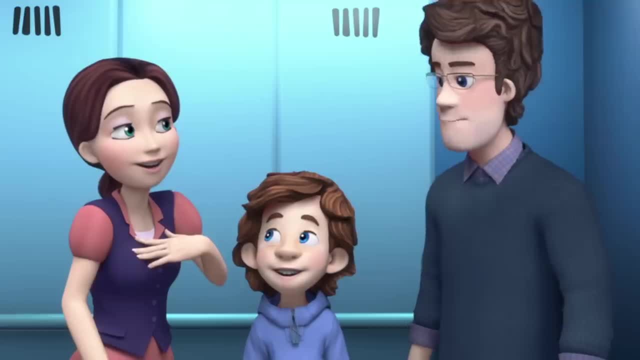 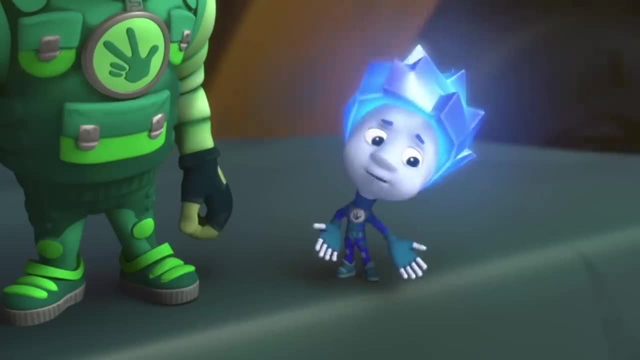 Oh, they fixed it. That was quick. Now we'll make it on time. There was no need to worry. Stop, It's way too high. Tom Thomas went to the circus without us. There's no need to get that upset, Nolik. 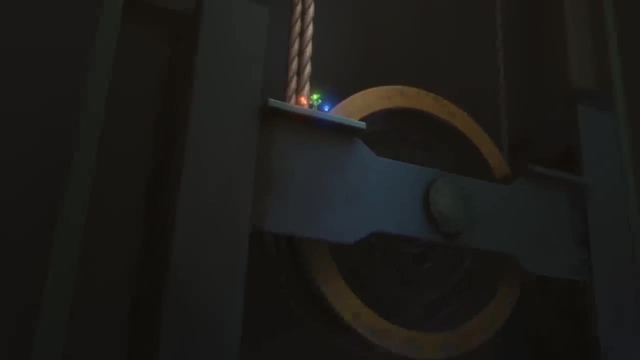 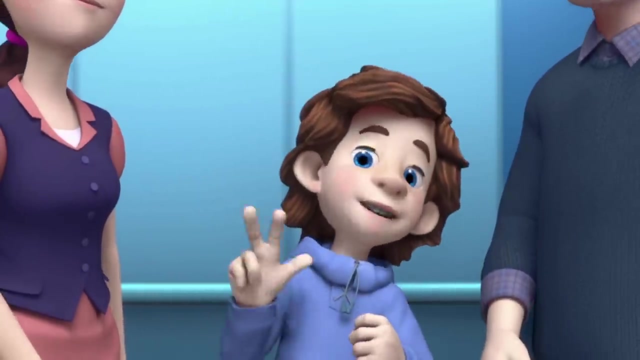 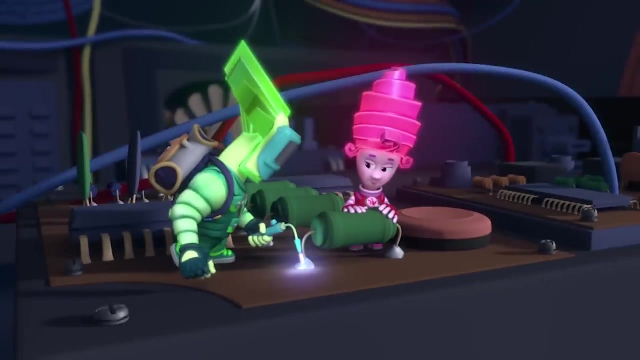 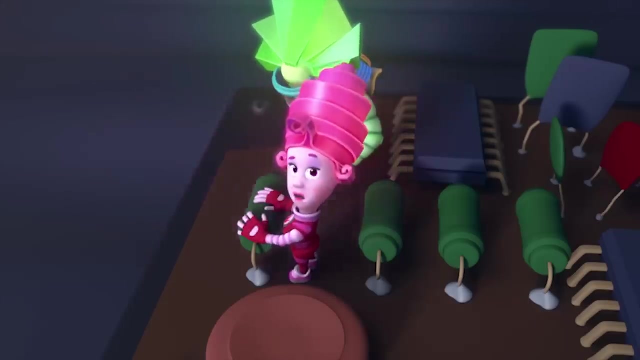 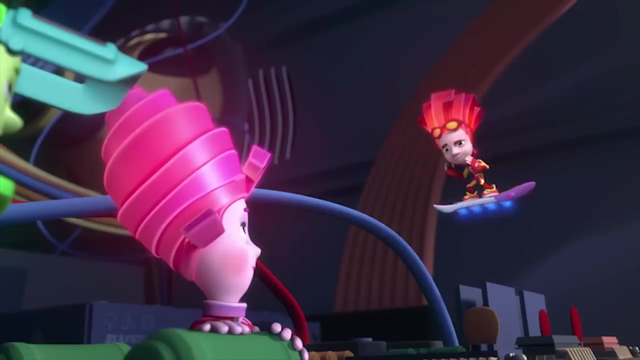 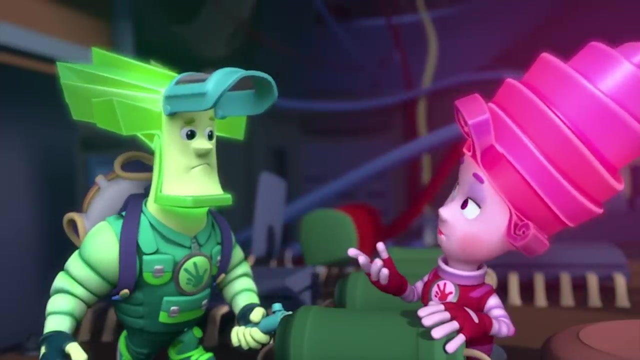 Our circus is as good as theirs, Right, Papus? Of course it is. Thank you. Thank you, uh. to who? What do you mean? who? The elevator repairman? He's an elevator repairman. You've got to get to the school right away. 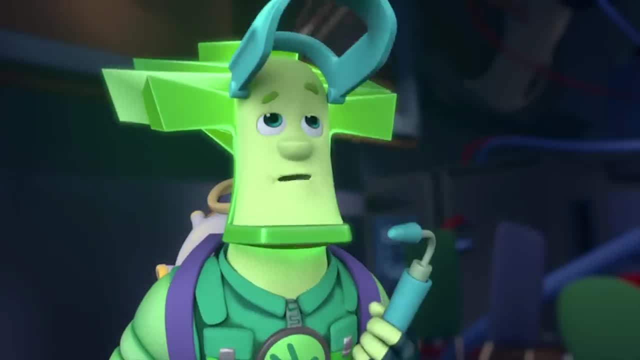 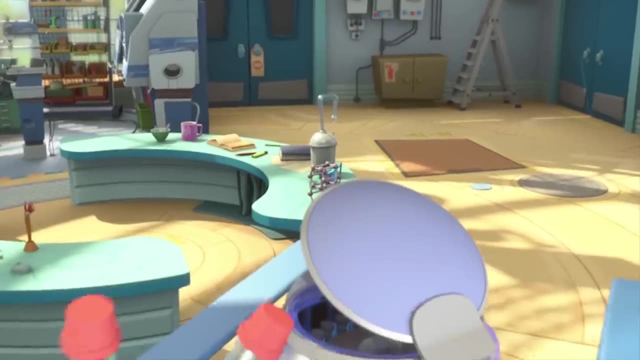 What did he say? That we've gotta get to the school. How come Did you hear why I didn't, did you? I wonder if Simka didn't go to school today. This is something serious, La-la-la-la-la-la. 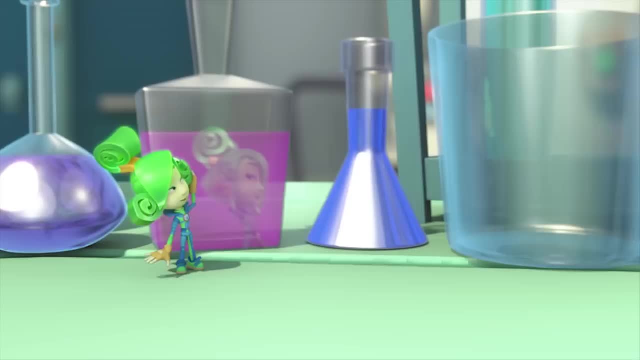 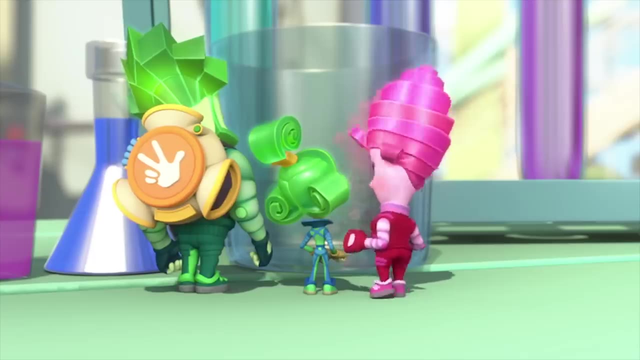 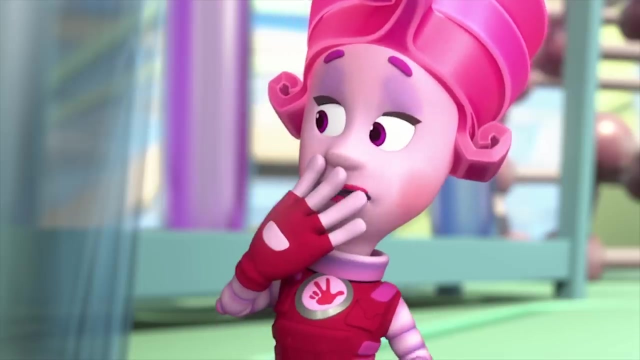 And that's five, six… I like this hairstyle. Seven, eight… Hi there, Hello Verda. Where's Grandpus? I'm not positive, But go and look in the chemistry area over there. Over in chemistry, Tell us, was Nolik doing anything wrong today. 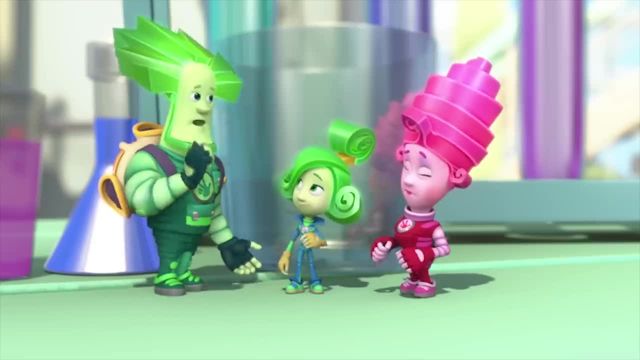 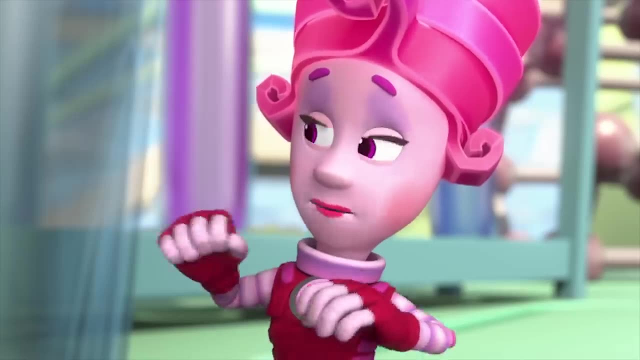 Nolik. He's always fooling around, Right, So we're not here for anything Nolik did. Maybe something awful happened to him, Like what? Well, how about anything? This isn't just a school for Fixies. 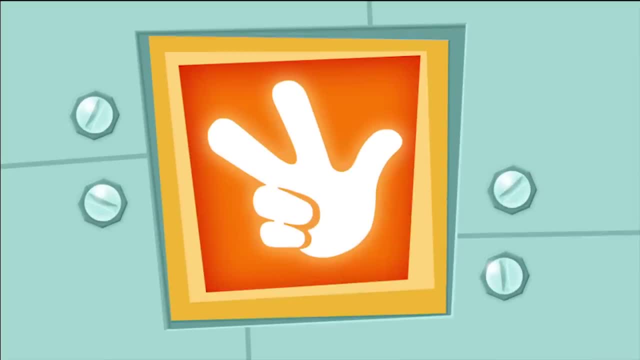 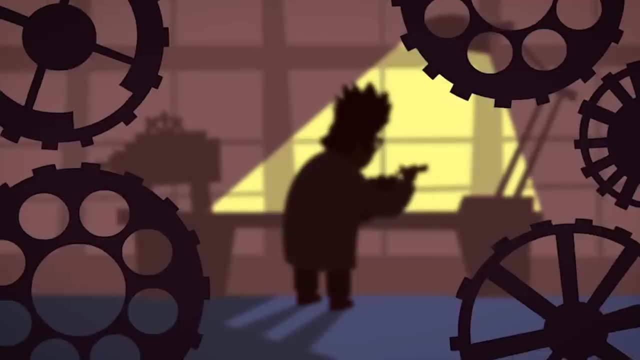 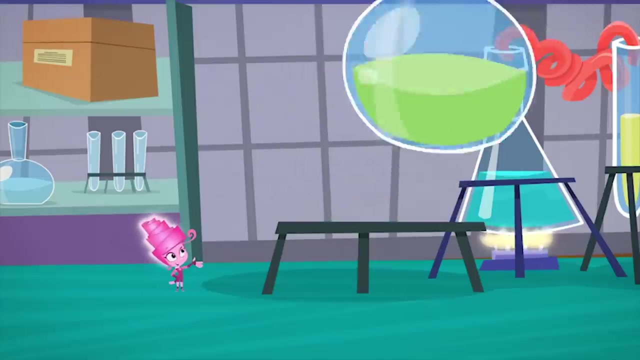 This is a laboratory. The laboratory where Professor Eugenius works is always humming. In the mechanical zone, Professor Eugenius tests all sorts of different devices to see how well they are made. In the chemistry zone, he conducts experiments on the quality and safety of food. 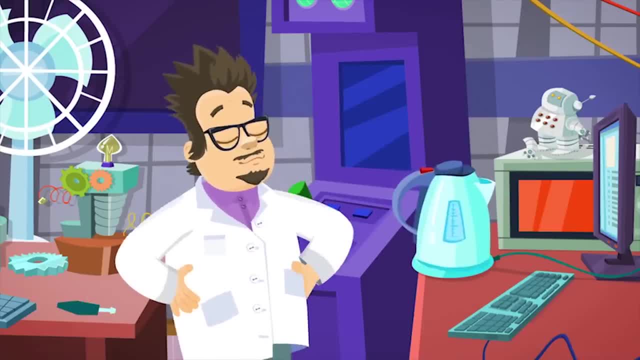 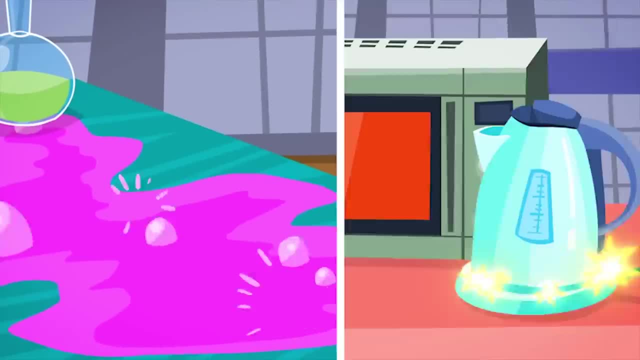 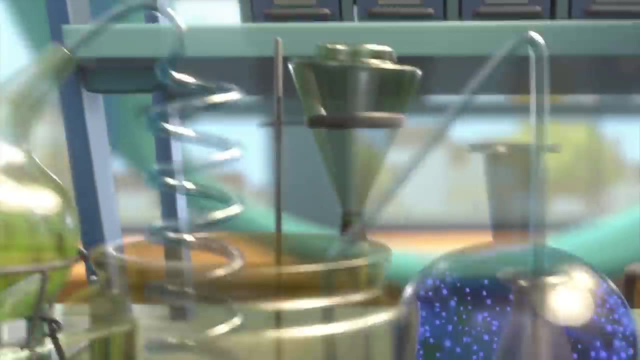 In the electrical zone. he repairs electrical devices and checks their safety. Unfortunately, the professor can be absent-minded and that can cause things in his laboratory to bubble, spark or even explode. Masiya, there's nothing to worry about yet. 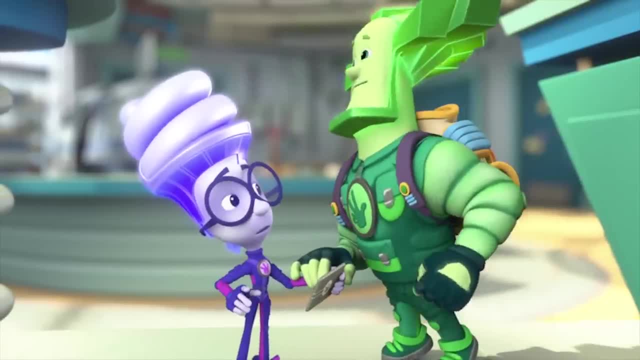 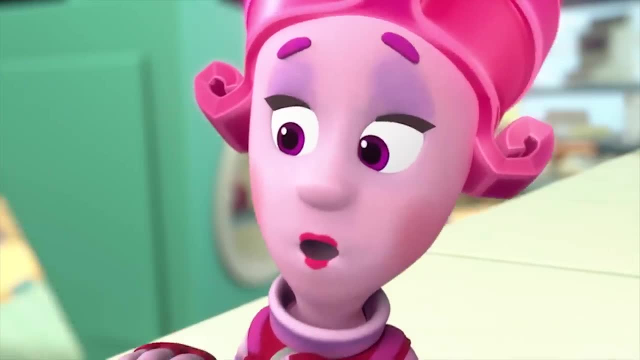 But how can I not worry, Digit? have you seen Nolik anywhere? Do you know if anything's happened to him? This is a laboratory here. Who knows what could happen to anyone. Like what, What are you saying? Like that? I told you, things happen here. 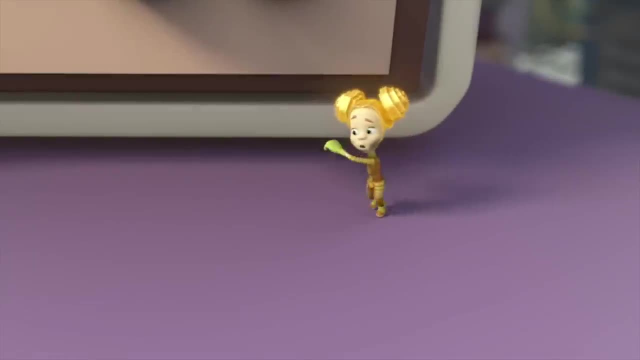 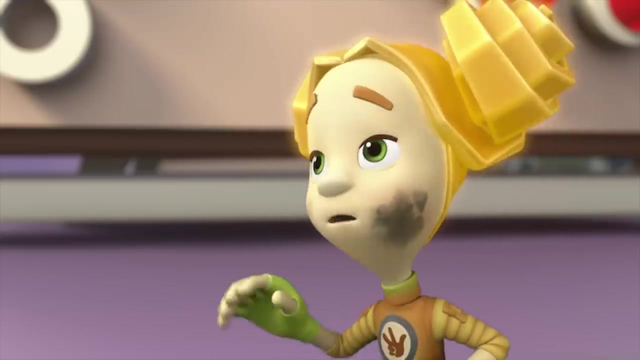 And where. Let's go Quickly, Masiya. no need to panic, Tula, It's so good you're here. We really need your help. What is going on? Ah, Oh bear, Oh Wee. 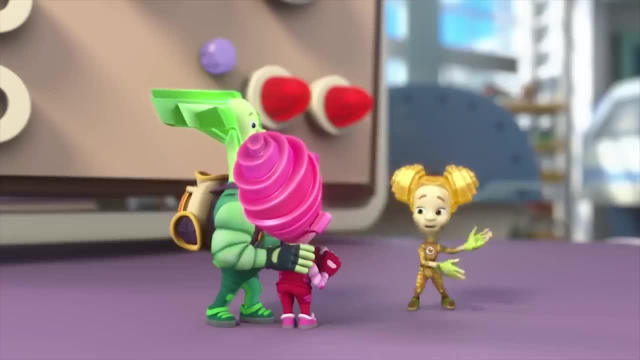 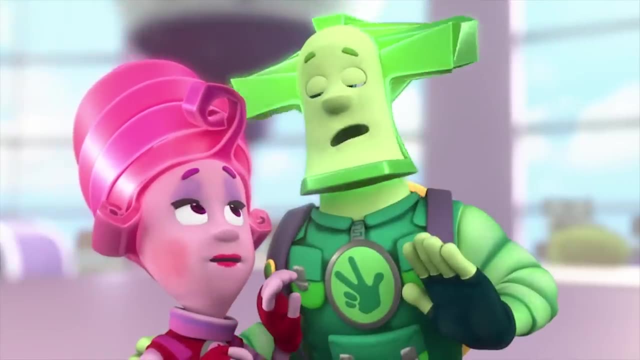 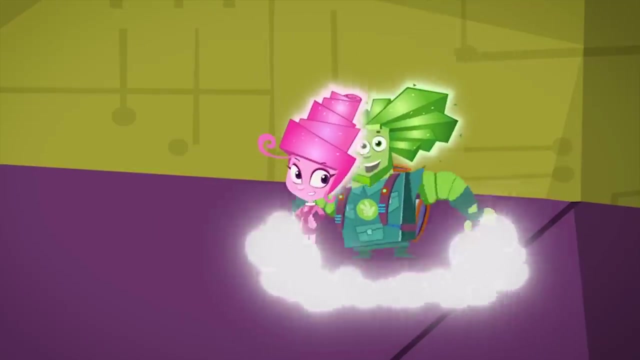 Grampus, What Where? In the mechanical zone there, And Simka and Nolik There. They're all there. Oh my children, Don't lose your head. Masiya is my wife and the mother of our children, Simka and Nolik. 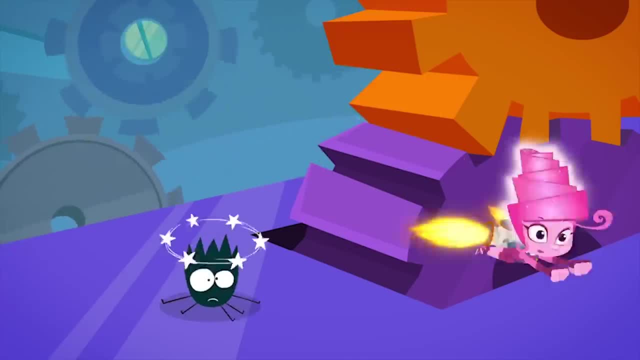 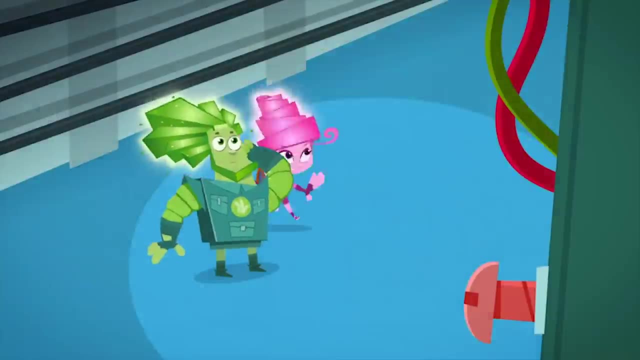 Masiya is a real beauty, a kind and gentle soul and a wonderful homemaker. She is also a very responsible and extremely skilled fixie. She is our family's expert in kitchen appliances and gadgets. Masiya works from morning till night. 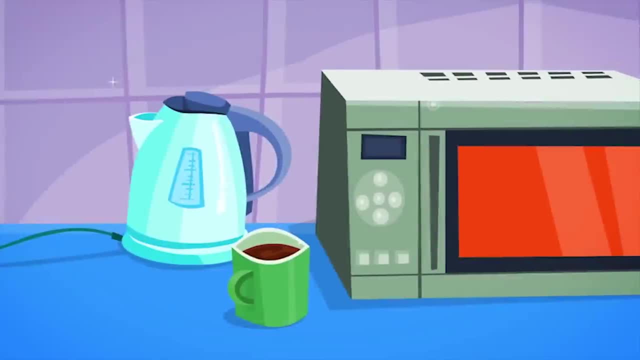 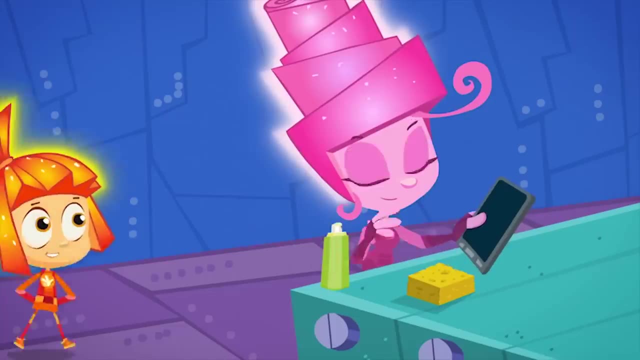 fixing and cleaning anything that is in need of her expert care, because she just loves when everything is clean and tidy. But most important for Masiya are her children. She takes loving care of Simka and Nolik and tries to protect them from harm. 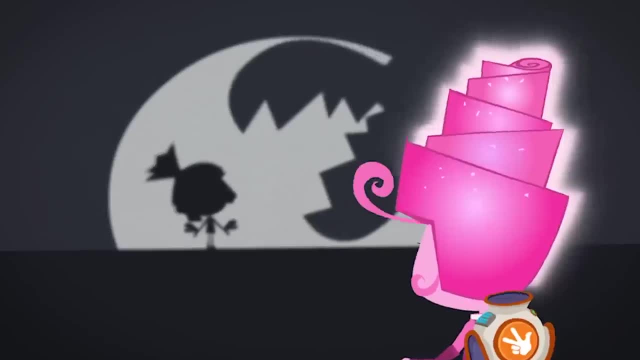 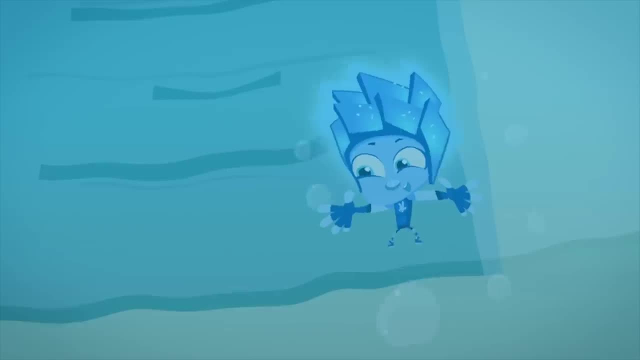 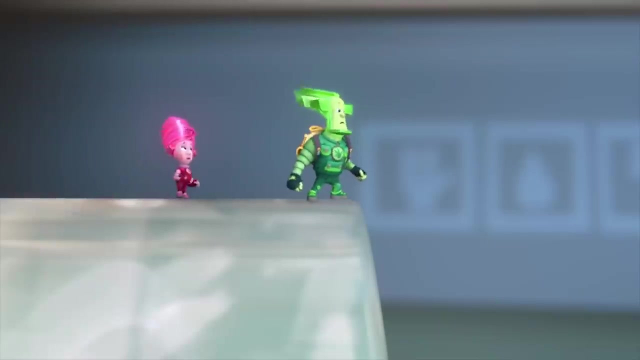 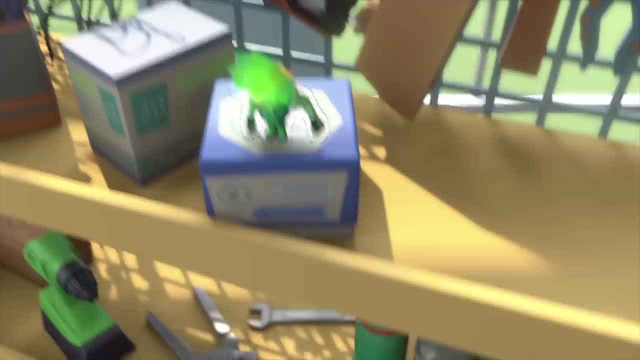 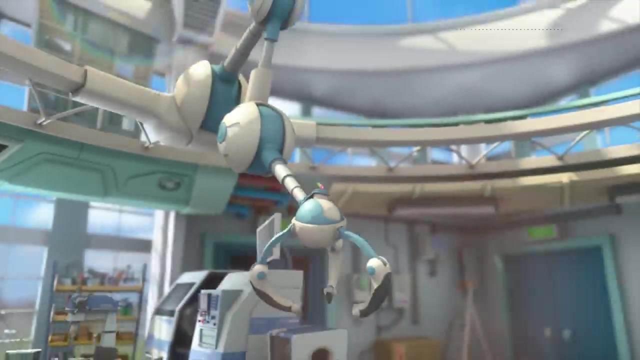 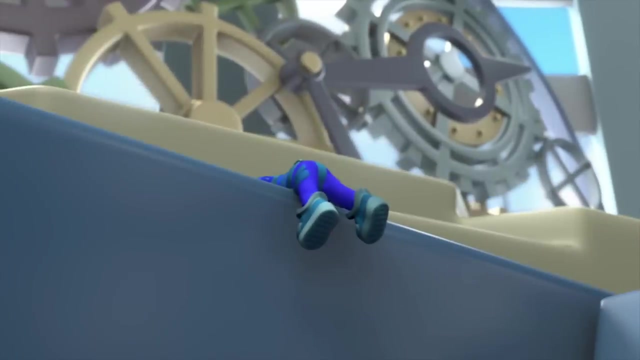 Masiya worries about them so much that sometimes her imagination gets carried away with what might have happened to them, Although our little Nolik can get himself into situations that even Masiya could never have dreamed of. Masiya Nolik. 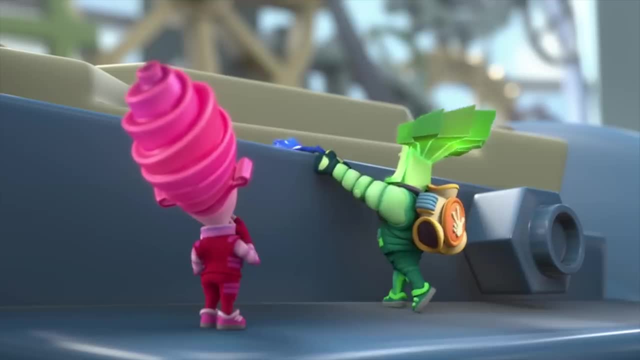 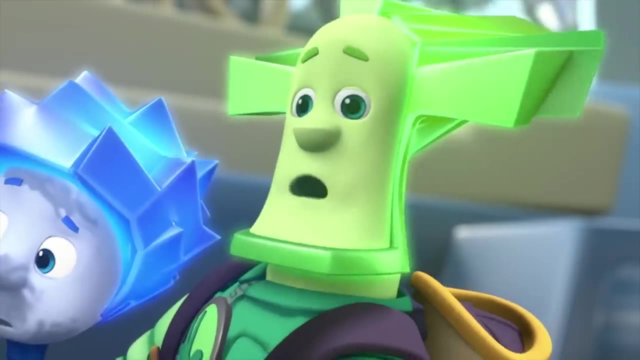 Hang on tight, We'll save you. Hey, You're alive. What's going on? I don't need to be saved from anything, So it's Simka we need to save, Not you. I don't need saving either. I'm fine. 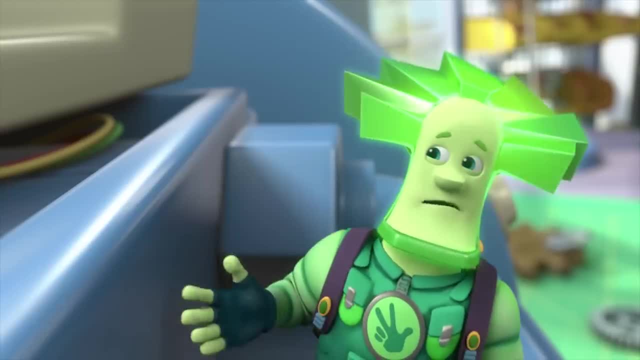 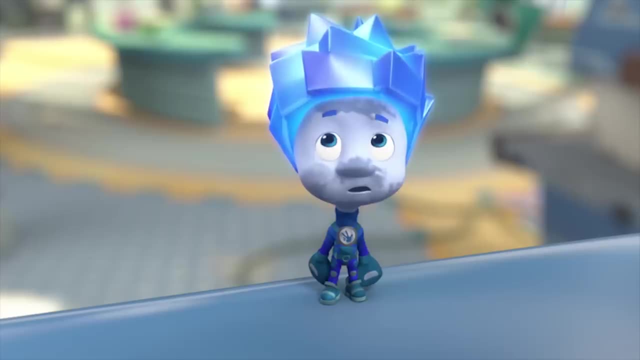 And what are you so worried about? Everyone is alive. Then why did you make us come here? I need you to help with a little accident we had, Nolik. Was this your fault? Oh no, It's not Nolik's fault. 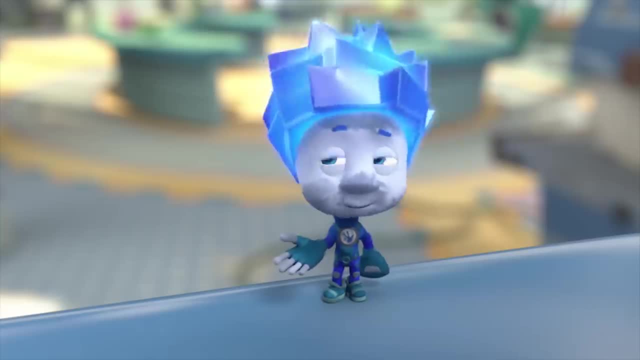 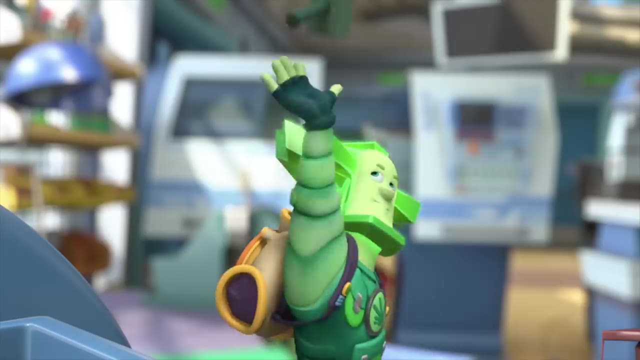 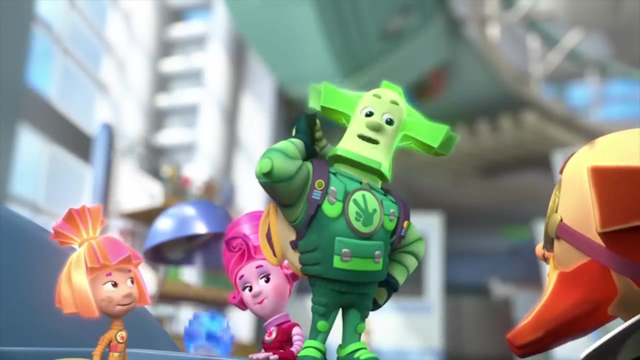 Quite the opposite. He was trying to help me fix it, Papus, we needed a helpers with one of the pieces that we couldn't get back in place. This one, Tideesh. Oh, a perfect repair. Huh, that was really the only reason we had to rush here. 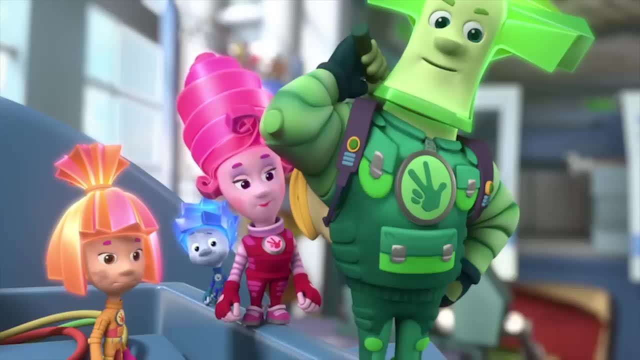 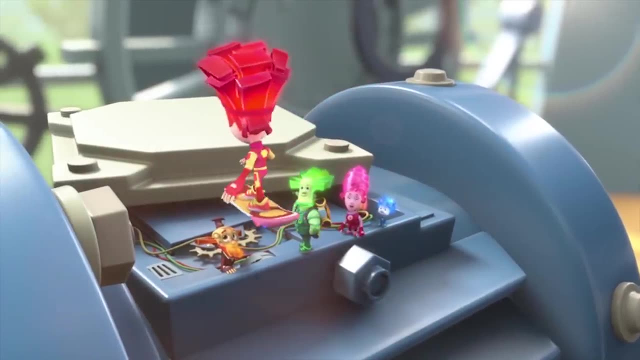 Why not? There was just no way we could let this wait, so I sent for you. But fire said… Why fire? Why is it always fire? How come you had to scare us so badly? I'm not the one who scared you. 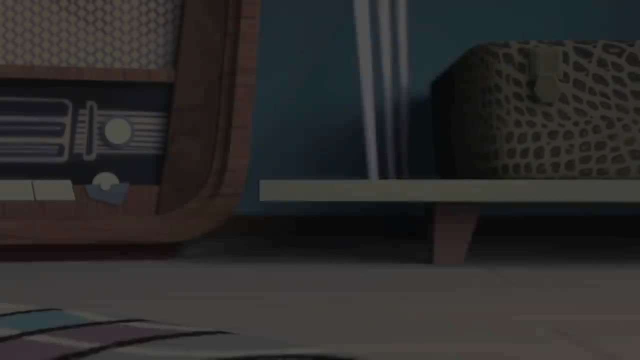 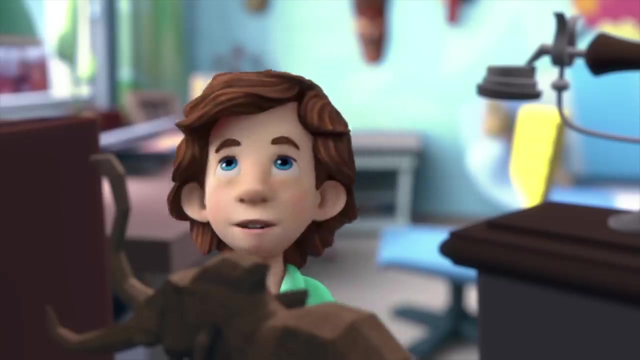 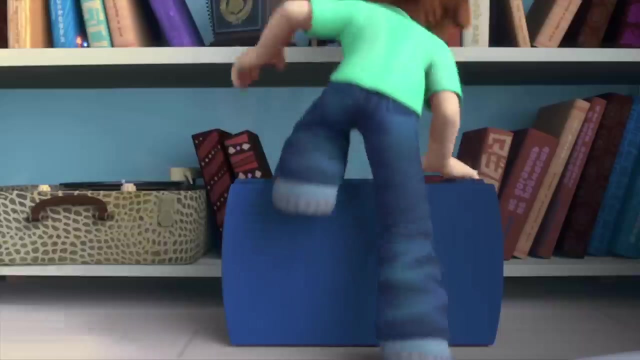 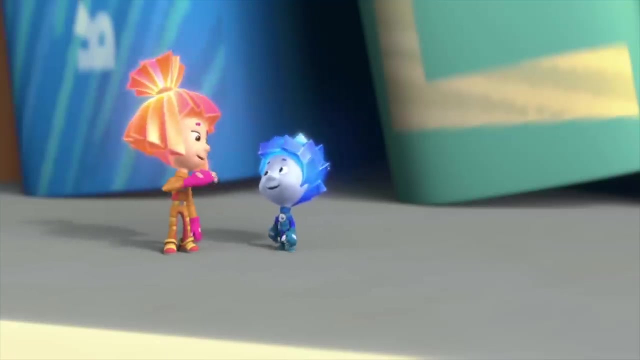 You did that all by yourselves. Hang on, There are these really cool things that I want to show you. Look how many things you got. You got all at once. Heh, Your dad's going to be so angry when he sees what you did with all of his tools. 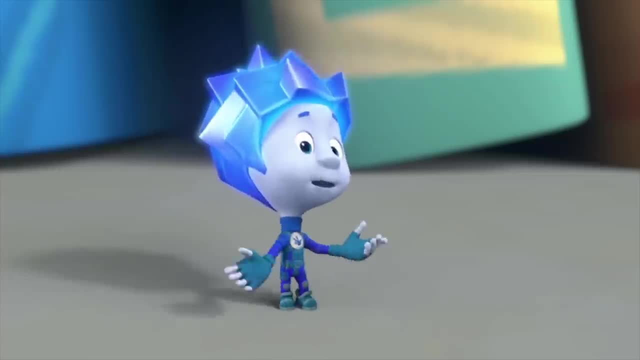 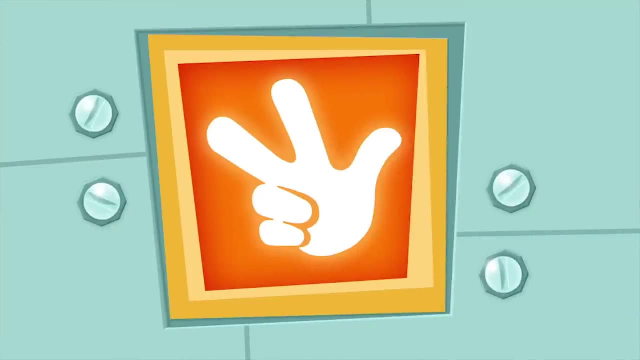 I'm going to put them all right back where they were And where were they. Open the box and you'll see It's neat. There's a special place in there for each one of the tools. Try hammering in a nail or drilling a hole with your bare hand. 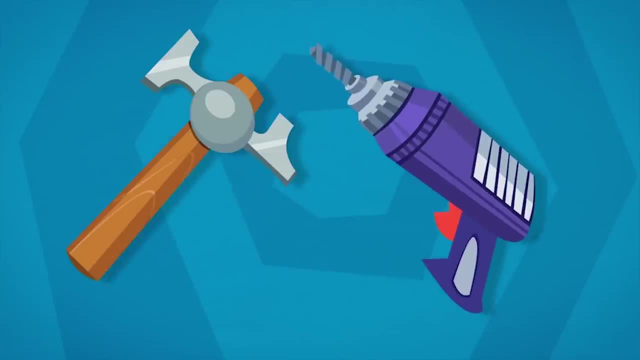 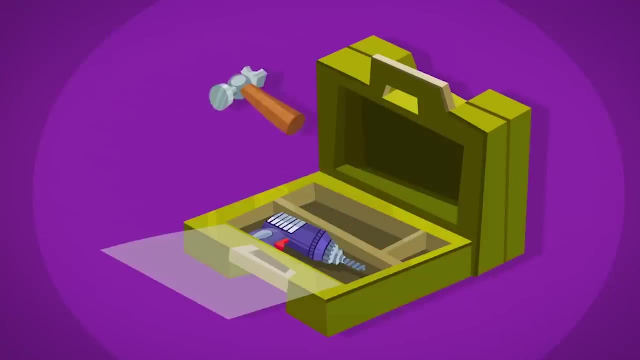 Uh-huh, there's no way. But with the help of the proper tools it's a piece of cake. But of course that's only if you know how to use them. Tools need proper care. If the head of a hammer is loose or a drill is dull, then you shouldn't work with them. 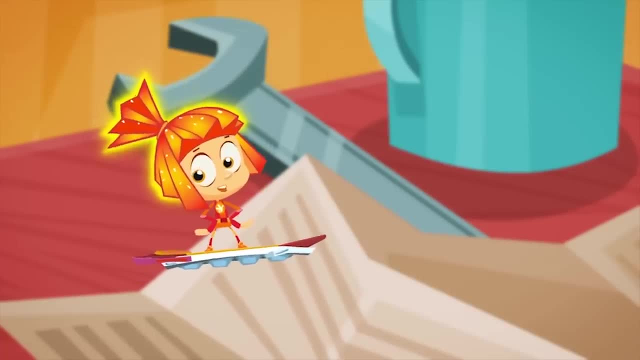 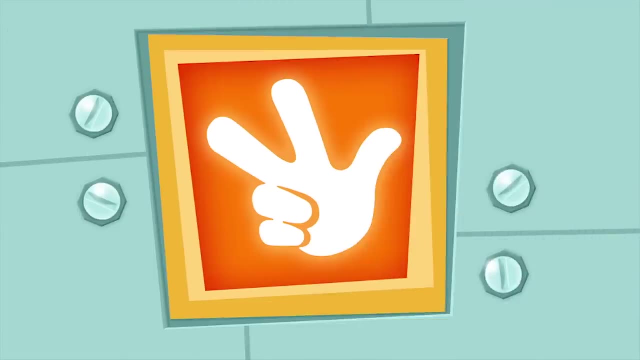 It's dangerous. And when you're done working, put the tools back in their places, Or you'll be tearing your house apart trying to find them the next time you need them. The pincers go here and the wrench goes over there. 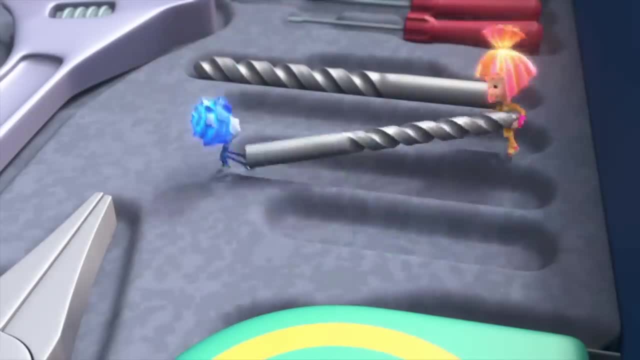 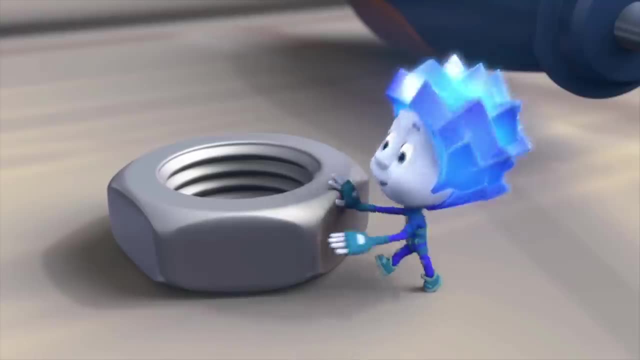 This drill bit's too long for this spot. Let's see if it fits in this one. Huh, Any idea what this tool is for? For splitting wood or carving stone? that chisels what you want to own. Oh wow, Simka, You're a real poet. 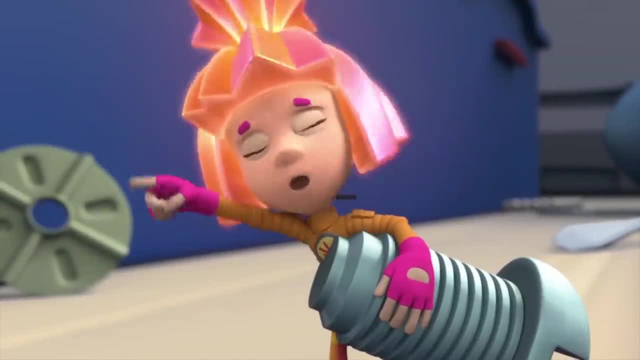 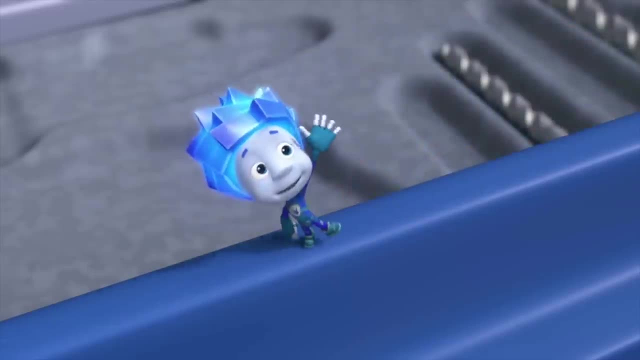 Now try to answer this little poem. When you have a thing to measure, this round tool is quite a treasure. This tool- right, I know what it's called: It's a measuring tape. Let me measure you, Nolik. 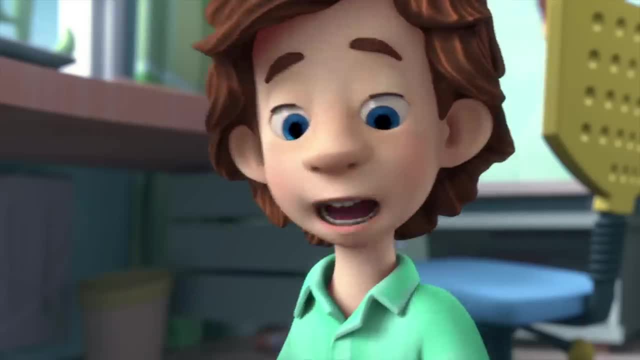 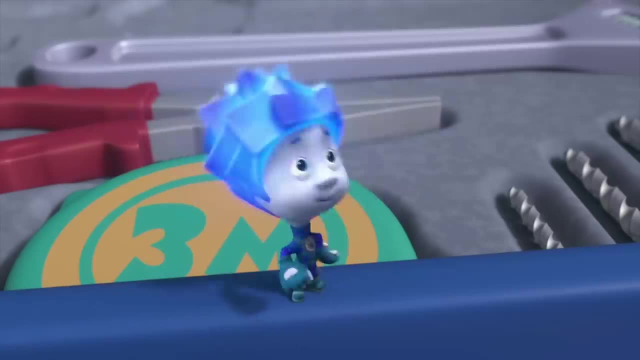 Wow, you've grown. You've almost reached one centimeter Class. I also have a rhyming riddle for you. When Bang's in Amsterdam, he's going to crawl into the wall to make sure pictures never fall A hammer. 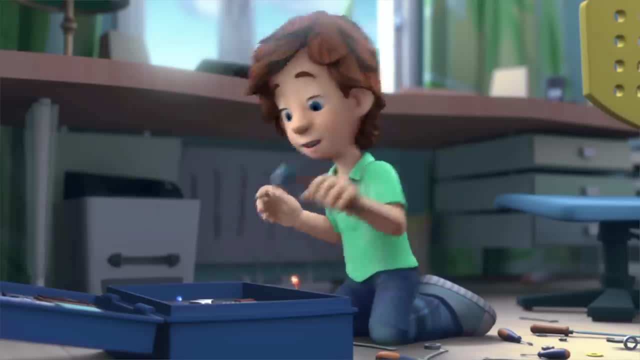 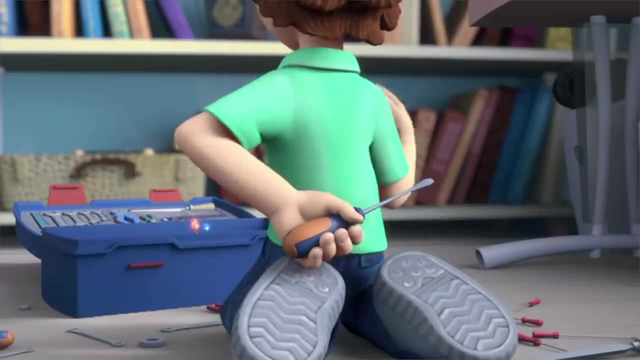 I was first and the hammer goes right here, And now I have one for you to guess. If you need to screw in screws, here's the tool that you should use: A screwdriver. I was first. again, You got it right. 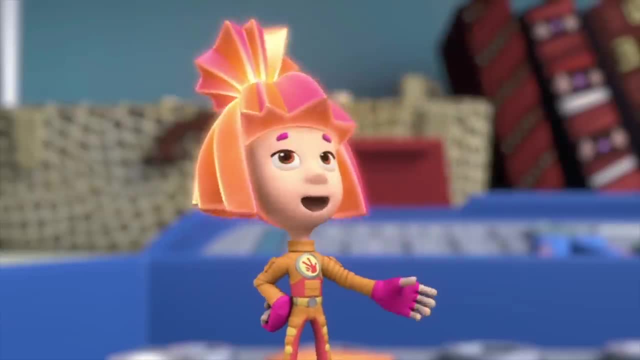 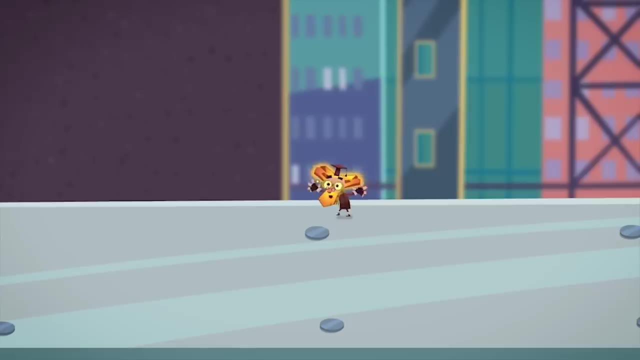 Alright, Tom Thomas, we'd better hurry. We still have a lot of tools here to get sorted out. Humans, just like Fixies, use hundreds of tools to measure. They use hundreds of different tools to do their work. Picking the right one depends on the task at hand. 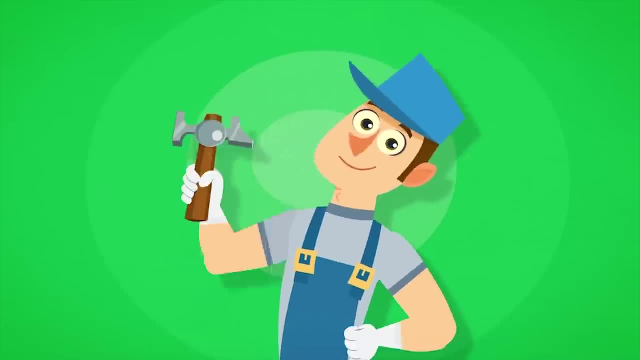 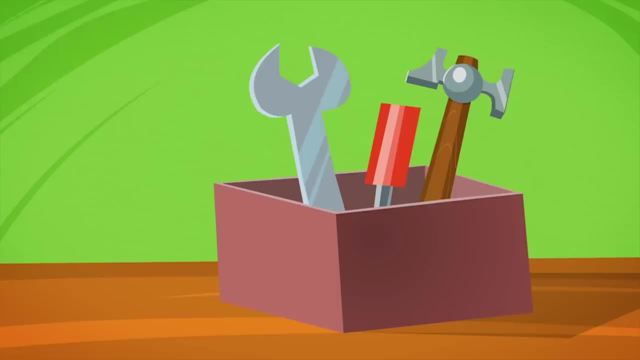 For instance, if you need to hammer in a nail, use a hammer, But you don't use a hammer for a screw. For that there is a special tool called a screwdriver. A wrench is the tool for tightening nuts and bolts. 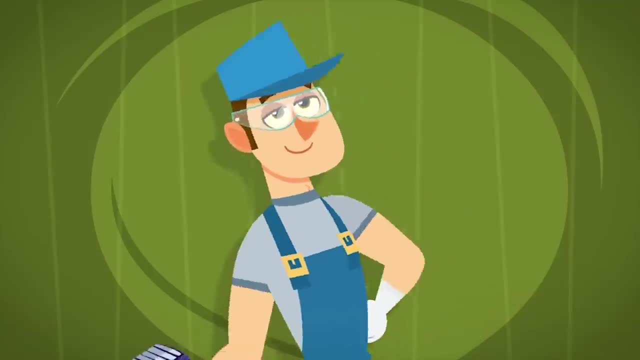 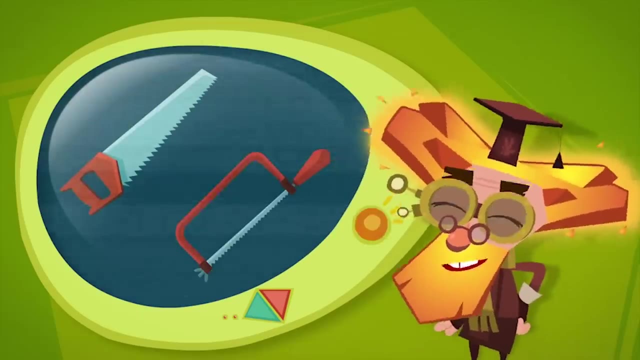 A vise is used to hold a part in place and a drill to drill a hole. If you need to cut a piece of wood, you should choose a saw. You could use a handsaw, for example, or a hacksaw. 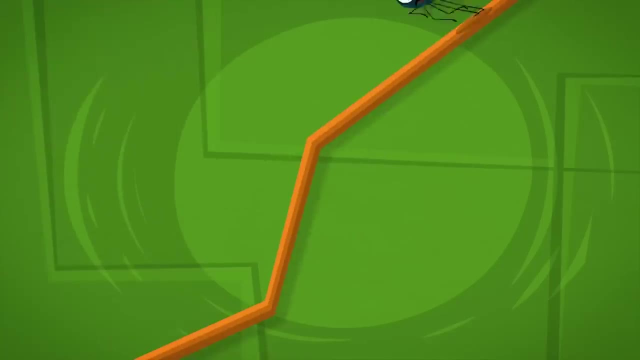 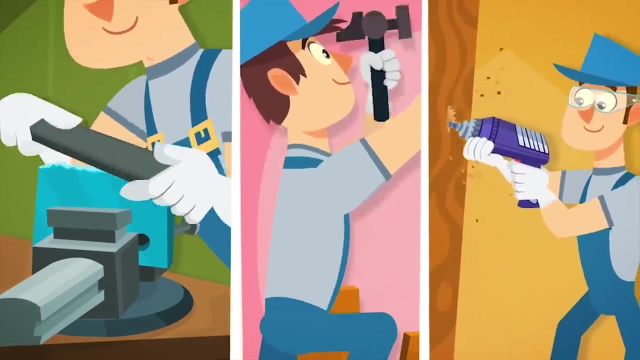 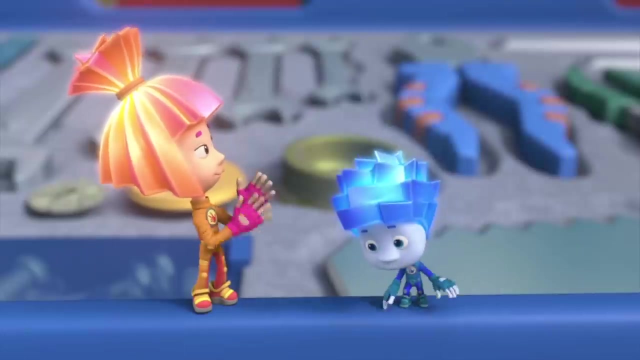 Different kinds of pliers can be used for snipping, gripping or bending. If you need to smooth something down, you use a file. If you learn how to work with tools properly, you can build just about anything. Looks like we did it. 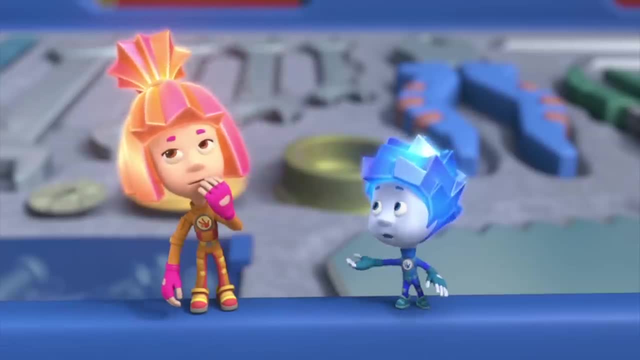 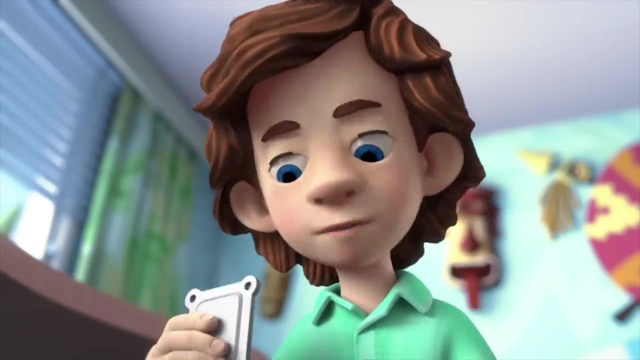 Just in time. Oh, and how about this? Do you know what kind of tool that is? I don't know. There's no place for it. There's no place for it in here. Just throw it out, Come on. And what if my parents use it? 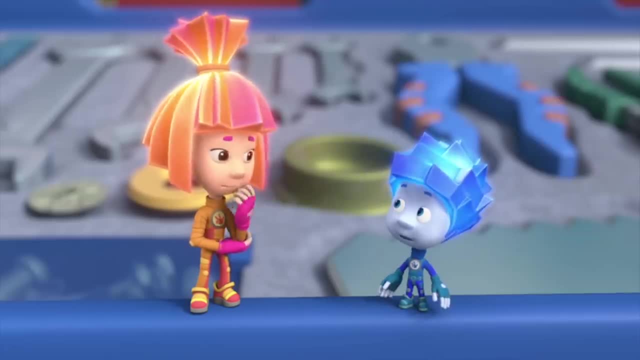 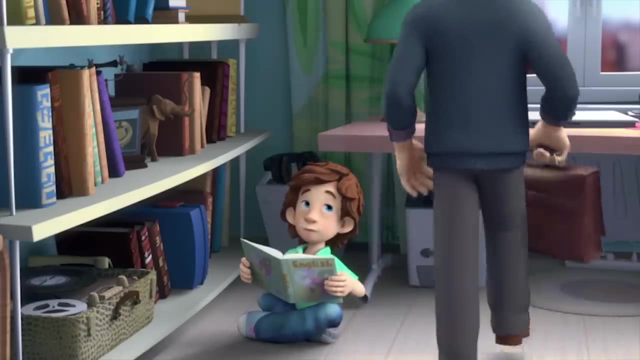 Looks like we did something wrong here. My dad came home. Tom Thomas, I'm in here, Hi there Reading Way to go, son. Huh, Oh, I don't get it. Where is it What? I put a piece of metal under the table leg so it wouldn't shake. 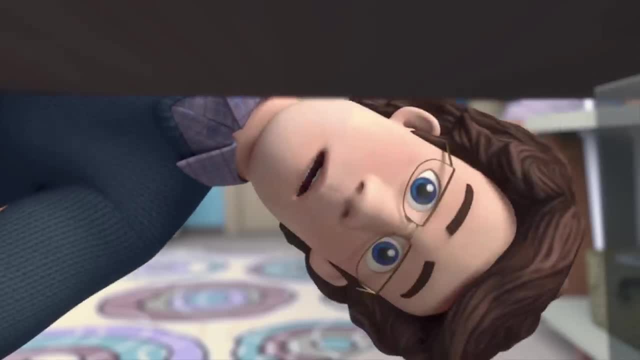 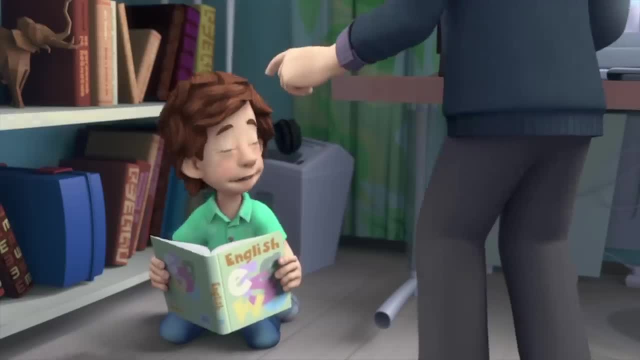 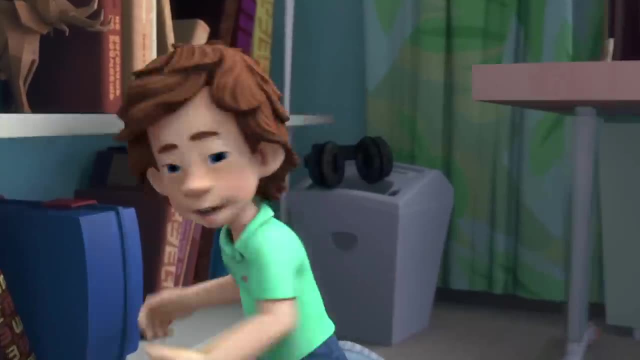 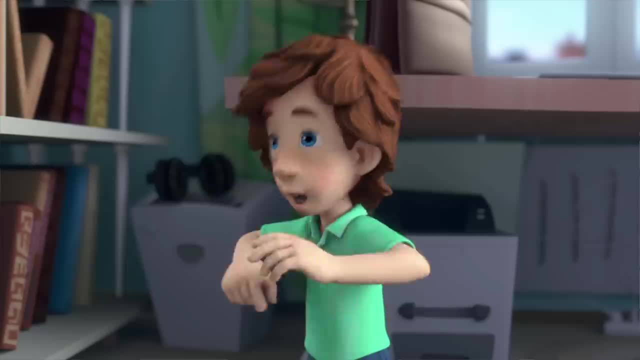 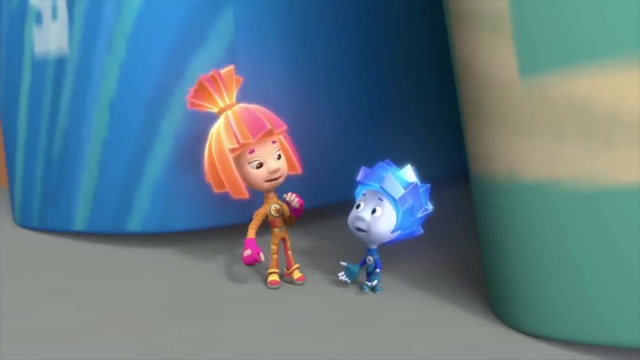 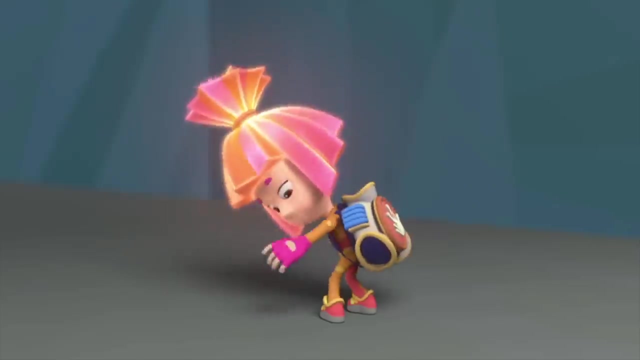 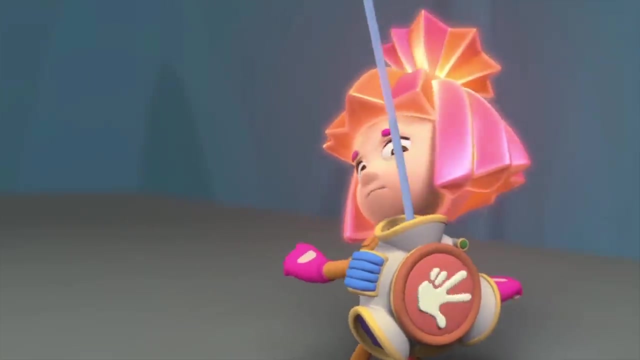 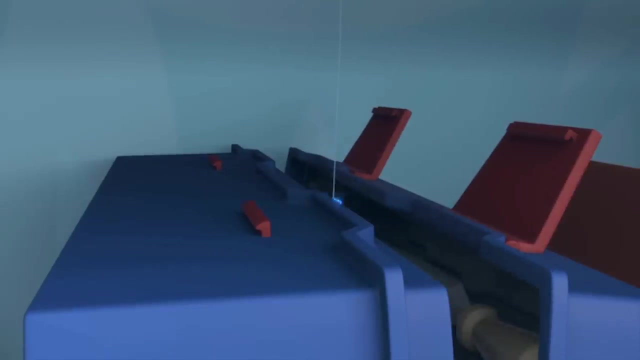 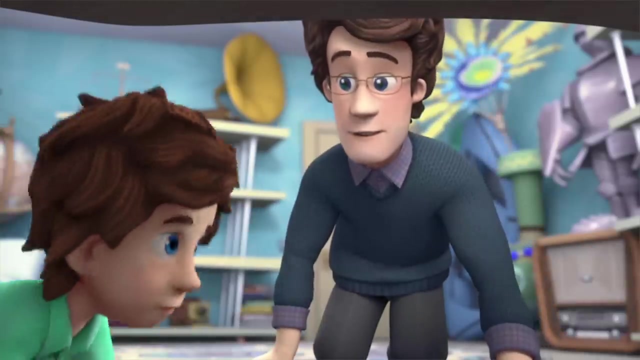 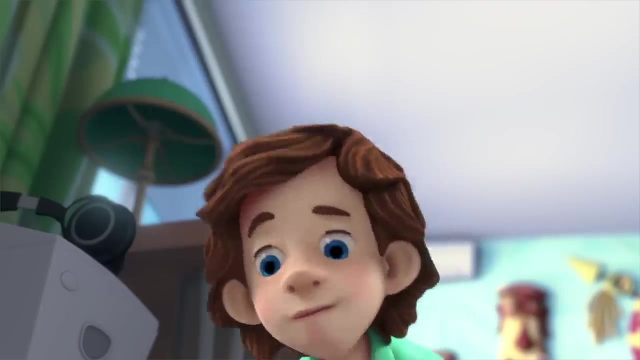 Uh, alright, What do you think he wants? He wants us to get that metal thing out of his dad's box. Come on, Let's go. You've got it. That's not working. That's not working. I found it, Dad. 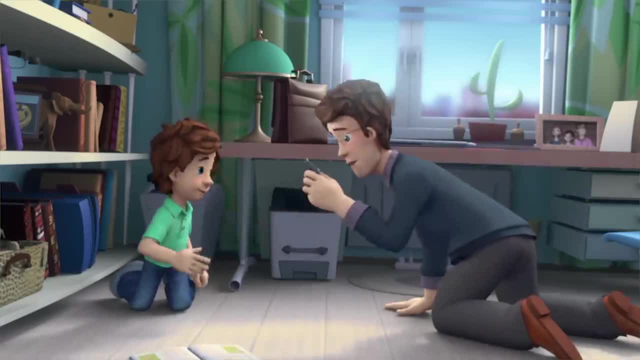 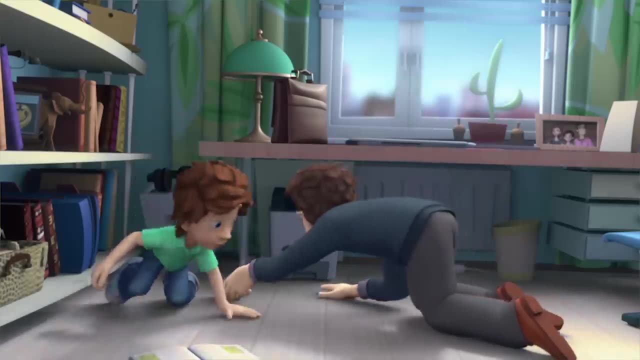 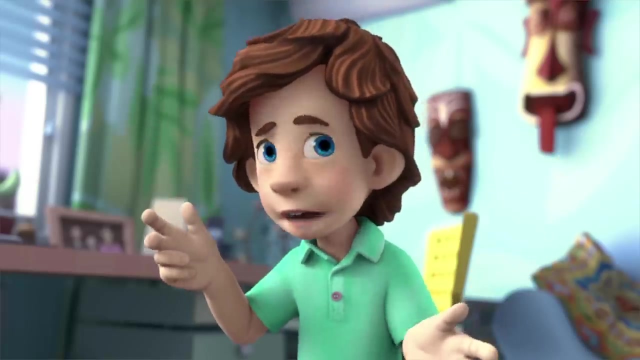 It was under the table, just like I told you. Huh, You were right. It's strange. How could I have missed it? Maybe you're just tired from working too much, Maybe Tideesh- What? It's a new word, Tideesh. 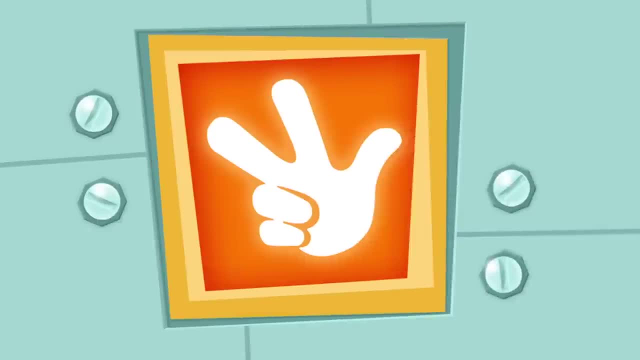 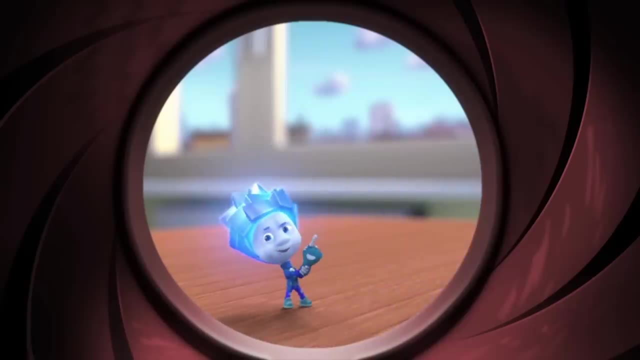 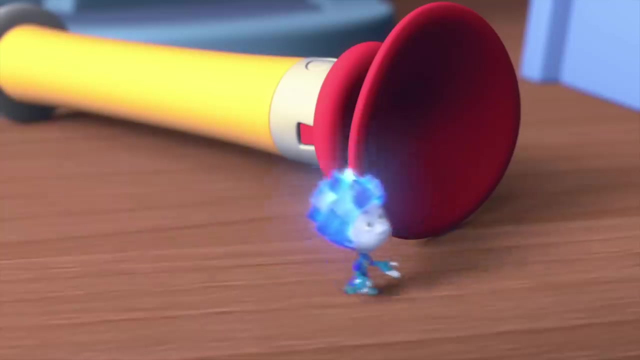 Tideesh, I do like the sound of it. The draftsman, Huh, What? Hi there, Tom Thomas. What are you drawing? I'm not drawing. This is called drafting. What's the difference, Tell me? is that a circle? 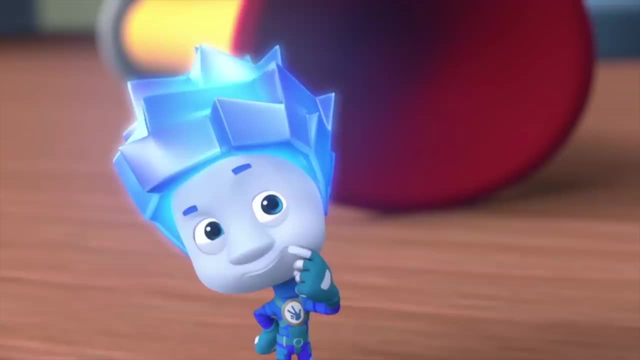 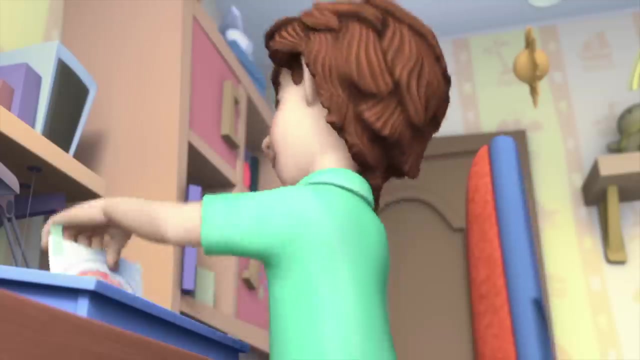 Sure is, And that It's a circle too, Only it's a rounder one. Of course, That's because I drafted it With a compass And now I've got a real target. So now I'll load my dart gun…. 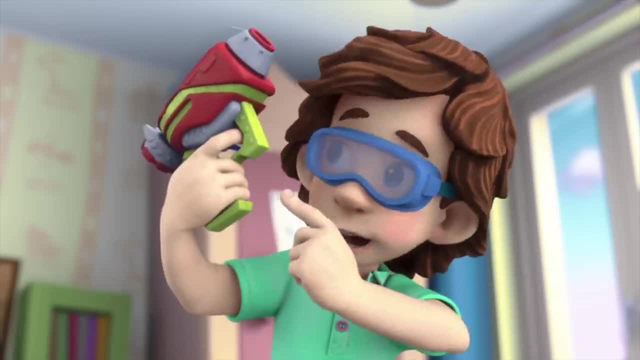 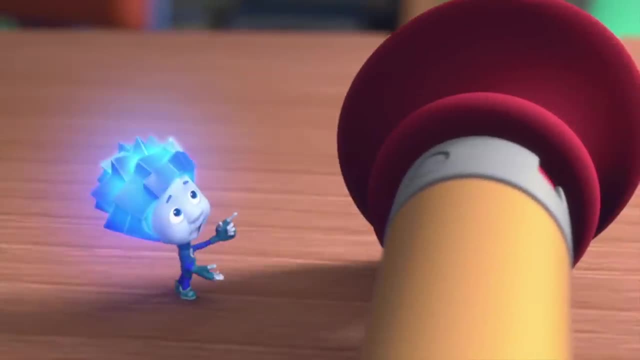 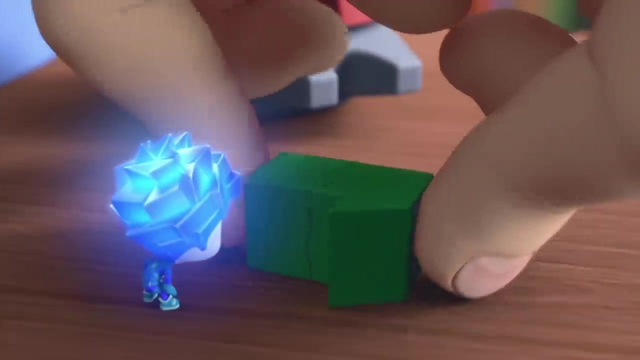 Whoa, Why'd you shoot that thing at me? It was the gun. I didn't even pull the trigger. What Did it break? Hmm, Let's open it up and see There, This little part broke. Let me go find Papus, He can help you. 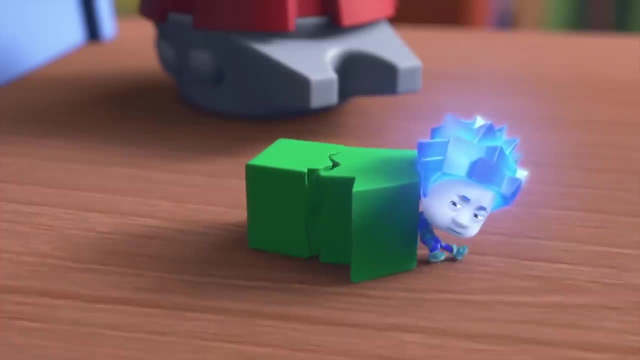 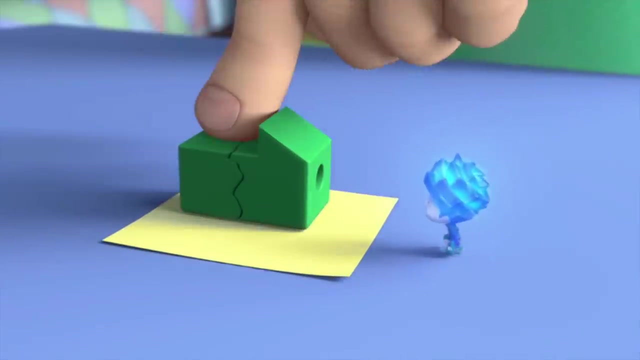 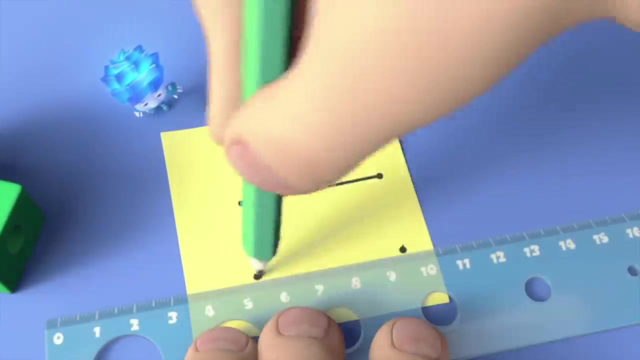 He can make another one, A brand new one. Wait, I can draft a technical drawing. Will Papus understand how to read one of those? Are you kidding? Papus is an expert at everything Done. Wow, Tom Thomas, You're a real technical drawer. 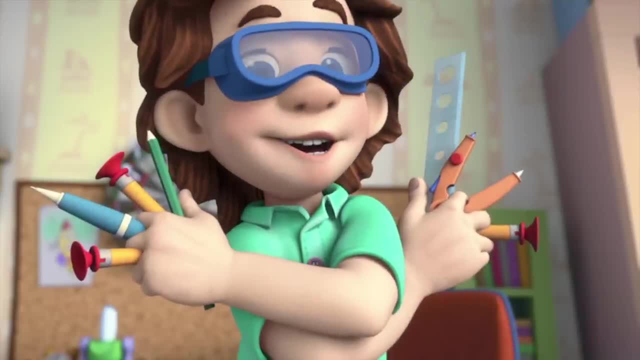 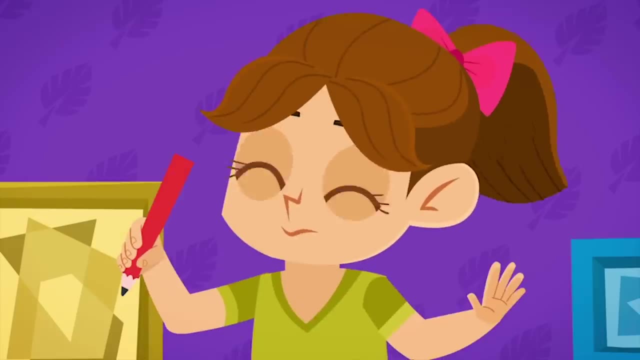 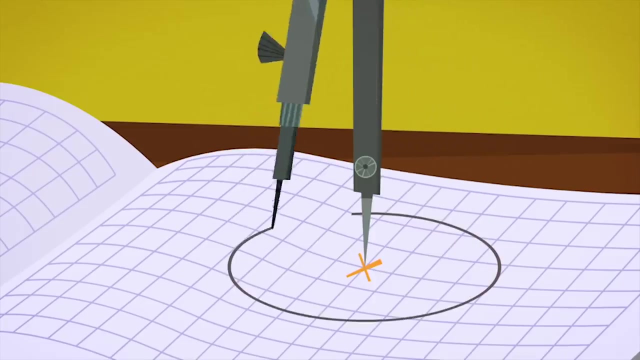 A draftsman Nolik, That's what they call it. Try drawing a perfect circle by hand. Can't do it? huh? Well, with the help of a drafting compass, your circle will turn out great. Just put the needle point in the center and turn the compass, and it's done. 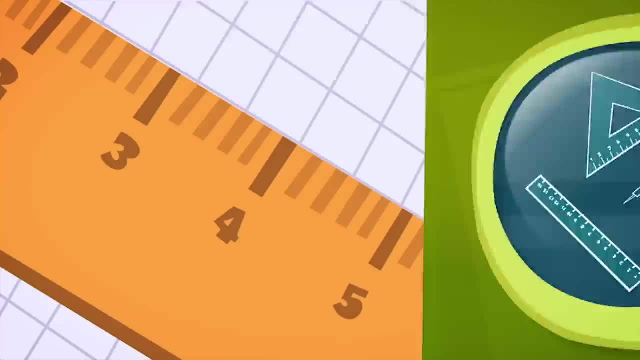 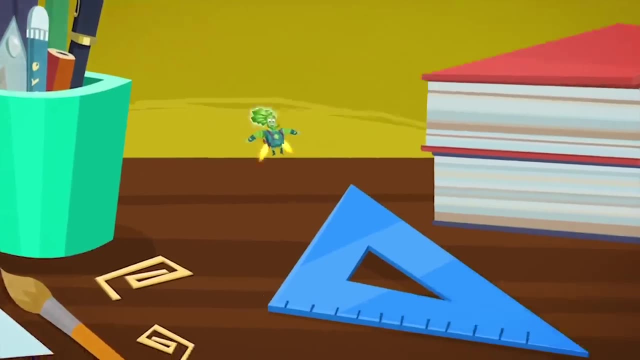 A compass is only one of the many different tools for drafting. For example, if you need to draw a straight line, use a ruler, And if you need to draft a frame for your picture, you can use a triangle: First draft one side and then the other. 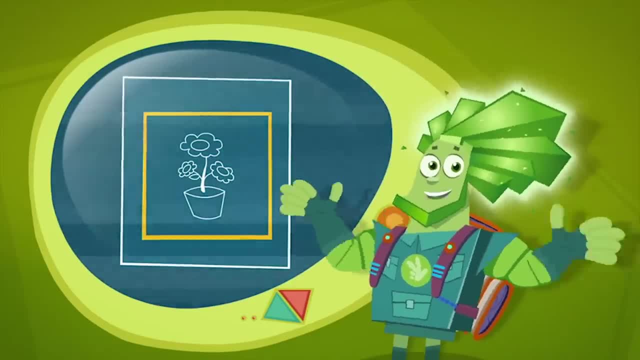 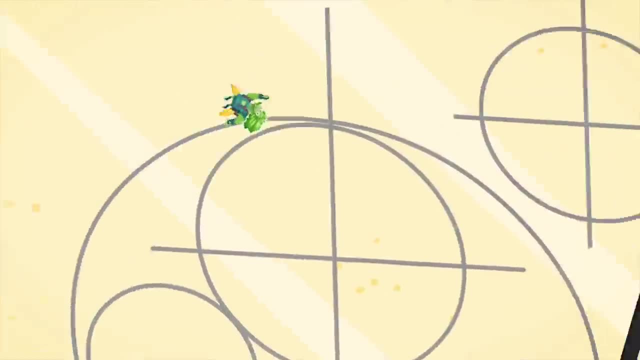 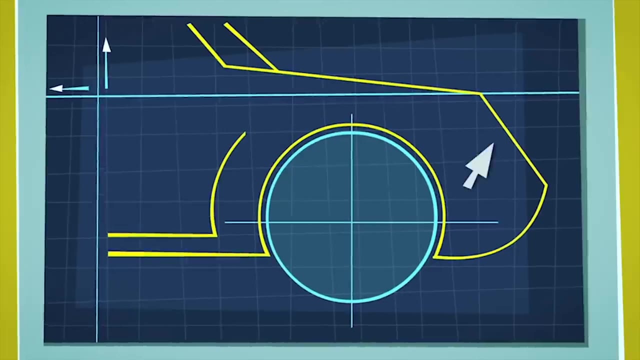 And then, to finish your frame, just turn the triangle upside down and draft the two remaining sides. You'll get a perfectly squared frame. There are also drafting instruments for making curves. They are called irregular curves or French curves, But actually now people use computers more and more for drafting technical drawings. 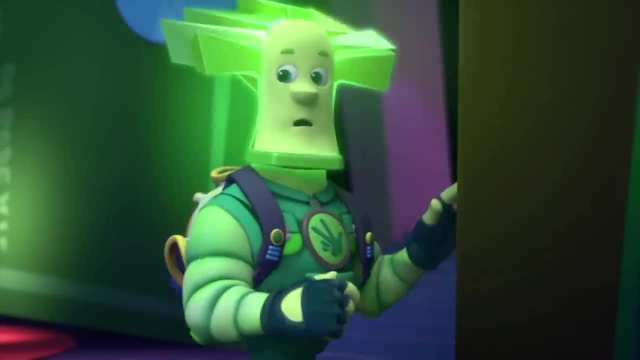 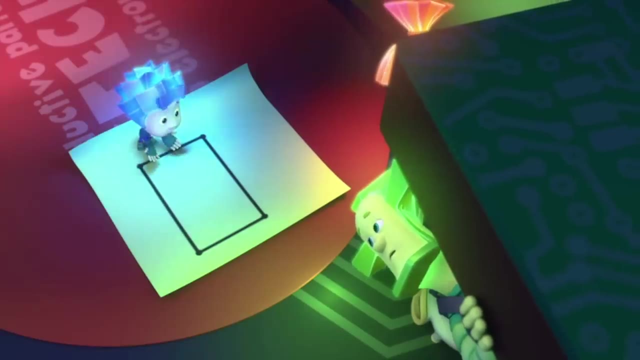 Papus: Huh, What, What happened? We really need your help. One of the parts broke in Tom Thomas' dart gun. Could you make it? What kind of part exactly? Look, here's a technical drawing, So you even know how to draw. 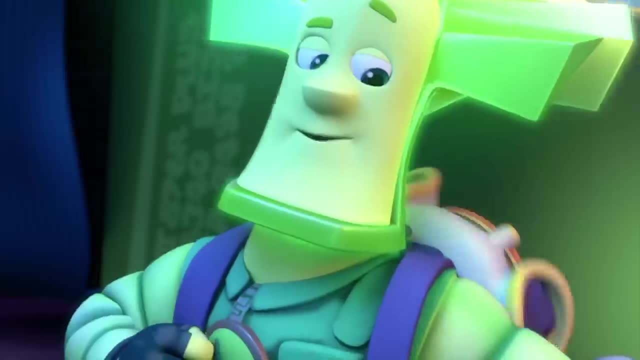 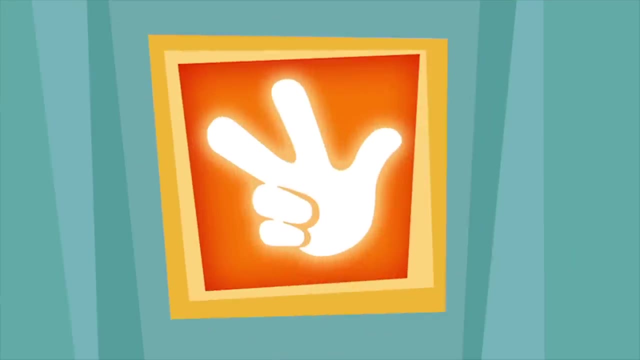 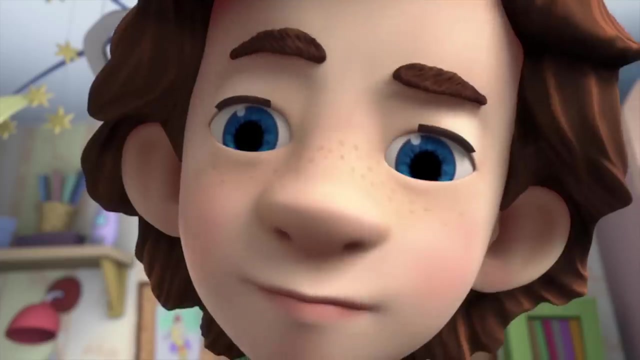 Yes, I even got a technical drawing. Very good, then Let's take a look at it. Here you go, Super, Let's see It's not going to work. You see, it sticks out here on the side. I need to draft another technical drawing. 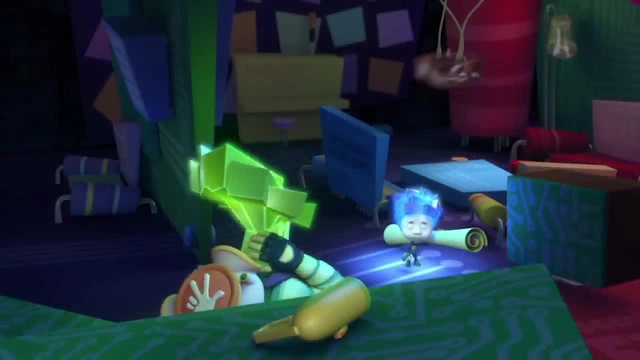 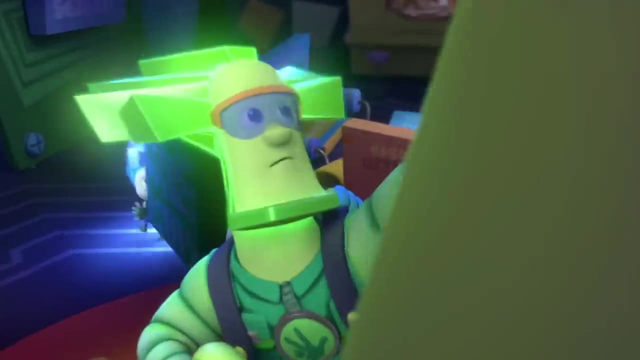 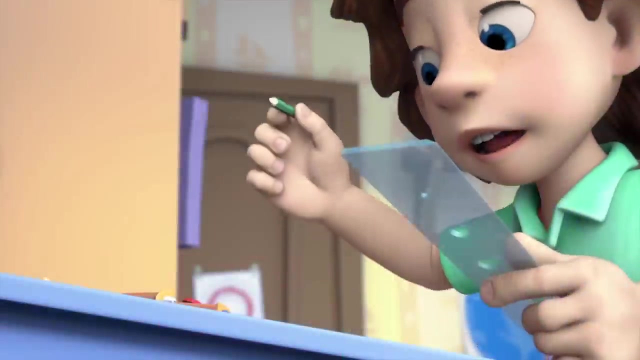 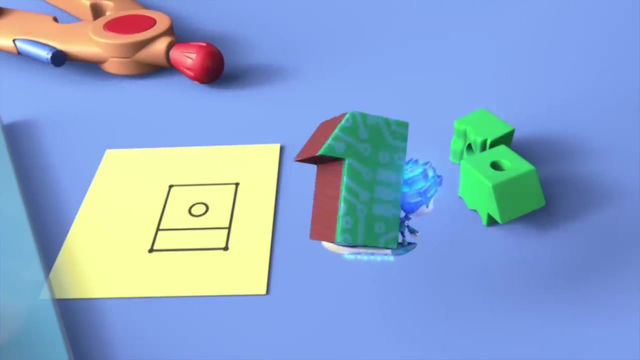 Papus Nolik, you scared me again. Forgive me, But the part has to stick out over on this side And you're sure? that's all. That's all for real, Tom Thomas, It's done. Listen, while you were gone I realized that the part needs to have a hole right here. 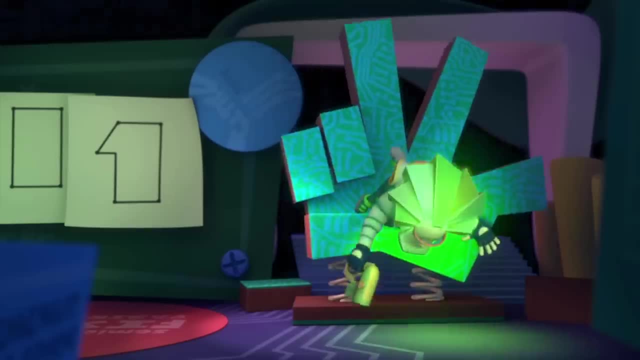 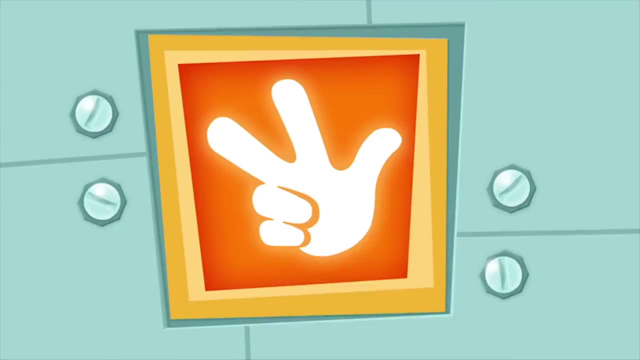 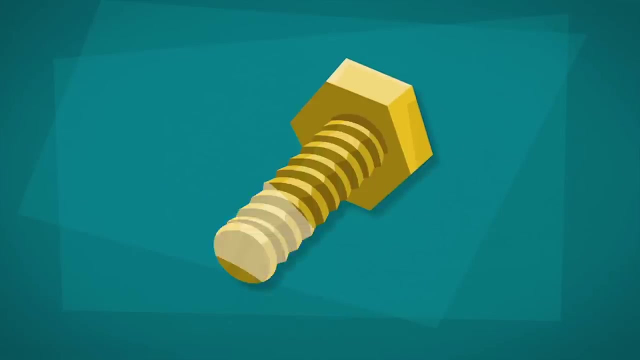 Papus. Again, Sorry about this, but there's a hole in this thing too. A technical drawing is a special kind of drawing. It has to precisely describe the thing that needs to be made. To do that, the drawing must be very accurately drafted and include all of the measurements. 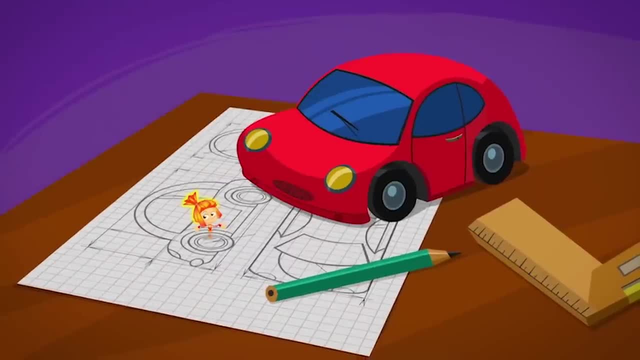 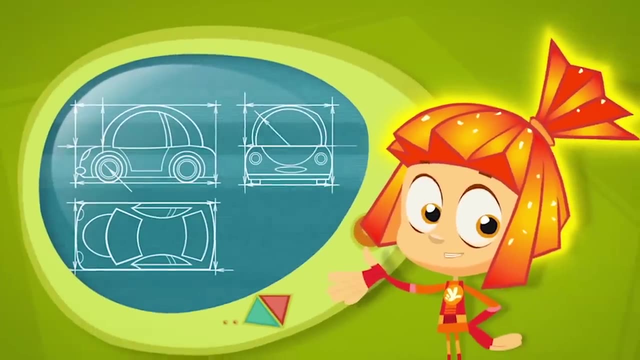 And that's not all. If the object is complex, it must be drafted from at least three sides, including the front, the side and the top. You see, the object looks different from every side. So if you don't want to work over and over again, learn to draft correctly. 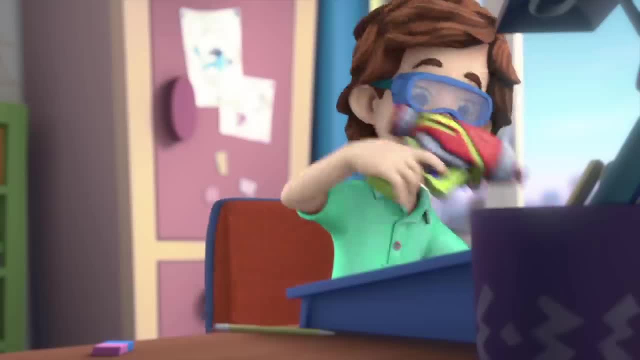 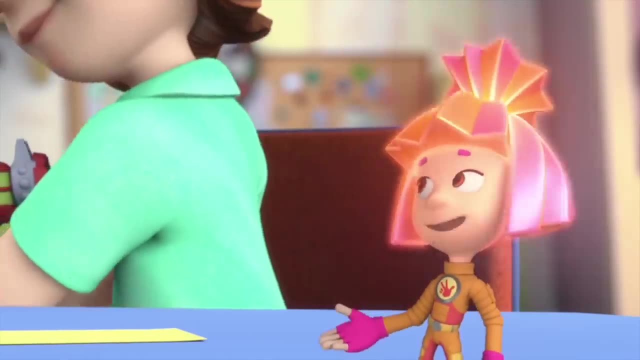 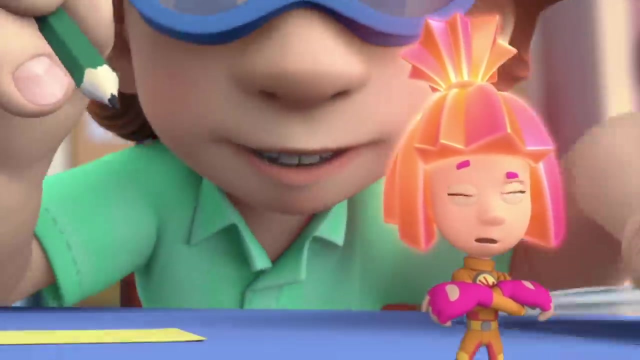 Kaboom, It works, Bullseye. And all thanks to our technical drawings. Yeah, After three tries, right, Some draftsman you are. Now I can draft all sorts of technical drawings, Even one of you, if you'd like. 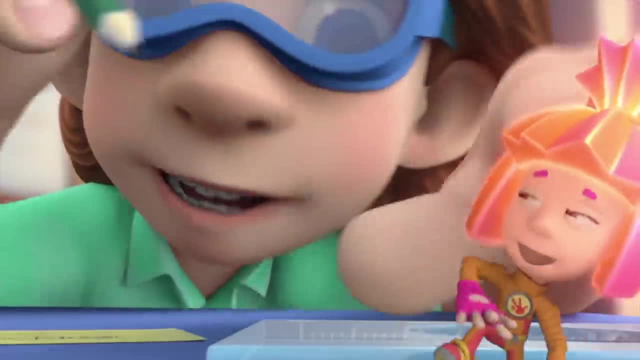 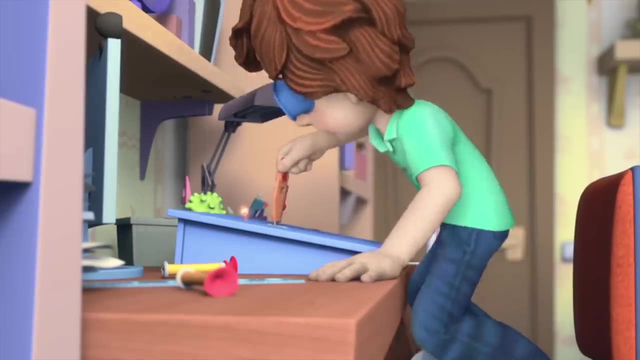 Ah no, don't bother. Hey, that tickles Great. Now do me a favor and turn. Hey, what are you doing there? Just stop. What's going on Now? I think I got it, It's done. 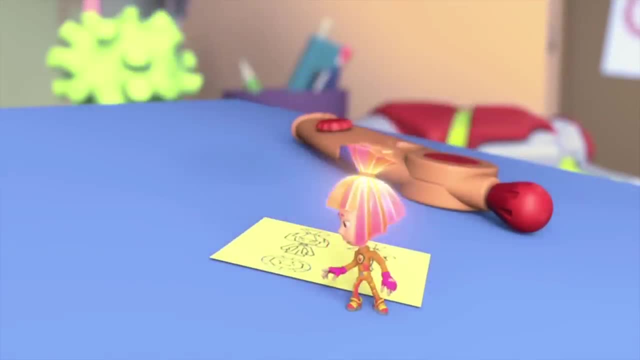 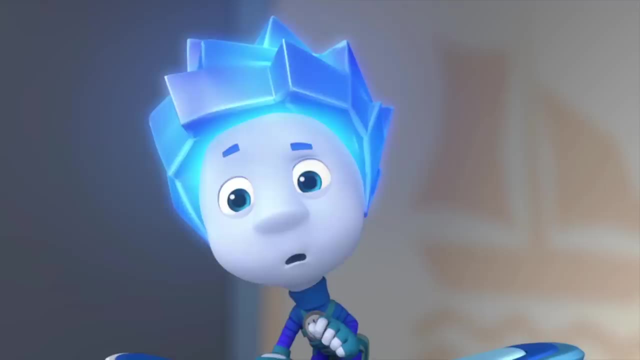 And what's that circle for? huh? That's the top view. You know what Simka? That's what you really look like from up here. Nolik, take this over to Papus. He can use it to make another Simka. 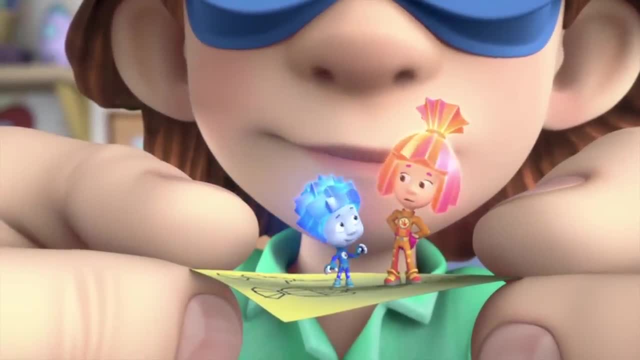 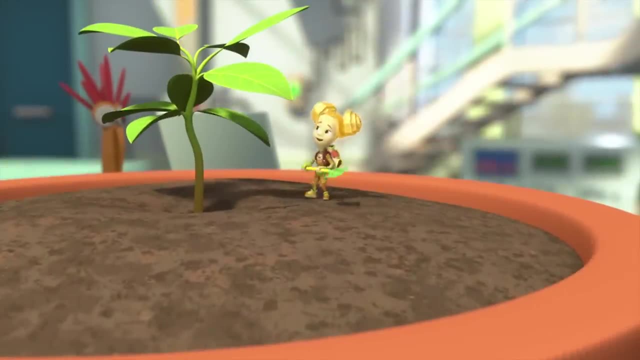 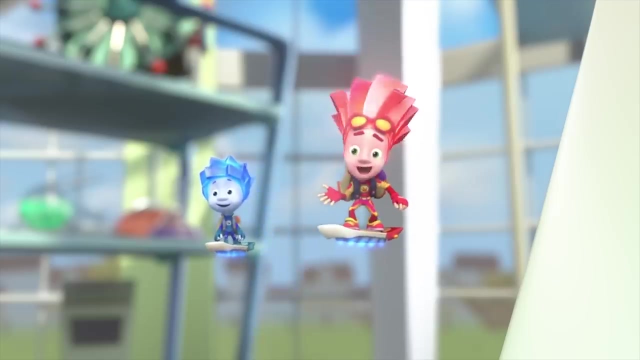 No thanks, Tom Thomas, For me one Simka's: enough Batteries. Oh, my little lemon, just you wait. One day you'll be a strong and splendid tree. She's talking with a flowerpot. Oh, you scared me. 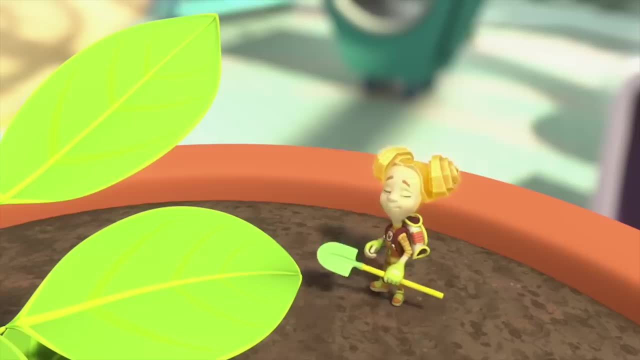 Do you like it? Like what My seedling, Don't? you see? It'll grow into a huge tree And there, amongst the green leaves, will be beautiful yellow lemons. Class From that thing, Lemons, Oh yeah. 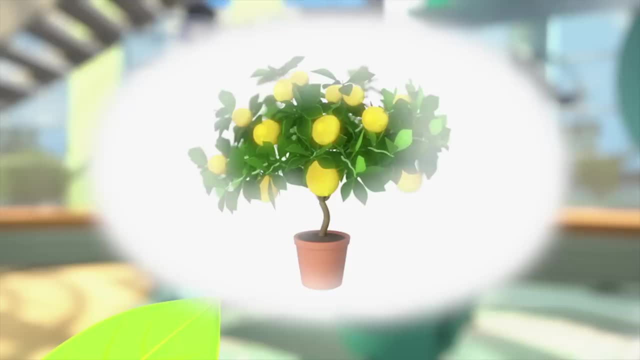 It'll grow into a tree. All it needs for that is to gather energy. Get energy From where? From our sun, The sun. It'll be so slow. All right, let's go, Let's go, Let's go. 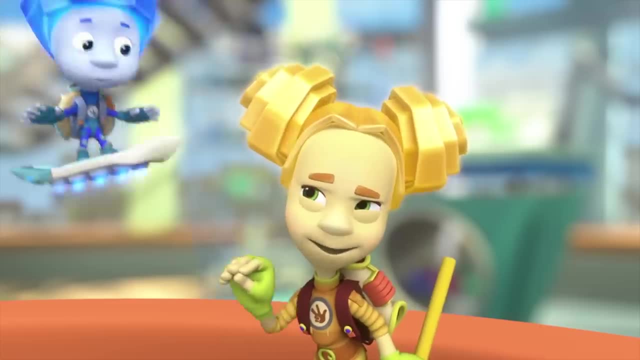 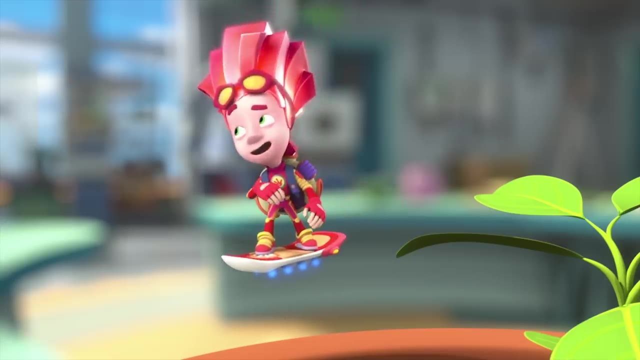 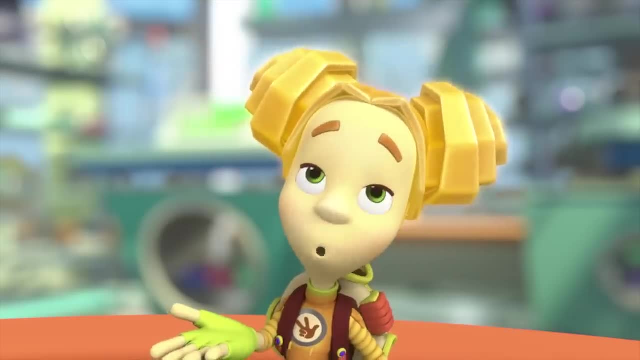 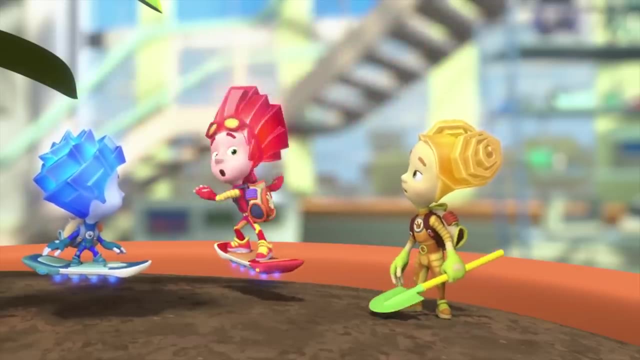 Batteries? I really don't think so, Zula. do you know how much energy they have? Let's just bury a bunch of those batteries in here and you'll be watching your lemon plant shoot up into a tree. Are you positive? 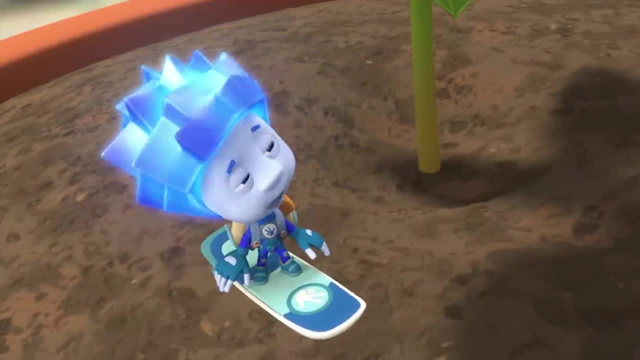 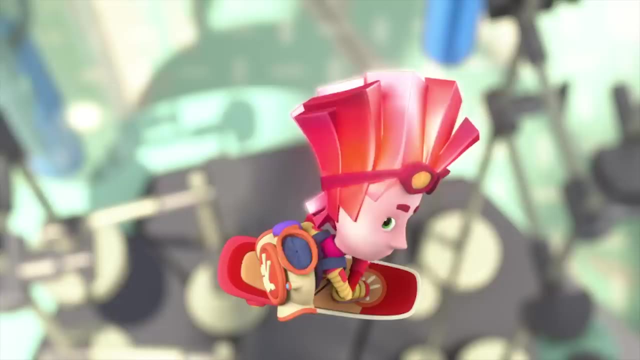 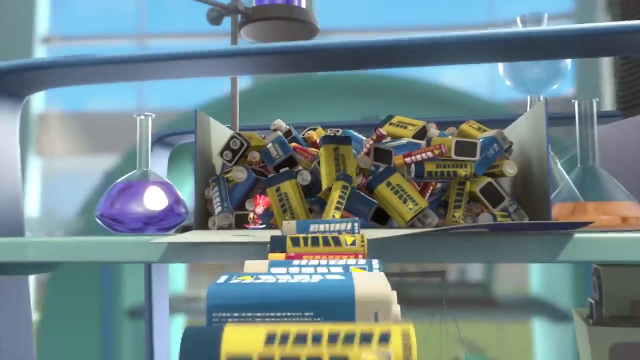 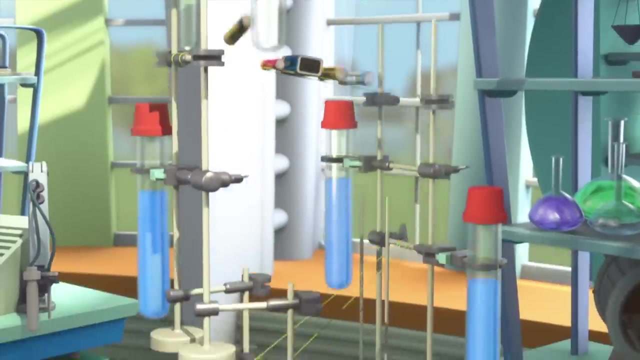 Absolutely. And where can we get the batteries? Over there, Professor Eugenius has a whole box full of them. We use them every day and need them by the ton Batteries- Batteries: They give power to appliances so they can run. 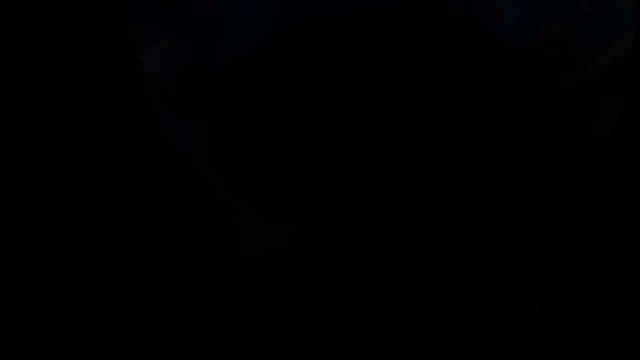 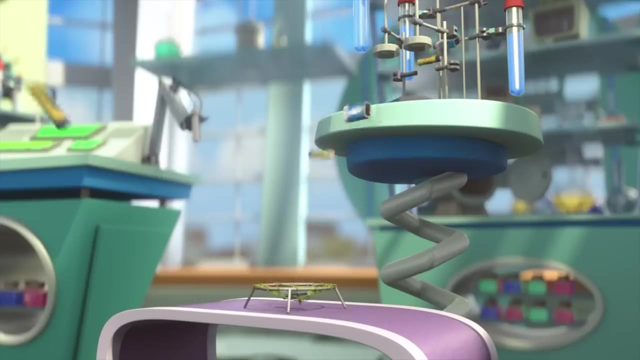 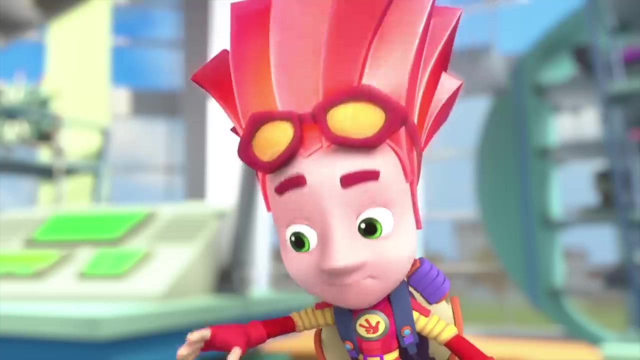 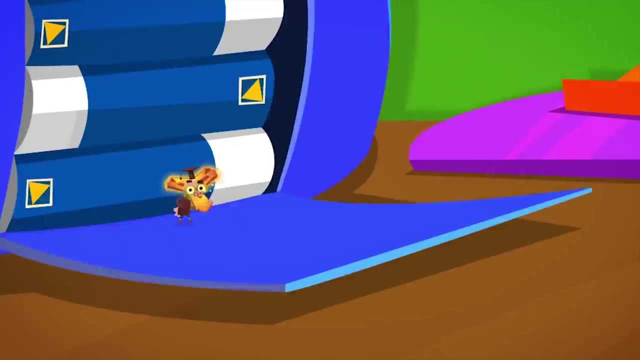 Batteries, Batteries, Batteries, Batteries, Batteries, Batteries. That does it. We'll be seeing the first lemons before the week's over. The first battery in the world was made in Italy more than 200 years ago. 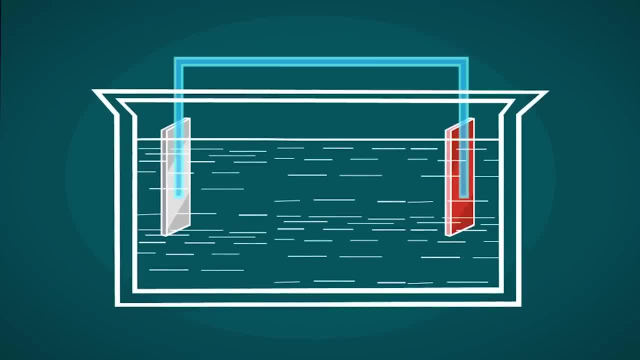 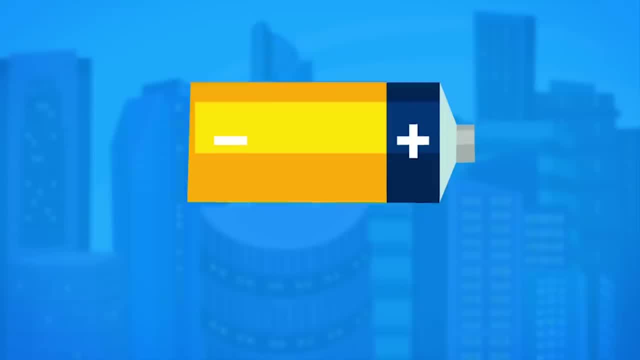 when two different kinds of metal were placed inside a bottle In salty water, electricity started flowing through a wire from one piece of metal to the other. Many years have passed since then, but batteries still work in pretty much the same way. Today, you can find batteries being used for electricity. 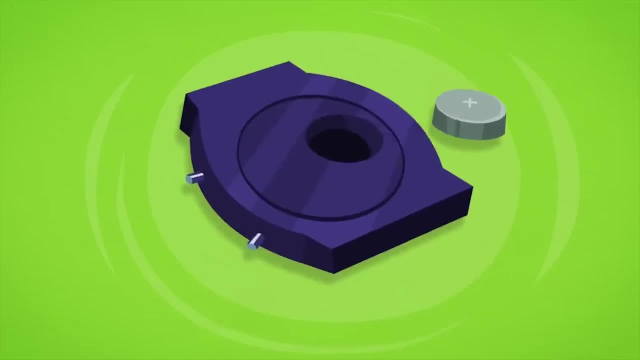 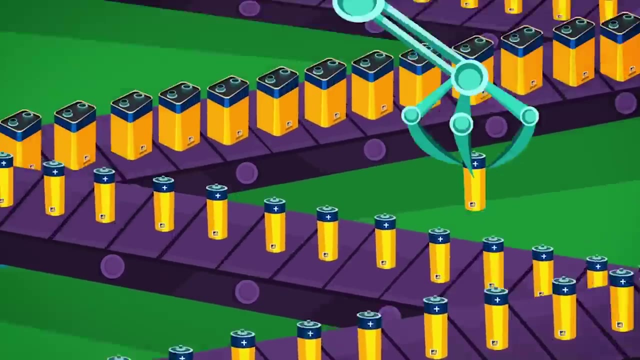 just about everywhere. Tiny batteries are used inside of wristwatches, while big batteries can power cars and even ships. With new batteries being produced by the millions, we have to think how should we get rid of the old ones? You can't just throw away batteries. 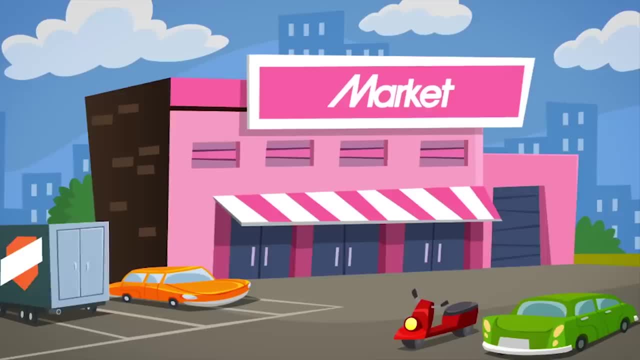 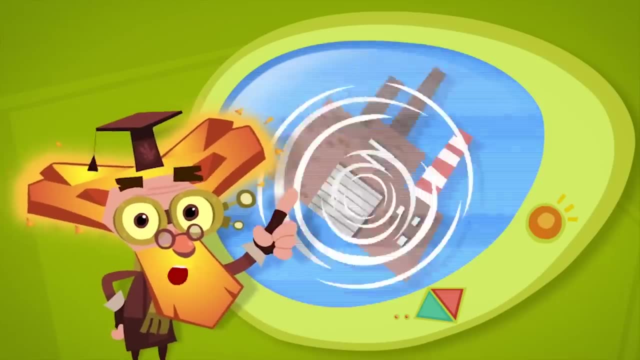 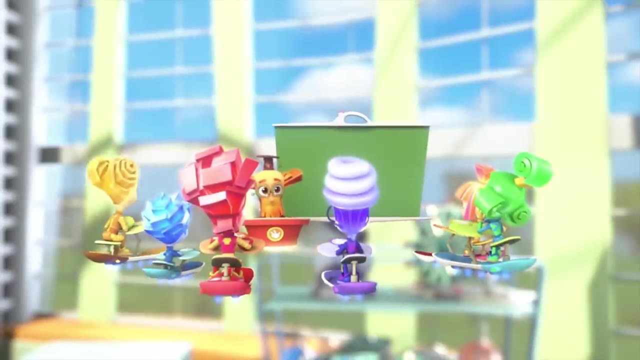 Because they'll poison our soil and water. The best way to dispose of batteries is to take them to a special collection station that sends them to factories for recycling. Yes, yes, It's a terrible idea to bury batteries. You can kill any plants that are growing there. 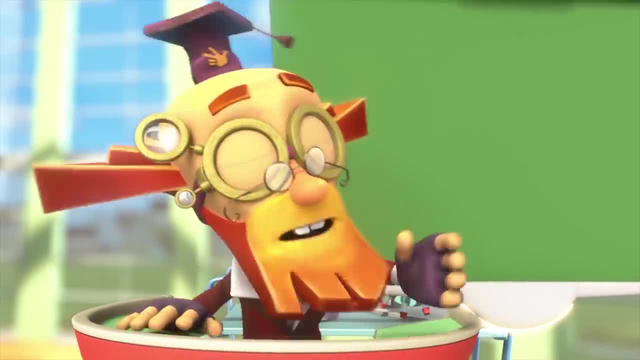 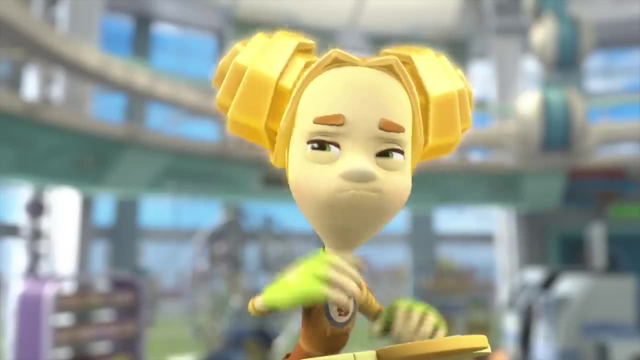 And this is the very reason why Professor Eugenius puts all of his used batteries in that box over there so he can dispose of them properly. Hey, where are they? Oh, my seedling, we harmed you. What? Where are the batteries? 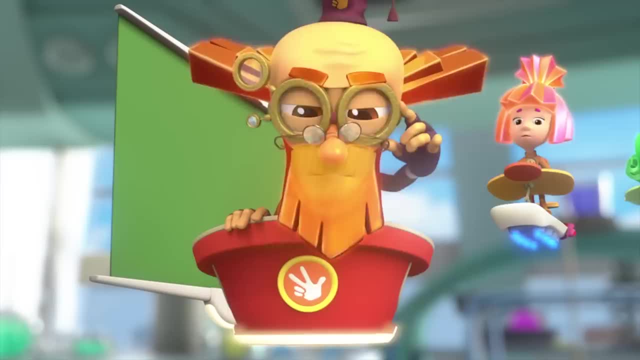 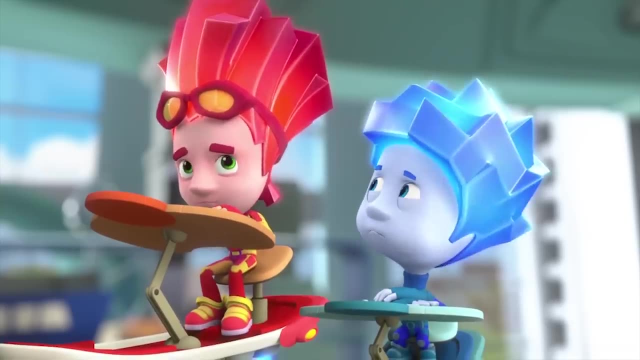 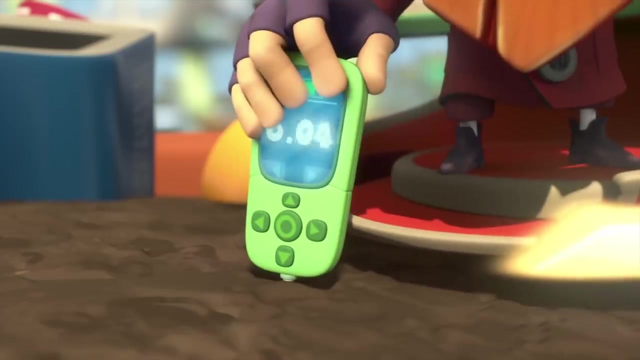 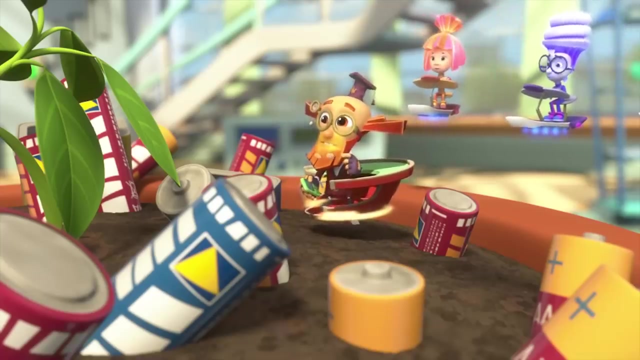 They're in the flowerpot. How come So the lemons would grow faster From the batteries? Who came up with that idea? It will die. Hurry, we gotta go save it. Hmph, the soil's contaminated. We've got to find a new home for this seedling. 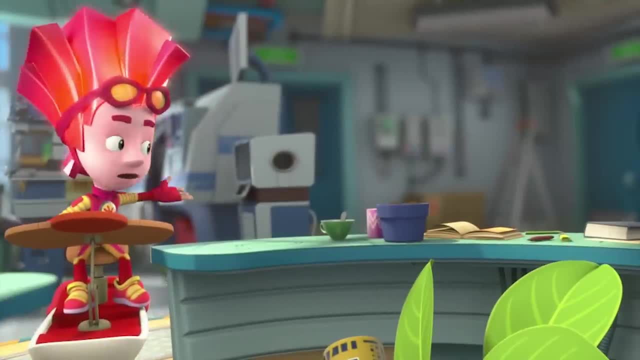 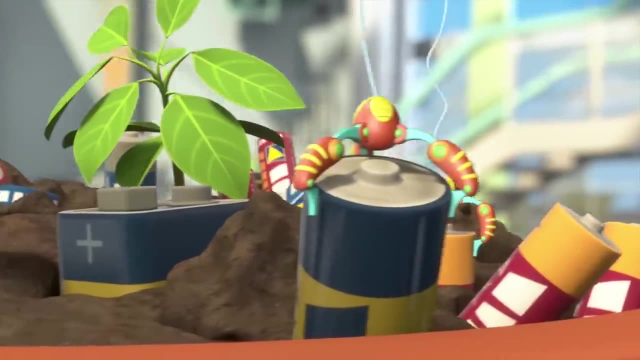 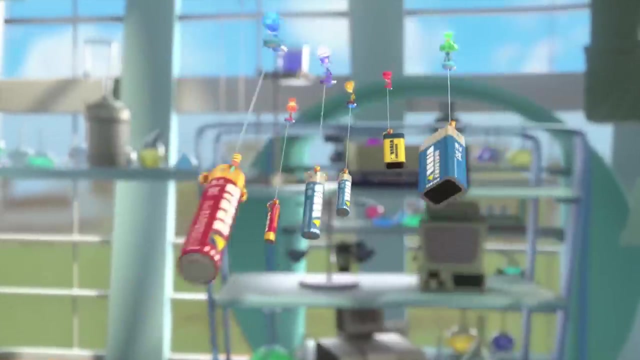 But where Over there There's a pot with healthy soil, Let's do it. Batteries batteries. They come in different sizes, shapes and colors too. Batteries batteries Could be yellow, might be green or maybe red and blue. 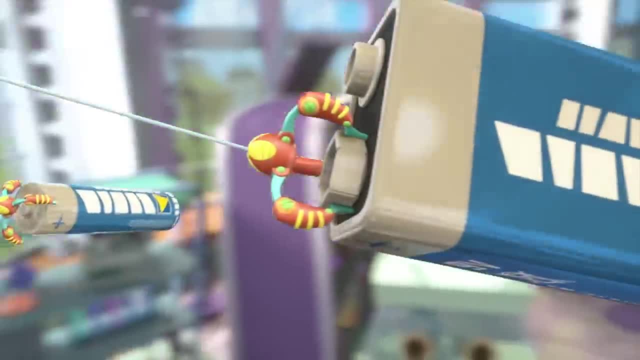 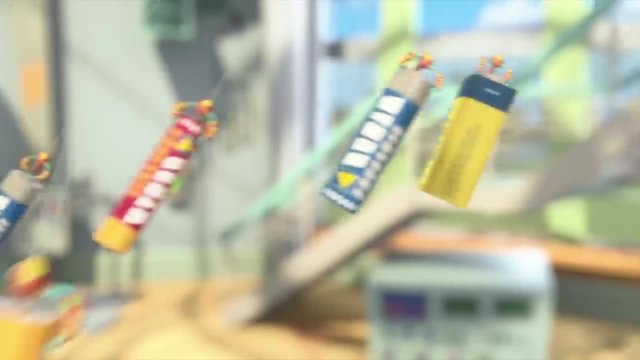 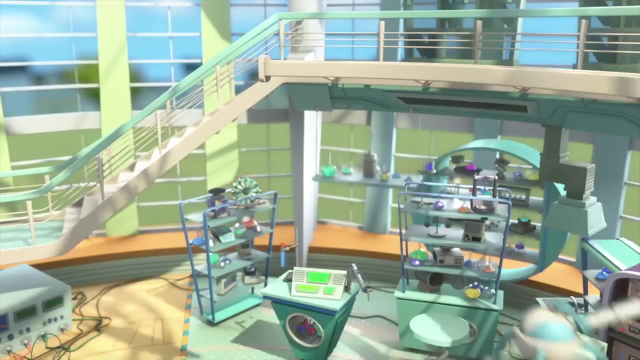 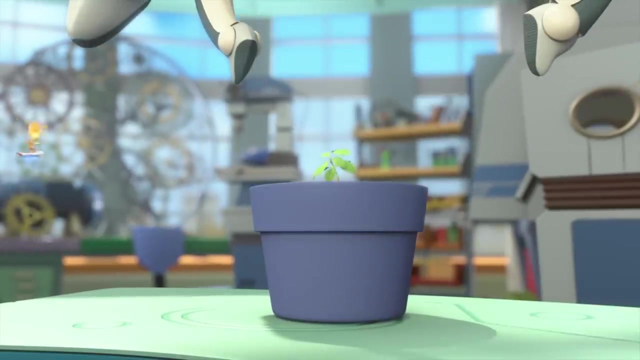 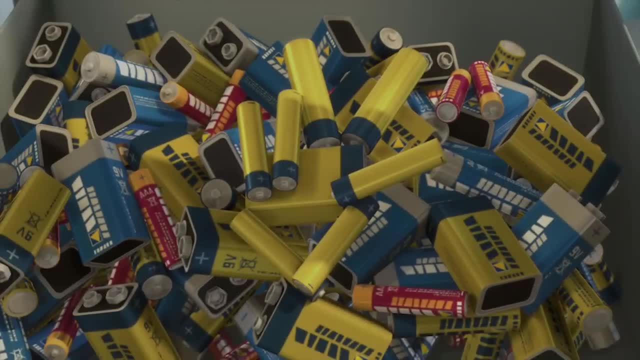 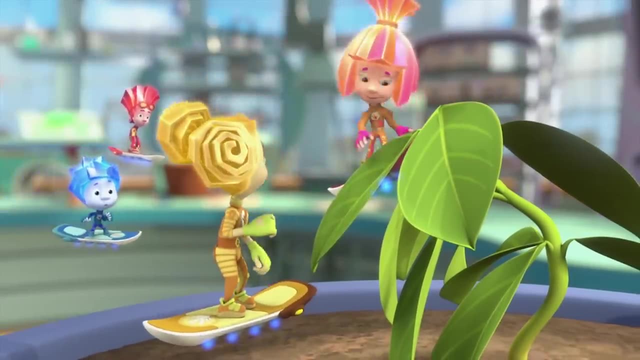 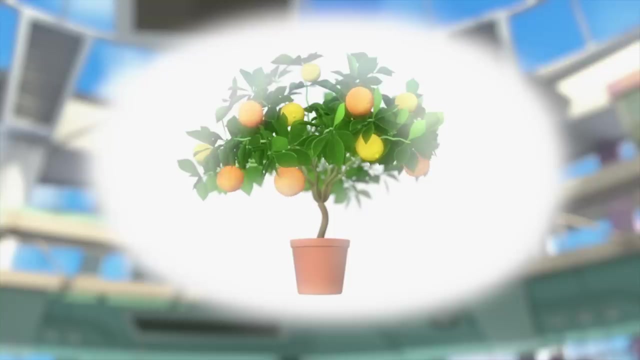 Batteries, batteries, Batteries. Don't cry, Tula. The seedling will be perfectly fine. It will grow big and strong with branches full of beautiful lemons And oranges And watermelons. It's a lemon tree Fire. 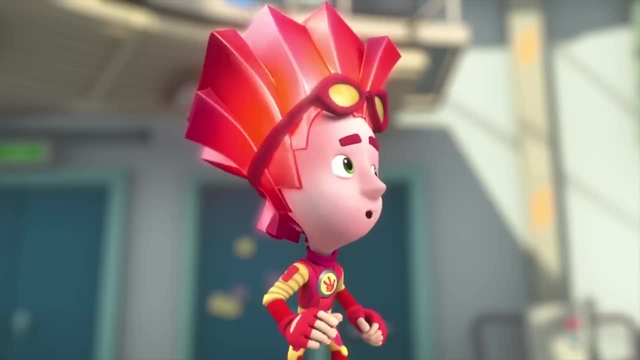 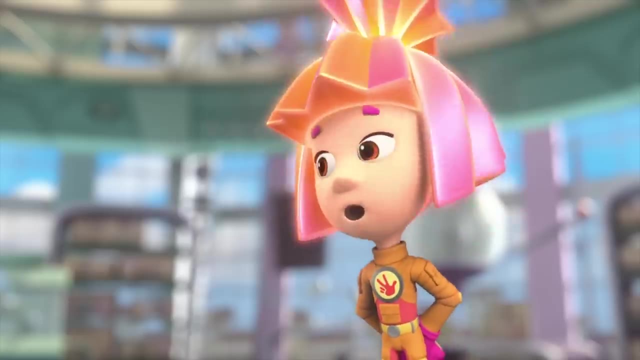 Will you ever stop going too far, Like with the batteries? Well, anyhow, batteries are cool, right? Look how many appliances can't work without them. You're right, Appliances can't work. Look The seedling's coming back to life. 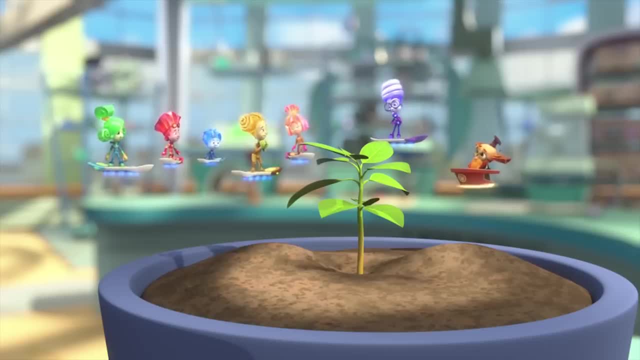 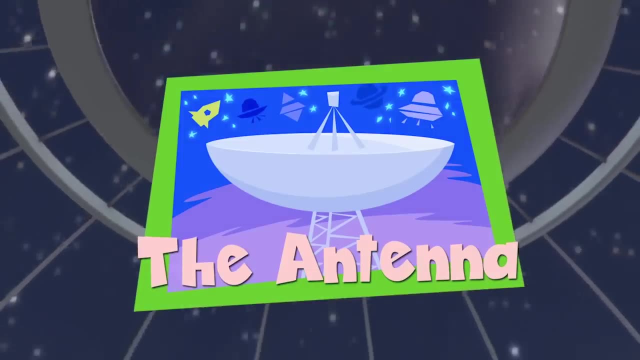 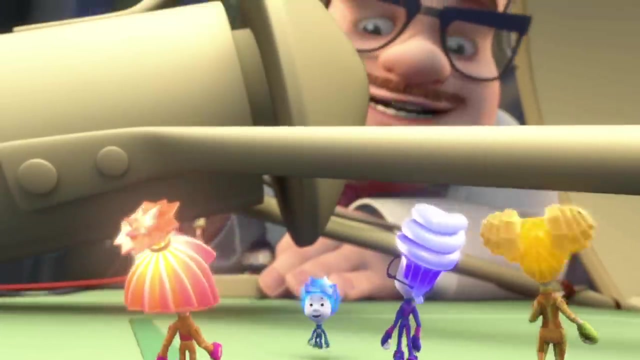 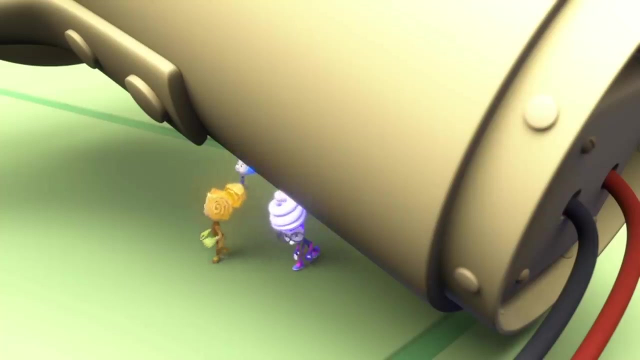 It really is, Tula, tell us, isn't it splendid, Splendid, The antenna. Wow, is this cool, or what? Ah, hello there, little Fixies. Did you come to see what I'm working on? Professor Eugenius, tell us what you're planning on doing. 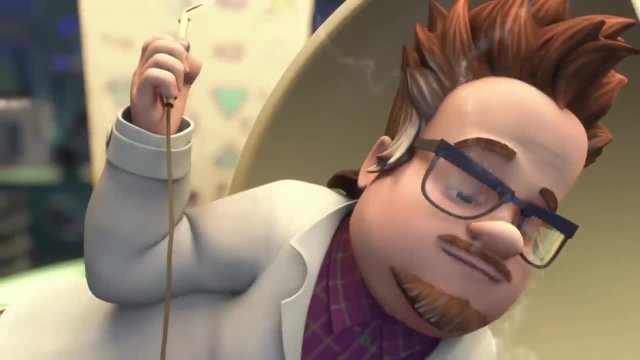 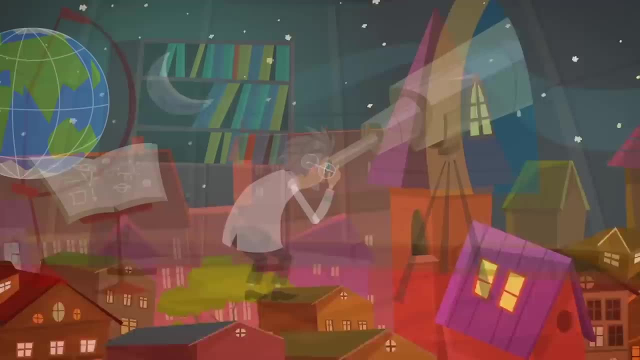 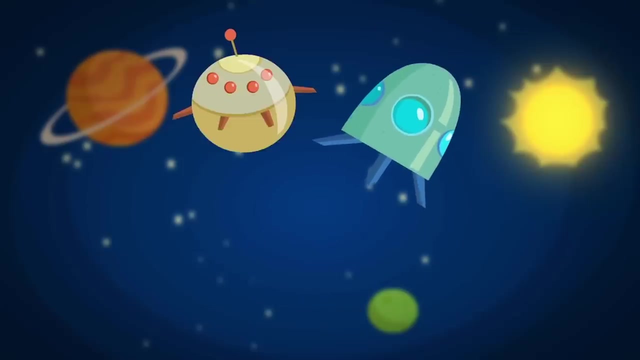 with this huge thing. Well, I hope to use this fantastic device to make contact with aliens. Since ancient times, people have wondered: is there life on other planets? What might aliens from outer space look like, And what kind of spaceships do they travel in? 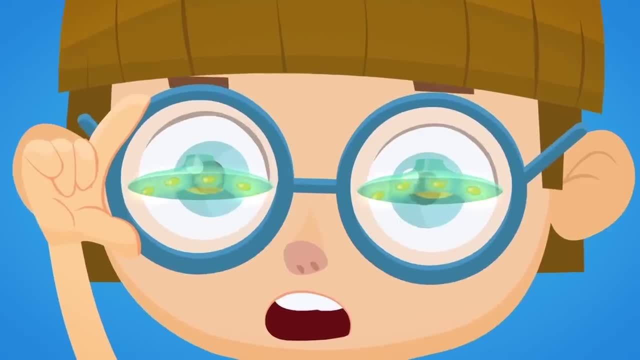 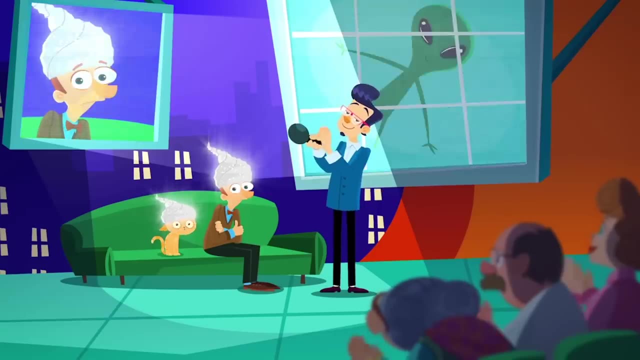 There are some people who say that they've seen alien spaceships and that they look like flying saucers. There are even some people who say they've actually made contact with aliens, But personally I'm sure it's just their fantasy And science hasn't been able to prove any of these stories either. 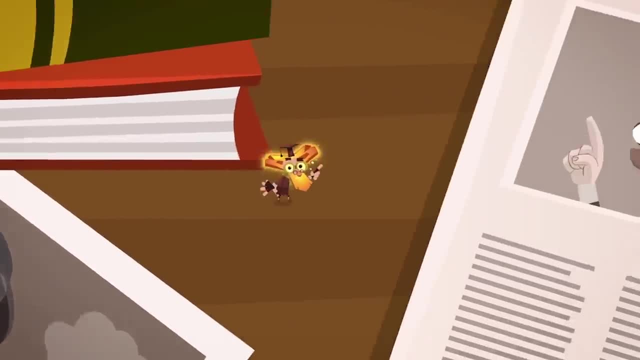 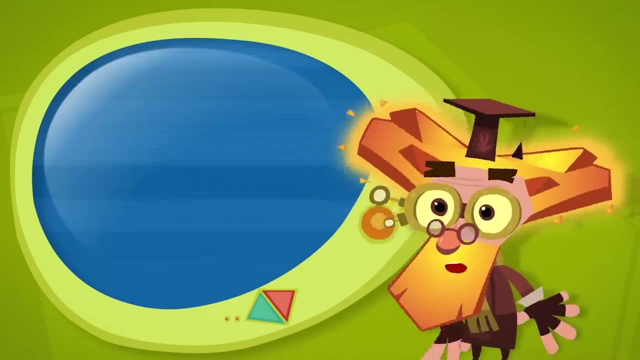 The one story that makes me laugh harder than all of the rest comes from a guy who claims that he saw aliens with his own eyes. Can you believe it? He said that there was a group of tiny aliens that looked like humans with glowing hair. 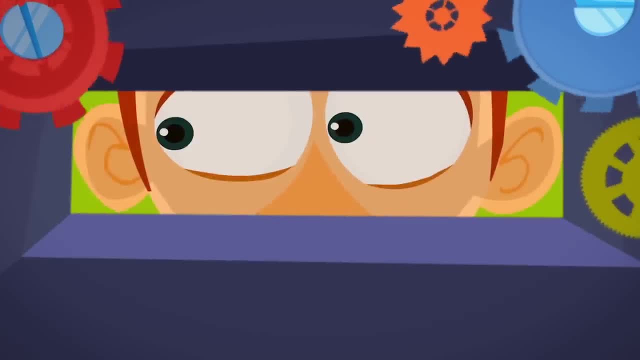 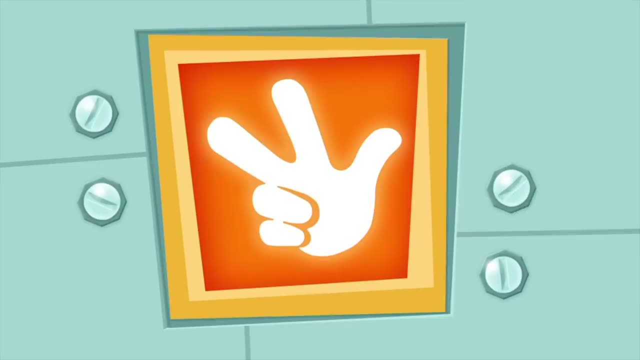 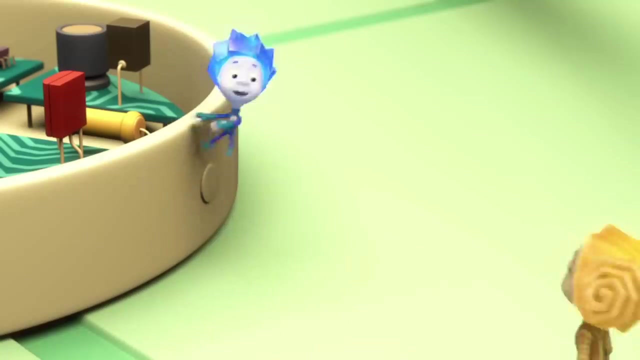 It seems to me that this guy just happened to spot a few Fixies who weren't able to hide from him in time. Ha-ha-ha-ha-ha, It's ready. And now what If the aliens are out there flying by the Earth? 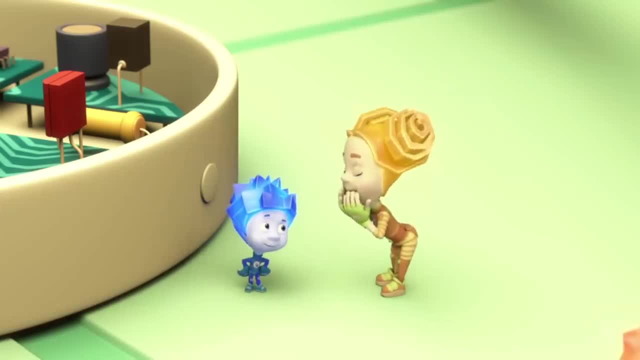 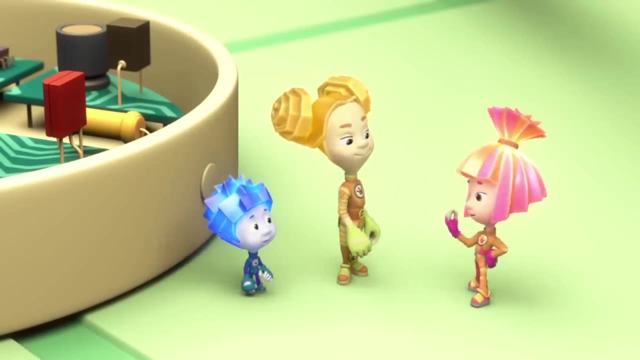 they'll see this plate, get hungry and come for food. Aliens don't need a plate like this silly. When they've got plates that fly Flying saucers, You're both silly. This thing isn't a plate at all. 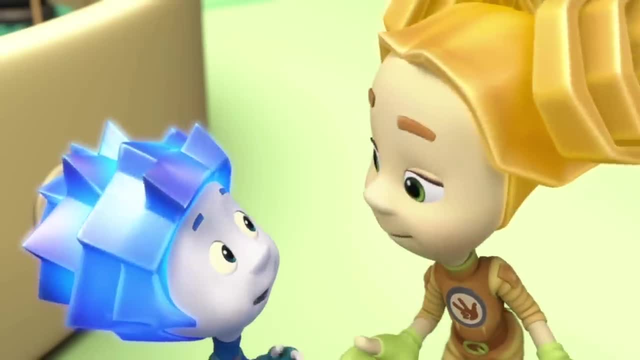 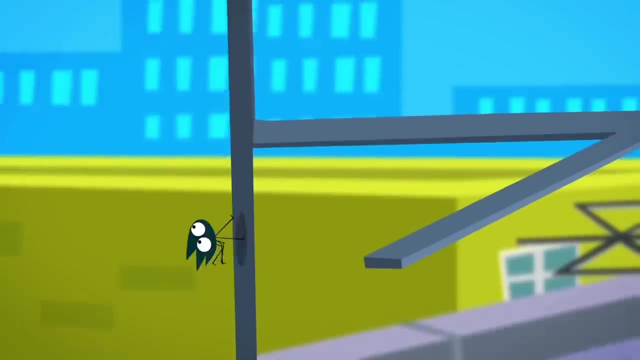 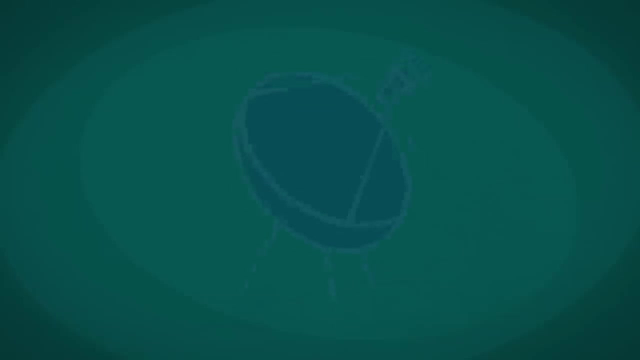 It's an antenna Antenna. Antennas help people receive information Radio signals. They come in all sorts of shapes and sizes, like this, this or this, to pick up a signal that's very weak. Powerful antennas that are shaped like large dishes work the best of all. 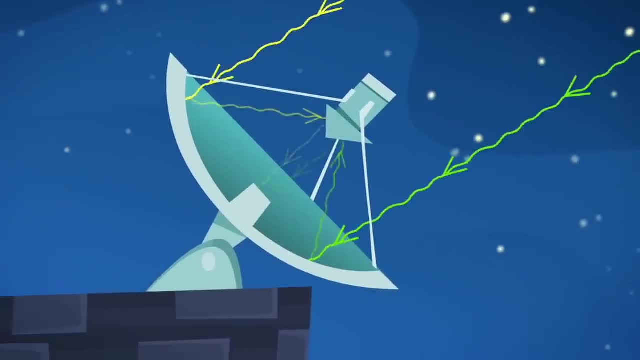 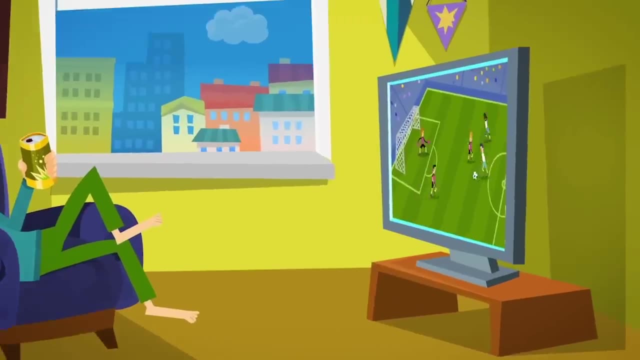 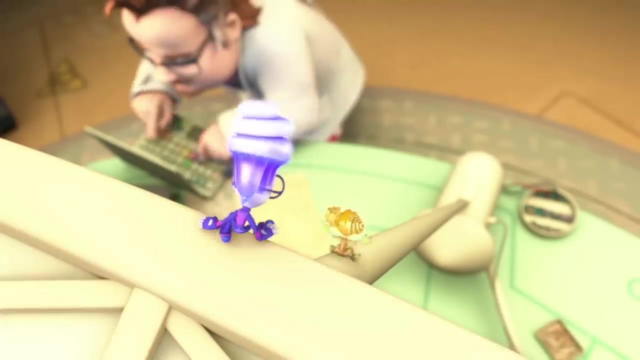 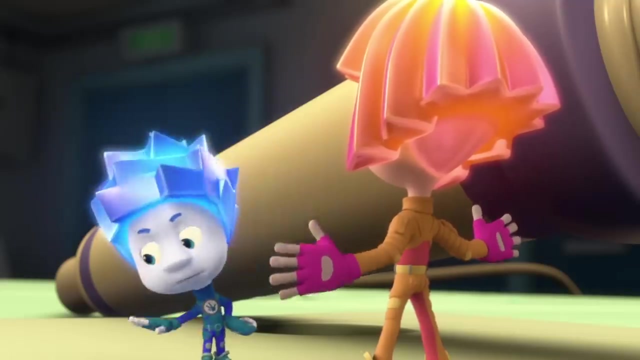 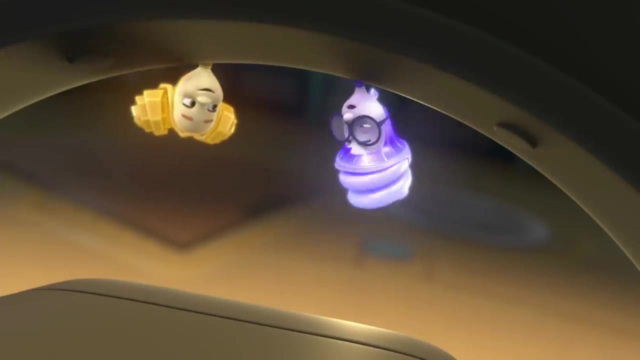 When radio waves hit the dish, the waves all bounce off of it and gather together into one point. This makes the signal stronger and clearer. The most powerful dish antennas can even pick up signals from outer space. And even bigger than that: A small, disgusting little. 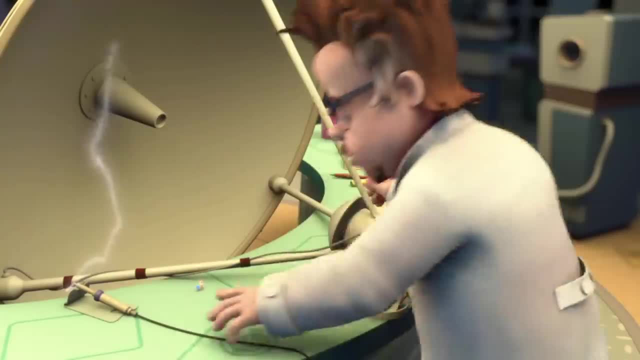 alien. What's that? Nolik, stop, You'll burn yourself. Don't treat me like a baby boy, okay? Ah, interesting. I wonder what's inside of there. Do you know? Why don't we go and take a look? 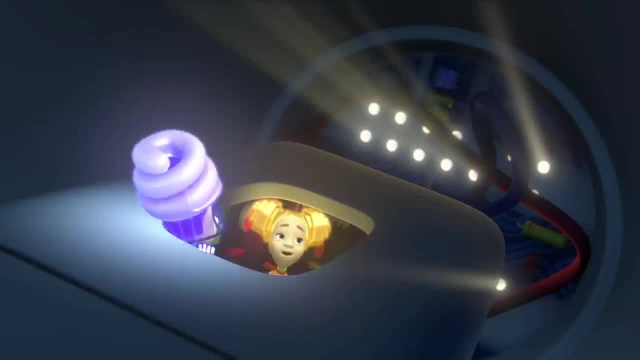 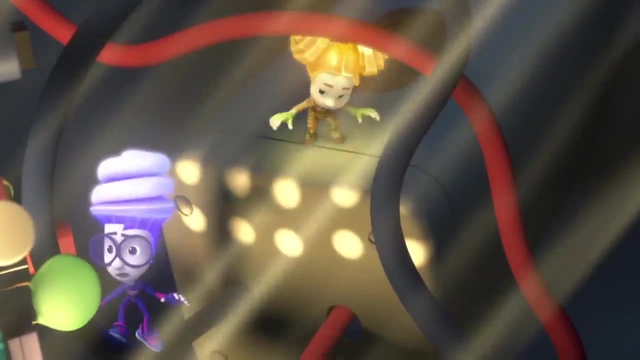 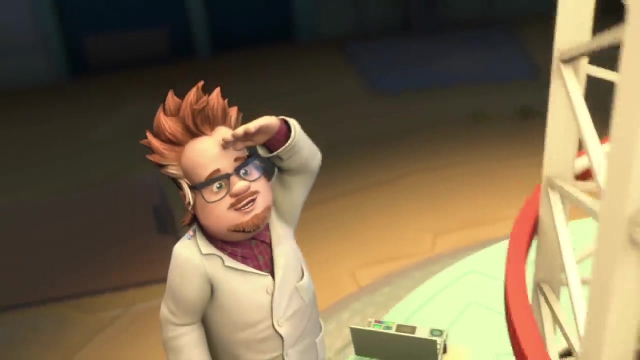 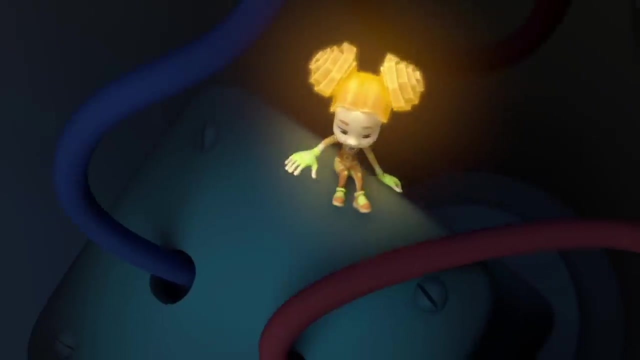 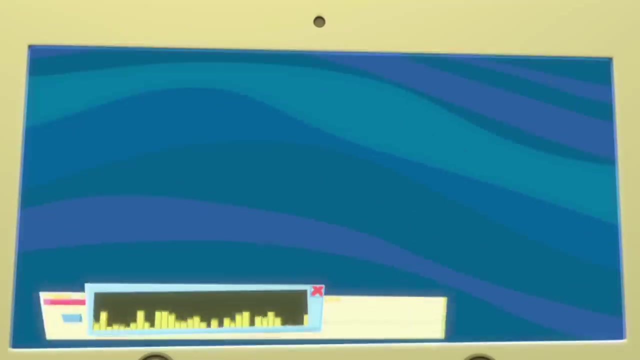 I was only trying to help him out. No need Nolik. The soldering iron is way too hot. And now a-ha Digit, Here we go. Nolik, Simka, let's see if we can pick up signals right away. 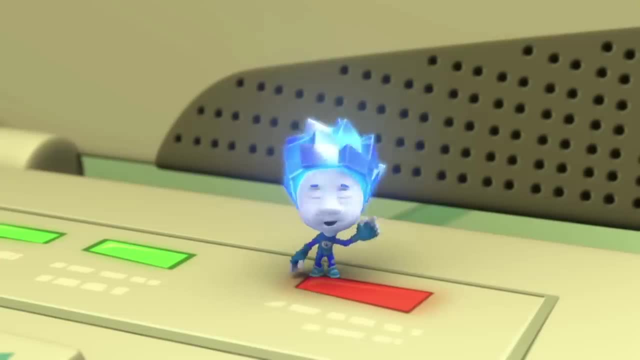 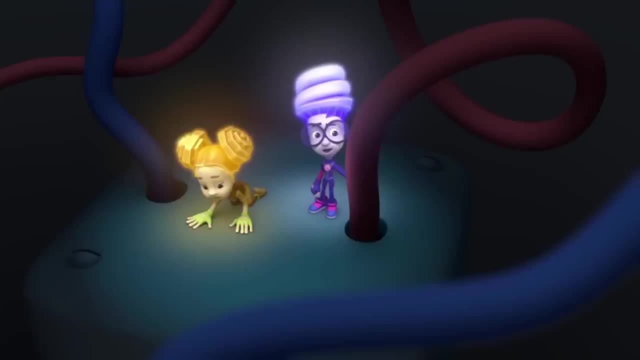 We're going out of space. What do you think? Is it night right now Where the aliens live? What if they're sleeping? Quit bothering the professor with your nonsense. Let us out right now. Can't you hear us? Please let us out. 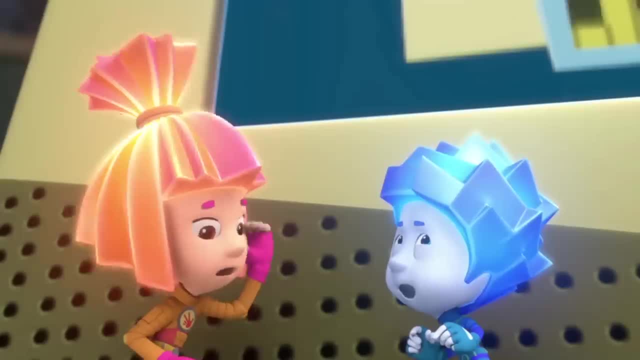 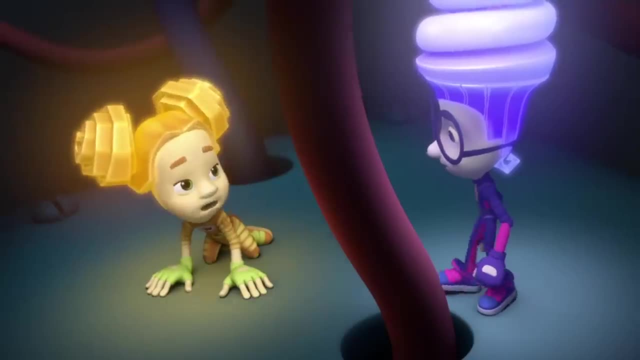 I'm afraid there's no way they can hear us from this far away. I can't hear any signals. It just sounds like static. Be patient, you guys, and keep listening Digit. we all know how clever you are. Can't you think of a way out of here? 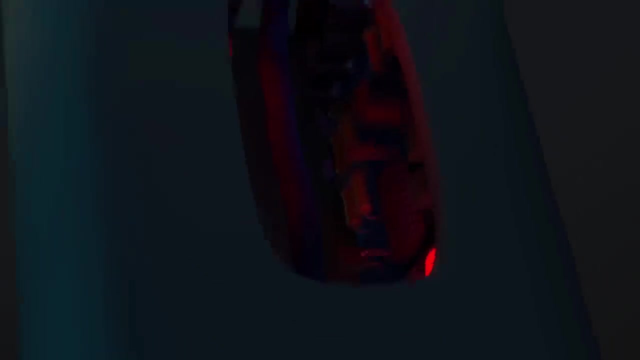 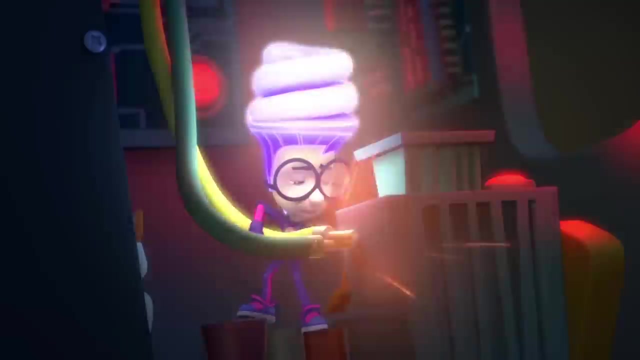 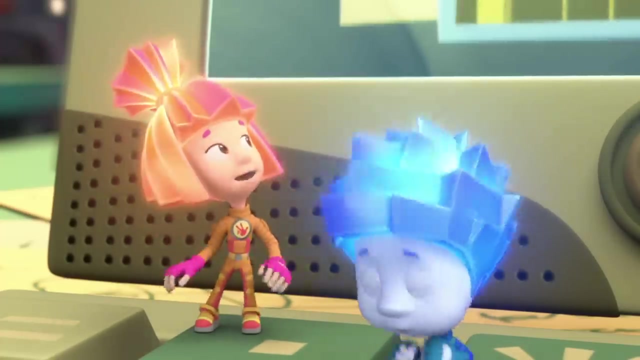 I think I can. I got it, Toola, You stay there. I'll use a special code, I know, to send a signal that we're in trouble. Wait a second. Do you hear that? Could it be a signal from the alien ray? 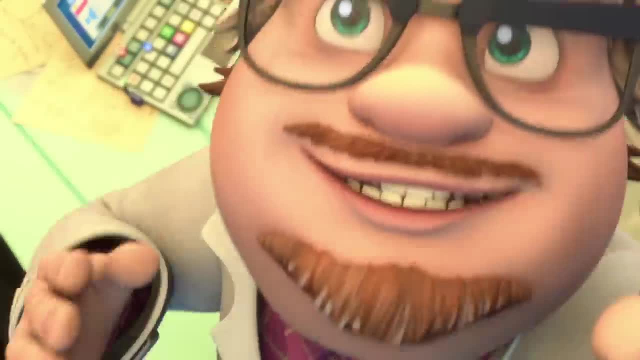 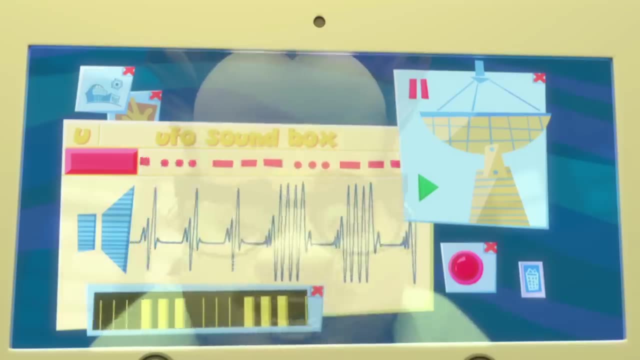 This is sensational. It means that somewhere in the cosmos are intelligent forms of life. Three dots, three dashes, three dots: It's Morse code. It's a signal for help that they're sending. You don't think the aliens are in trouble, do you? 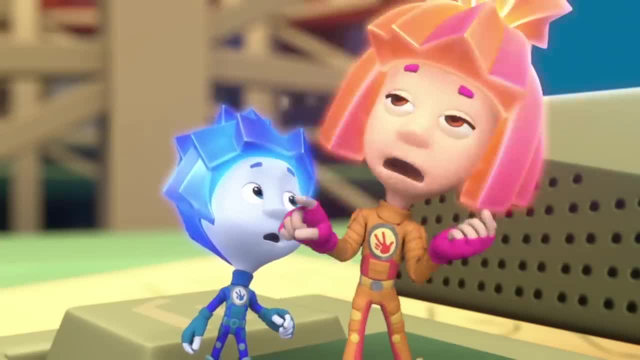 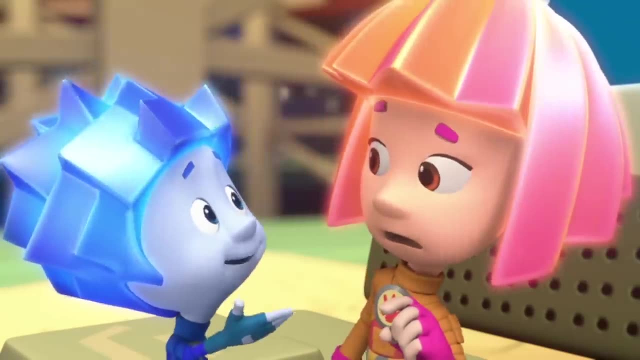 Yeah, I think so. And who do you think they learned Morse code from out there? Yeah, that's strange. There are hardly any Fixies that know that code Digit does. And where is he, you know? And where's Toola? 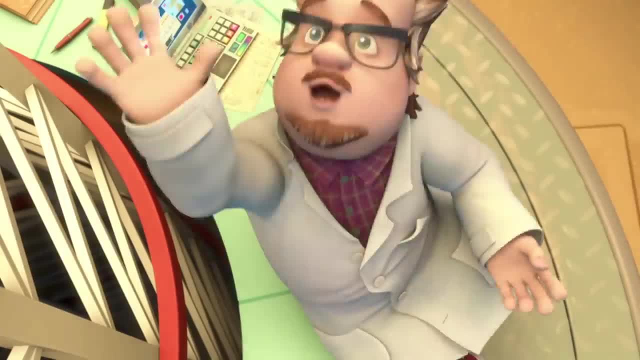 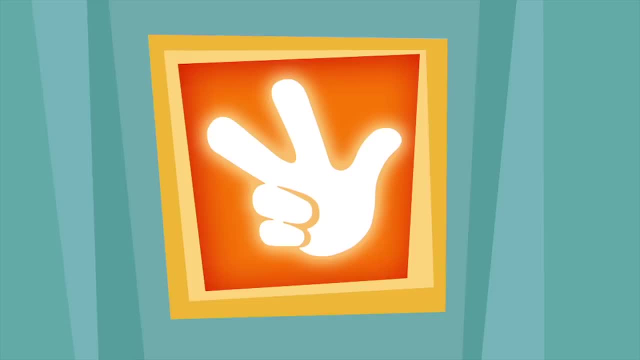 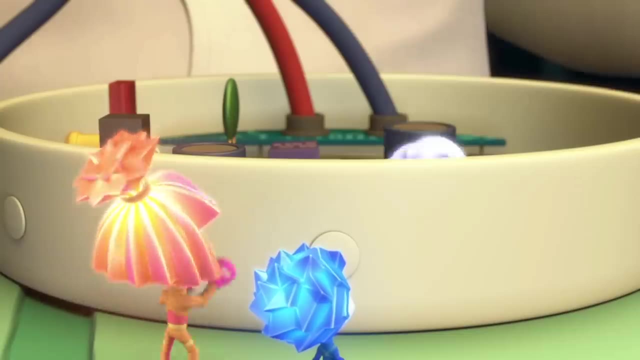 Well, well, I think I know exactly with which aliens we made contact. I think I know it too, Professor Lower, the antenna Greetings to you, oh, extraterrestrial visitors, Hi there, It's good to be back, Oh. 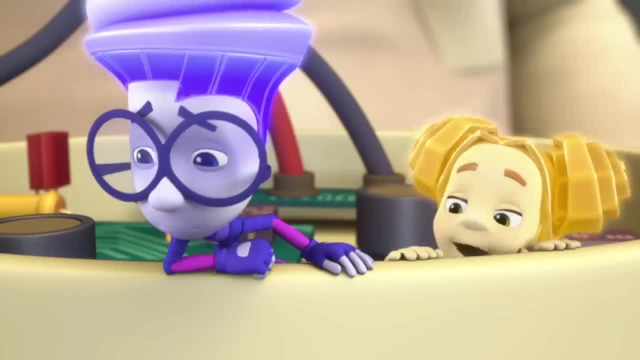 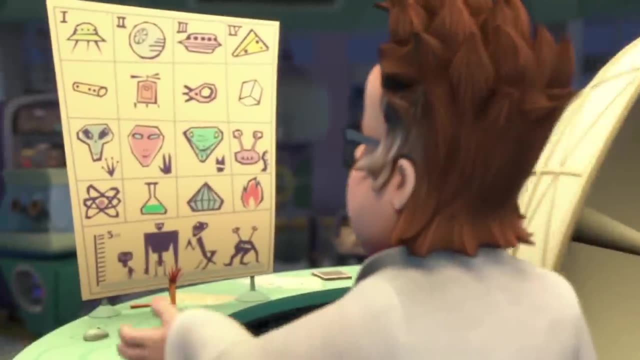 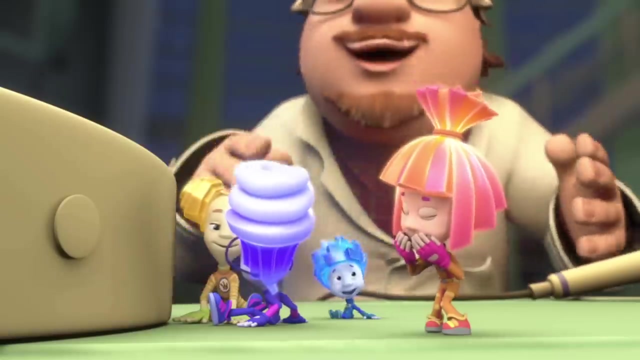 What a shame. I was really hoping that we'd find intelligent life forms out there. It's alright, At least we found two unintelligent ones: The Fixie Phone- Tom Thomas, I'm Tom Thomas, I'm a fox, I'm a rabbit. 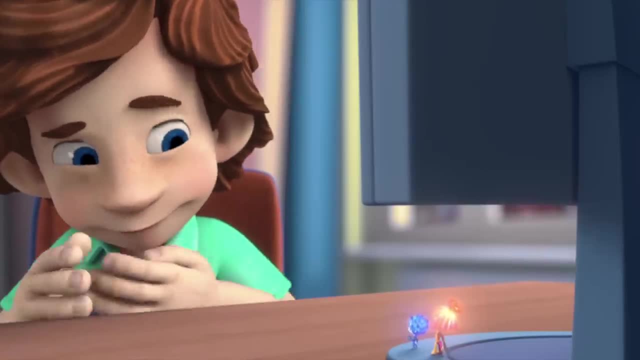 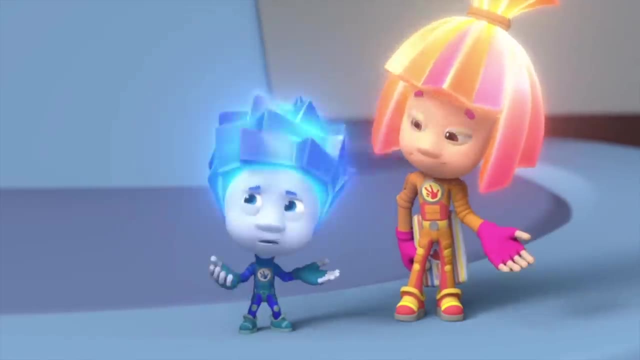 Tom Thomas, Try to guess what we have with us. You guess what I have: A banana, A race car. No, not that Chocolate. A pair of socks. Do you give up? My dad bought a new phone for himself and gave me his old one. 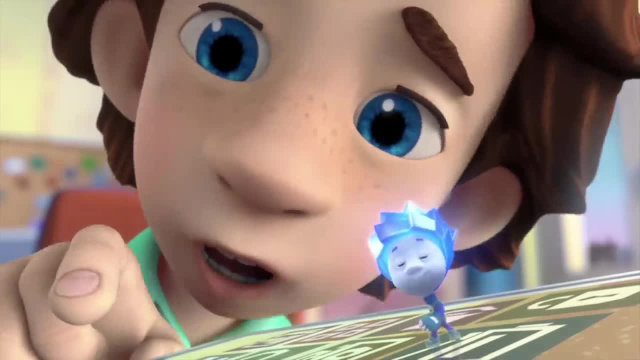 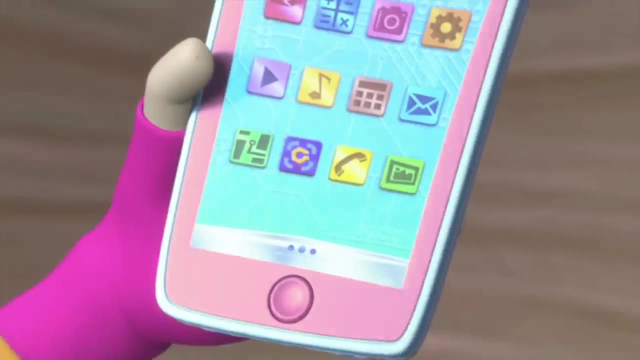 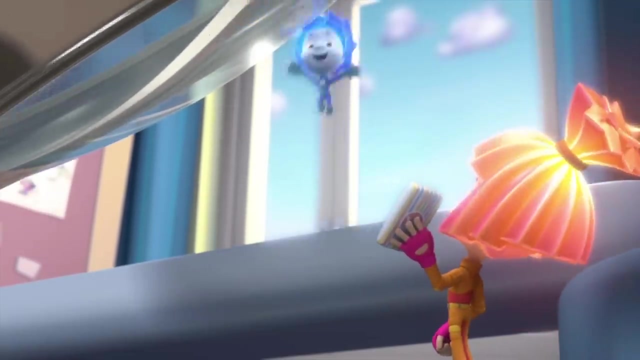 He said I can keep it. Oh wow, And what have you got? Look, Ah, you got a telephone too. It's better than that. This is a fixie phone. Papus got himself a new fixie phone and gave this old one to Simka. 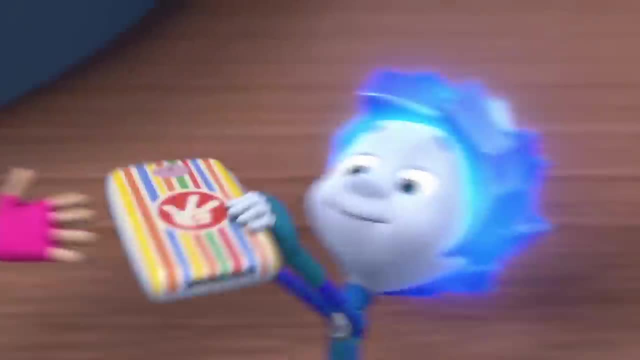 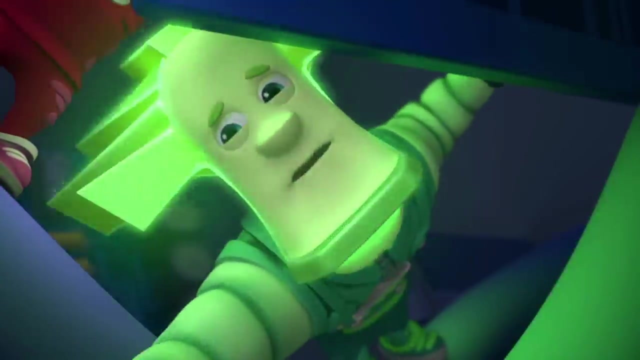 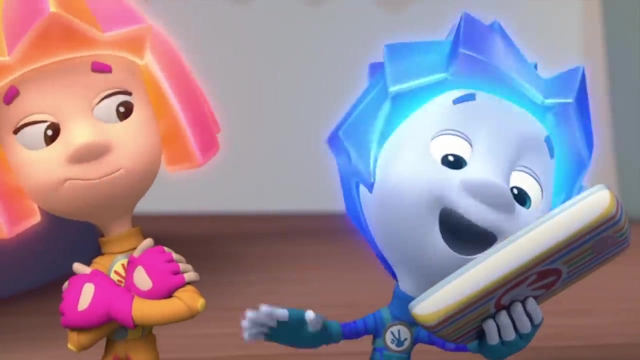 And can you make calls on it? Take a guess, Come on, let me show him. Hi there, Papus. Hi, Nolik. Why are you calling? Just to say hi, Nolik. don't just call me if you know I'm working. 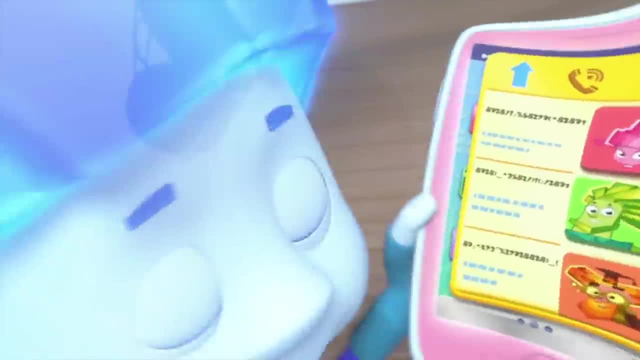 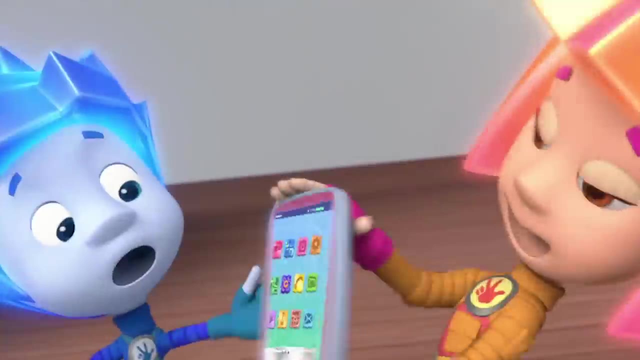 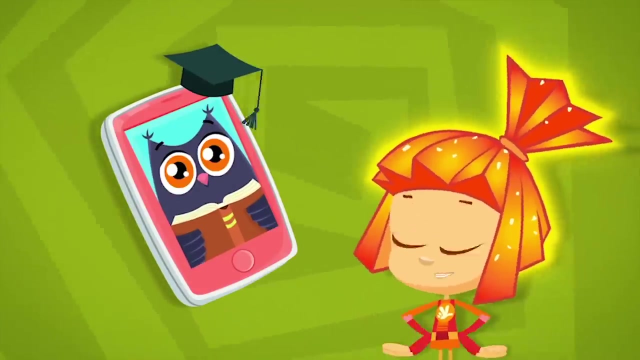 Alright, See that, See that. So what? I can make calls on my phone, Calls to humans, that is, But to fixies you can't. A fixie phone is a smartphone made just for fixies. Not only can fixies call each other with it. 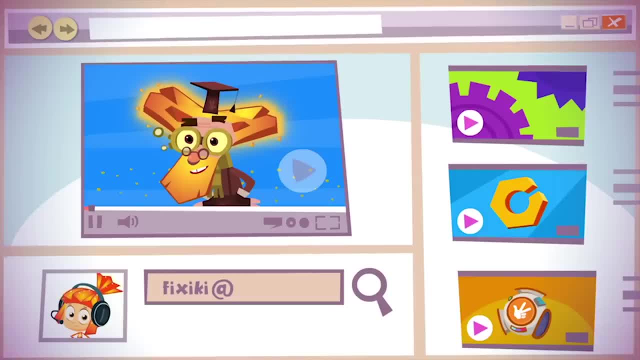 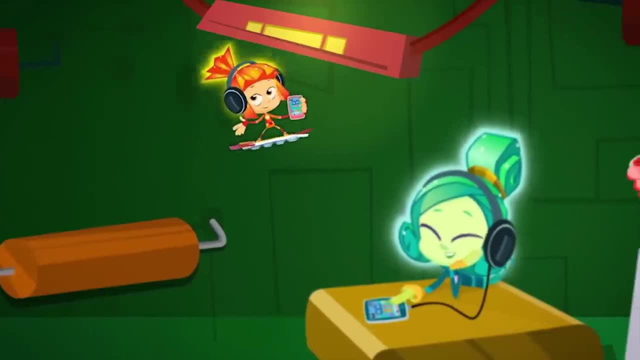 but they can get onto their own special fixie Internet. On a fixie phone you can find a camera, a flashlight, news, games, movies and fixie diddies. Those are the fixies' favorite songs. Fixie kids love them and so do their parents. 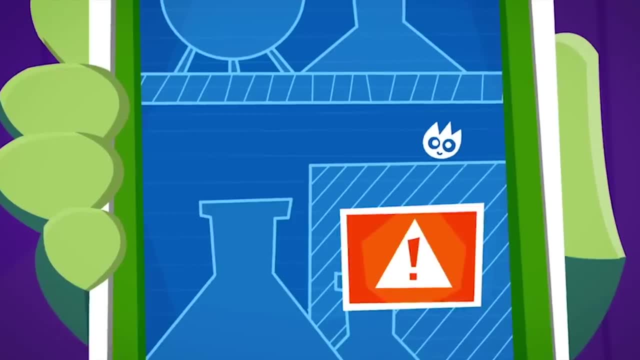 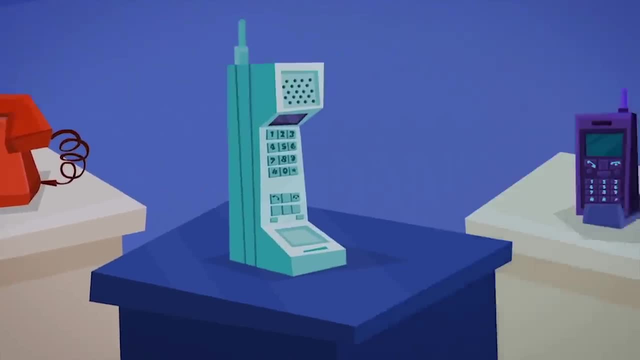 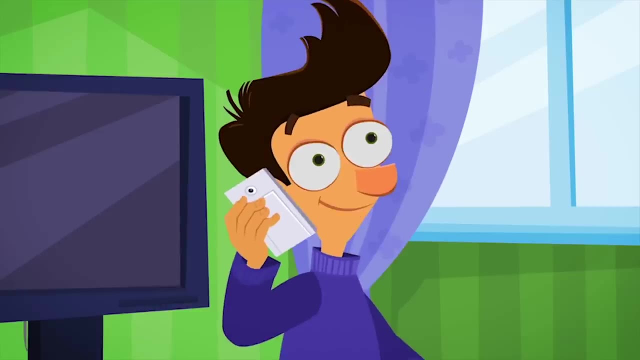 because fixie phones can easily let parents know where their kids are and whether or not they're in trouble. Over the years, humans have learned how to turn telephones into mobile phones and mobile phones into smartphones. They use them to call each other and to go onto their Internet. 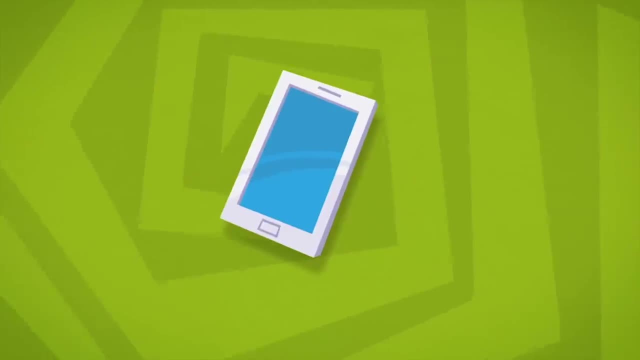 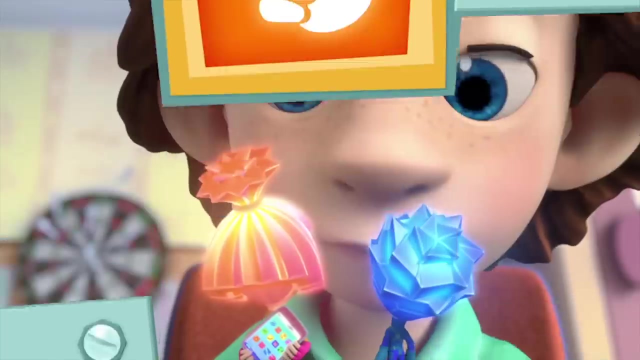 A smartphone is almost as powerful as a computer, but they still have a long way to go, A long way to go to be as good as fixie phones. Yeah, that's really cool guys. Only this phone does the same. But can your phone do this? 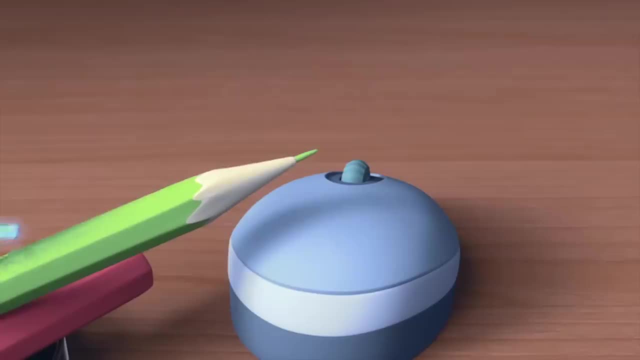 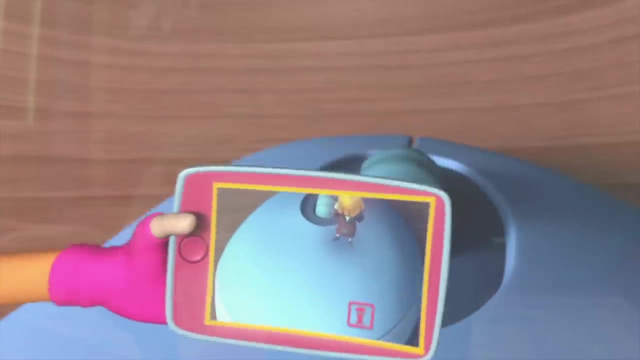 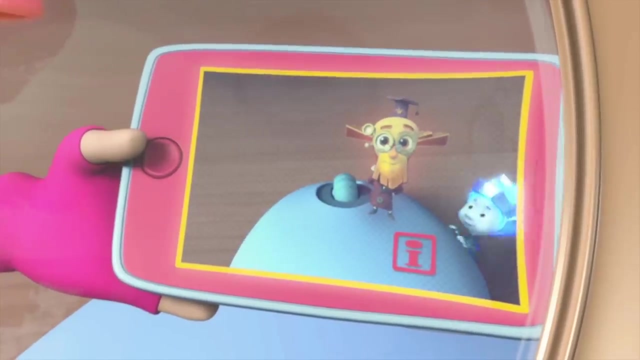 Take a look over here. You mean here It's just a mouse. And now look here, Whoa, But he's not. he's not on there, But look, he's here. And that's not all. Watch, A mouse helps the user navigate around the computer. 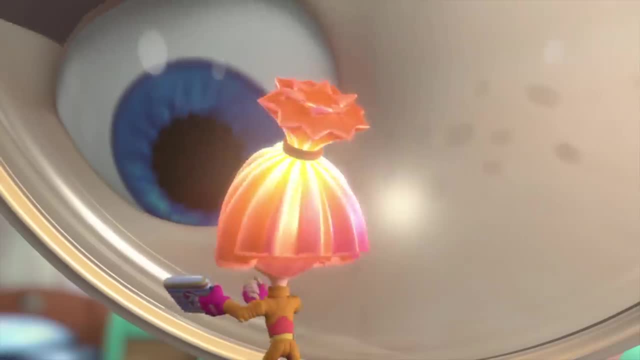 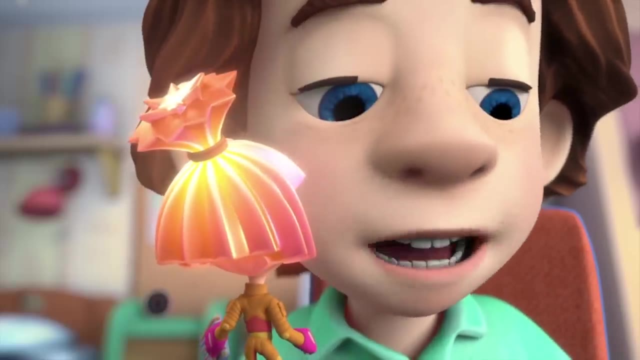 And when we move it You get it. No one else can see the fixie except for you, And he can help you Super. Oh, it'd be great to have my own fixie phone. What are you talking about? You're not a fixie. 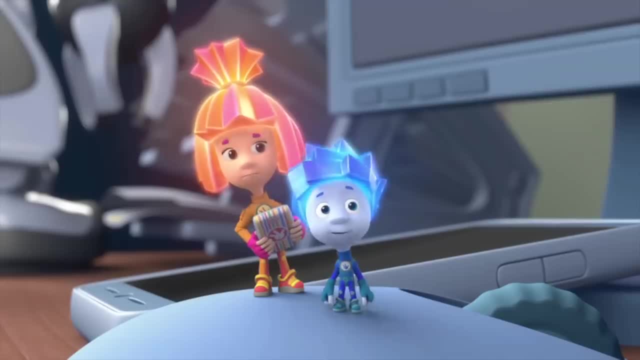 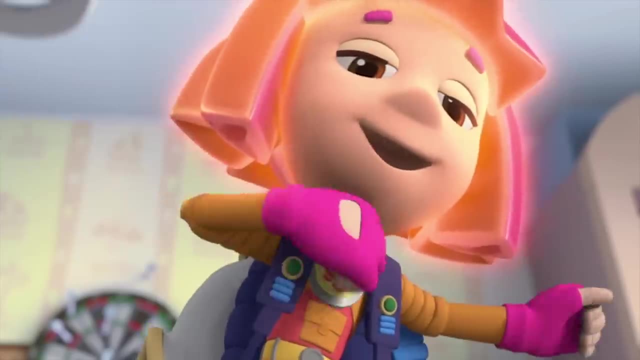 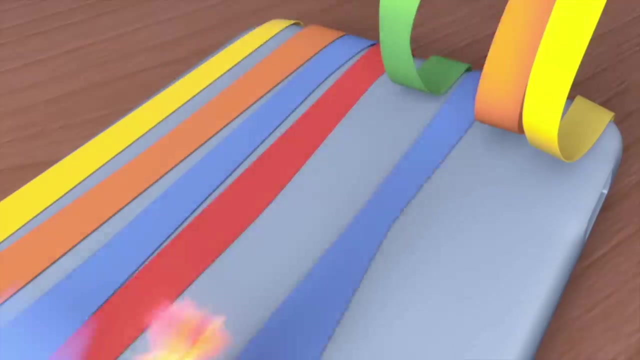 What a shame. I'm off to school guys, He gets so upset he even forgot to take his phone. I have an idea: Bingo, My smart phone's my best friend. I love to hear it beeping, So I keep it by my side, even when I'm sleeping. 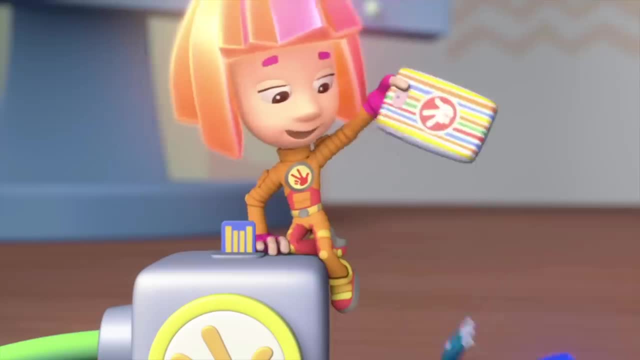 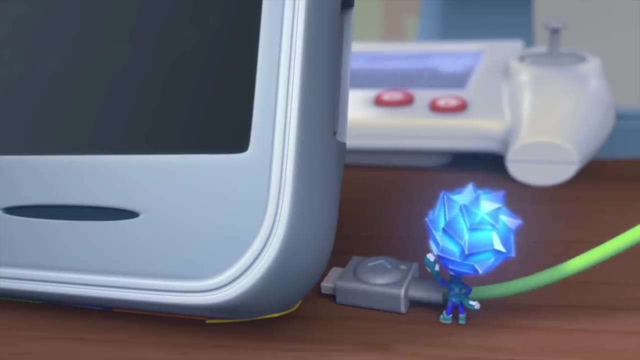 Bing bong all day long, Bing bong all day long, Bing bong all day long. even when I'm sleeping With my phone, I play alone. I don't need my brother. Soon they'll make a brand new app to replace my mother. 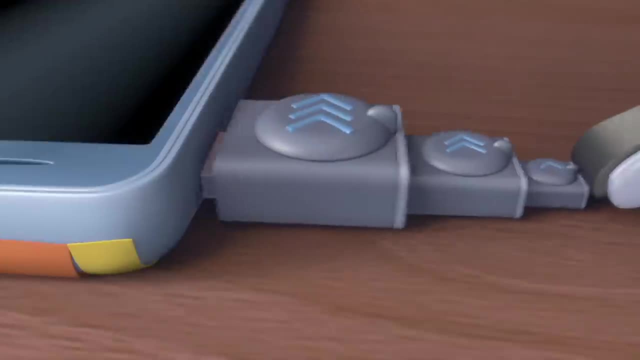 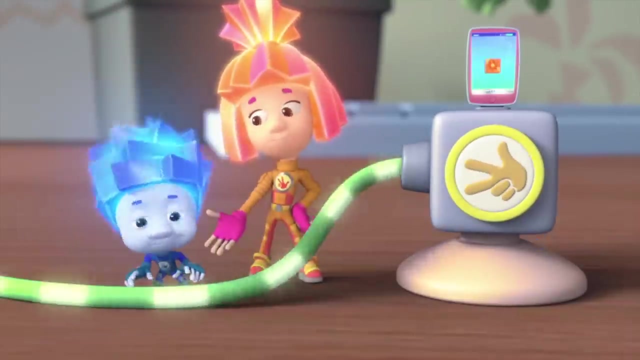 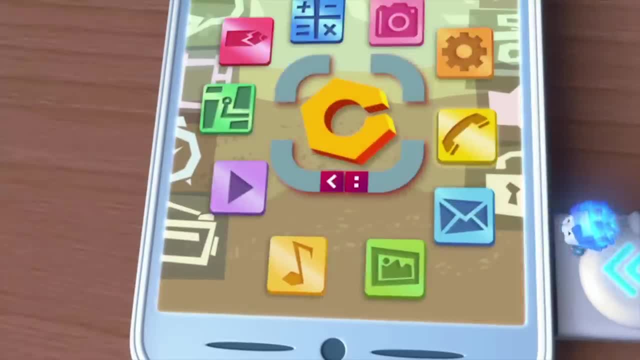 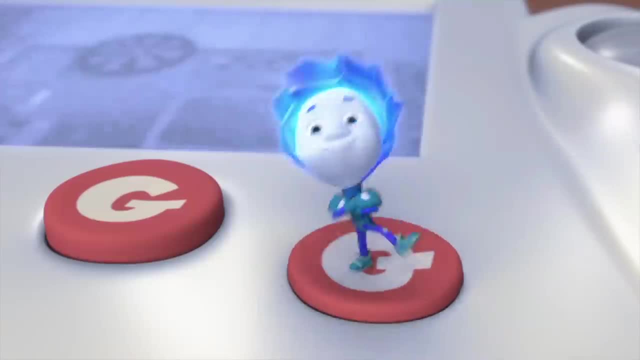 Bing bong all day long. bing bong all day long. bing bong all day long. now I'm out of power. Bing bong all day long. bing bong all day long. bing bong all day long. now I'm out of power. 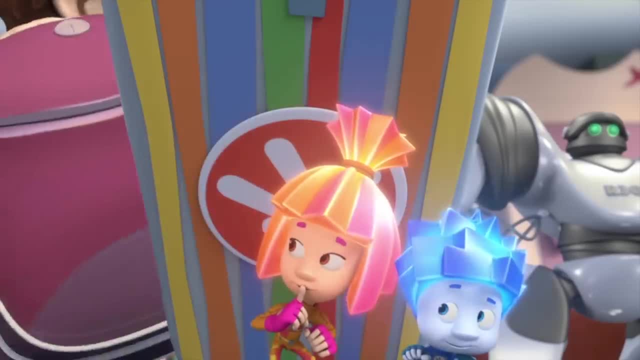 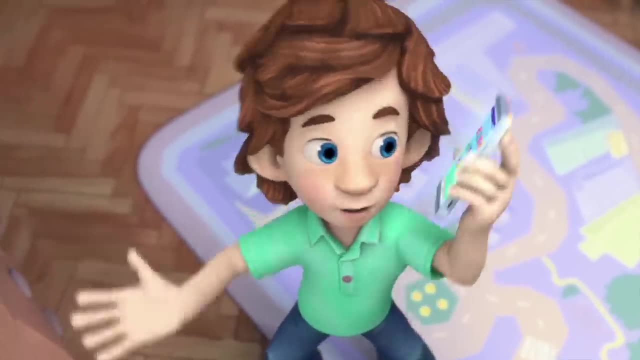 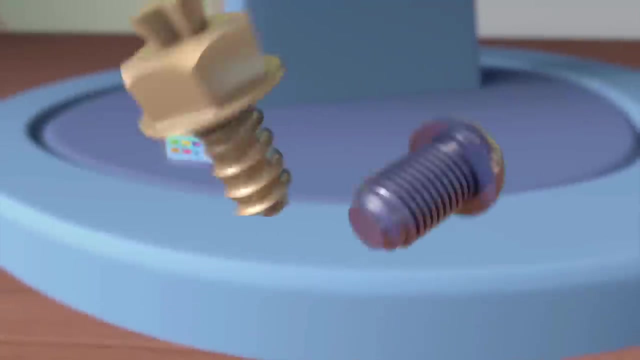 We finished Piddies. Look, it's a Surprise. Wow, this is great. Now I've got my own fixie phone. It's just like you've got Well pretty close, Tom Thomas. Tom Thomas, let me use your phone to call myself. 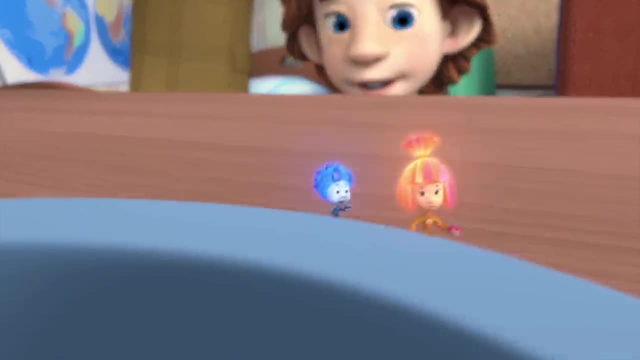 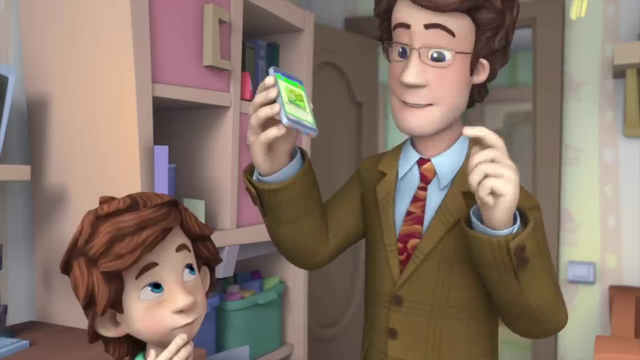 I need to find my phone. Oh wow, you've changed everything in here. Where am I? I guess I'm Papus. Ha, what a funny name you came up with for me. I'm Papus, And this is what you came up with for me. 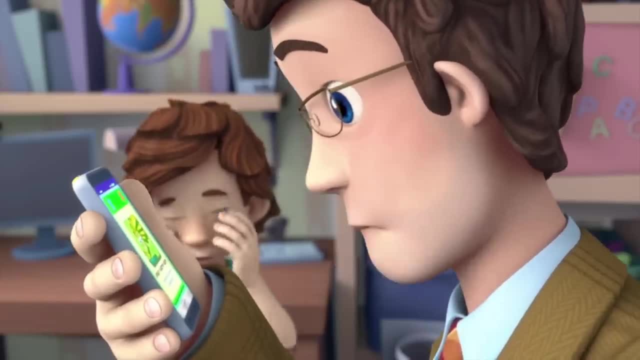 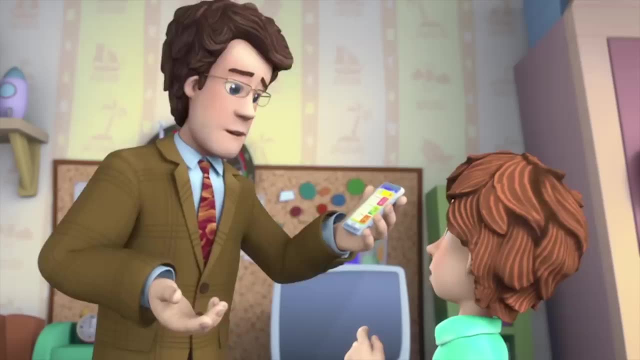 Nolik, just stop, I don't have time for your fooling around. What? Who is that? That's? uh, not Nolik, Who is this? Do you know who I just called? Does anyone know who this phone belongs to? out here. 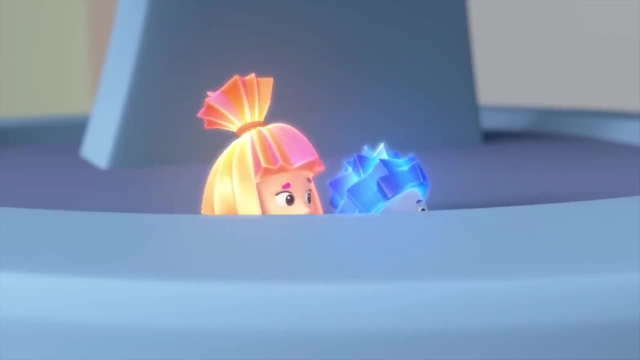 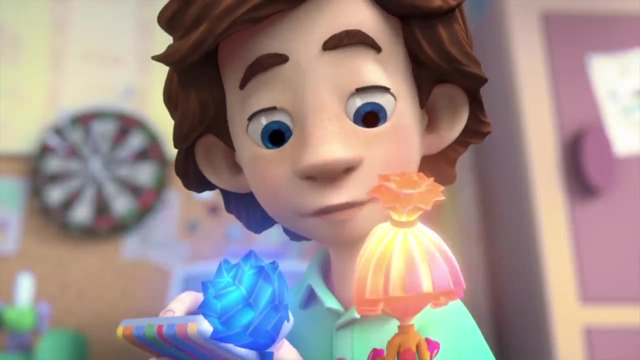 Ugh, your mother found it. I'm coming. We'll fix those numbers later. Pappus is going to really give it to us. Give me your phone, Tom Thomas, and I'll delete all the Fixies' numbers from it. 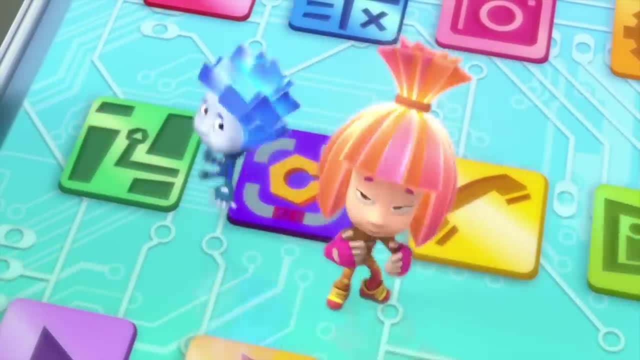 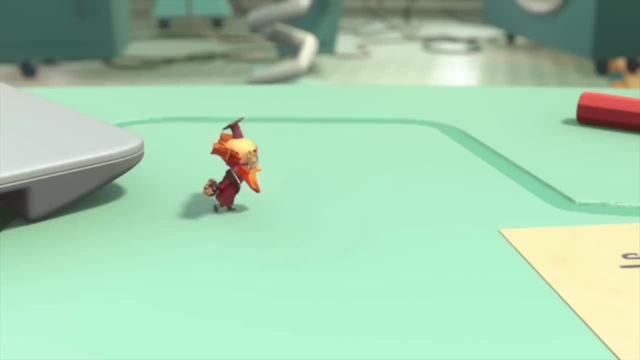 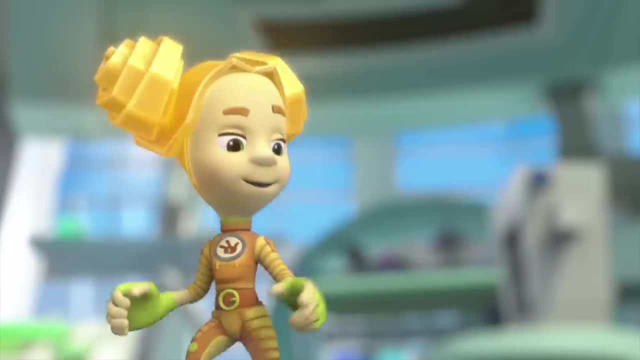 But how can I call you up then? Why would you have to call us? We're always close by The Suction Cup. Where's Professor Eugenius? Did you see him? Not yet Strange. He told me he'd be here today to conduct some tests. 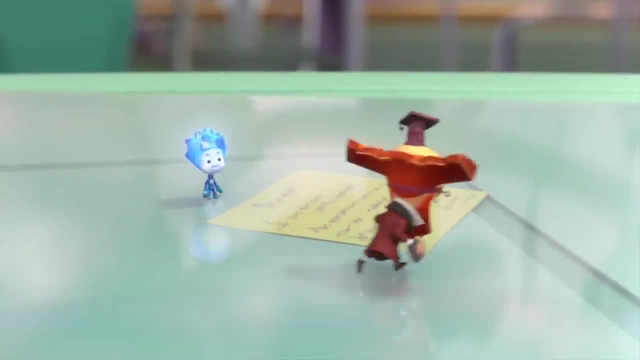 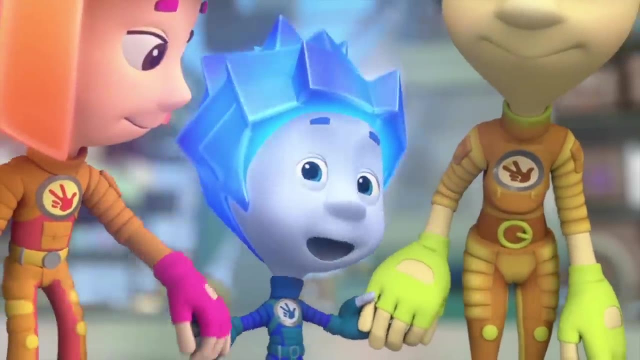 Rampus, right here under the glass, there's a note. Dear friends, That means the note's for us. That's because Professor Eugenius can always count on us. I'm off for a conference today, So what should we do? 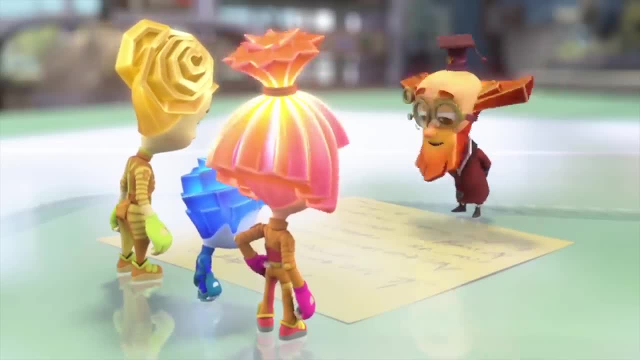 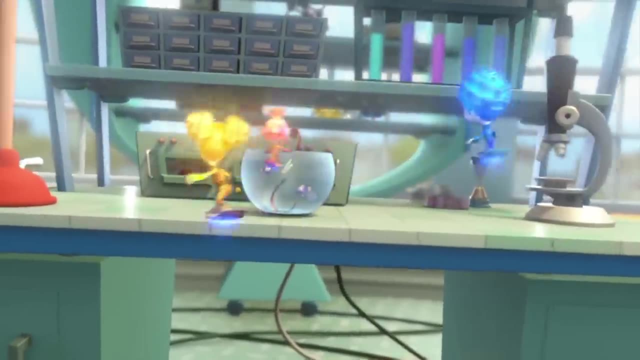 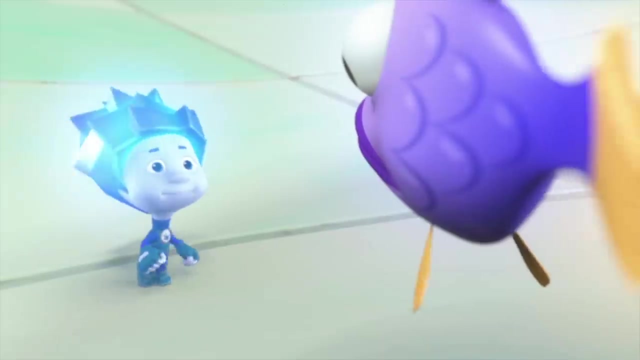 While I'm away. please keep an eye on each of my tests. There's the wristwatch, And where is it? It's right there. Look How come the watch is in the water, So the fish can know what time it is. 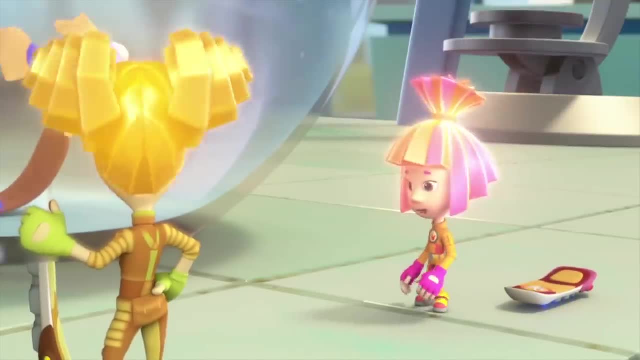 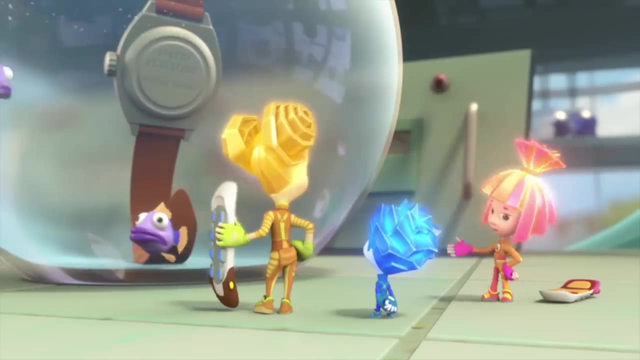 Nolik, don't be silly. This is the test he made for the watch. You see, It says water resistant right there on the back. That means that water shouldn't get inside of it, I see. So the professor needs to check if it will work under water. 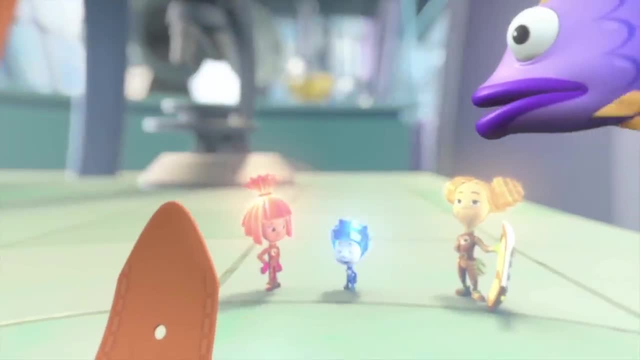 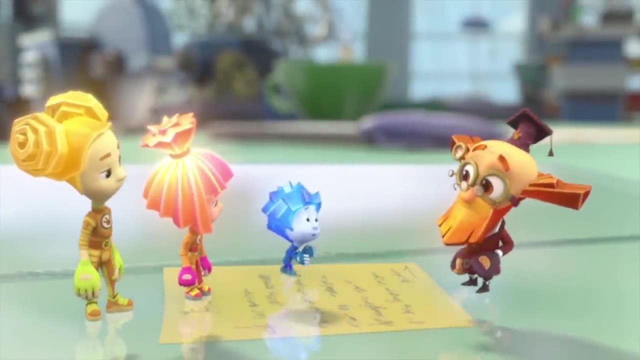 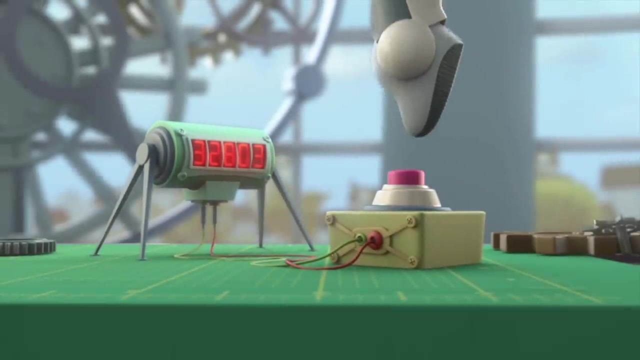 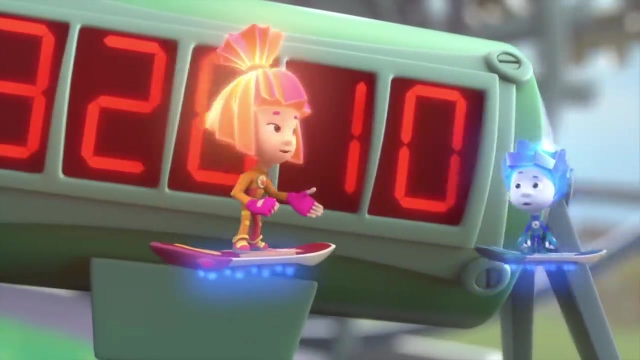 Understand. Yep, I got it. The watch is in the water. What Is working? So now the doorbell test. We'll go look It's over there. What's that thing doing? It tests the button to see how fast it wears out. 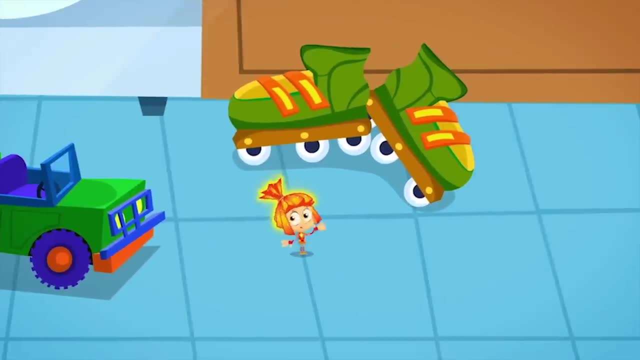 To check the quality of appliances, toys, sporting goods or just about anything, they need to undergo serious testing. Take, for instance, telephones. They need to be tested with both heat and cold because they have to work in places as hot as Africa and as cold as the Arctic. 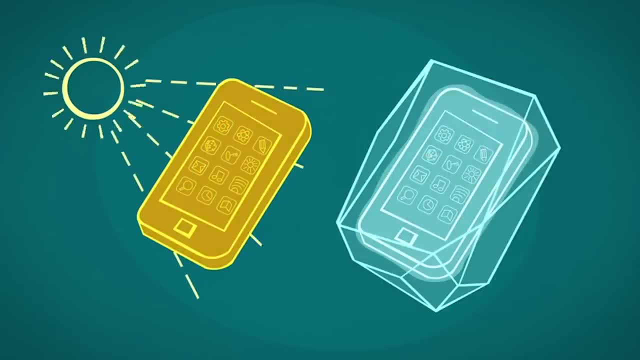 Computers are tested to make sure they can be shaken and rocked too. That way you can be sure they'll work on a desk at home or outside, in the parks or while you're taking a ride. Different kinds of products need different kinds of durability tests. 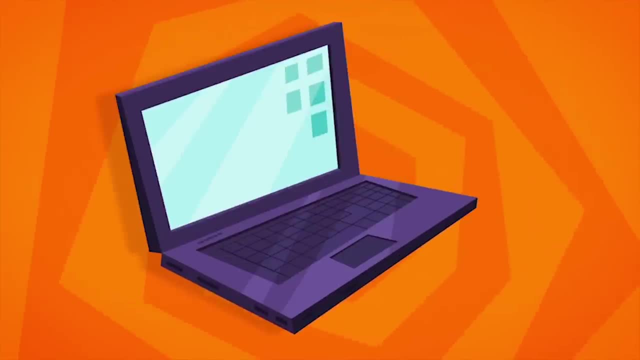 For example, athletic shoes and car tires are rubbed and squeezed on the back of the car And the back of the car is also rubbed. So what's the difference? The back of the car is rubbed, The back of the car is rubbed. 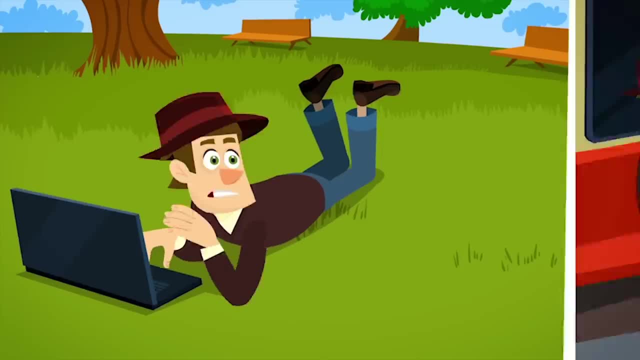 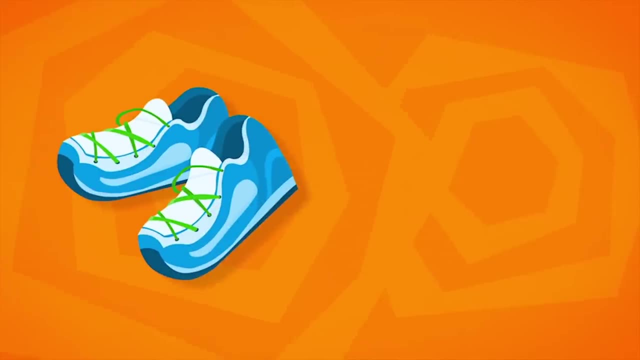 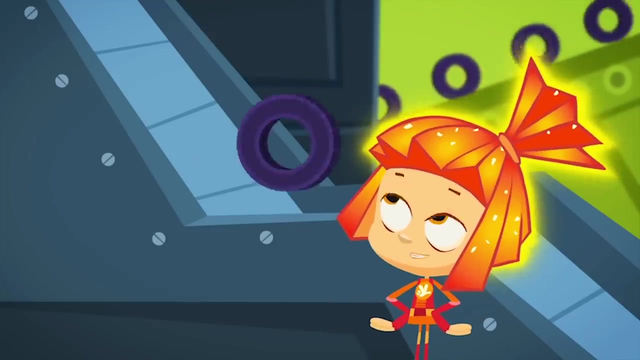 And the back of the car is rubbed. So what's the difference- The back of the car is rubbed And the back of the car is rubbed- And how long they are going to last? Yes, testing is very important Without testing a machine or appliance. 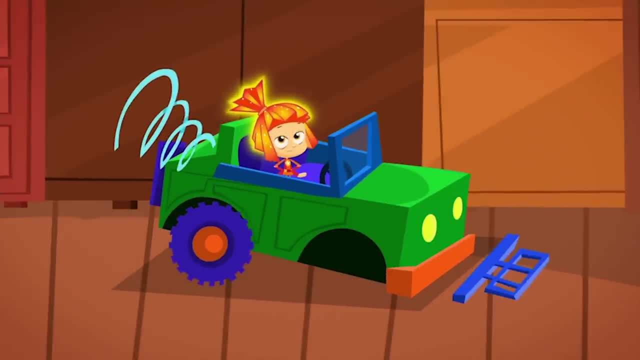 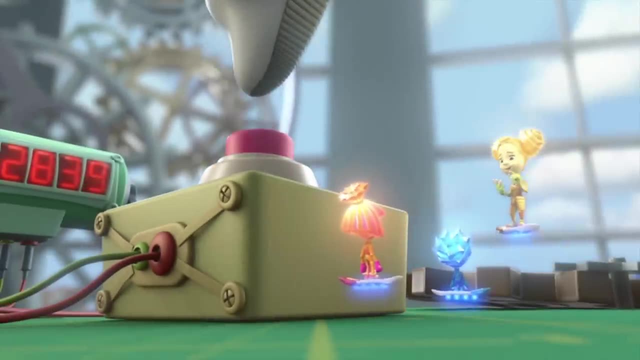 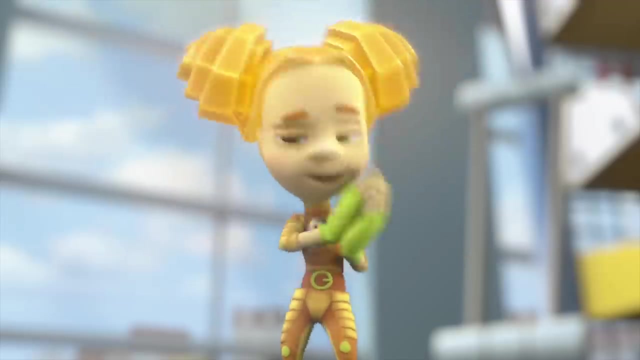 will let you down at the very worst moment. If guests come to visit once a week and once every month When the hooligan comes, pushes the doorbell and runs, then I figure this doorbell will last right around 400 years That long. 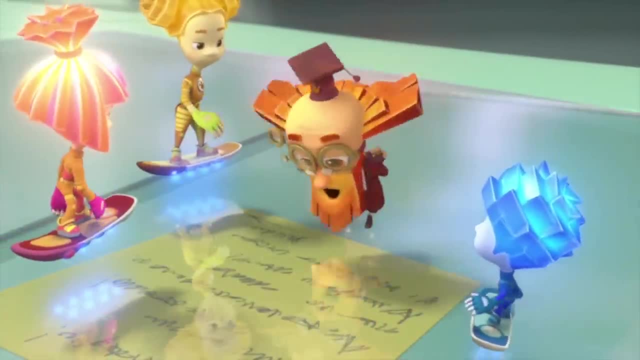 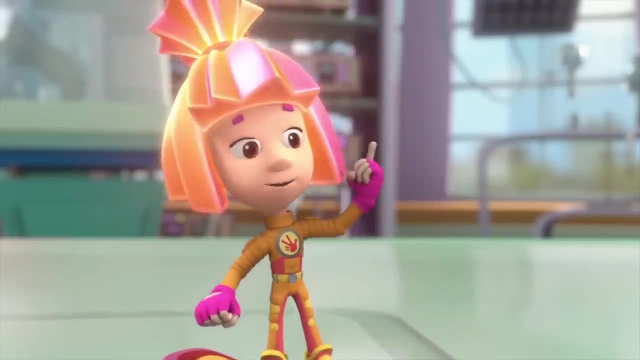 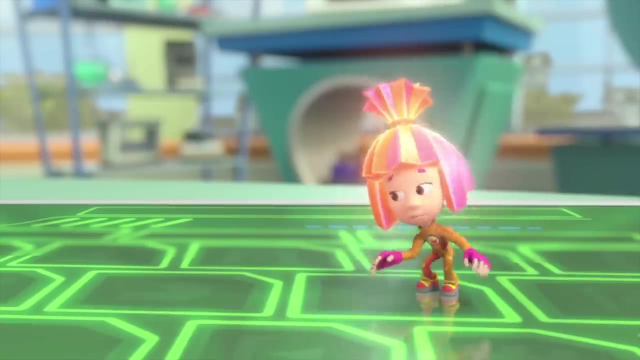 The doorbell is still working. That's very good. And also… What I don't know. We need to turn the note over to read the end. But how, Oh, raise the glass. that's all Uh-huh. 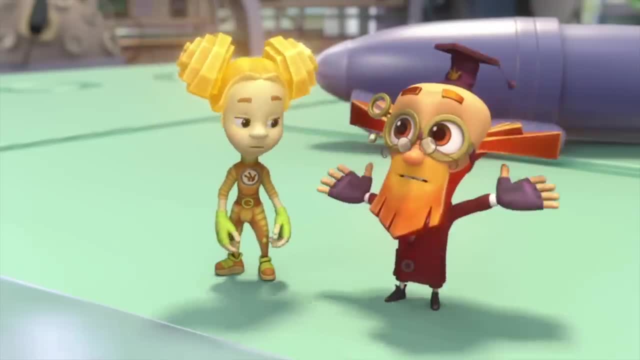 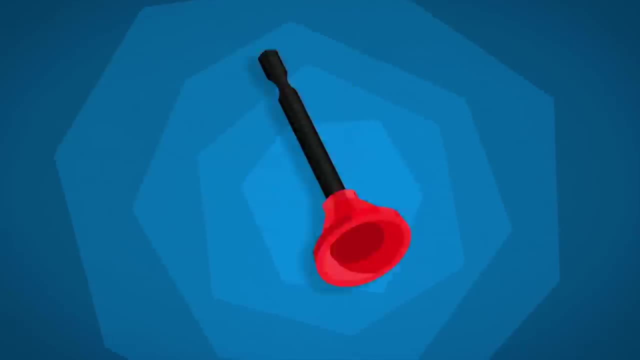 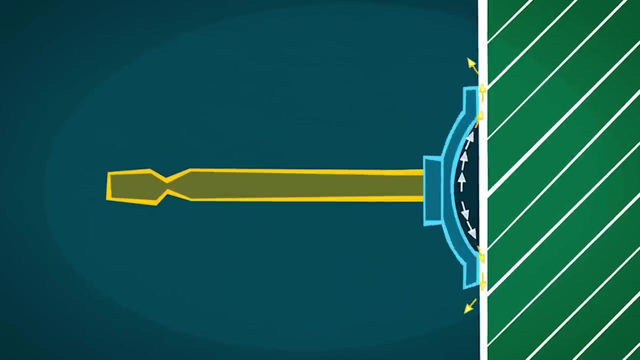 I can't get a hold of it. We should find a suction cup. A suction cup. Suction cups are made out of rubber or other elastic materials. When a suction cup is pressed against a smooth surface, the air inside is squeezed out. 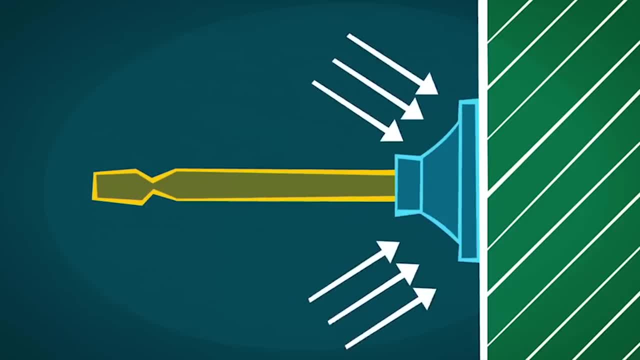 The air outside wants to get back in, and so it pushes down on the cup. The rubber inside is pressed against the smooth surface, and so the rubber inside is pressed against the smooth surface, and so the rubber inside is pressed against the smooth surface. 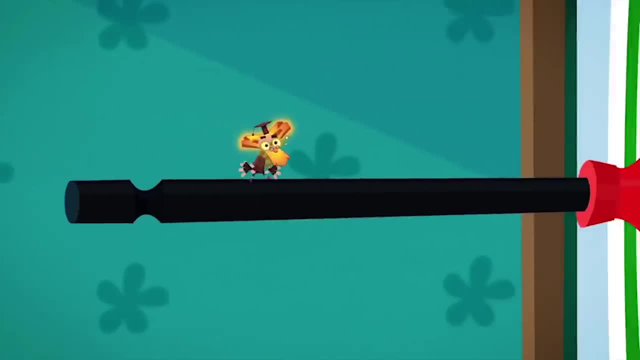 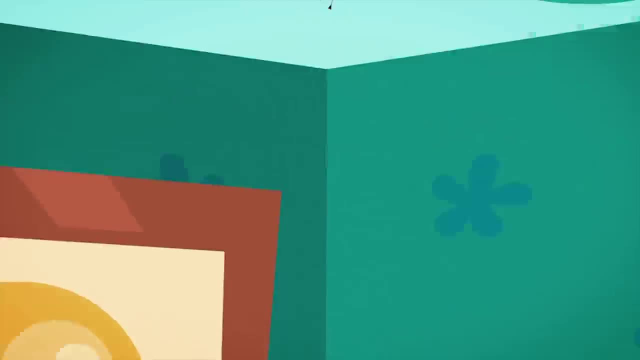 and the rubber edge of the cup won't let the air leak in, So the outside air keeps pressing down and the cup keeps on sticking. And that's how a suction cup sticks to a surface: by using the power of air. Wait a minute. 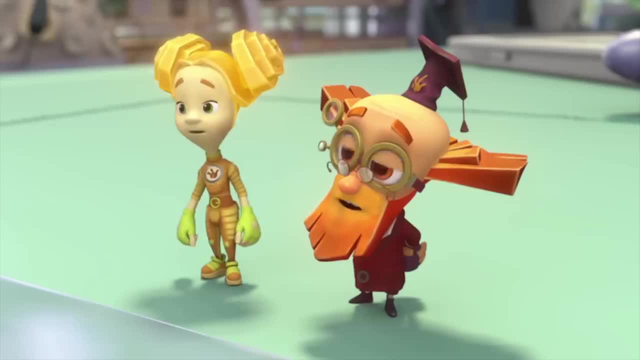 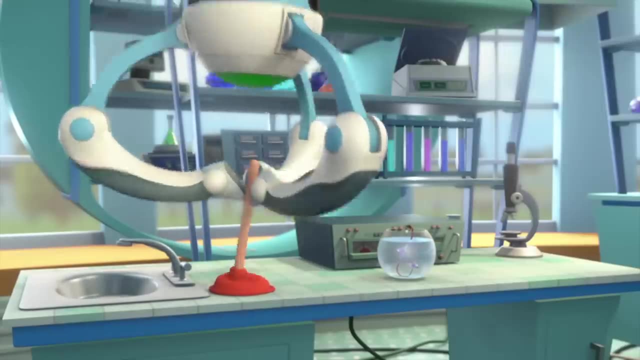 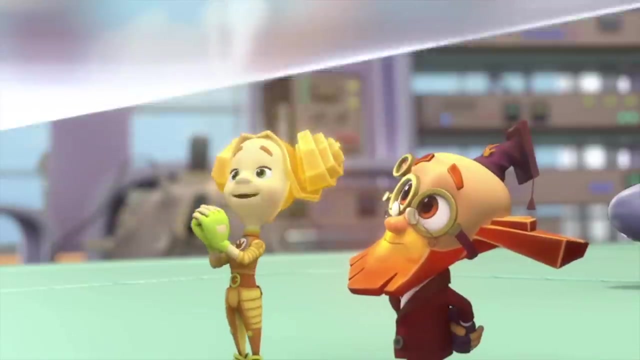 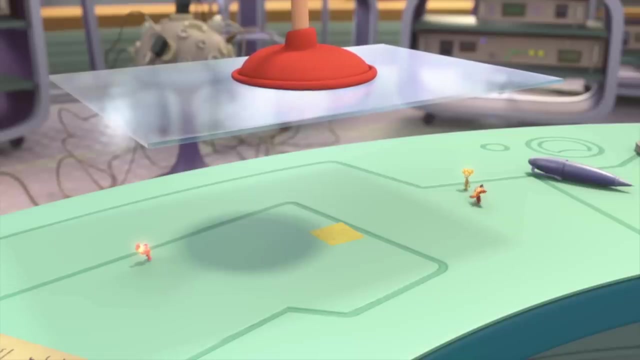 I know where there's a really big suction cup that we could use. That's a huge suction cup, Nolik, Tideesh, Tideesh, Tideesh. Well done, Nolik. Only we need to hurry before air gets under this suction cup and it unsticks. 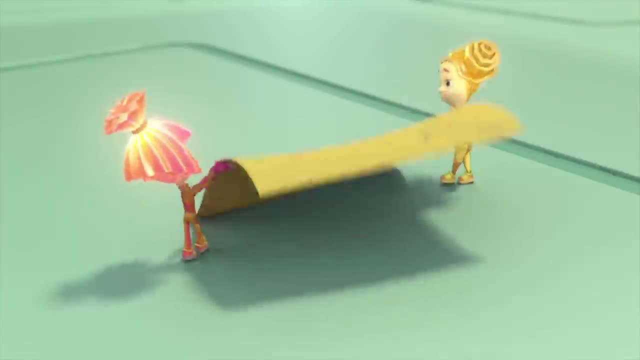 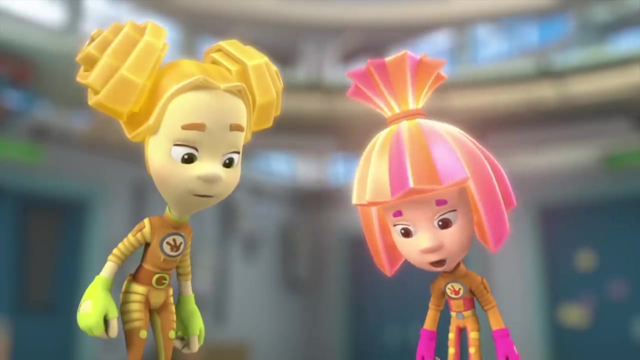 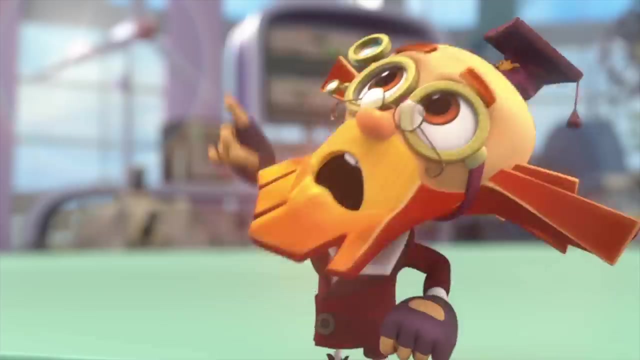 My suction cup will never unstick. Well, let's see what it says here. Zipka, you'd better hurry And make sure nothing gets broken here in the laboratory while I'm away. Huh, and what could get broken around here? 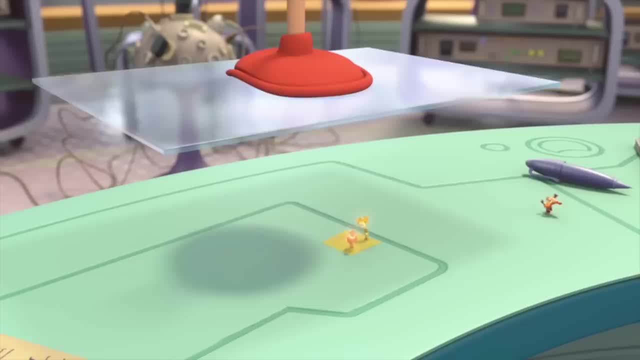 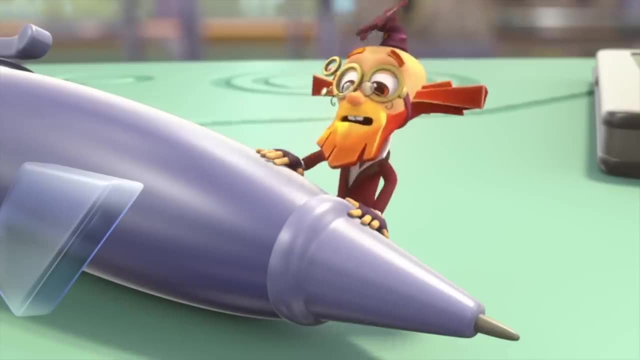 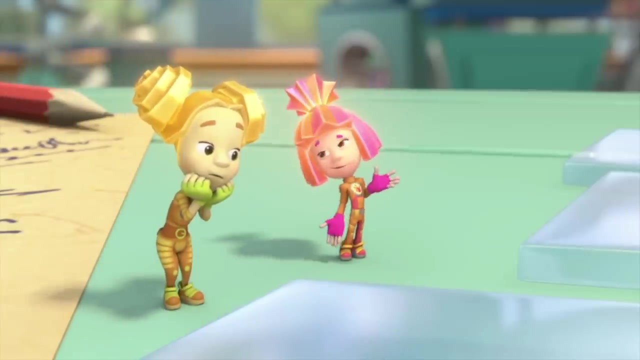 Ah, The glass Look out. Yeah, so much for that. And who's going to clean up all this broken glass? You don't know. Nolik, He told us to use that suction cup. No, Zimka, She was reading way too slow. 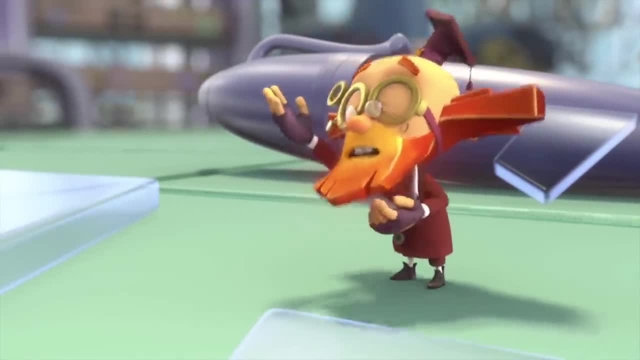 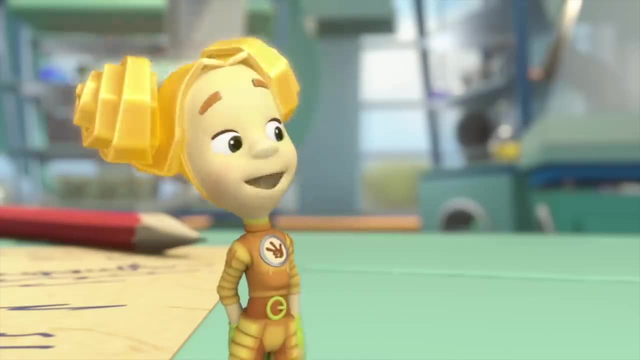 Listen, there's no need to fight. I came up with the idea of the suction cup. I should clean this. Come on now, Grampus, We'll clean up this mess. Professor, I still think the suction cup was a great idea. 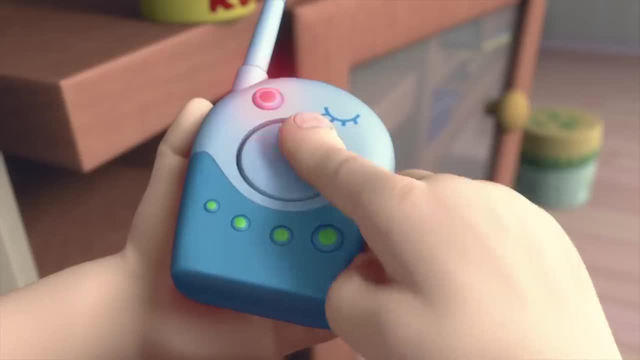 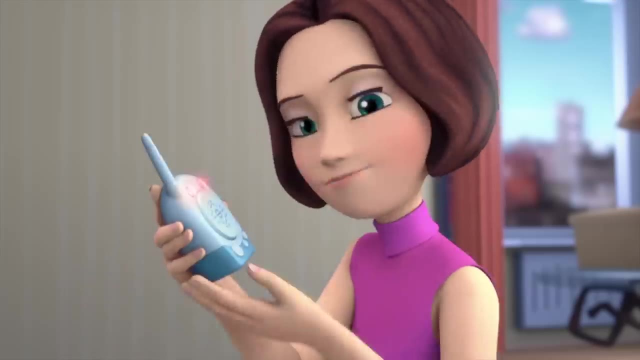 Oh, It's my old baby monitor On Check, check, Checking One, two, three Checking. It's working. Why don't we give it to the Johnsons? They just had a baby the other day. Uh-uh, This is mine. 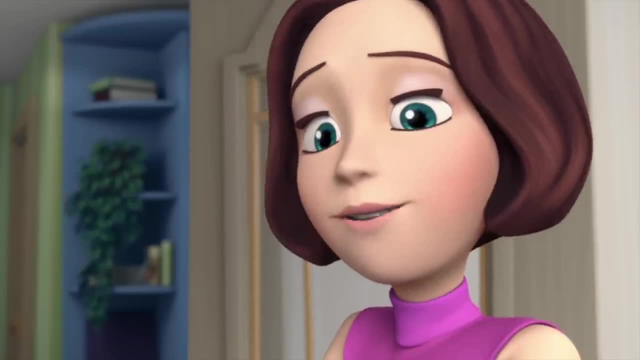 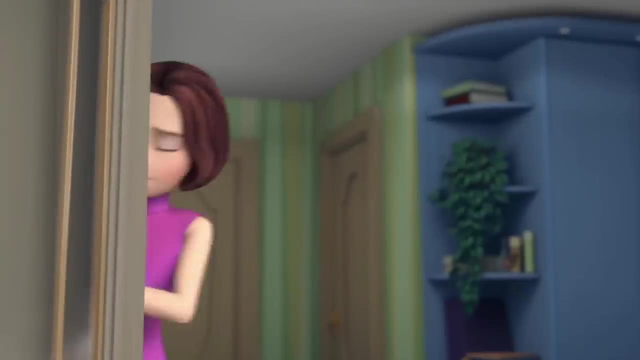 And I'm planning on using it. Aren't you a little too big for it? No, I'm not big at all. Well, I didn't realize that you're still a little boy, And a greedy one at that. They're never going to notice this. 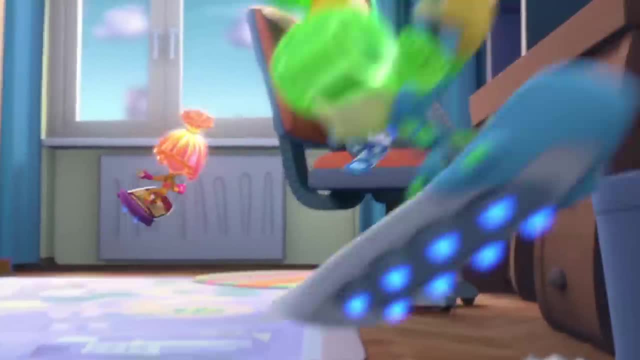 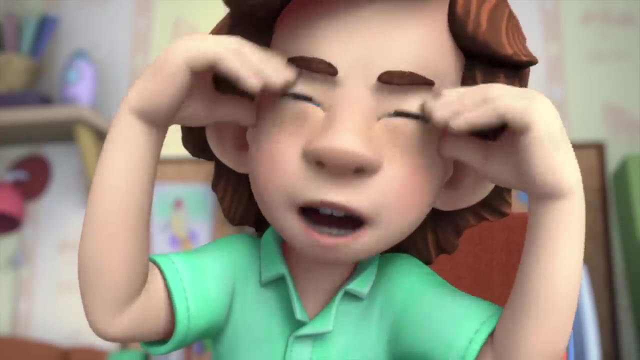 Hey, Fixies, are you here? We're here now. Why did you call us? I've got to show you how I turned into a baby To a mind reader. I find that just a little hard to believe. OK, then I'll show you. 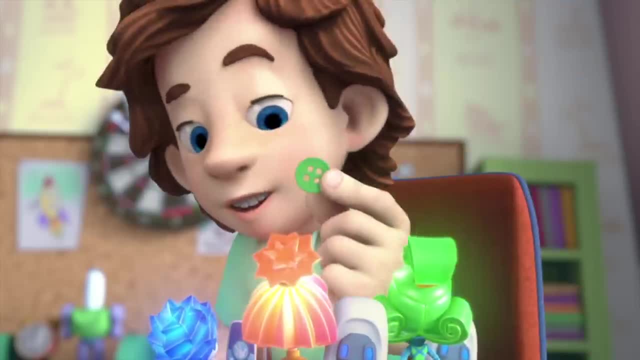 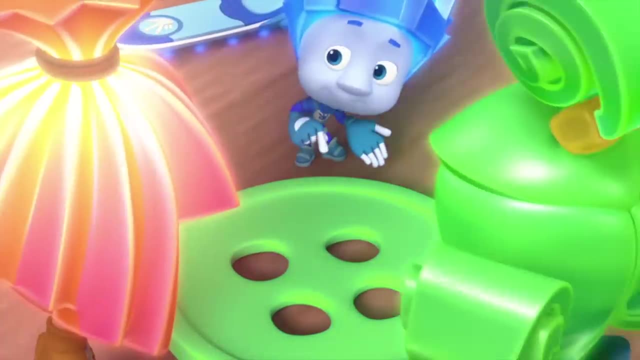 I'll leave you alone and then you'll hide this button wherever you want. Then I'll come back and find it. You got it, So where's a good hiding place? Well, we've got to think of one Right here under the keyboard. 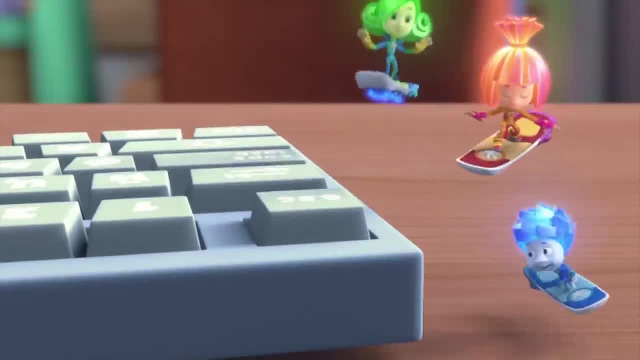 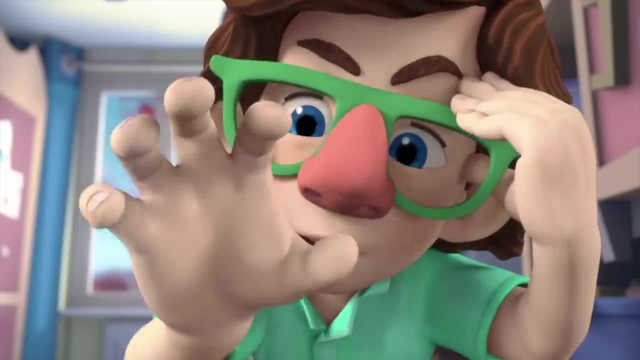 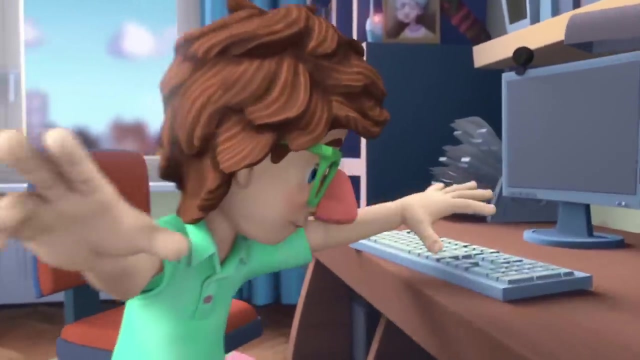 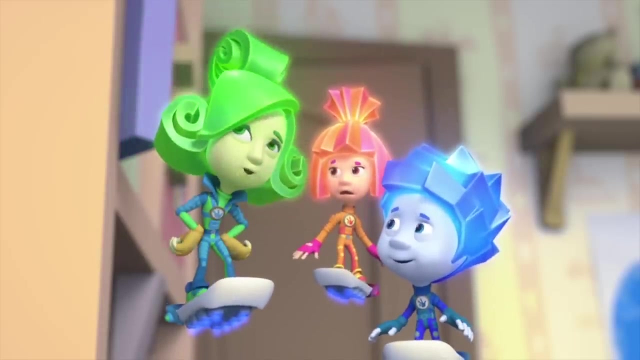 Great, Go on, Nolik, Come on in, We're ready for you. And now I'm going to read your thoughts. Here I go. You hit the button here. Look, Ta-da, He really does read minds. Oh, that was a lucky guess. Bet you can't do it again. 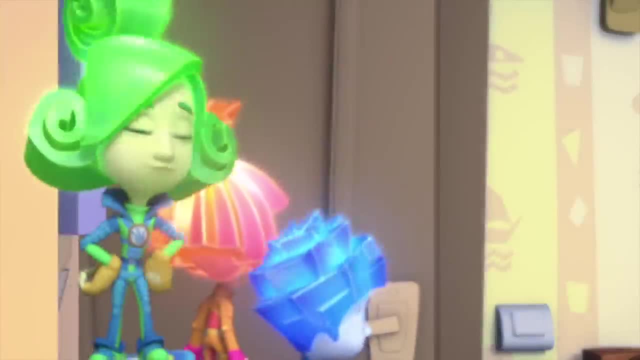 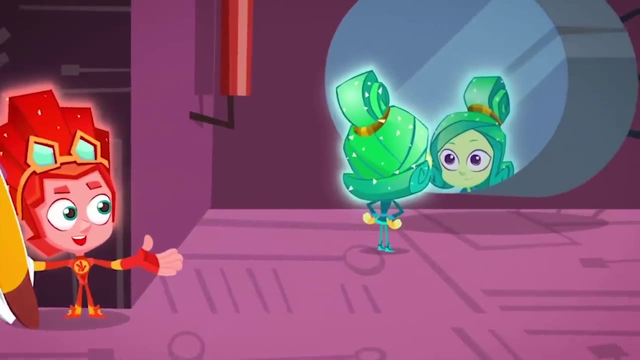 Well, I bet you I can. We're going to have to be sneakier. Verda, She's the most beautiful girl in our world. In our class She knows it too And doesn't hesitate to use it. She can even be a bit sneaky. 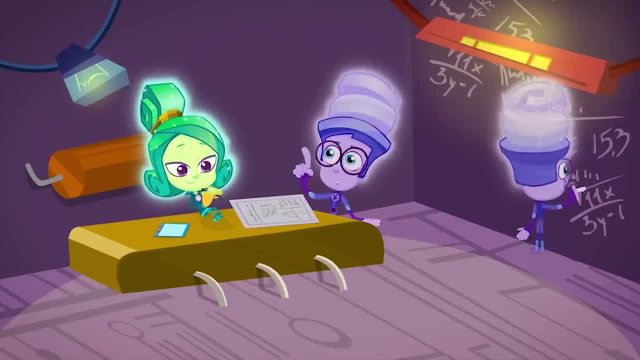 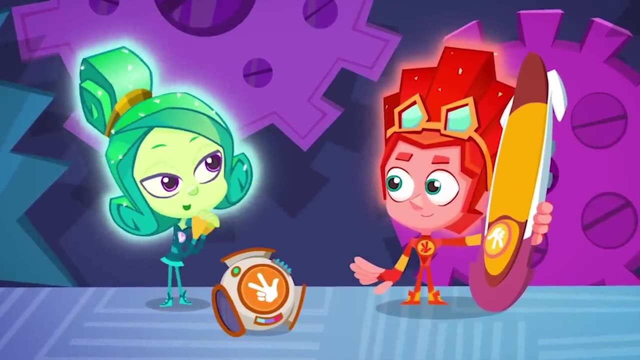 Like when she needs help with her homework. then Digit suddenly becomes her best friend. But if she doesn't want to carry her pack-o-mat, she'll say Fire, please help me. You're just such a strong fixie. But all us boys like her just the same. 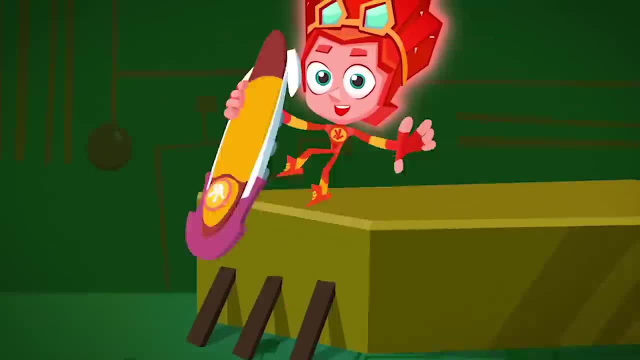 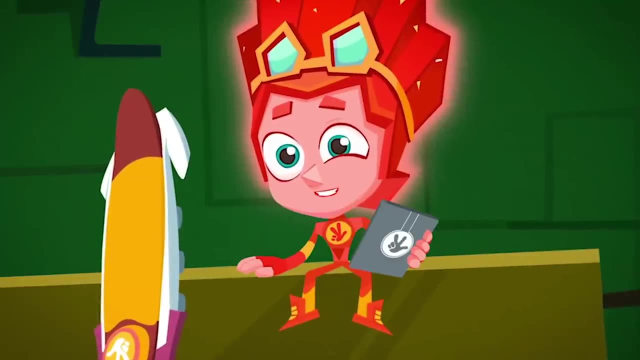 Digit does and Nolik does, and I guess I do too, Although I really like Simka more, Or maybe Verda does, Or both of them, I haven't decided yet. Verda can be difficult and even bossy sometimes. 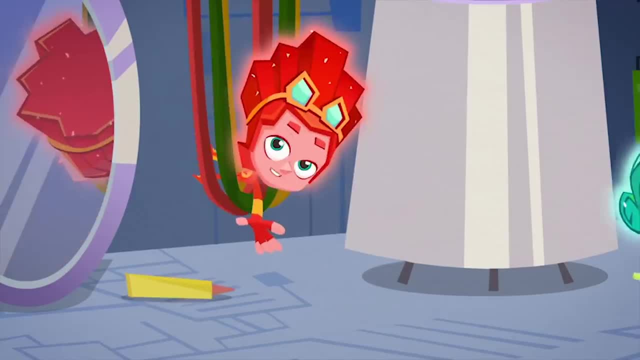 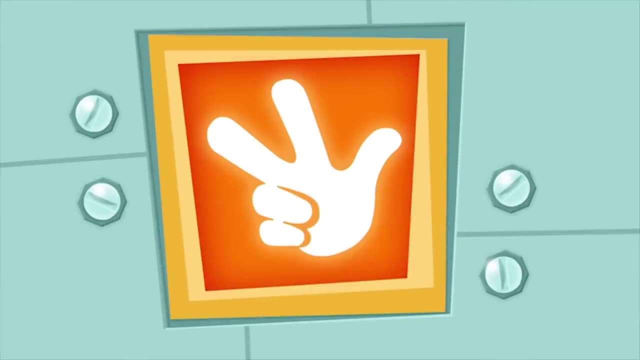 But one thing I know for sure: Verda's a good friend, A friend that will always come help. Well, that is if she's able to pry herself away from the mirror. I think that we should throw it down into this pencil cup. 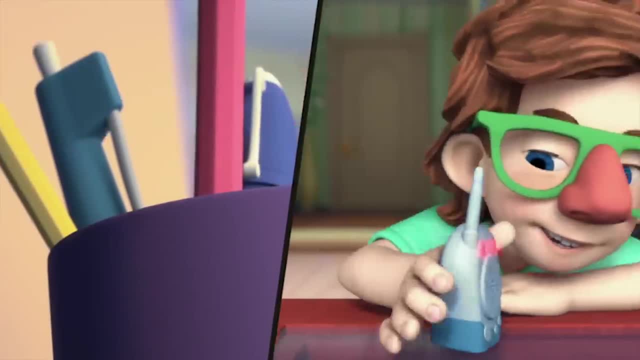 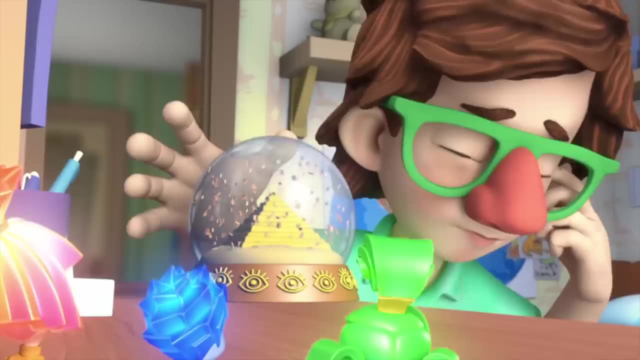 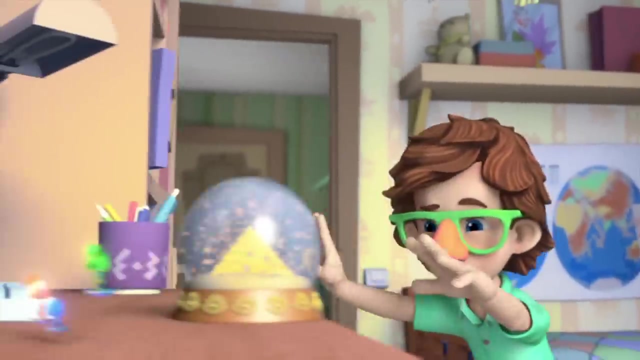 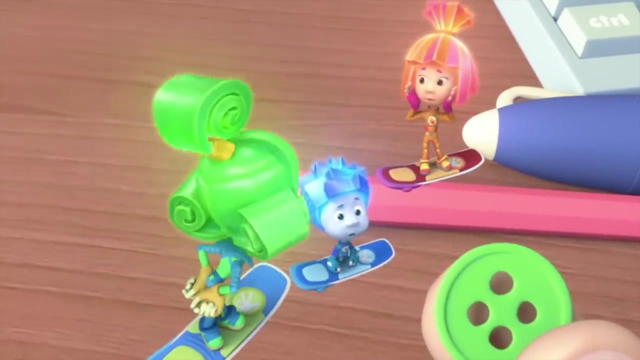 But then we concentrate on another place. That is good, but it won't work. Fixies, Come on in, Okay, Uh-huh, Hmmm, Ah-hah, It's in here. Tideesh Simka, were you thinking about the cup? 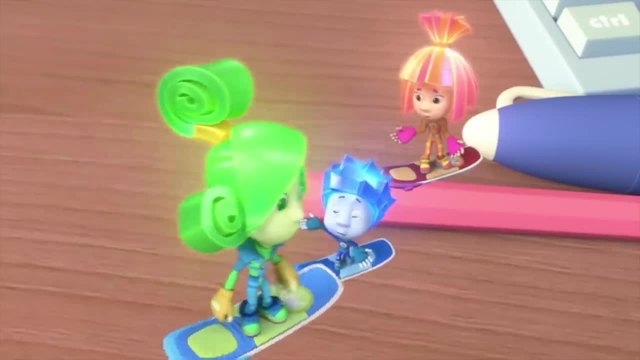 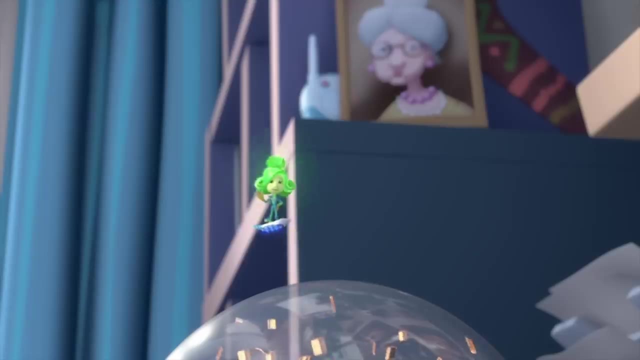 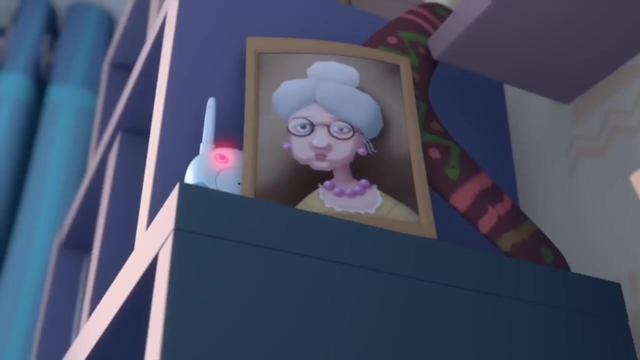 No, I swear, And my mind was blank. Then who did? huh, Who, Uh-huh? Tom Thomas, What do you say? we go again As many times as you want. Shhh, I know how he's been doing all of this. 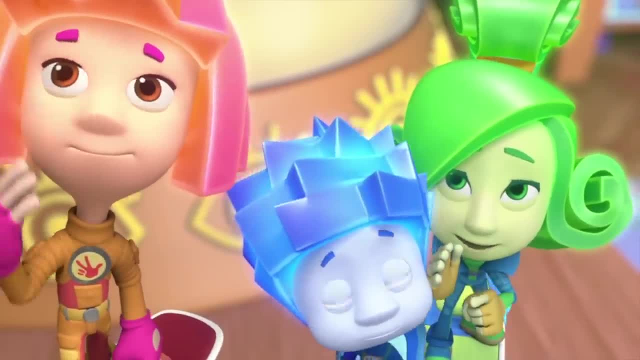 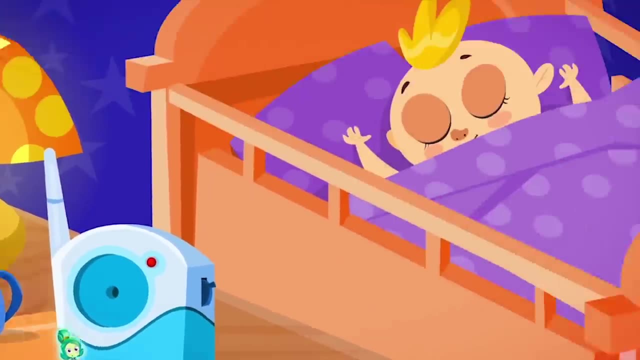 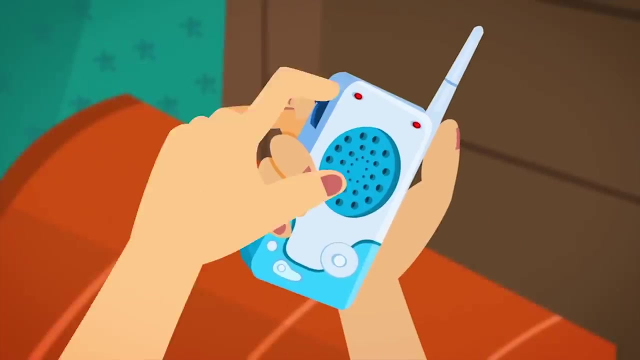 It's a baby monitor. That's how he can hear what we're saying. I don't get it. A baby monitor helps parents watch over their babies. The system has two units that look like wireless telephones. The parents keep one of the units by their side. 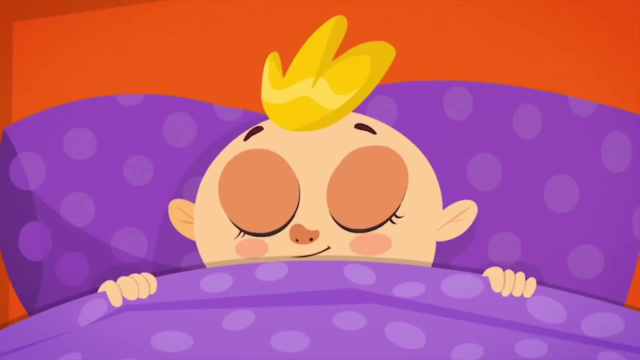 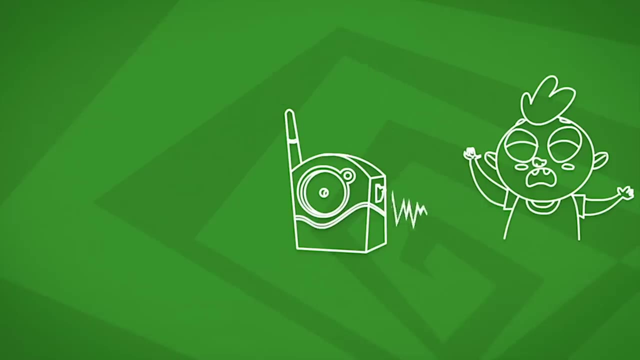 and put the other one in the room where the baby is sleeping. If the baby suddenly wakes up and starts crying, the unit in the baby's room will pick up the sound and send it by radio waves to the parents' unit. Mom or Dad will hear the crying and go and comfort their child. 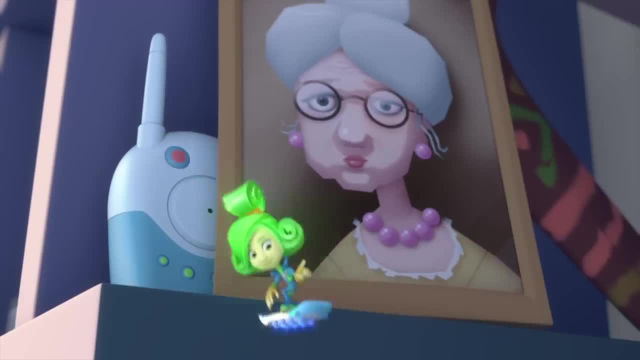 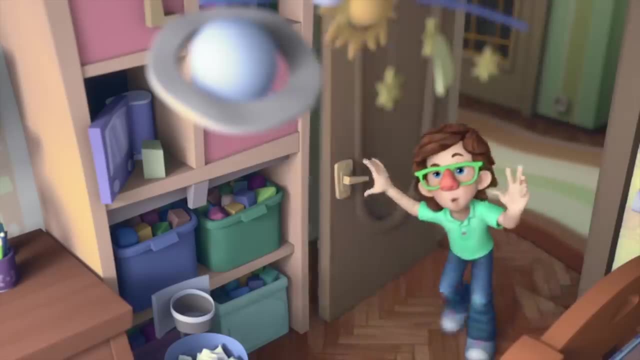 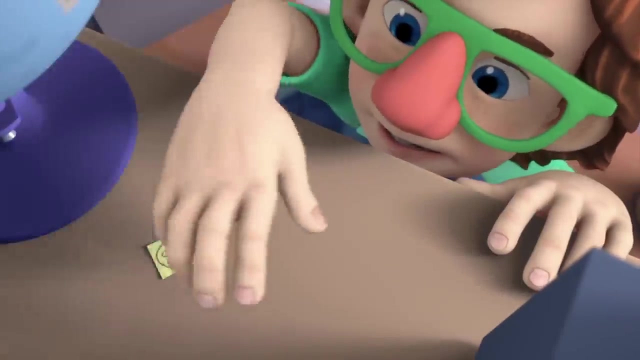 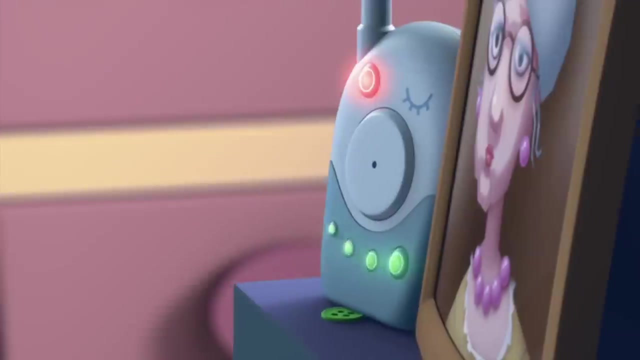 And so he's listening to us now. Shhh, This time I know what we should do: We'll hide it under the globe. Go on, Hmmmm… Uh-huh… Ah-hah, Huh, Where is it? If you read our minds, you'd find your button under the baby monitor. 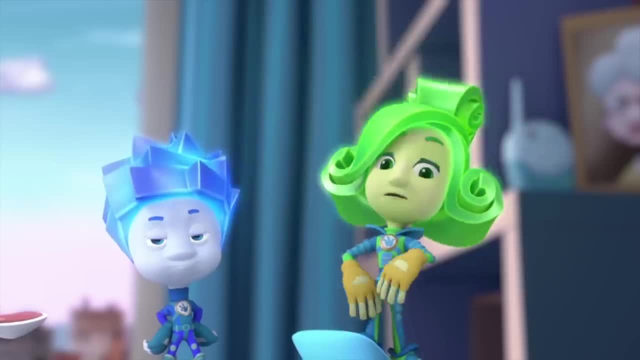 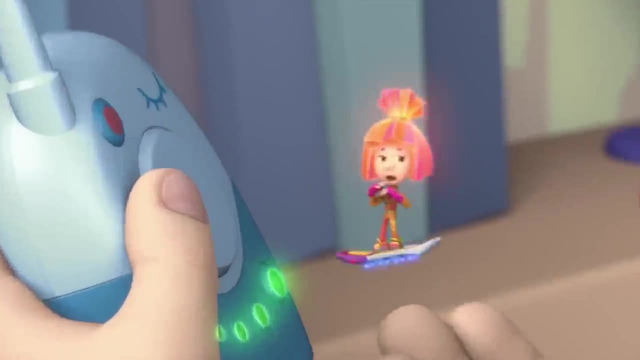 You tricked me. That's really not nice. And spying on us is nice. you think I'm sorry. I just thought it'd be fun. Well, anyhow, Tom Thomas, you're too old for this thing, Unless, of course, you still need it. 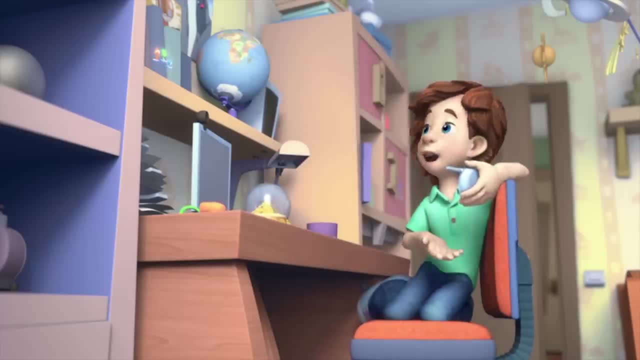 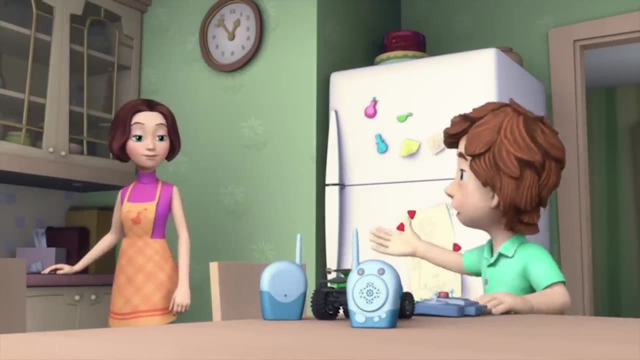 I'm not a baby, I was just, you know… checking it. I'll go and give it to Mom. Mom, I'm not greedy About what. Let's give this monitor to the Johnsons and this car is for their baby boy.